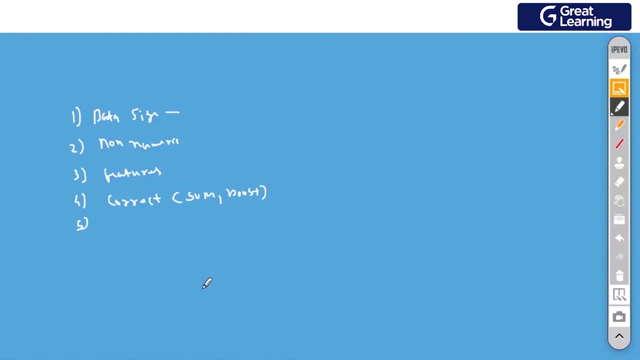 two. Yeah, They have a capacity to learn. Yeah. So this is one issue. Our ML is, you know, an algorithm which we have to train and then we can use it. It does not have auto-healing or auto-correction. 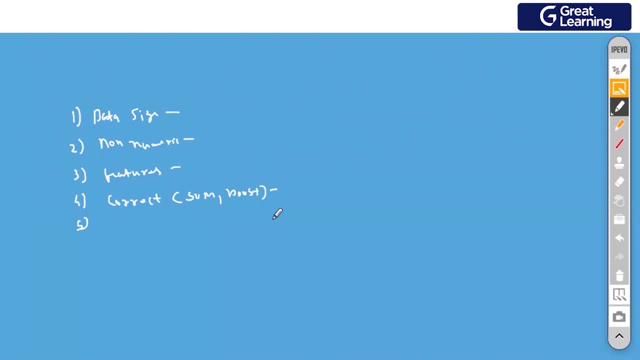 system Right. And fifth one I will say is: somebody already featured non-numeric data, So I will say what, if you want to- And that was you- can use that, Okay. Finally, what I have made it clear to me is that you know. 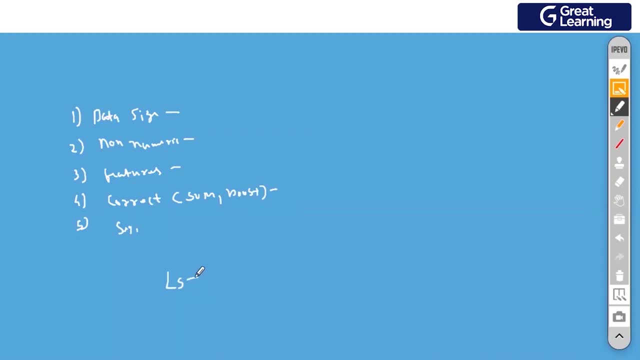 you have to have a specific model of the same as the one that we are now Exactly So like. if we want to do that, it must have to have a specific model. So if we do that, we can do that. 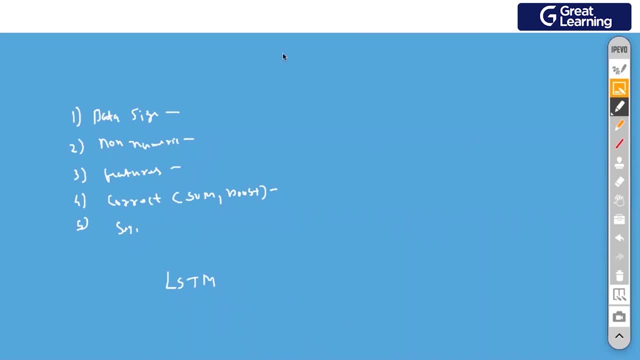 We can use that, So now we can. I think a lot of people use LSTMs. This is a good question. I will explain it in a few. So this is how I use LSTMs. Okay, So I have a few. 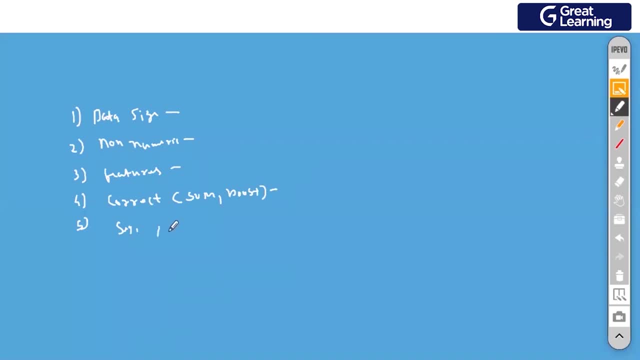 Okay, So I have a few LSTMs I know of, So let's see what that means. So this is how I use it. Let's see how I use it. This is how I use it. Okay, I cannot say this is a sequential data Sequence in the sense I showed you people, Arima, for example, time series forecasting. That was a sequential stuff. Sequence means what happened some 10 years back. there is chances that at the same month or same time the same thing might happen. the seasonality part of it. 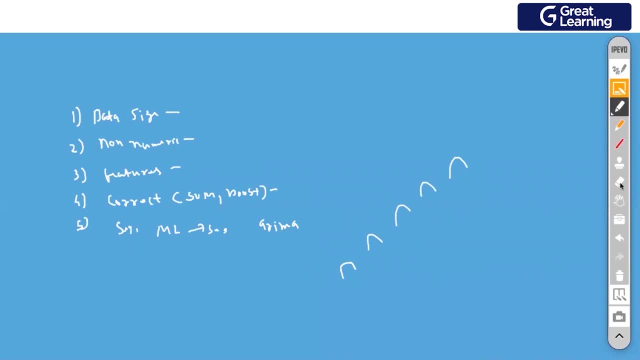 What if I want to take care of something like this onto machine learning? Sometimes it is not possible to do it And there are hundreds of more reasons. So I will say: for our cause, the best reason could be non-numeric data. What do you mean by non-numeric data? Say pictures, say text, say voice. We cannot process it. Up to some point we can process using machine learning. After that we have a limitation here. 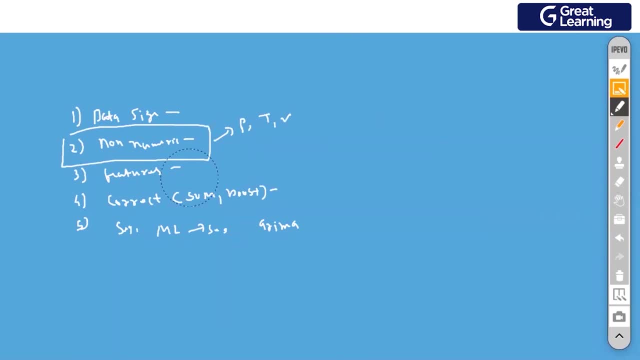 All right. So now what I'm going to do is let's try to build some algorithm into machine learning. See also, one more thing is, even though in our course we say machine learning is over, but actually machine learning is the whole box under which you have two parts or three parts here, which we call it supervised learning, unsupervised learning, reinforcement learning. After that we have something called artificial intelligence, And then I will say some mixed bias. 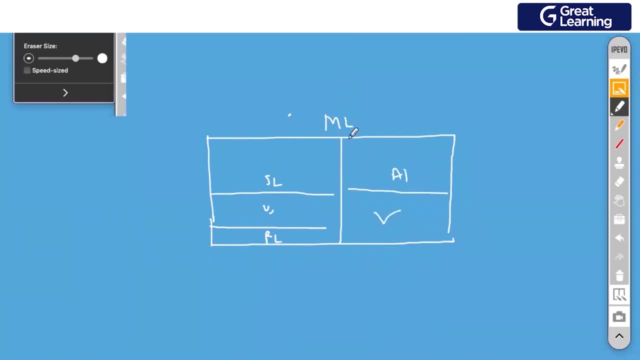 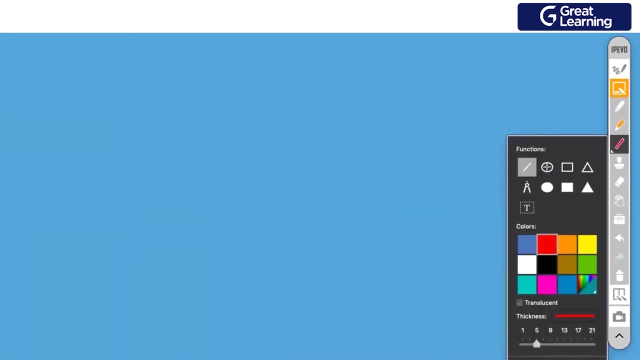 Yes, So still, it's a part of ML only. But from now what we are going to do is say I have a box, I will not say what it is. We have some empty box here And I'm giving some input to that box. Yeah, So let us say my input is defined like this: Now, when I give an input to this, I'm expecting a certain output. So before I get an output, I have some expectations. Let us say my input is: 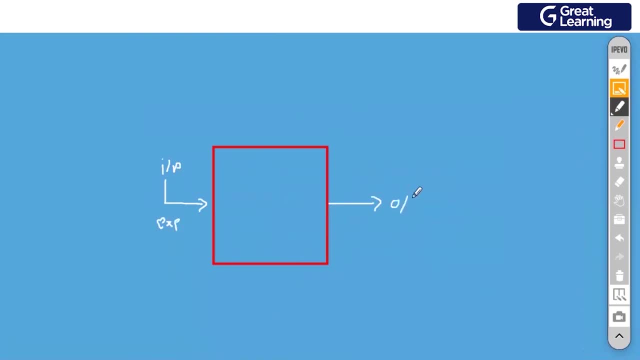 expectations are exp. i am getting an output here. i'll say expected output, otherwise we'll get confused. now what we are going to do is we are going to analyze this output. is it as per our expectation or not? so how do we analyze? let us say we analyze using a function. i will use a function. 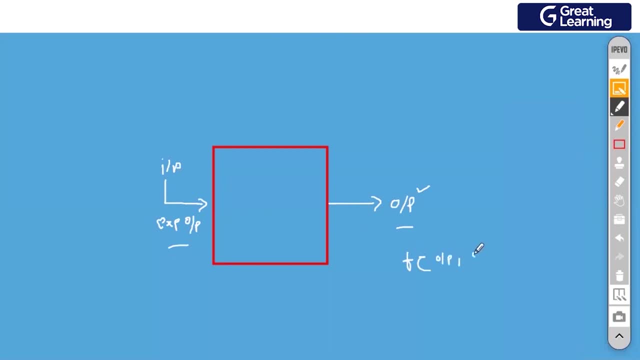 basically to operate on our output versus expected output. all right now, if this function is of certain value, let us say the two values can be good. another one value could be bad. let us say: if the function is in bad value, what are we going to do? we are going to go back and make some. 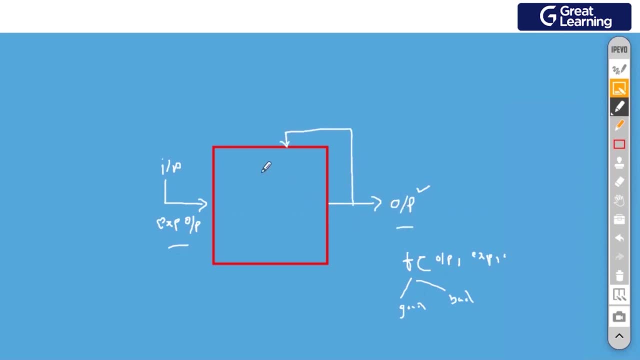 corrections to this box. now, what made this output bad? can i say this particular box made it bad. it bad because of this box. we are getting some unwanted junk over here. agreed everybody? yes, so what is our duty back? go back and try to fix it. you keep doing this till we come to the phase. 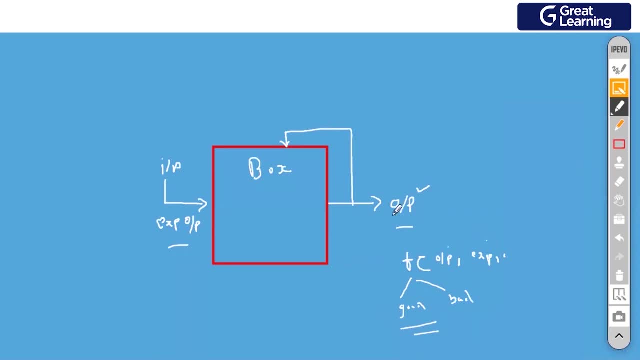 which we say, good, we will come to this. what are these things? but till we find that this and this is matching, i keep reading this. this is what is an example of a neural network, a very simplistic approach, all right. any issues into this? no, no, okay, now there are two, two parts that you people 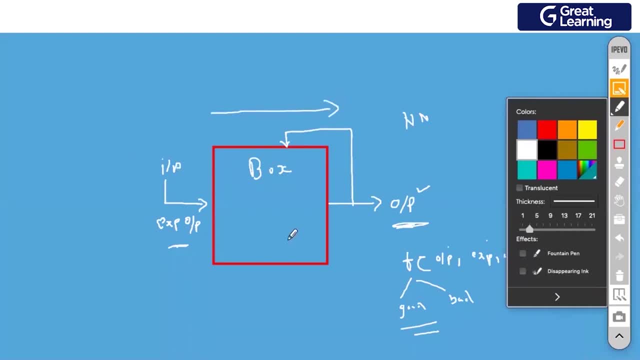 observed here. one path was called forward path. forward path was where i gave my inputs and this box amplified it or de-amplified it. we don't know if the box made some changes on it and gave us an output. this is called forward propagation. now, since we found out that this 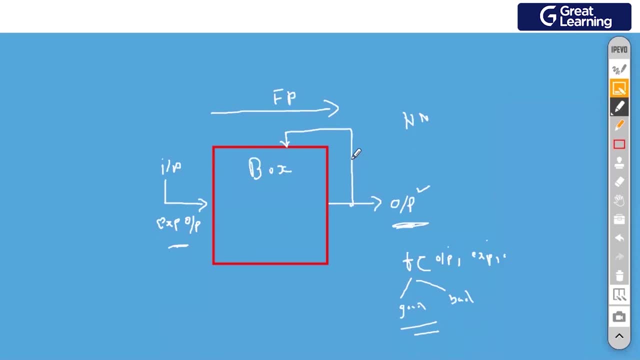 function is of not a good value. we went back and we corrected our box. this is called back propagation- as simple as this. all right, so these are the most important parts within your neural network to understand that we will give some input, we'll get some output and we'll keep training it. 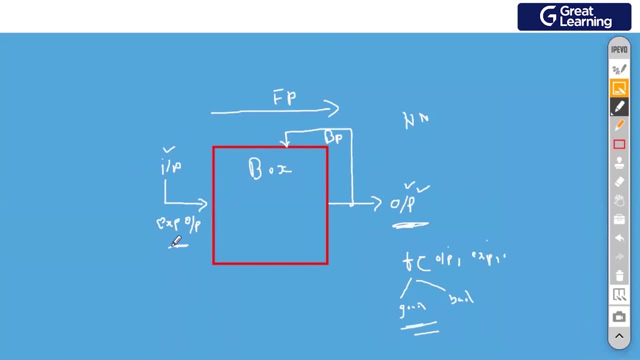 till we are satisfied that, yes, we are getting expected output out of it. okay, one more example. i usually give this very silly example. let us say: um, this is a kid, for example. okay, and you are teaching some tables to the kid. say: you have taught five tables, yeah, so by giving input the kid is learning, yeah, so you? 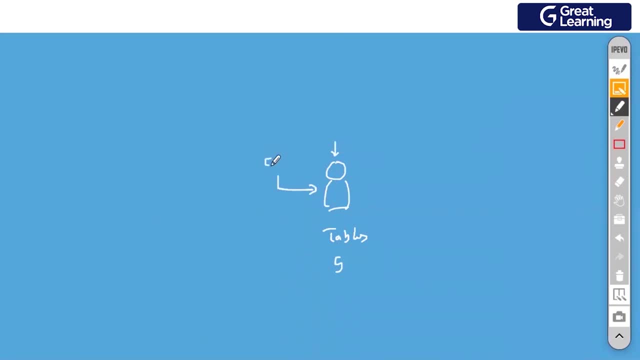 made. you did something such a way that the kid knows the table. now you asked the kid: five, five, for example. the kid says five, fives are 32.. so what do we do? immediately? we go and correct. we keep doing it till the kid comes and says five, fives are 25.. this is also another example of 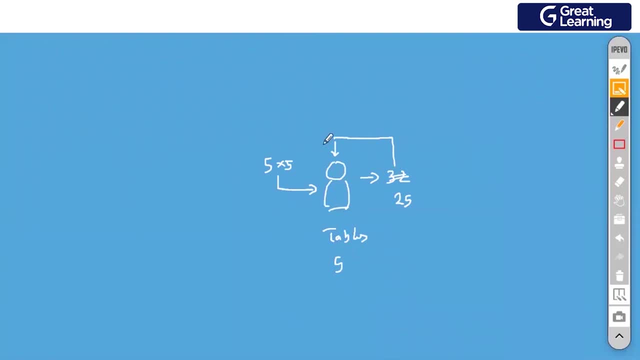 neural network- forward prop and a backward prop to correct it, and keep doing it till you are happy with the answer. okay, now let's talk about that box that we were talking about. now. what exactly is this box? so just give me a moment. i will open up my ppt and then we'll fire up. 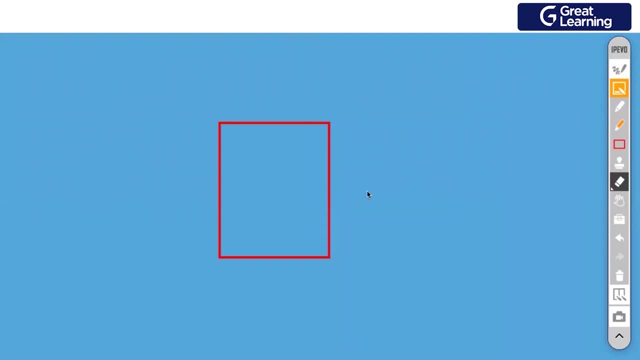 one, one question here. yes, when we go that we go for the backward correction, in that case it is assumed that we know the input as well as the output and we are putting into the box and verifying that whether the box is giving me the output. but in the case of prediction, we really 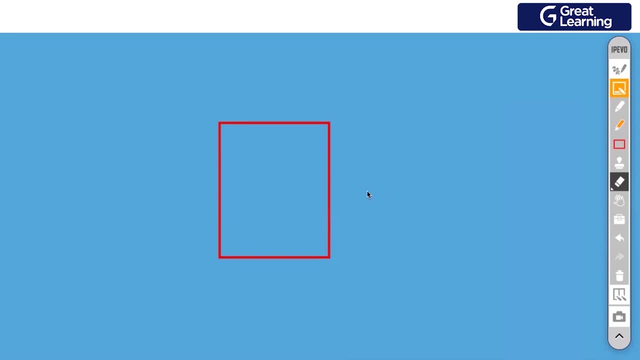 do not know, basically, the future prediction. we really do not know the output. so how does this really work? okay, so for any machine learning, whatever box i showed, you know, whatever we did, supervise, unsupervised, ai reinforce whatever we saw. the very first phase of any machine learn technique is: 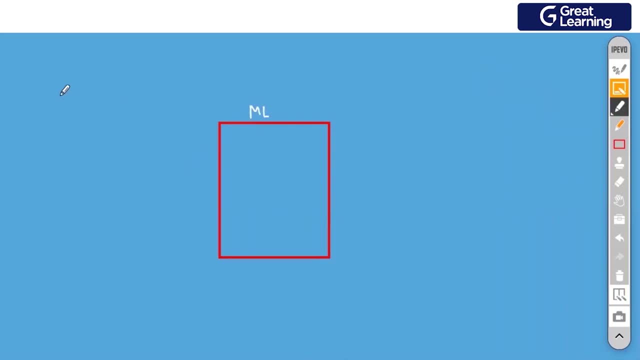 machine learning, basically. so for that we need a set of independent data and a set of target data. no matter what you are doing, if you are doing text processing, if you are doing voice processing, image, no matter what, the input matrix remains same. all right. so what you have? you have got some input. 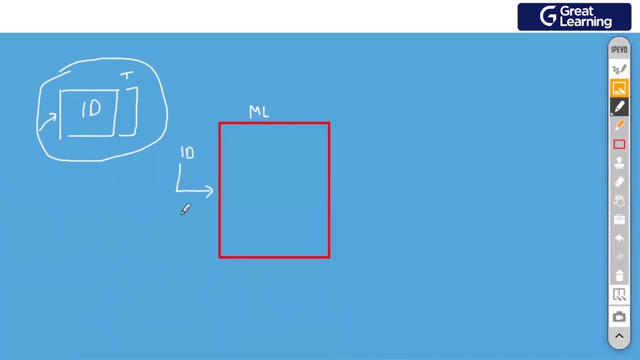 for training, that is, we call it the independent data. then you have got some tags. you remember, guys, y actuals. right, this is what will be our reference point and whatever we get output we will have, we will call it as y pred say. we are going to compare always y pred with y actuals. 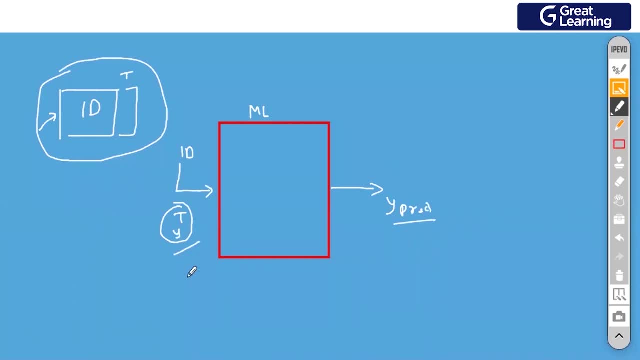 always, no matter what algorithm you're doing. And then, if you are asking your future predictions, once our machine is learned, Once the difference between both of them is reduced to our satisfied level and the machine is learned, you have to disconnect this. You have to disconnect our input and you give only your futuristic output, which will be only your independent data. 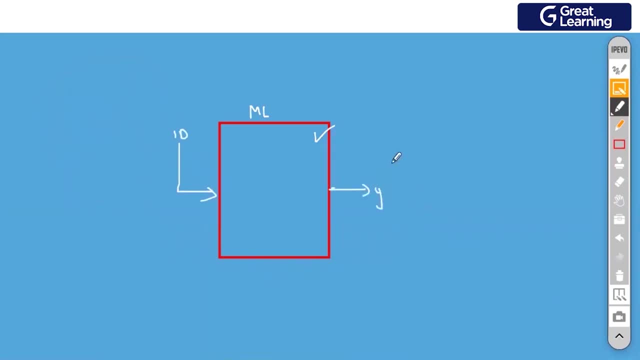 So that you will get why. All right, that's more of a learning phase. what you exactly? What, Yep? So this is a common stuff for all the machine learning, No matter what. it is The first thing we have to make it learn. Now there are some algorithms like LSTM and all that I was just talking about. 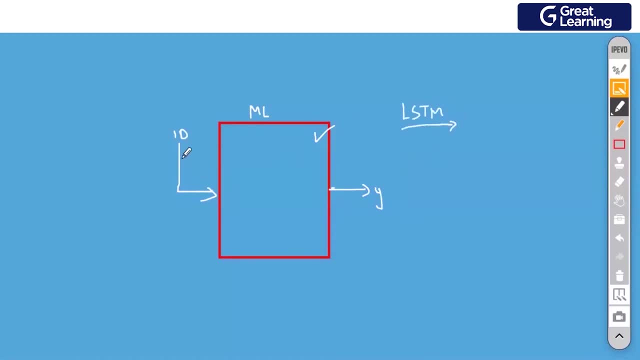 Yes, indoor those things, we can predict some something without learning much of it, but we'll come down. So when we come to NLP we will look at. let me not confuse you guys right away. Okay, for now, this is what does the architecture we are going to look like. now There are some questions. Let me see. 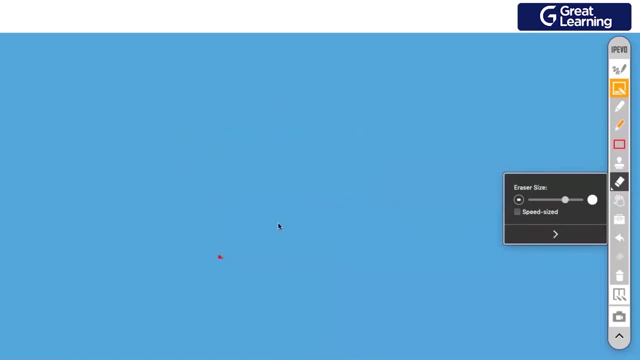 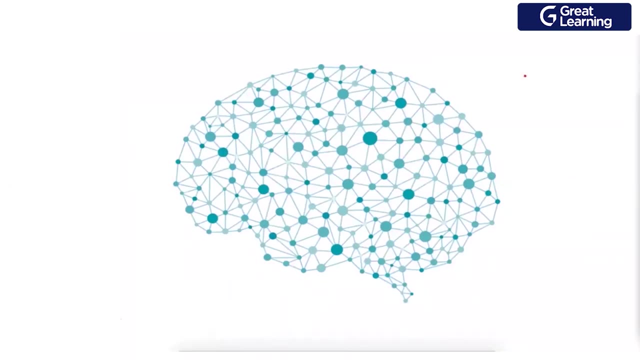 Okay, all right, Okay, so now Let's go to this PPT: how to interpret neural network. So let's keep, Let's take the inspiration This is. this particular topic has been picked up from biology, Okay, and neither of us are export onto that, So we will make our own version of neural network, Let us say, your brain. 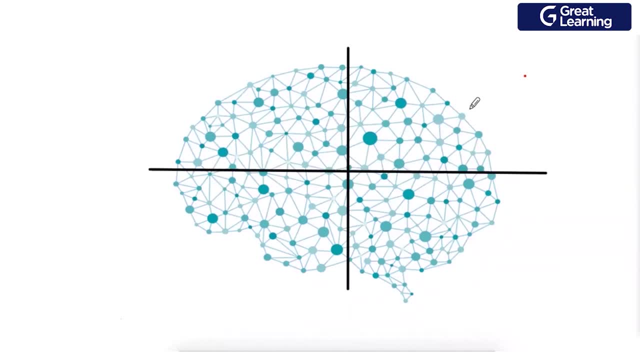 Neurons, the neurons that are there, and please remember there is no neuron in your brain which is not connected To the one some other other way it can reach from here to, let us say, to some other neuron. Yeah, so that is the first part of it, which is called fully connected neural networks. 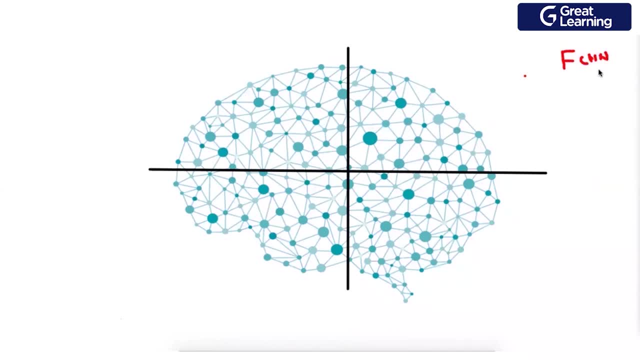 This is the basic of all the neural networks. That means each neuron is connected to all other neurons in the Network. All right, Now let us say you divide this into four parts. This is part number one, two, three and four. Now, when this brain was newly formed, that means when this was a baby. 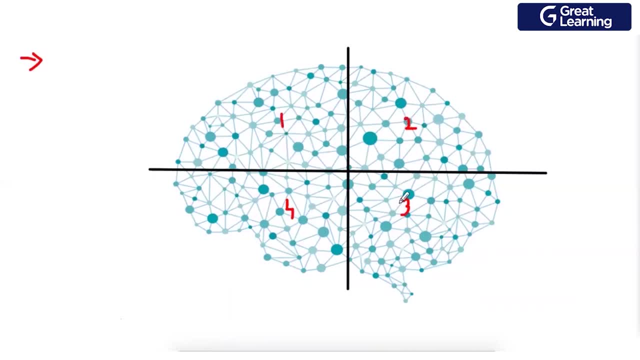 and that that point of time, all these four were of almost similar. these zones were not differentiated. now, what are these zones, you may ask me? let us say this is my happy zone, for example, this is my sad zone. okay, we will not compare it with real biology, because if we do it, we are going to fail on to that. so I'm just 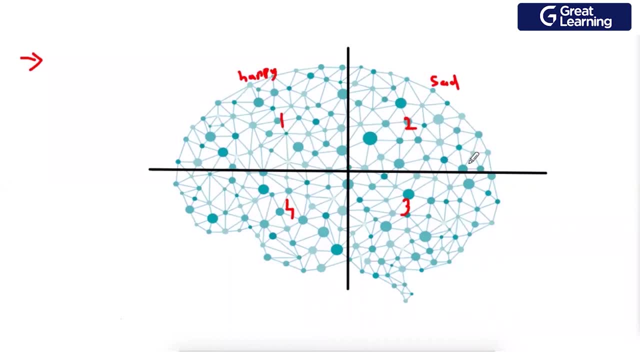 showing you certain neurons belong to happy, certain zone to sad, certain zone to say relax part of it or sleepy part of it, and certain zone to the anxious part of it, for example. okay, let us say, when the baby is newly born, they have not seen much out of the world. so what they do is they mix up all the emotions. 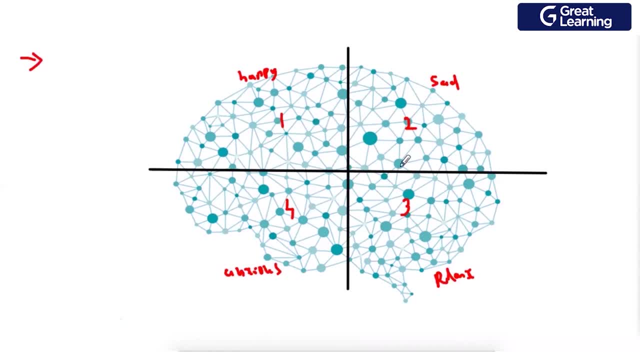 sometimes they keep crying, sometimes they're happy. they don't get it now, when, when lot of events happen day to day life and the person grows up to some level, there are certain learnings that the person does and the person tries to store those learnings in each of these neurons, depending on the zones. 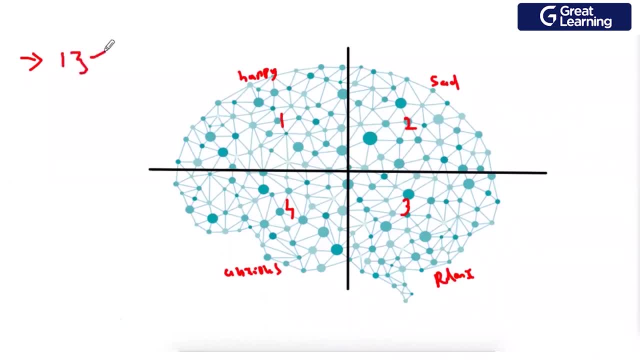 so let us say after, let us say at the age of 13, if a kid passes with a very good score, definitely the neurons over here will be active, all right. so please remember, a neuron can be activated and a neuron can be deactivated. that means in the happy phase, all of these will be deactivated. all right, they don't. 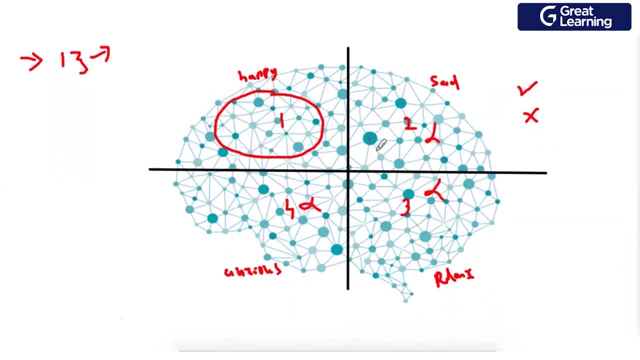 continuously keep running. the electrical signal is sent from one to another one only in certain triggers situations. all right, so this is what is the theory behind why we use neural network. so from here now we will try to put this whatever I said on to the machine- part of it, so let's see. so what basically you? 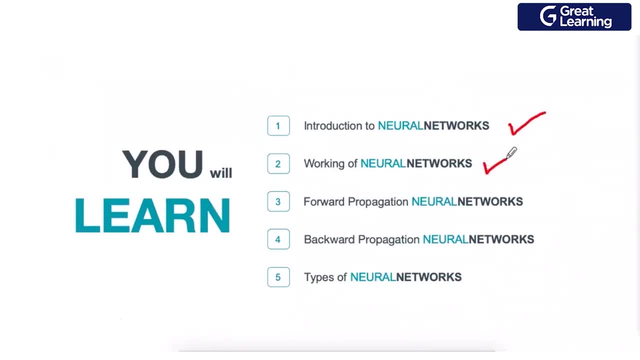 will learn at the end of this particular session as intro to neural networks, working of a neural network, forward propagation, backward propagation and types of neural networks. so we will see to this on a very detailed because now, whatever for five months you have from your course, we will try to explore all. 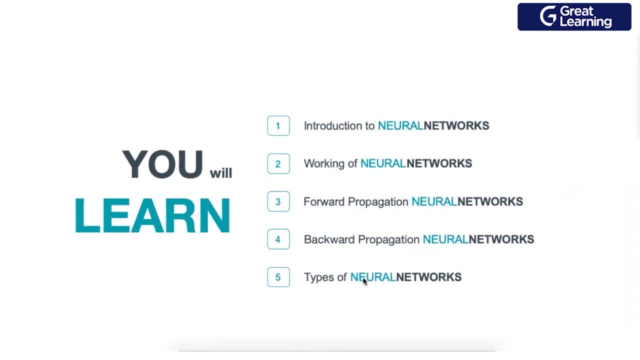 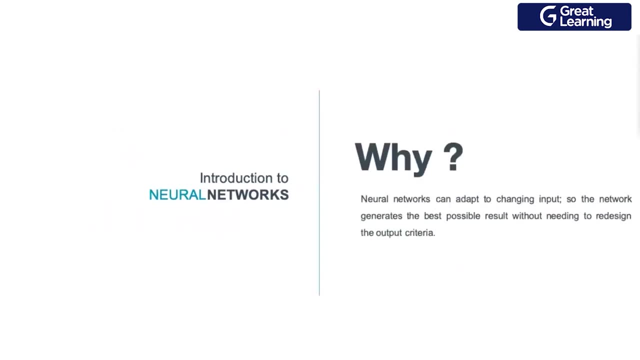 most every type of neural network available in the market right now. next one is: what exactly? so I explained you what is a neural network. why do we use neural networks? so please remember it's a very simple: neural network can adapt to changing input, so the network generates the best possible result. 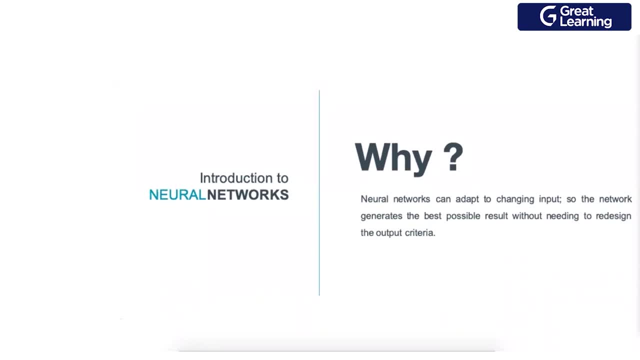 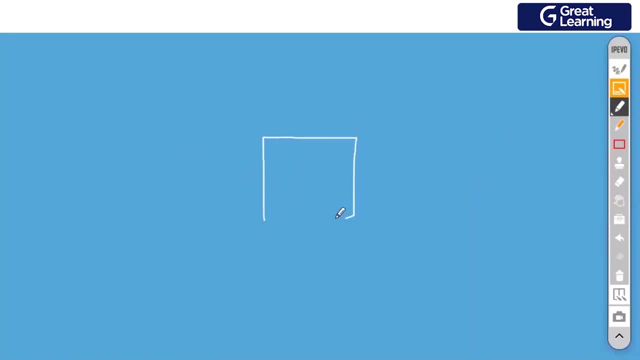 without needing to redesign the output criteria. what do I mean now? let us say, for example, we take a linear regression. yeah, in linear regression, if we have baselined our equation, you people remember this equation, right? I think we started our interaction from this session itself. yeah, now is it possible for me to change? 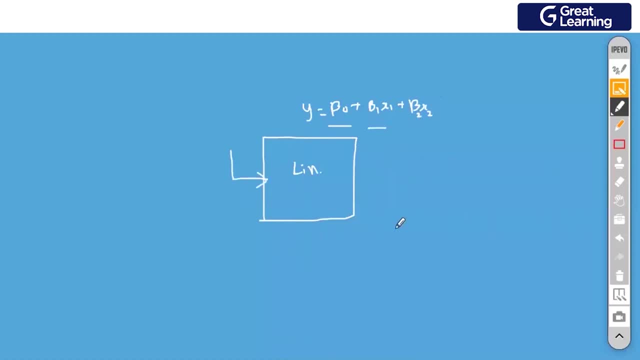 the inputs. if I change the inputs, will this work? we are not sure. if the inputs are very close to what we trained it on, yes, it will work. if they are not, it will not work. this model will crash. what if I tell you that there is a possibility of 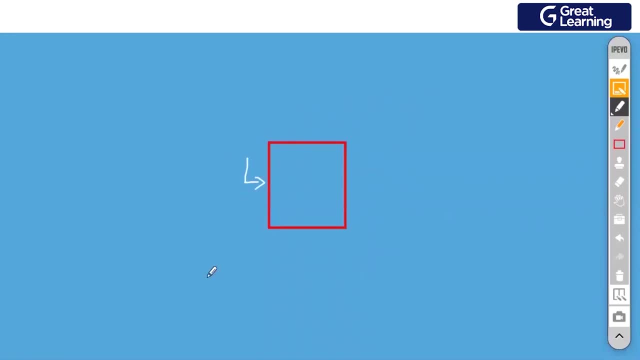 making a machine and model. no matter what you are going to give me, I will relearn myself always and I will deliver it out. what if I have got a self learning kind of stuff? yeah, so I will say this is more robust to changes, this is more adaptable and this is more quicker in the terms of 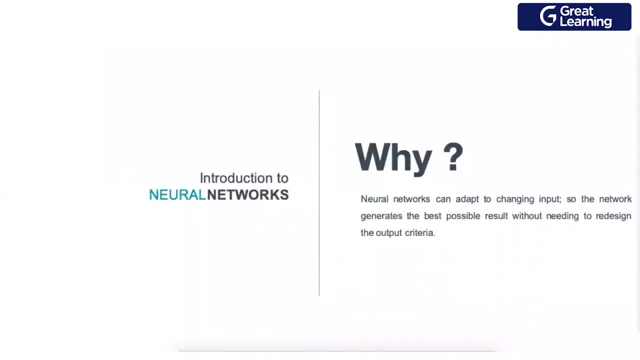 learning. yeah, so this is where you are going to need your new neural networks network. so the box that I just drawn, the whiteboard, that was only material. usual guys do stop me if you find it difficult to understand. yeah, now next one, what is the application of it? so, basically, I hail from deep learning background. this: 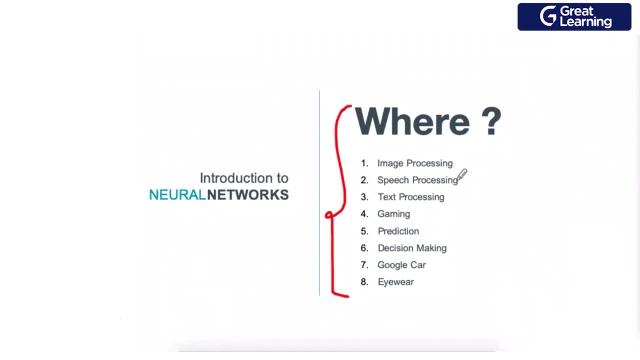 is what I do on my daily basis in my job. now you can use deep learning for anything. whatever you have done so far- classification, regression- you can do the same thing on neural network. so the first thing I would say is decision making, that is, your prediction and decision. second thing is, if you want to, 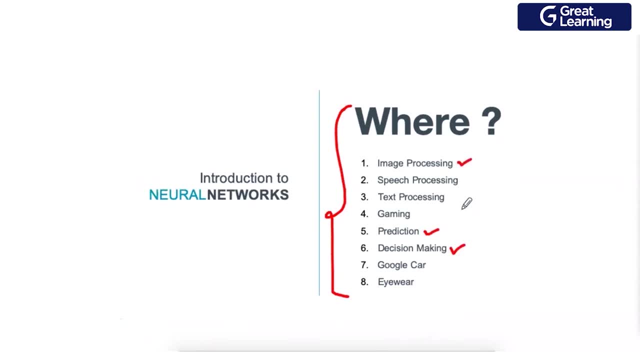 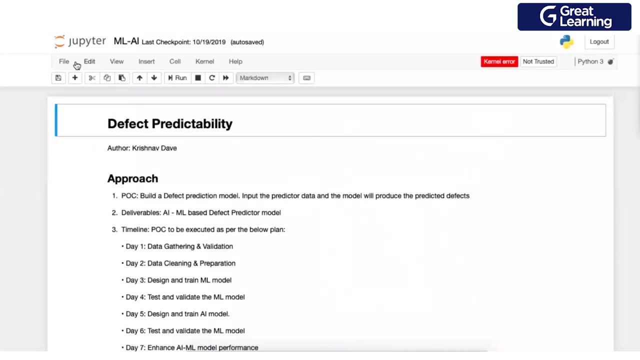 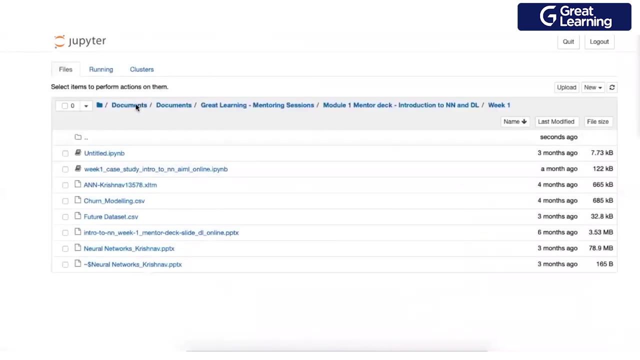 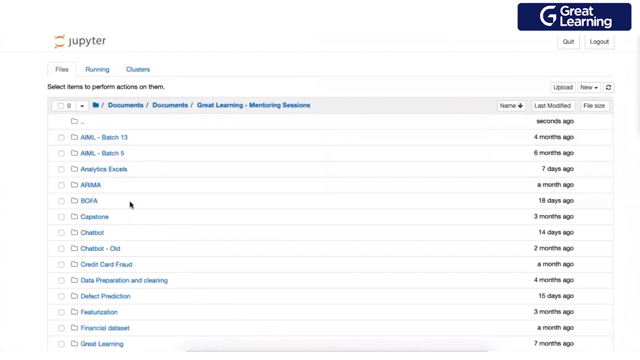 go a little more complex. you can talk about image processing. so what do you? what do I mean by image processing? so let me quickly show you then. then do you think you know the deal is much better than a mill? yes, definitely, okay. and then then why? why the people use a mill? then 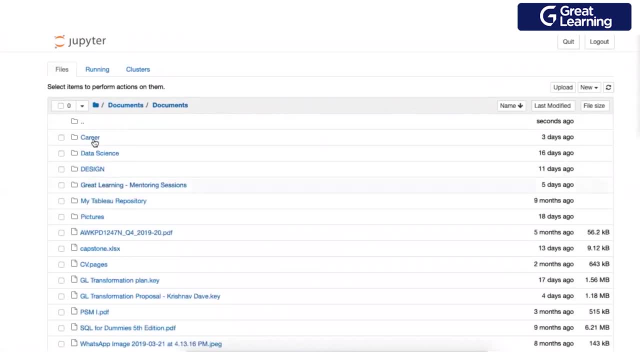 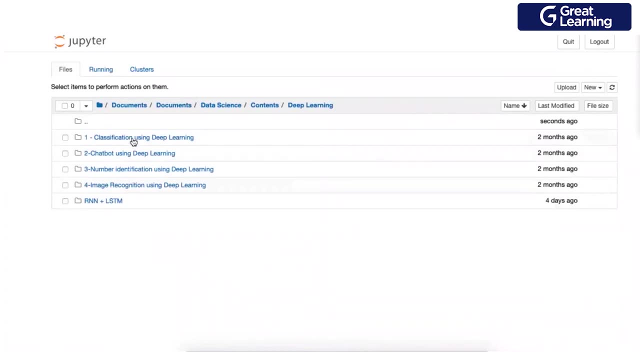 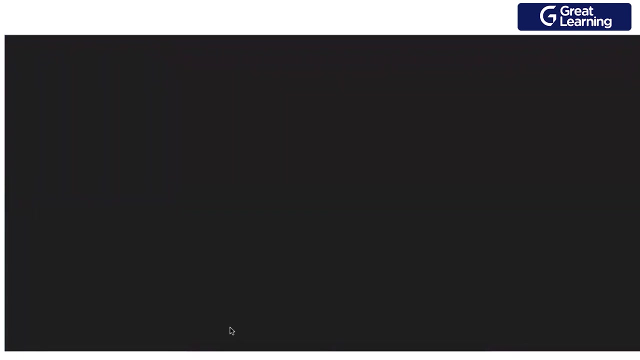 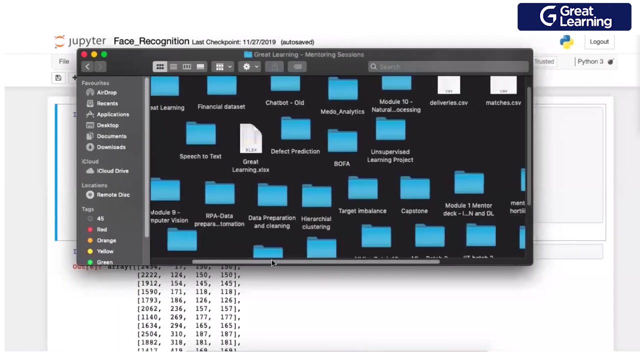 yeah, I'll tell you why. why do we do that? just give me a minute, okay. data science contents deep learning, you, yeah. so now let me take you guys through a very simple application of neural network. it is not simple to code but, yes, down the line we are making it more and 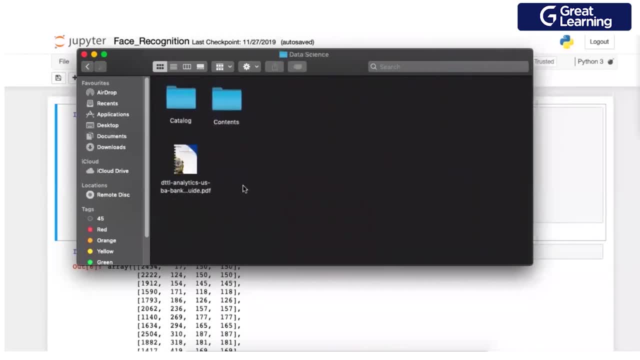 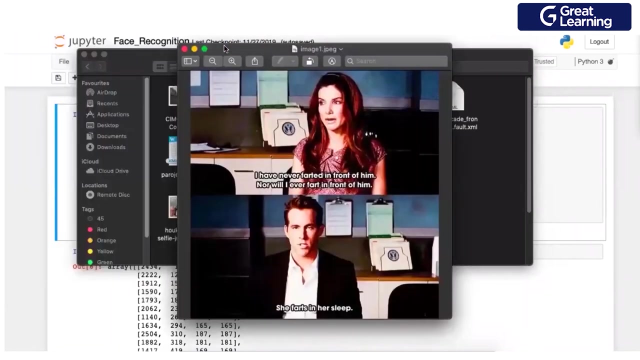 more simpler. I have too much actually over here. contents, deep learning, image recognition and image. let us say I have a screenshot from a particular movie, all right, so this is a screenshot for me. now I want to automate certain things over here, so I will give you an example. if you people 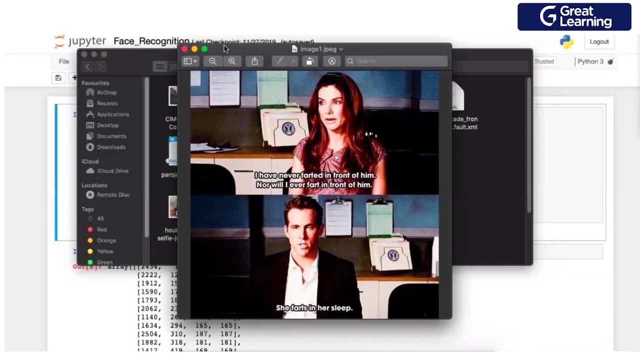 are on Netflix or Amazon. if you click on the star cast, the particular scene which is going on, they will give you the, they will match it up who is there in the particular scene and they'll give you the description of the star cast. hey, we guys observed that if you stop the screen immediately and check for the 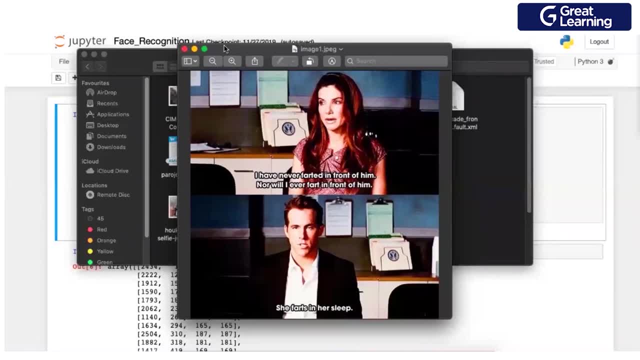 star class at F輝 on Amazon Prime will get the names of only those people live who are there in the scene. have you seen that? no, nope, yes, yes, in prime you get to see correct. how do they do it? very simple, what do we do? 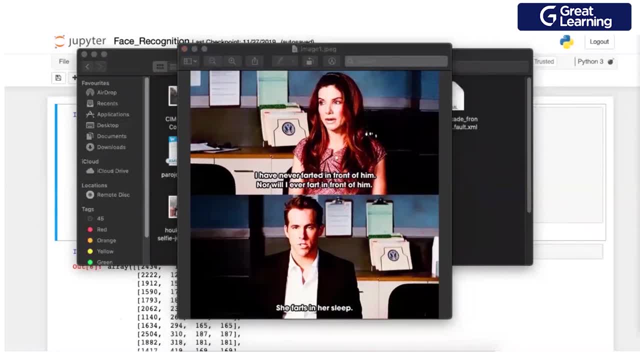 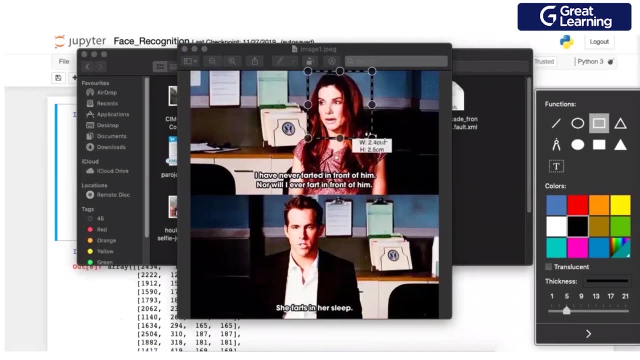 is when you click on to that star cast button. amazon prime uses its own image recognition system and tries to create a boundary- okay, let me use a different color. tries to locate a face in the image. you would have also seen these kind of stuff nowadays flying around. 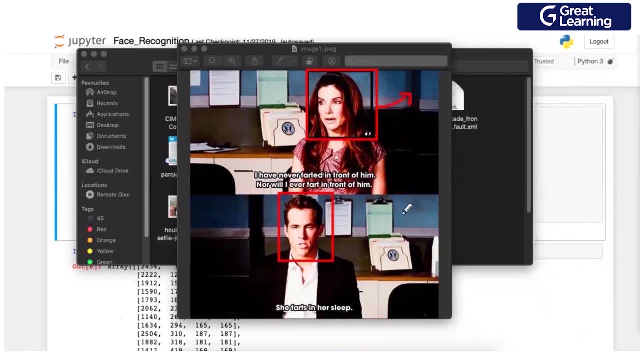 on YouTube if you are talking about AI. no, they will see people who are walking and they would have made one box around the people who is walking and they would have said: this is a person who's walking. it's become a trend now to post all these things on YouTube and 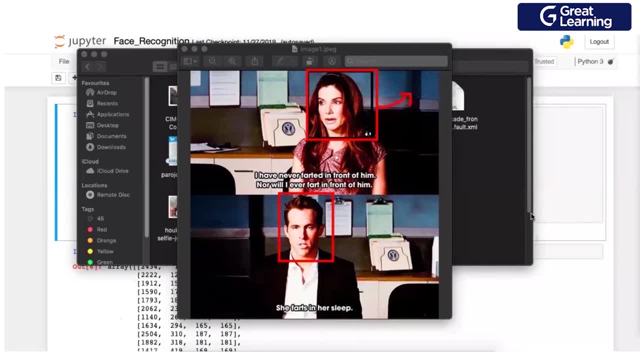 LinkedIn just to show that, oh, I work on AI- part of it, yeah, but it's not a rocket science. we are going to learn down the line now, this is what I want to do. so how do I create a conscious image in the image of a woman and what is the target variable? what is the target? 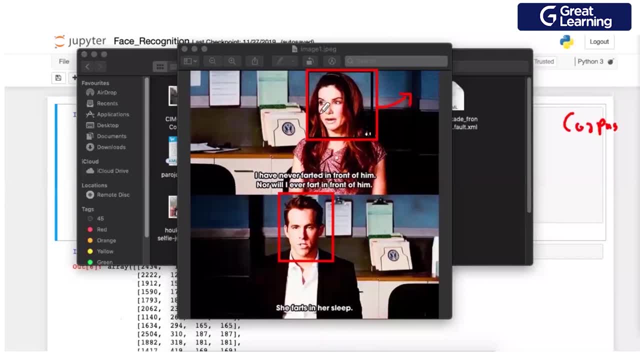 variable. and how to do this very simple. first of all, you need a big corpus. corpus means a back-end data saying that we don't. we don't know whether we'll get image of this lady or not, we don't know whether it's there in Corpus, but yes, we will get a lot of images. 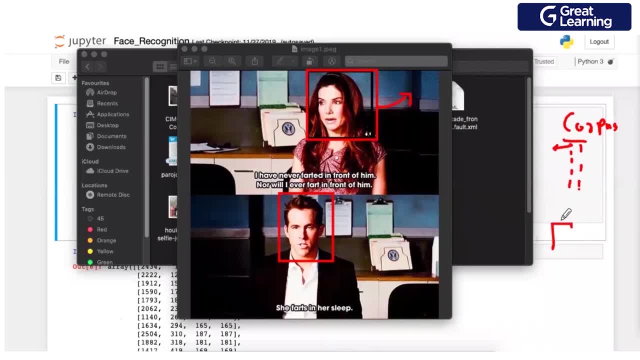 of men and women and if it is a man, the tag attached to it. so if I say the independent variable is men, the target variable attached to that will be men. that is the image. is men the target variable attached to the image? and, yes, so when you go to the image of the 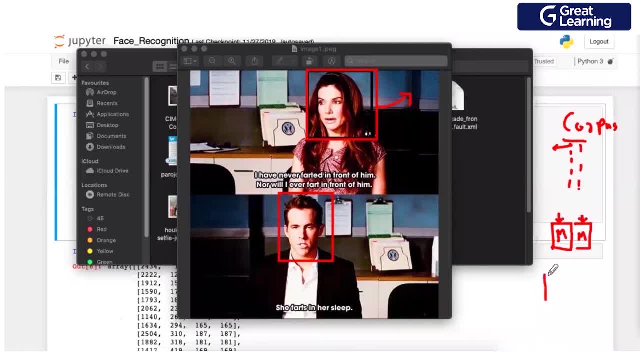 to it as men. so this is how I tell my neural network: that I am giving you an image as an input. you have to adjust your whatever is inside such a way that you have to give me. so whenever I give you this image, you are supposed to tell. 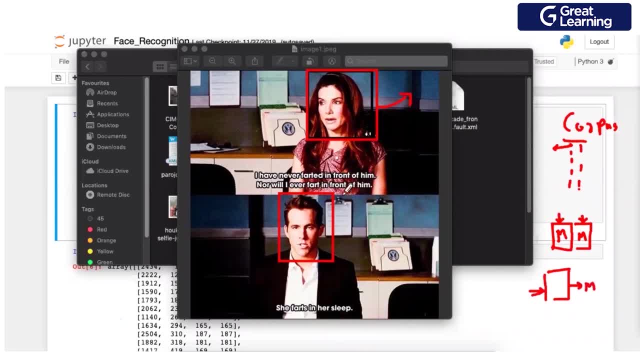 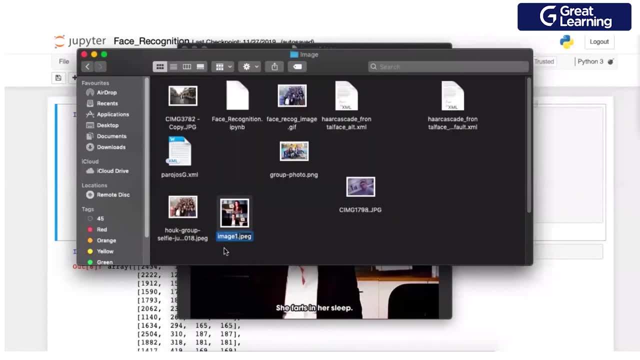 me. it's a man, you know. so this is how we do it. so let me now show you how do we do it. so this is an untagged image. let me try to copy the name of it, and now we will try to push some kind of brackets on dude. yeah, let's see. so all I need to. 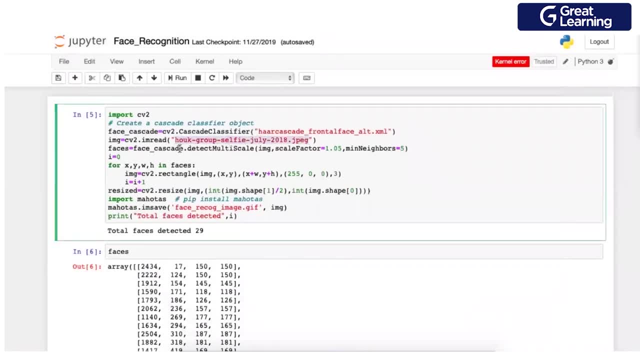 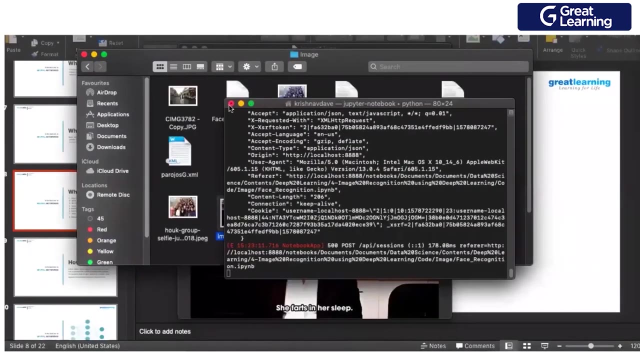 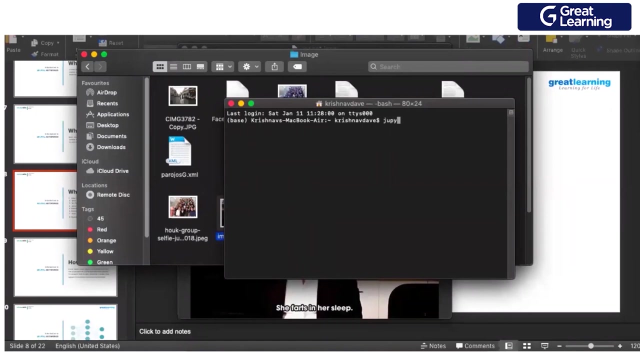 do is. this is my version of image processing. okay, so just hold on for a minute. a kernel is dead. just give me a minute, guys. why am i showing you this? is so that you'll get to know. why are we learning deep learning. otherwise, if I would have started neurons and all, it will be the same as our video. 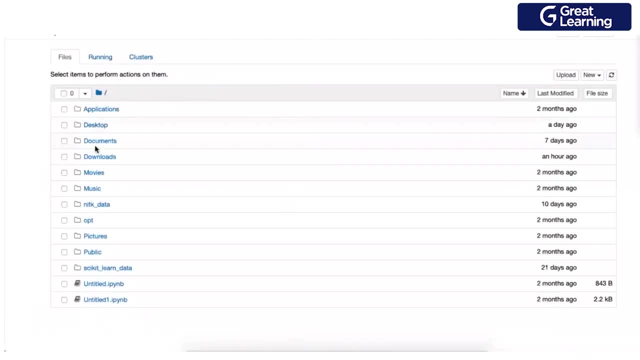 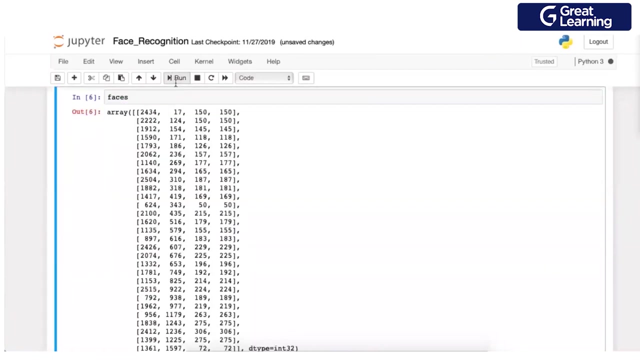 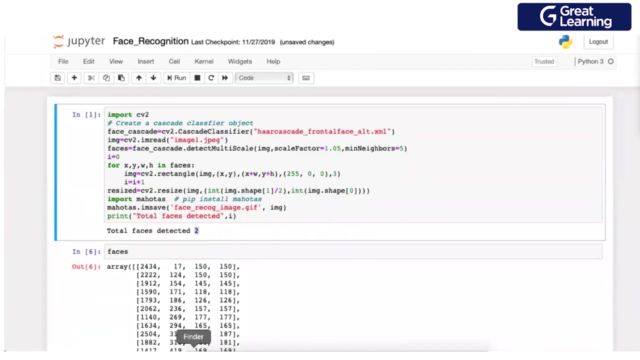 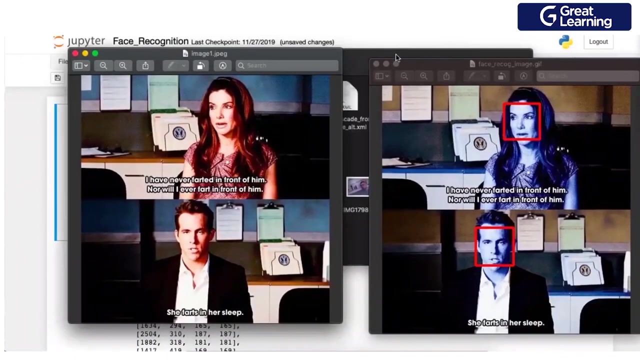 yes, and here I will paste our image. yeah, processing. yes, it is showing me there are two faces that he has detected. did you see that? and later on, if I you go and see here, this is my output image. it is very simple. it is showing me, and we have detected two faces here, the next. 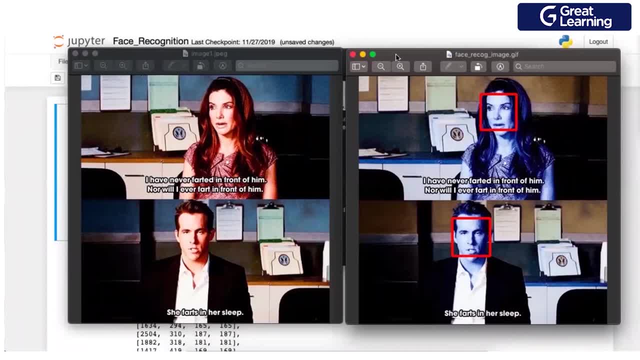 version of this could be: find out who the celebrity is. so what we have to do? we have to give an input corpus of all the celebrities and we have to retrain a network saying that if you get this particular image, whoever this actor is all right. so this is how Amazon and IMDB and all these people do it. if you want. 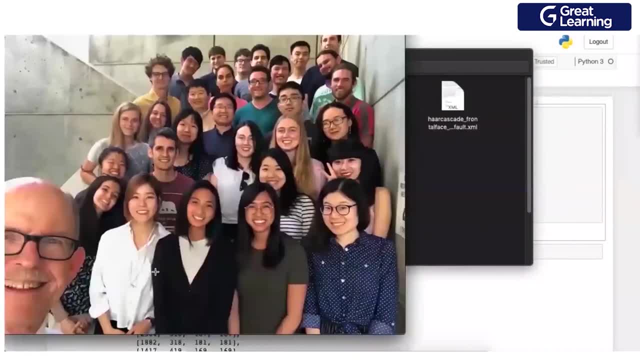 to take one more image. you can do that. so this is how Amazon and IMDB and all these people do it. if you want to take one more example, let us say we take a complex example. look at this image: it's pretty example. let us say we take a complex example. look at this image: it's pretty. 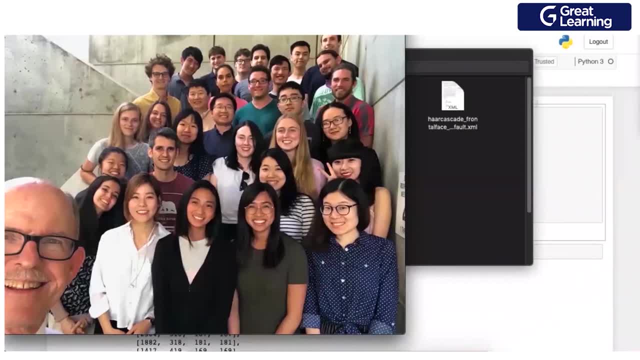 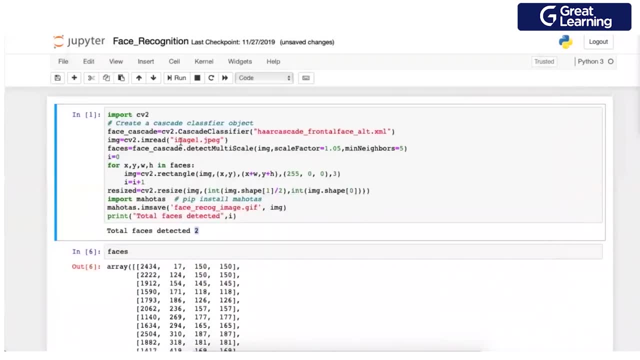 huge right. so what I will do is I'll try to push it across through a neural huge right. so what I will do is I'll try to push it across through a neural network. so I just let me copy the name of the image, will input it. so this is a 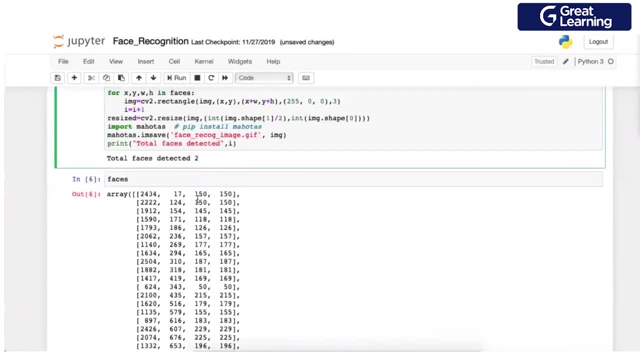 network. so I just let me copy the name of the image. will input it. so this is a pre-trained neural network. I'm not re if you observe there is no neural network. pre-trained neural network. I'm not re if you observe there is no neural network. 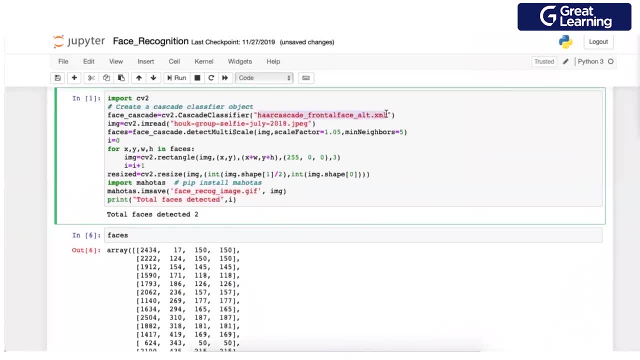 running here. why? because my neural network is currently lying into this running here. why? because my neural network is currently lying into this particular format. you don't have to keep running your neural network every time. particular format: you don't have to keep running your neural network every time. 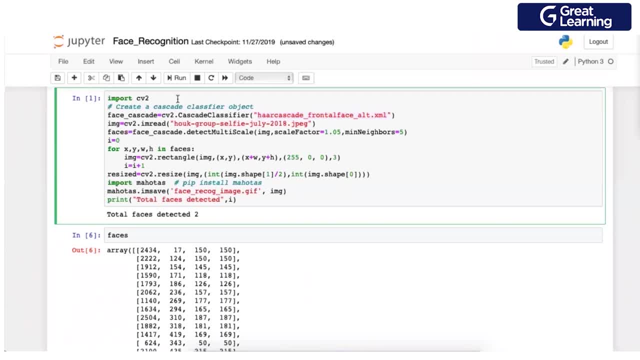 particular format. you don't have to keep running your neural network every time. you can store it, pickle it, and whenever you, you can store it, pickle it and whenever you. you can store it, pickle it and whenever you want it. you can export it on in this. want it? you can export it on in this. 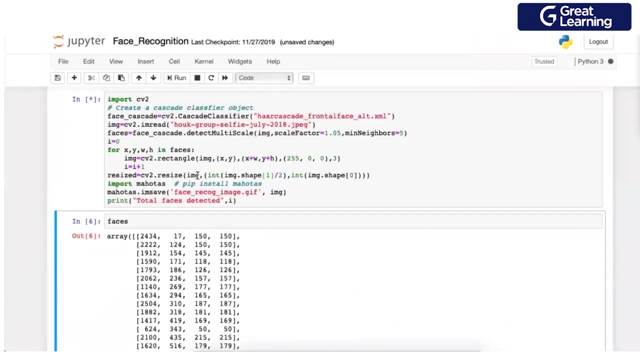 want it, you can export it on. in this case, I have an XML file which does my case. I have an XML file which does my case. I have an XML file which does my job now, if you all take some time. job now, if you all take some time. 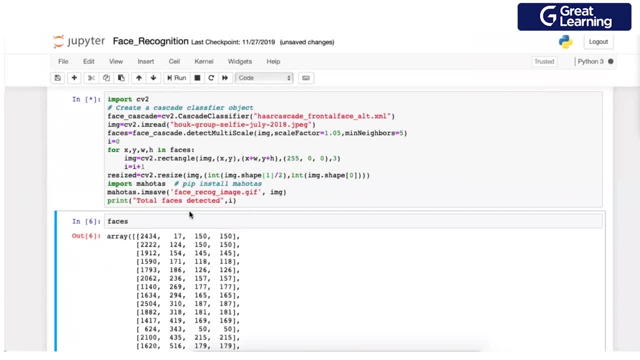 job now, if you all take some time, because there are a lot of faces there, because there are a lot of faces there, because there are a lot of faces there, and it will show me how many faces are, and it will show me how many faces are and it will show me how many faces are detected. if you observe these saying we. 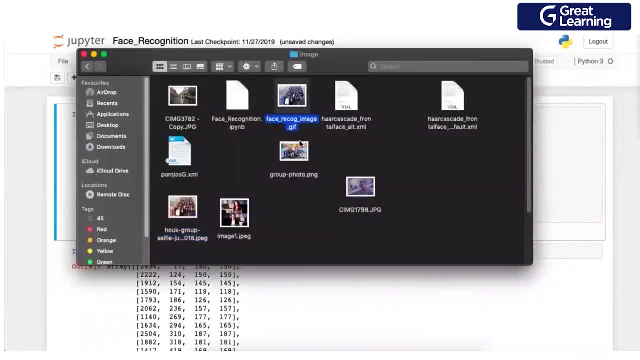 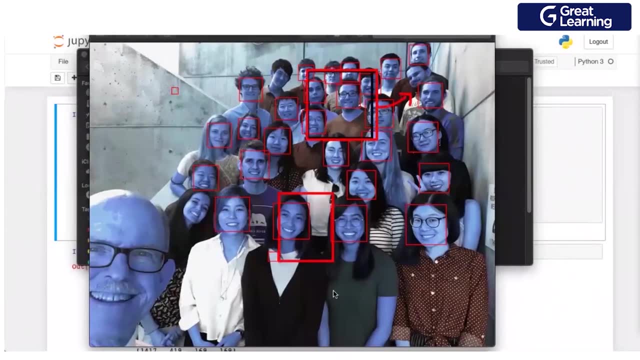 detected. if you observe these saying we of 29 phases detected, let's go and see the output. this is how the output looks like. yeah, and you will observe, some of the faces are not detected in your. when you spot those faces- 1, 2, 3, 4- what is common between all these phases, can I? 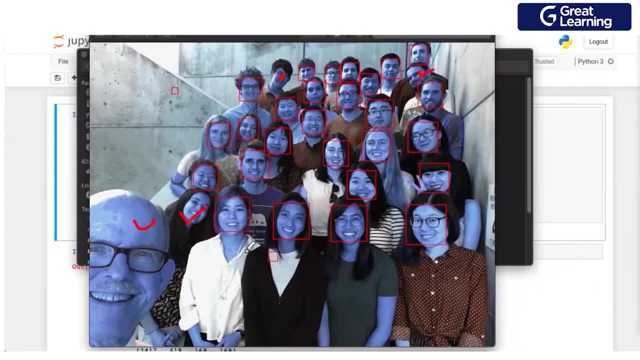 say they're tilted. yes, yeah, so there is no box around it. that means the corpus that I've used to train this particular neural network needs me to have a straight face or full face for this particular person. the full face is missing. all right, so this is how you. this is the end application of a neural 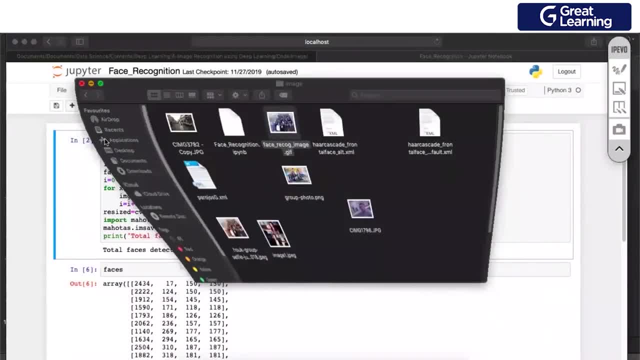 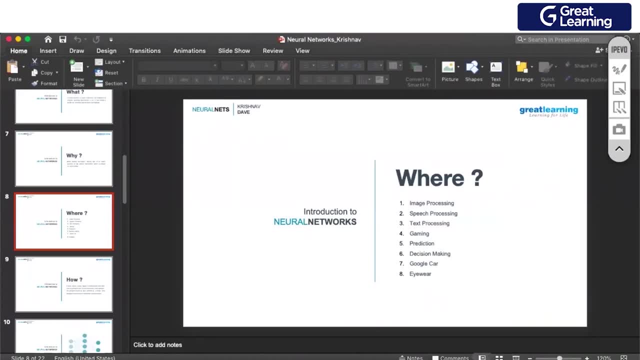 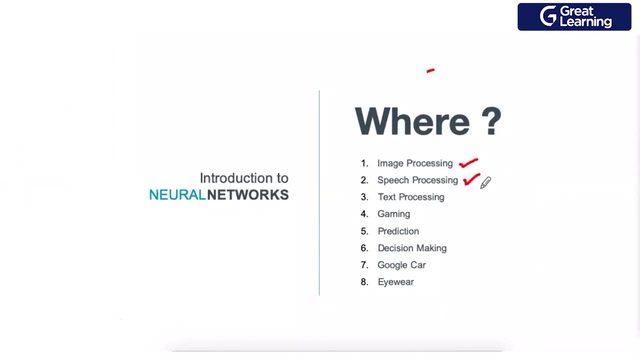 network. I will say clear, we will go deep into it down the line in computer vision session anyway. so this is how we do: image processing using neural networks. okay, speech processing, so I can talk something and from the corpus the network can pick up and it can tell me what I spoke about. okay, so not sure you have seen this earlier, but this: 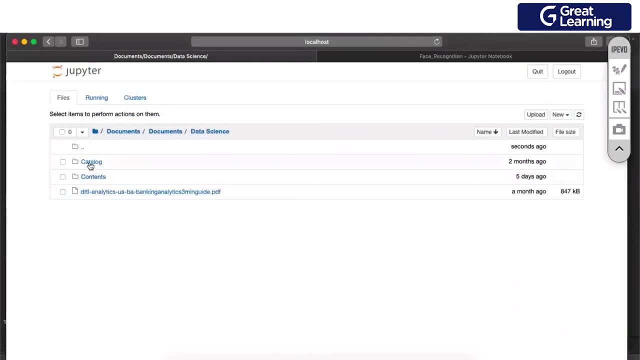 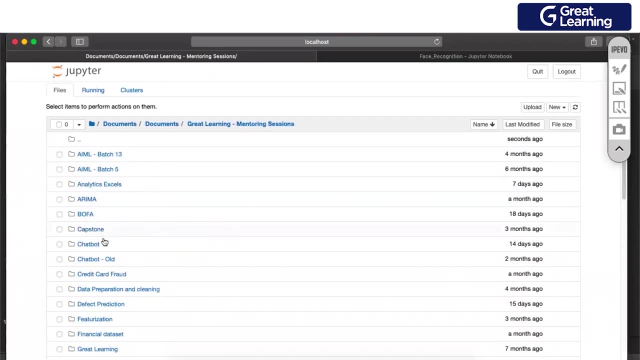 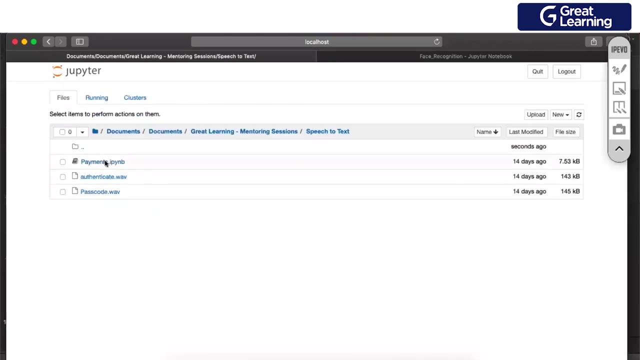 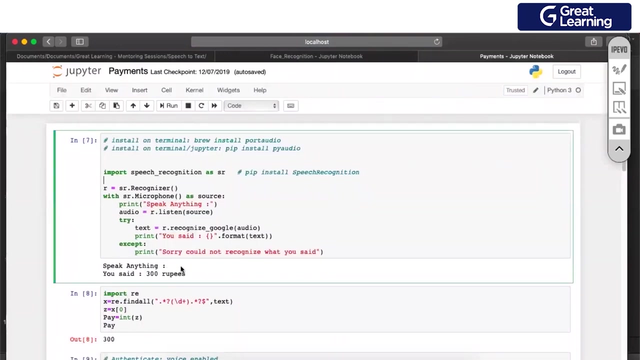 can be a minute. nope, and deep learning, great learning. yeah, so this is my speech to text converter, so just observe. I will talk something and after once I talk, it will populate here and it will tell me what I spoke about. all right, so hello everyone. you. 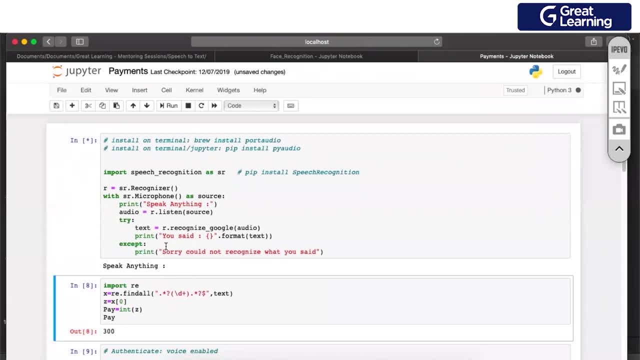 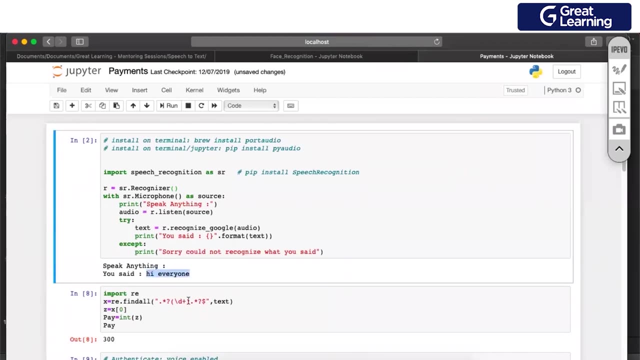 hello everyone. you want to say something? yeah, so yeah, you can. that's that's okay. let's say that's something I have done. yeah, that's okay. so I'll sorry 一 rotate'd. sorry, the mystical that's a bit is so one. so I'm still новая. 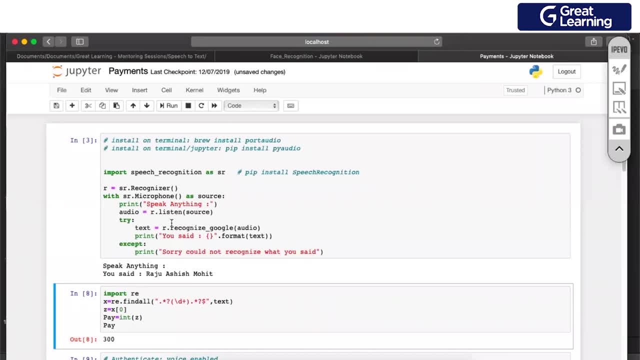 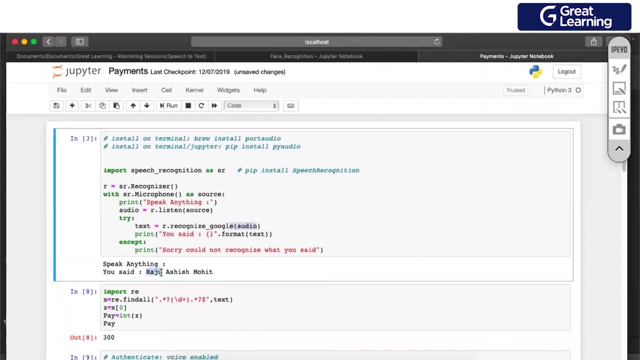 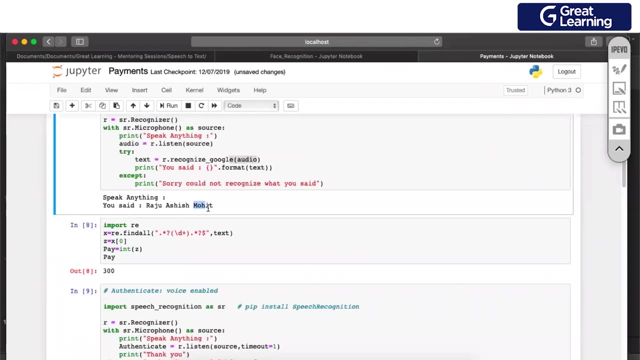 Did you see that? So how does it take it? What are we doing is, basically, we are running some kind of Google audio in the backend, So it is not only understanding what I'm saying, but it's also trying to translate it and move. So, basically, this particular bot, what it does is it's a payment bot. So if I say, pay 300 or 500 rupees, it identifies what I'm saying and then tries to pull out the money out. 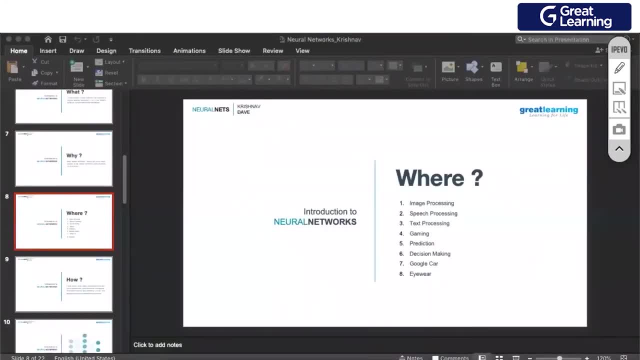 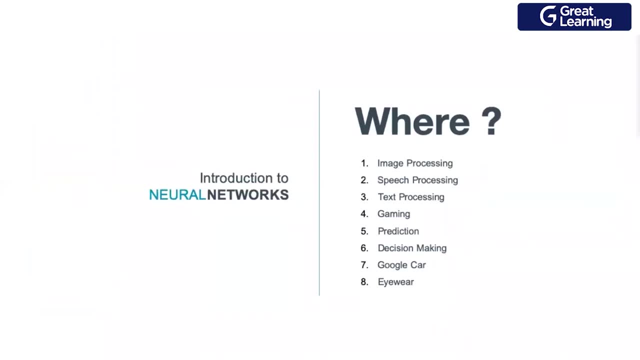 Yeah, So this is one more application where you can use your neural network for voice bot text part of it. So text is not in our certification context, but I will show you guys down the line how you can use this for text also. Yeah, Again, gaming, I'll say it's a very big industry. when it's out of my scope also, It's very complicated And on the futuristic next five to 10 years, you can expect something like this to grow up. So I'll give you one example. There is a startup who is working on an eyewear. 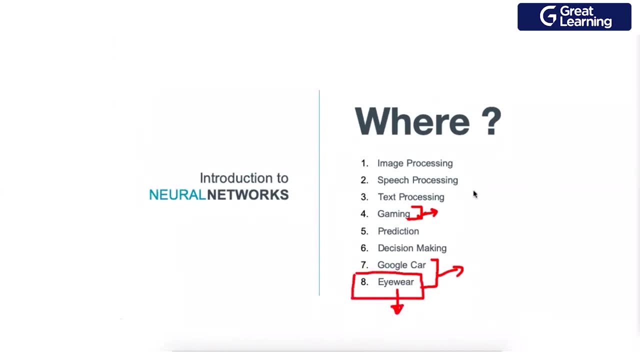 For visually impaired people, So that particular eyewear will recognize what is going around the world. So let us say the person is sitting in a park, So if he wears those glasses, the glasses will analyze what is going around in the park And those analysis will be sent via voice to the blind person saying that there is a dog who is a white colored, He's running, There are three kids who are playing football. It looks like it is going to rain. 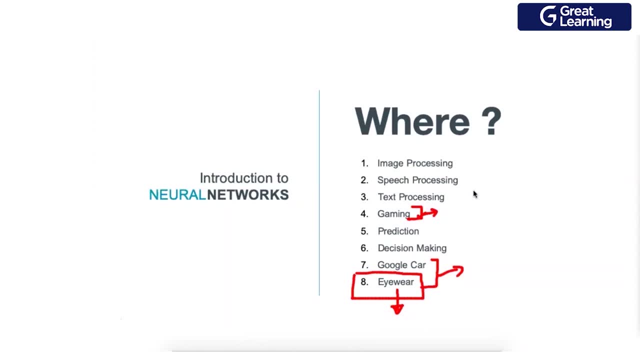 Yeah, If the person is walking, it will caution the person. I'm able to see there is a car coming. Please hold on, You know. so whatever challenges he has because of no vision, they can overcome this. So probably next four to five years, you can expect this to be very common. So computer vision and AI is working towards this. So this is where you are going to use this. I'm not sure how many of you are going to actually work on this industry, But, yes, a very good place to work in for next five years. 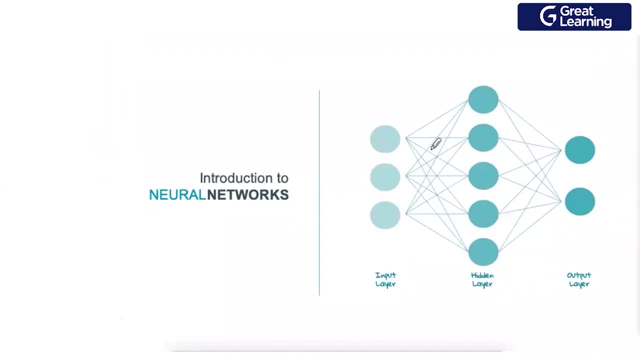 Now coming on to the real part of it. Now, what exactly is a neural network? We saw the applications Very good. Now this is how a simple neural network looks like. This is an example of fully connected neural network- FCNL- Because, if you observe, each neuron is connected to all the neurons in the next layer. 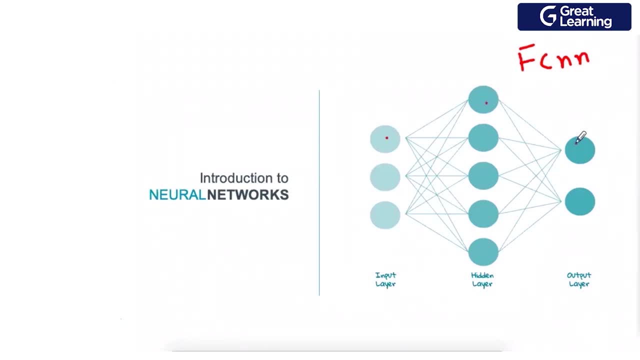 Right, Each neuron is connected to all the neurons in the next layer. So we are not leaving anything, We are fully connecting. Now what actually happens? Let me show you. So what we do is we give an input. Now each neuron or each line that you see over here has got a weight, some random number you can say, which gets multiplied to my input and goes to the next neuron, The whole game over here. So if I ask you now, let us say we talk about some of these machine learned algorithms, Let us say we talk about SVM. 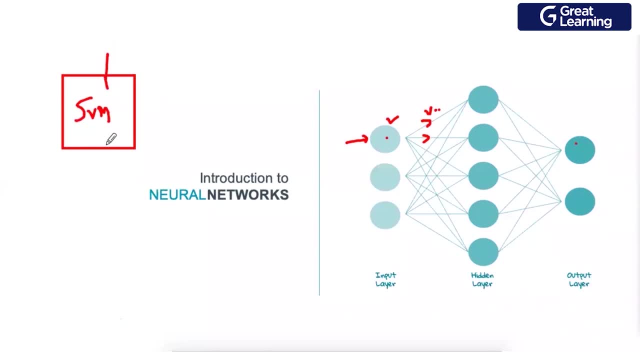 Can somebody tell what exactly we learn in SVM? We give some input, right, We train the model till it learns, And then we say, okay, the model is trained. So what is those things that we are learning in SVM? If somebody can highlight that, 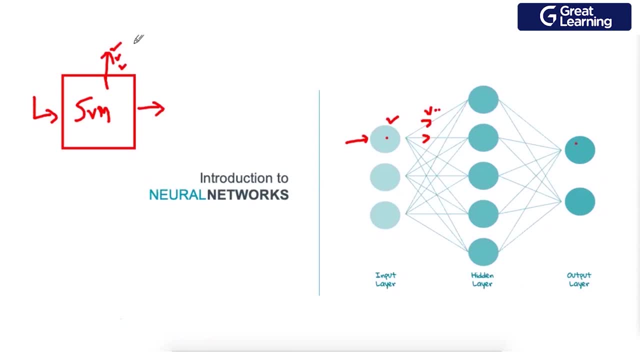 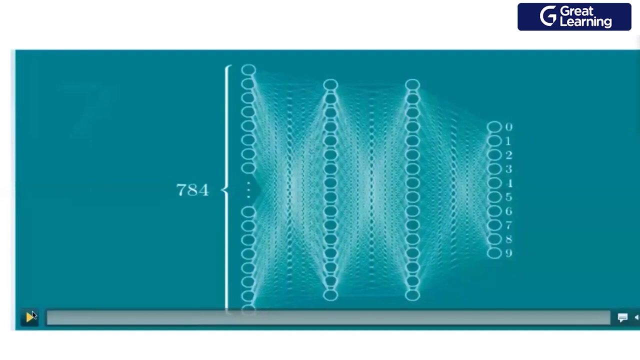 The pattern and the input, Perfect Pattern series, whatever- which can define the whole pattern. So let me show you a small clipping And after that we will go on To an Excel file where we will simulate a neural network. Okay, So, just observe this clipping for now, And then we will see what happens. Okay, So you will observe there is one number seven which, if you observe this number seven, we have divided this seven into some kind of pixels or numbers. Those pixels and numbers are going in the first layer as an input. Okay, And if you observe, some of these are on, some of these are off. 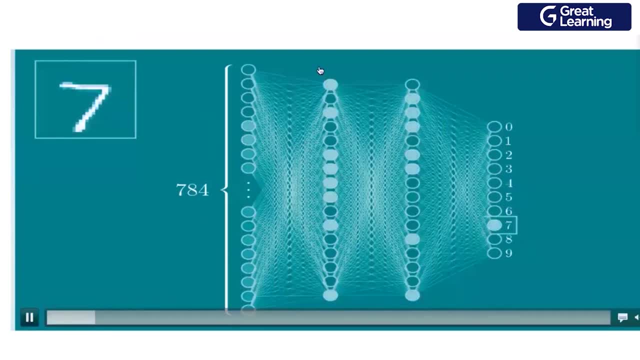 So if I rewind it, yeah, So this is my some layers in the box and this is my output. So if I give a number two, you will observe this particular neuron will come as an output, saying that I have identified that the image belongs to number two. Now the image will belong to number one, So this one will be highlighted. So this is a very simple example of classification. New people agree. This is what we do in a machine learning also, right? 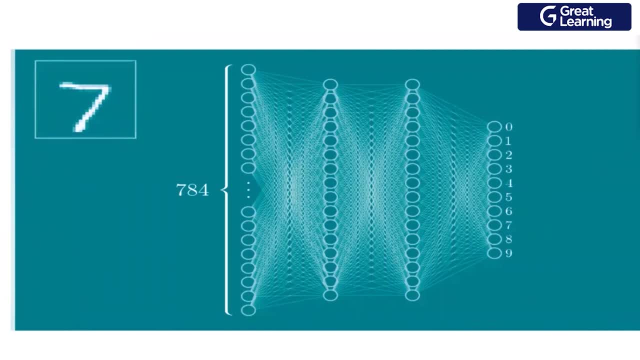 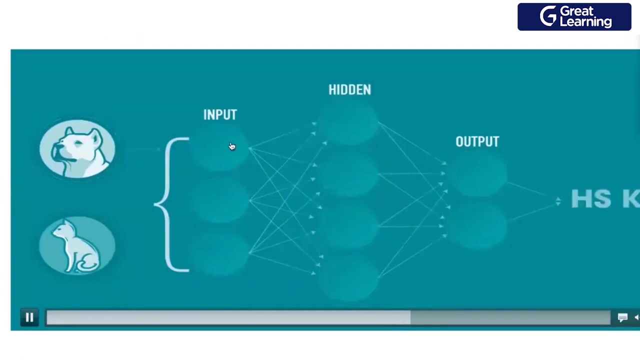 Yeah, We classify. The only Change here You guys will feel something new is how do I fragment this number seven into the inputs, how I give it to them, what happens here, and how the output is it. That is what is the today's challenge. I will explain you guys how it happens. Another way of understanding a neural network classification could be as simple as this: If you observe, there is one image of a dog which gets penetrated into some of the environment And finally I say: it's a dog. This is how we do object detection. 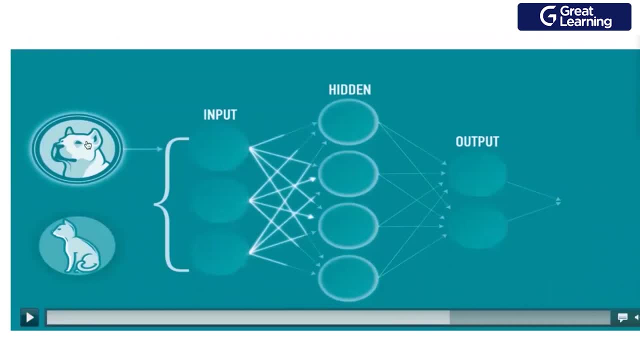 You give any object. If the neural network is trained on that, it will be able to identify, no matter what breed, what angle you have taken the photo, whatever it is, you'd be able to detect that it is a animal, which is a dog. 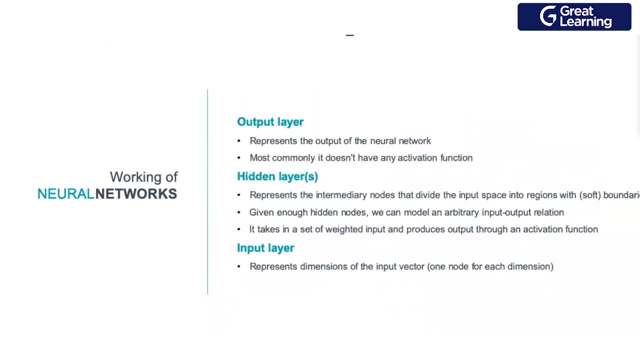 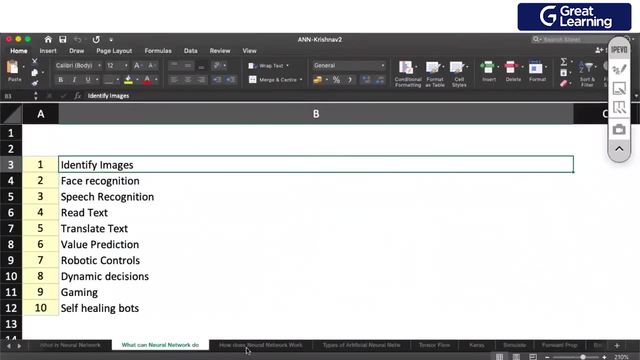 Okay, So now there are three layers which are most important here. One is called the input layer, One is called the hidden layer And one is called the output layer. Now let me shift you guys to the Excel file and we will simulate something. So we'll start from scratch. 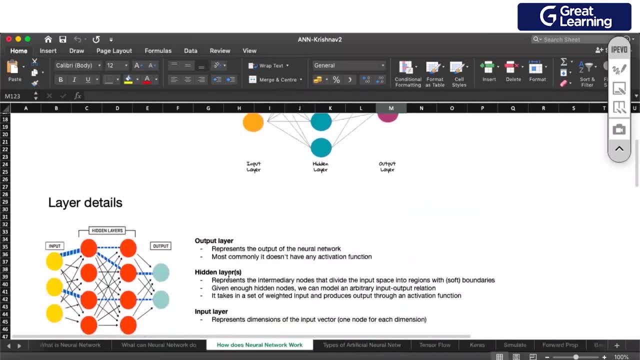 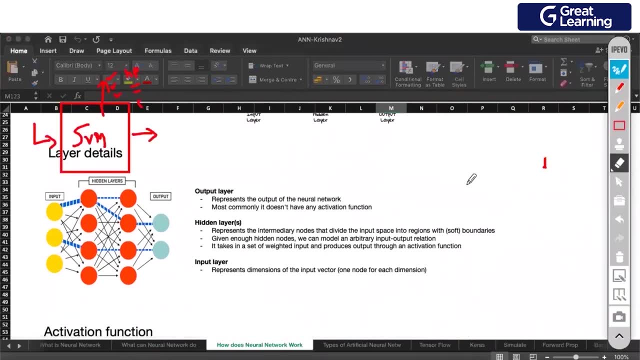 Yeah, How does a neural network work? As I said, we have three layers: input, hidden and output. So please remember, as we are talking about neural networks, the complete operation, whatever it is, it should be in the form of numbers. no matter if we are dealing an image, or we are dealing voice, or we are dealing text, whatever it is. image number goes in, number comes out. Yeah, So let's see how it is. 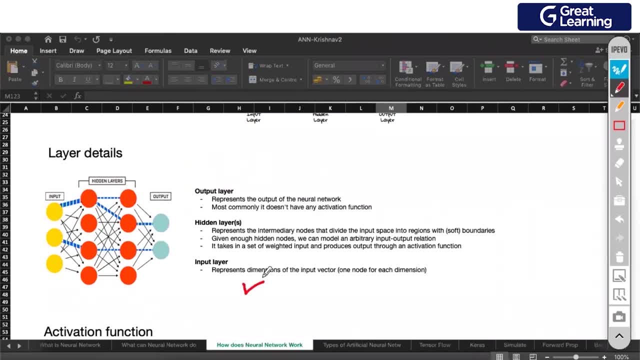 So the first thing is your input layer, So represents the dimensions of the input vector. Now let us say I have a data set which looks like this: It has around one, two and three columns independent data And this is my target data. Yeah, So if I have three columns, that means I'm supposed to have three inputs to this. That means each neuron in input represents one dimension. 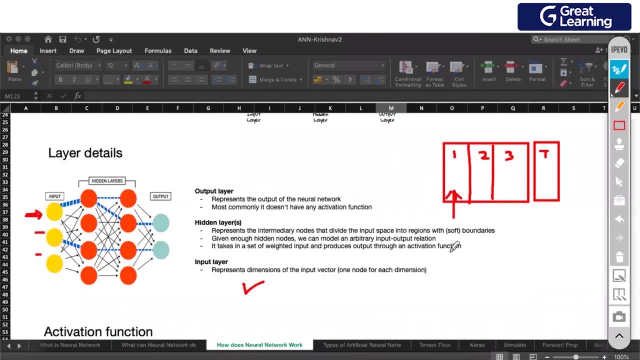 All right, Good. And each neuron in the output represents my target column. So let us say, in target, if I have zero and one, So this neuron is supposed to detect zero, This neuron is supposed to detect one. That means if I give a combination, let us say the combination of zero, zero, zero That means when all three of them are zero, it is going to highlight that this is your classified output. 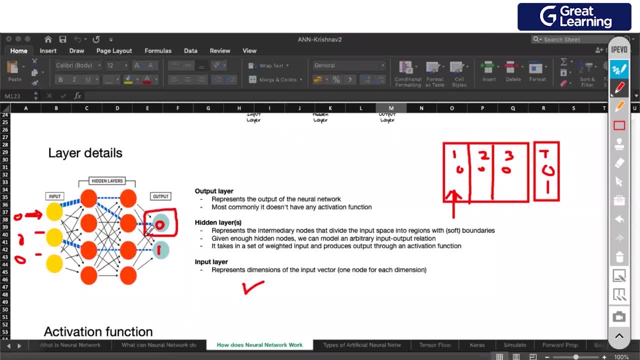 Okay, So this is input and output. This is how we decide input and output. Now comes the hidden part of it. Now, what exactly is a hidden layer? Hidden layer is randomly- I will not say randomly, but it is our choice- that- how many neurons you want here, how many layers. some of them have 10 layers, some of them have two layers, four layers, whatever. These are nothing but the same neurons, But the only thing: they are connected in some other different way. All right, So you've got three layers. 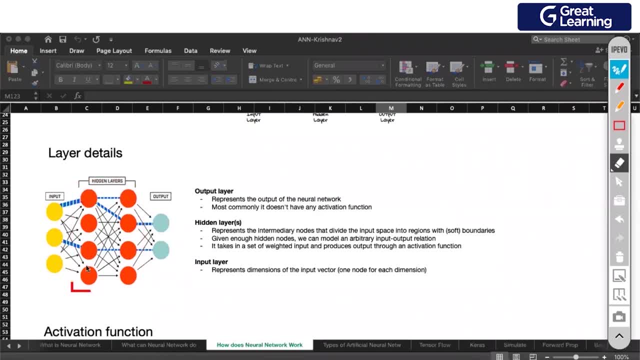 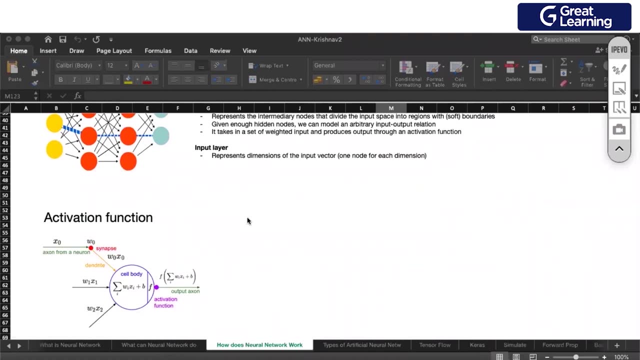 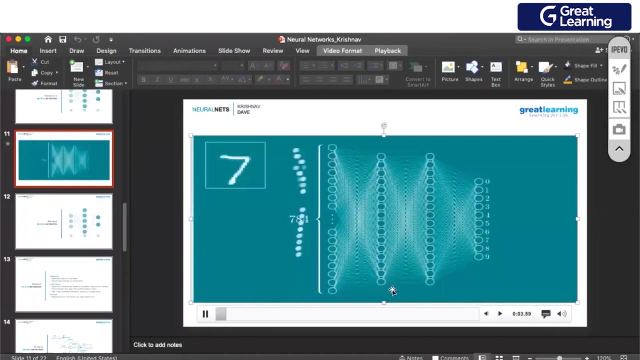 So you've got output, output and hidden. Any issues under this Simple? Don't worry about the calculations. We'll see, But so far so good. All three layers are okay. Okay, Now we'll talk about something called activation function. Now, what is an activation function? If you observe this PPT carefully, you will observe that not always all the neurons are on. Did you see that Some of the neurons are off, Correct? 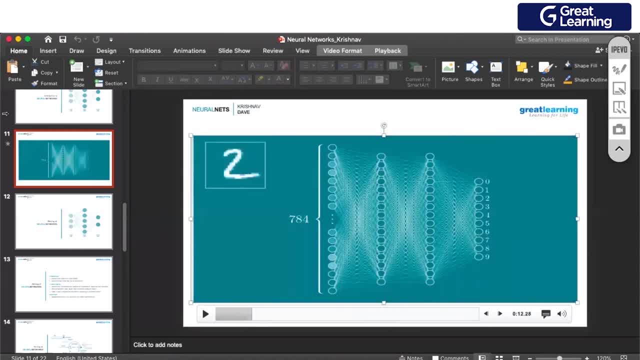 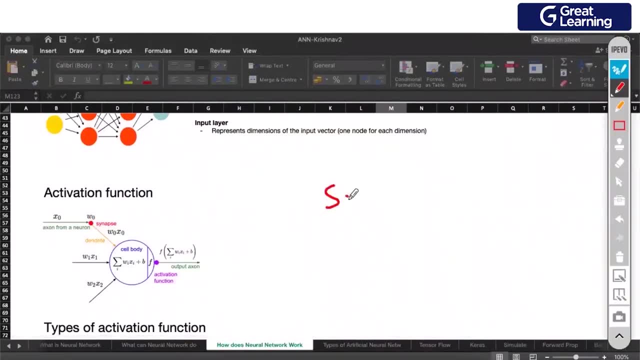 How this happens. This is the job of activation function. Activation function acts like a switch. Let me define one activation function right away. So at any given point in Actor, this is first my activation function that requires an activation function That 123 put into AC. 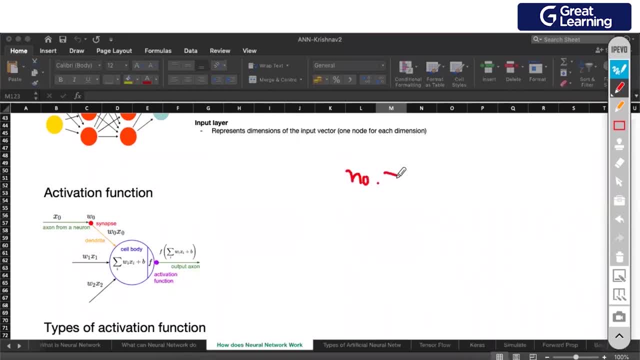 And in an AC activation function I create my rotation Centれた, which is going to be past the 29 on a rate. not er is one zero, A is by no means zero, indeed, So at any given point in proper. So that comes to be the other queue of particulars, So that comes to the changable At random. I am using numbers here andacağım combination which is outer assured here down. Of AC function is actually a number, which is you get welding to not have a four. I am executing this function or nothing other than cancel lunch, because a two- expenses cause animation in the finished code. we need the other two Rest problem come together tucking and canceling this line and ending the equation. 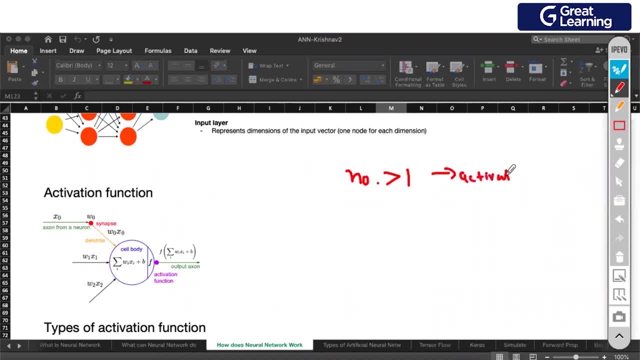 activate that, i will say: pass the number to the next neuron. if the number is less than one, i will say: switch it off. now in my input, if i give a number of 1.2, what's going to happen? this is your function. you will choose this one and you will say that. 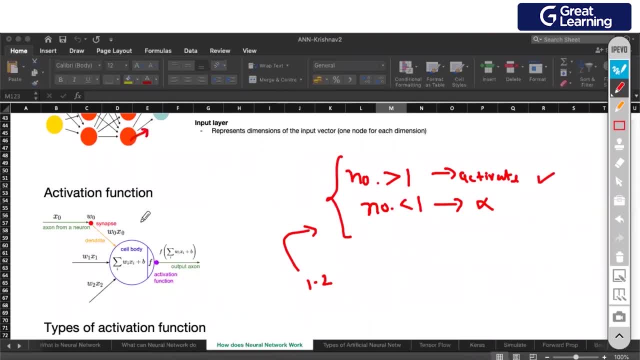 that current neuron is active. pass the number to the next neuron. allow the number to pass through. these are called activation functions. this is a simple one. i've shown you. okay, let us dive deep into this activation function theory. so there are so many functions available like this. we'll go one by one before that. 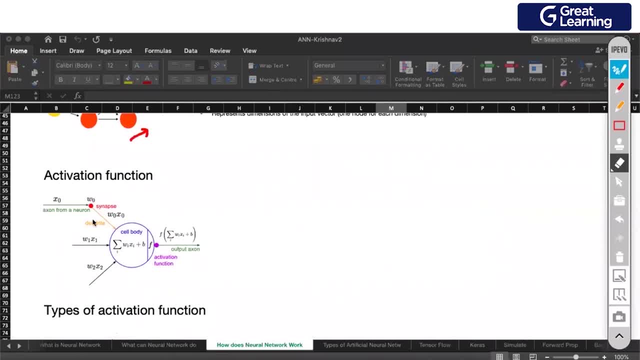 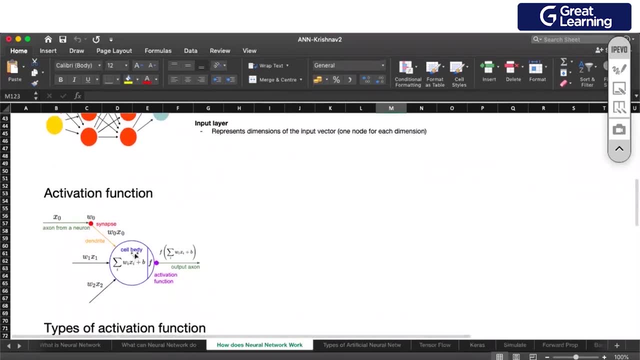 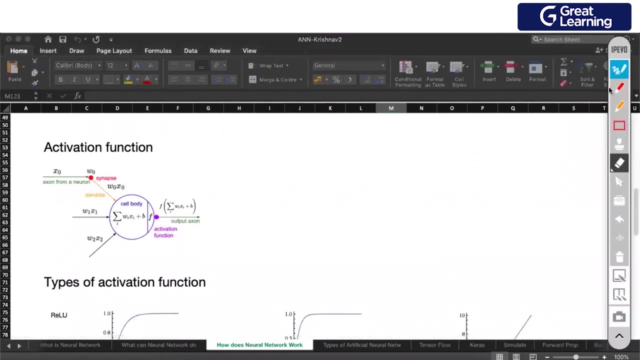 let me show you what happens in the neural neurons. so imagine this is one neuron, this one and this neuron i have represented here, for example, any of the neurons, all of the neurons have same kind of look. what am i doing? i'm giving some input to a neuron. this is my input. x is zero. 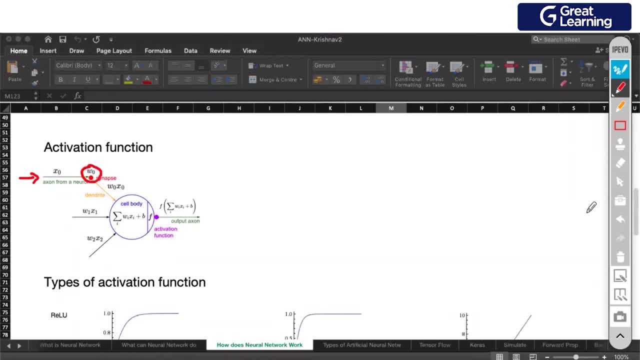 there is a weight. and if you ask me what is this weight, i will say: randomly chosen number. okay, during your forward propagation, when your, your network is built, we randomly assign some number, say r, a, n, d, n, and we put some number. yeah, that random number gets multiplied. 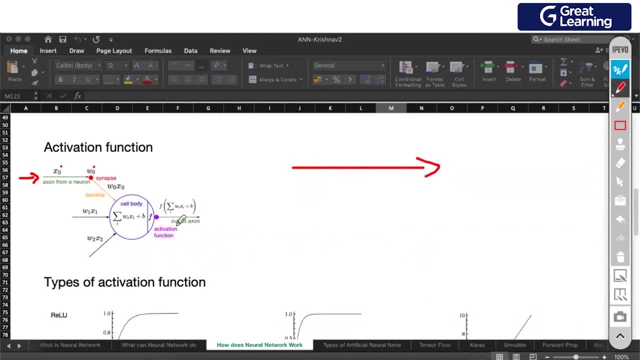 with your input to become w0, x0. that w0, x0 from the other neurons, we get w1, x1, x1, w2, x2. so these are inputs from other neurons. all right, all three of them are coming and converging here. so if you want to see an example, just have a look. 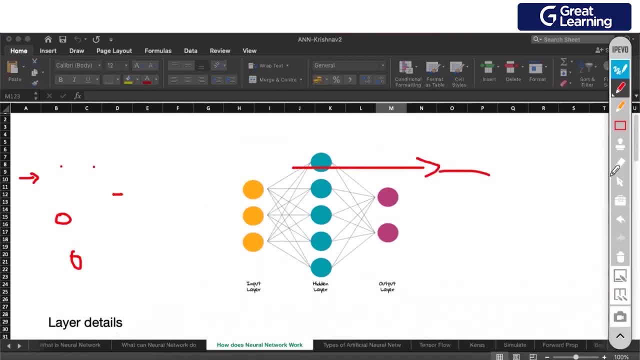 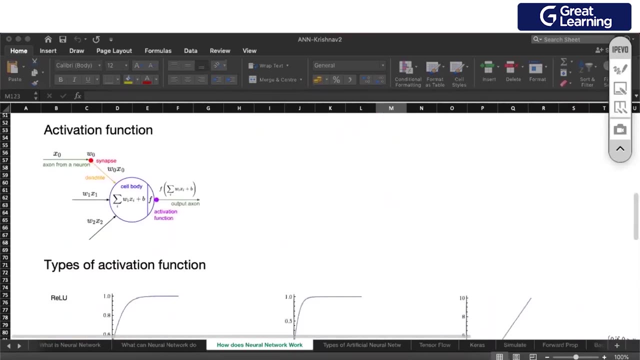 here. so if i say we are talking about, say, this particular neuron, how many inputs are coming? one, two and three. so this is my x, 0, x 1, x 2, all right, so you can imagine that way: now, inside this cell, inside this neuron, what do we have? we have an activation function. 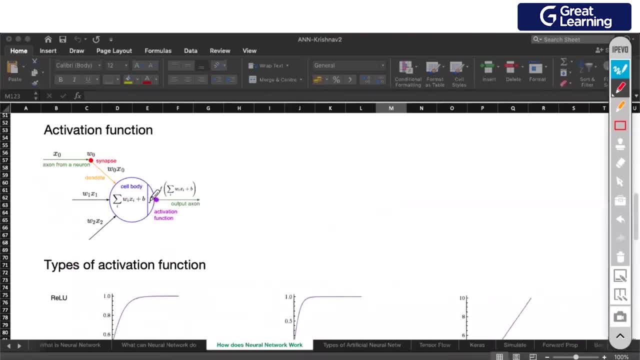 we call this as an activation function here, f, and also there is one random number called bias, which we have to add it with our addition of all three of them. so if you observe here what is this? w 0 x 0 plus w 1 x 1 plus w 2 x 2 plus. 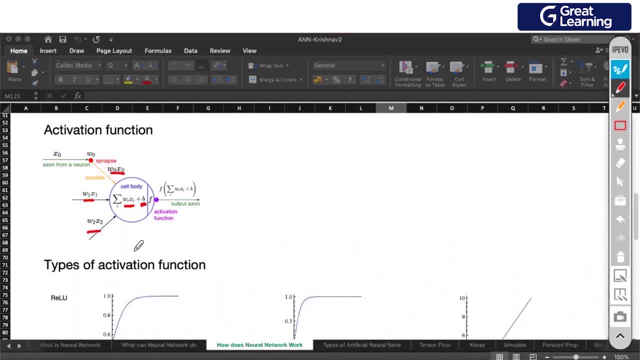 some random number called biasing factor. all right now, if this particular operation is greater than certain value, the l, it is allowed to pass. if it is, if it does not satisfy my function, it is not allowed to pass. okay, now let me see. let me show you what. 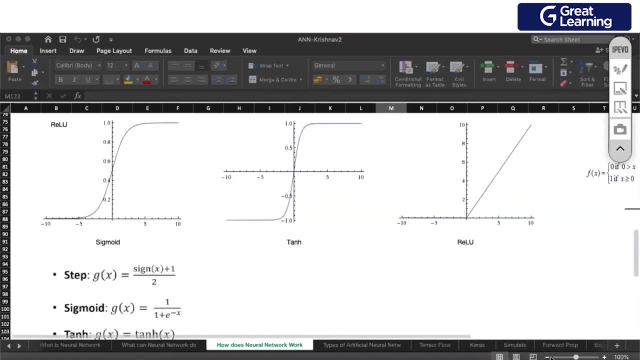 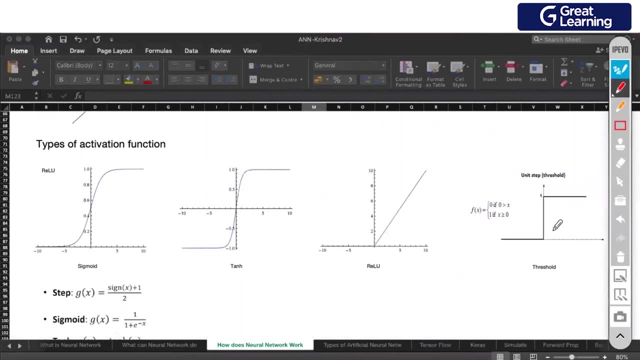 are these functions? so if you observe we have got looks like very complicated activation functions, but actually they are very easy. we'll start with the easy function, this one. have a look at this: unless and until your output is greater than zero, it will be, or else it is zero. this is. 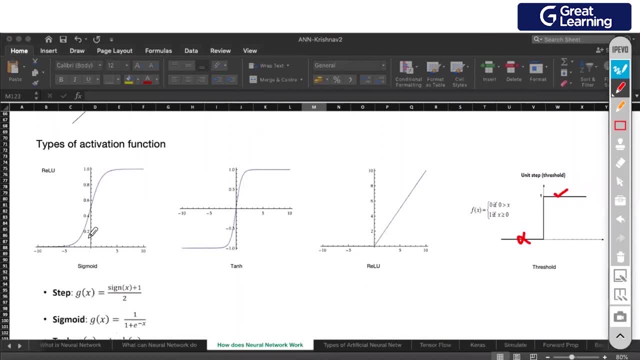 called step function. second one is: say, if you have a function which you could want to customize, so let's call this segment function. now this segment function is considered to be regular. well, let's say, in tw Spielberg it's very complicated enough, so this segment function is going to be. 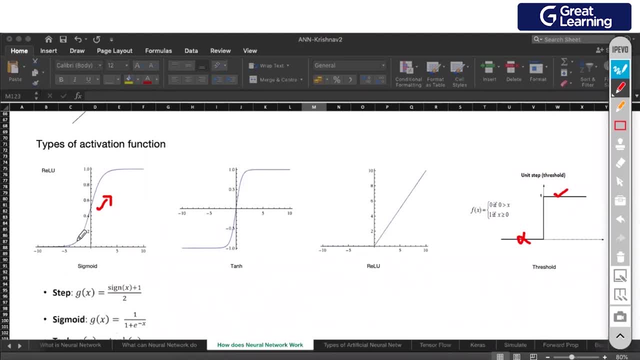 required. okay, so let's remember what is your segment function has its function. if your input is between, say, this phase and this phase, it will continuously increase. if your input is less than this, the value will be zero, and if your input is more than this, it will be a static. 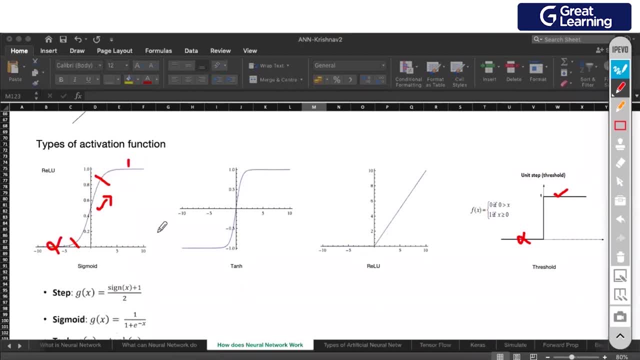 value of one if you expand this a little bit more, okay. and one more thing: this is not relu. i don't know why i have written relo here. this is wrong. this is sigmoid. and if you expand this little more on the depth part of it- but you have to cross through zero- that becomes your tangential function. 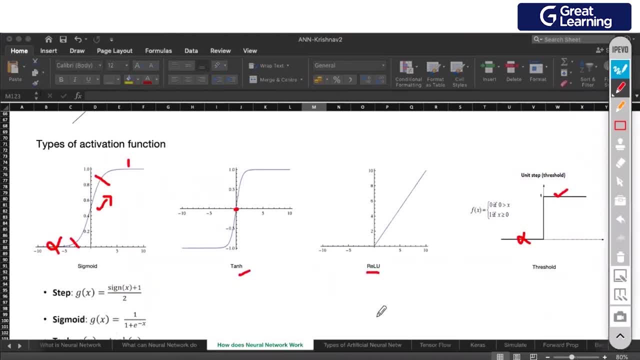 all right, third part is called relu. okay, so what is relo? basically rectified linear unit. so if it is less than zero, it is permanently zero. if it is more than zero, it is a linearly increasing curve. this is one of the most popular activation function we have used. we are using, actually. 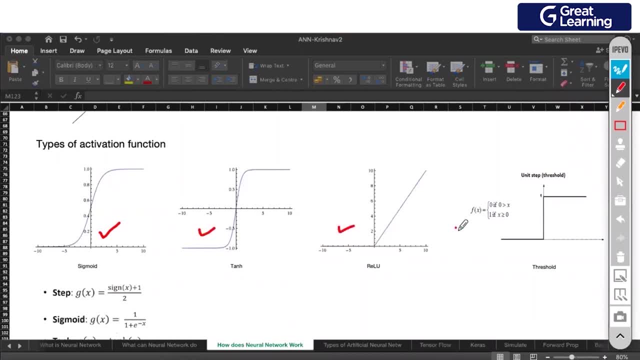 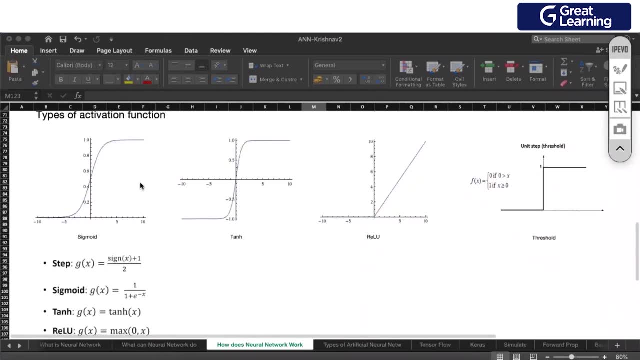 so, depending on what type of inputs you are having, you can use one of these. so, down the line, when i train, when i will show you guys how to write case studies and how to decide your networks, at the time we will try to choose all this stuff as per our data. yeah, and there is one more important. 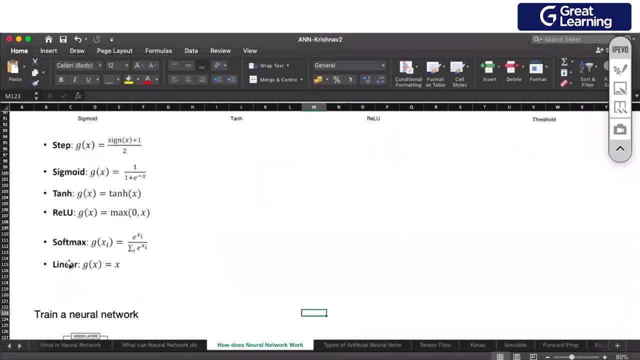 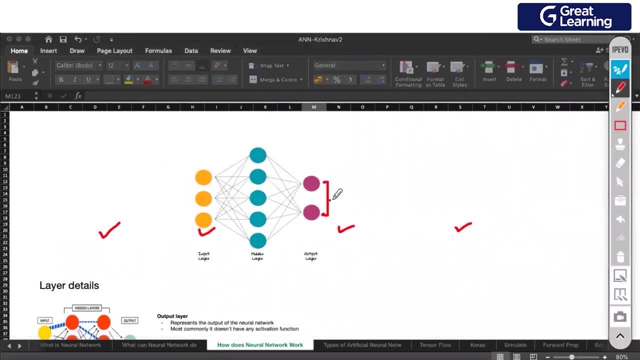 activation function called softmax, whenever you have a categorical output. now we just saw that you. there are two type of possibilities over here. the output could be categorical and output could be regressive correct, the same thing we have done in machine learning. also, if your output is categorical, the default function, activation function- you will use only on output. 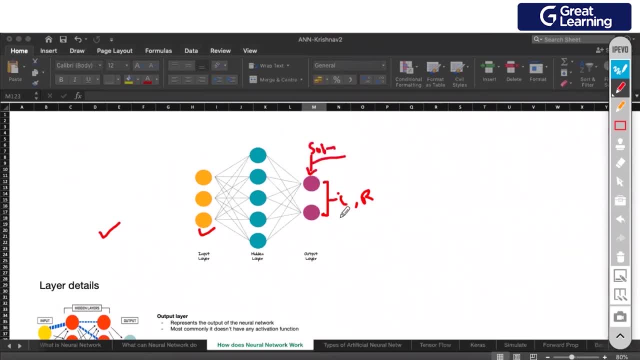 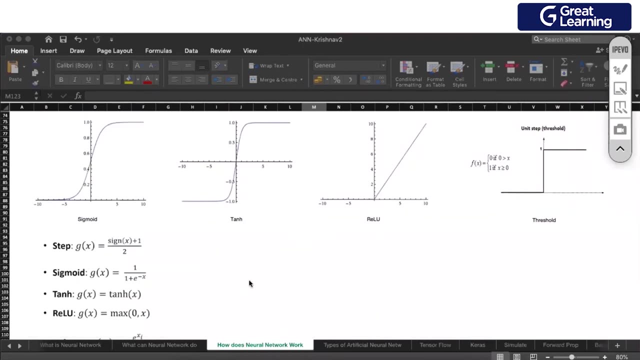 layer is called softmax. it is a categorical activation function. if, in case you have no categories, you have regressed outputs, regression as an output, in that case you can use any of these categories. are we clear? all of you true, yeah, yep, so how? what are these functions? and all we will 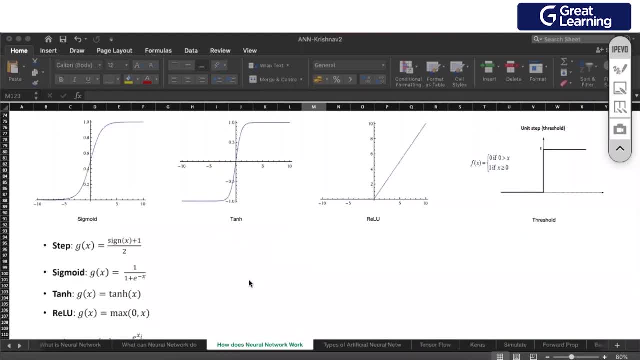 see when i show you the stuff. but for now are we clear. we have sigmoid and relu and threshold. these are some of the most important ones, and why do we need it? just to manipulate our number and let it pass forward. that's it all, right now. moving on to 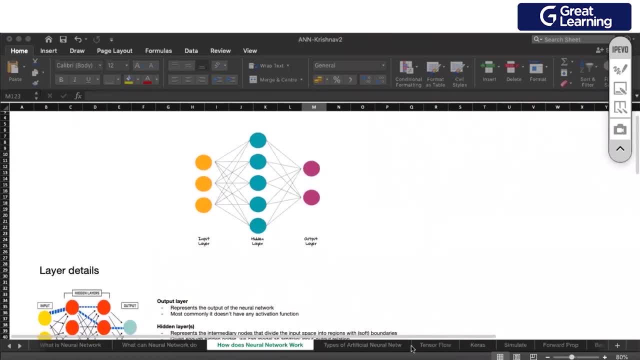 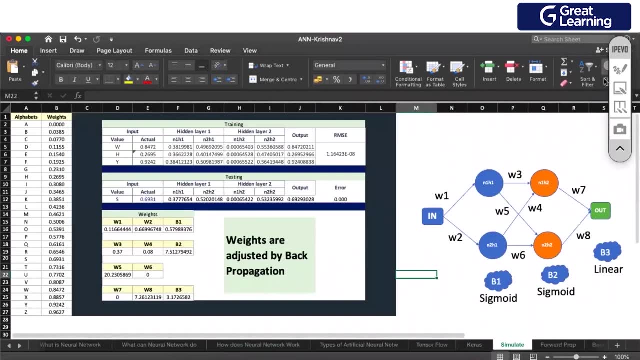 the next step. so this is how overall, on a very high level, neural network works. now let's try to simulate one. so i have simulated a neural network in excel file. now let me show you what it is now, please. we cannot do this on a higher level, but on a very simple neural network. you can train it up. 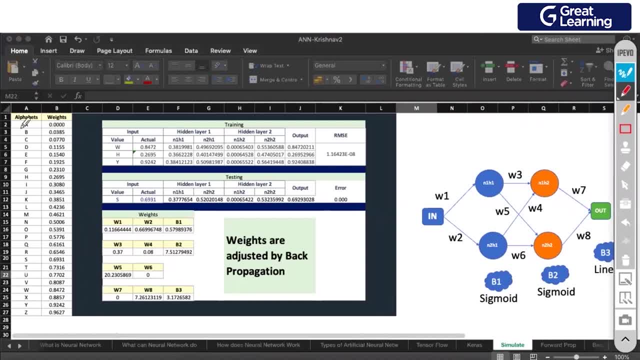 now observe my network. so, as an input, what do i have? i have got some alphabets from a to z. now, please remember, computer does not understand what is a, what is z? what we do is we do somewhat cheating at the back of the screen. at the back end, we tell the computer that if this is the number, it should be displayed as this figure. 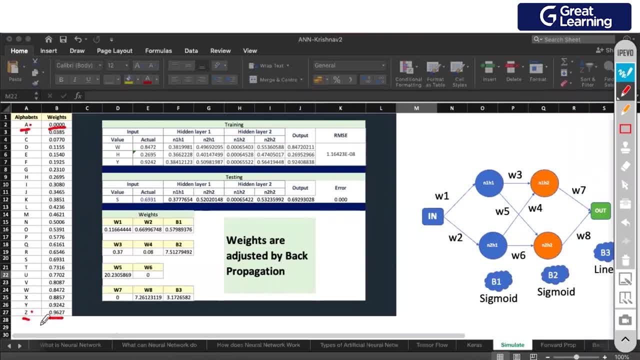 if i get this as a number, it should be displayed at this figure. everybody agrees to that. yeah, binary logic and all. if you have studied in the computer science and all this is what it is. same thing applies in neural networks also. so say, for our sake, what i have done is i have taken a to z. 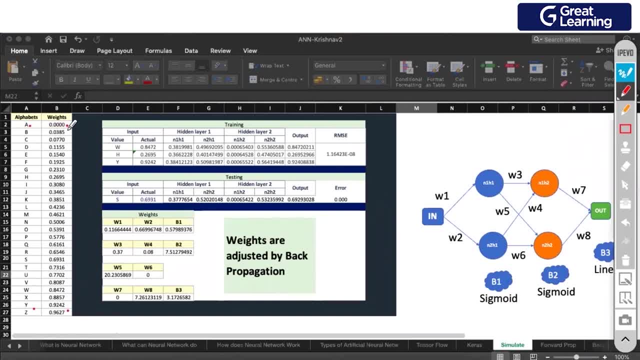 and i have divided numbers between 0 and 1 in 26 equal distances. all right, what is my job now is my job is to train a network such a way that, when i give, when i say that w, h, y- okay in english spelling- it should also give me the same numbers as an output, but in the form of. 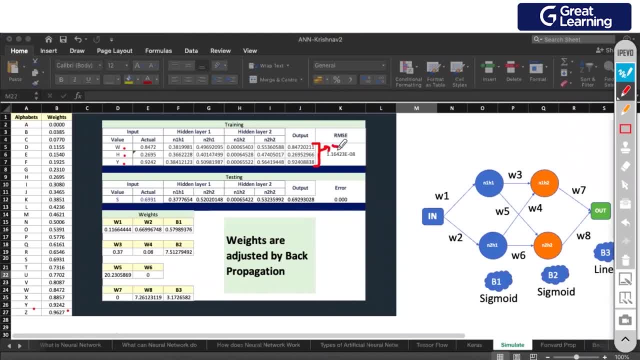 numbers, and then we will map it up in the form of digits, sorry, in the form of letters. all right, now let me show you what exactly are these calculations and what we have done before that. how many inputs do i need? so if, if you remember, i say total number of independent columns is equal to your inputs in this, in? 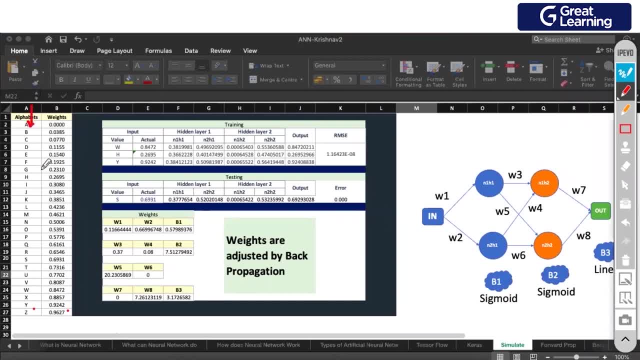 this case, can i say i just have one independent column, which is a agreed, so i will need only one input. how many outputs do i need? it is okay, first of all, what is it? is it a regressor or a classifier? it is a classifier. look at the numbers. okay, uh, one way you are right, because we are. 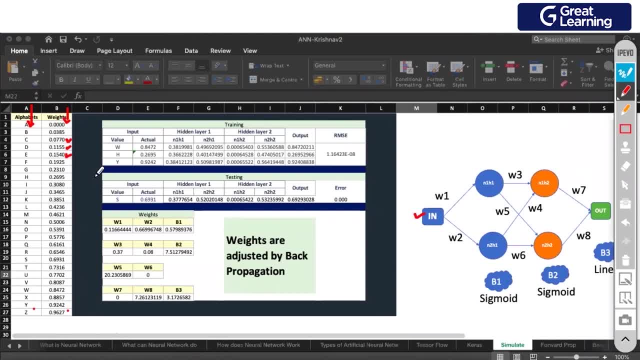 passing abc, but in this case we do not have softmax in excel file. so what i've done is i've made a regressor and then later on we'll. we will try to classify, but perfect answer. so it's a classifier with one output. so this is one input, one output. all right, and then you may ask me, okay. 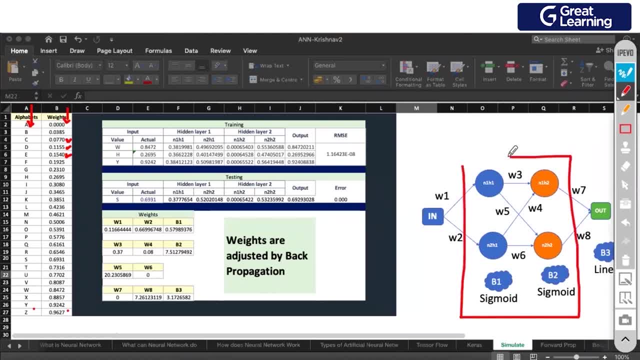 what are these other things? these are my hidden layers. you will see down the line. what are these and how i design this. all right now. let's try to pull one number. say, i pulled out w. what is w? equal 0.8472? that is what my actual value is. this is my actual y. all right now. what i'm doing is i have 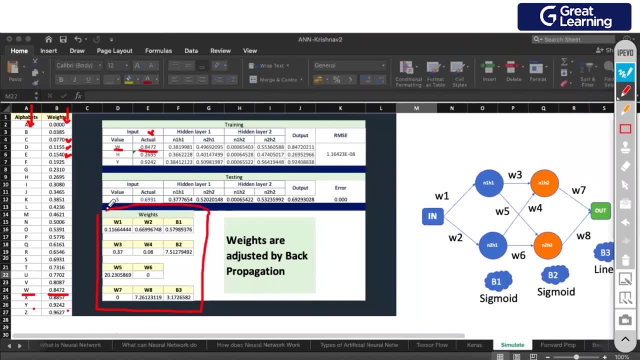 to choose some random weights. do you people remember we talked about weights, randomly chosen data. now let me randomly choose some weights. so i will make it say 0.8, uh, four, five, four, two, 45. uh, say 80, okay, 67, some random number, whatever we like, all right. so i have chosen some number as my weights now. 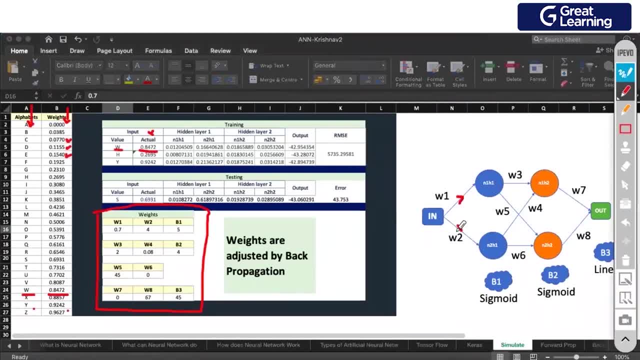 what are my weights? where do my weights lie? my weights will lie on each of this line. so this particular weight- 0.7- that you are seeing- is a weight given to this line. so when my input- 0.8472- goes to this particular neuron, it gets multiplied with this weight. 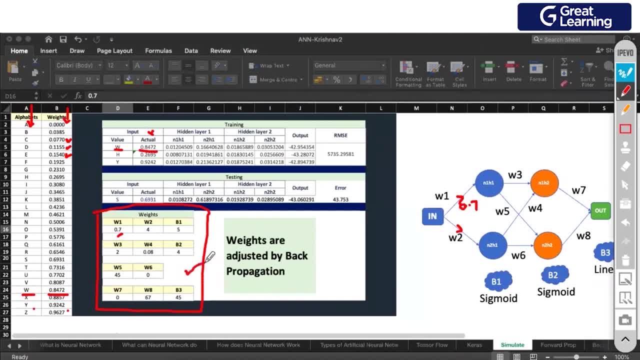 are we clear onto that everybody? what are these weights? this is my biasing factor and these are my actual weights. okay, guys, do let me know. are we okay with this any? any issues with the concept is fine, but just one. just one thing. i don't understand how this random. 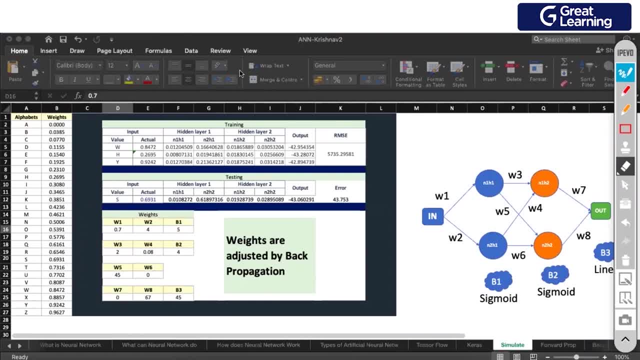 number comes in picture, because when we say that the output is dependent on the input as well as the weight which is coming up, so the weight, the number which we are choosing for the weight, is something which will influence the output as well. exactly perfect. so what is our job then? to back, propagate and 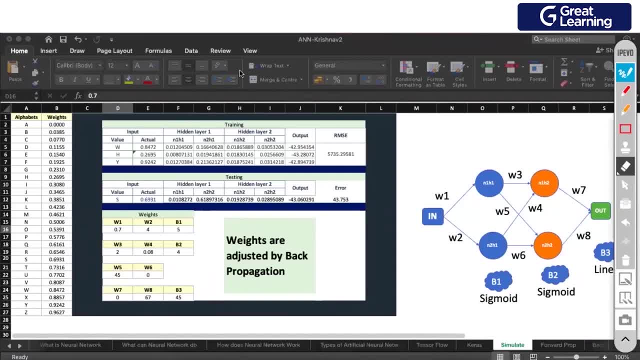 Adjust the weights such a way that my actuals and my prediction should match. Okay, So basically that's part of learning in this case. So, Exactly, the whole game here is to adjust this weight such a way that The output that we get here matches my input. 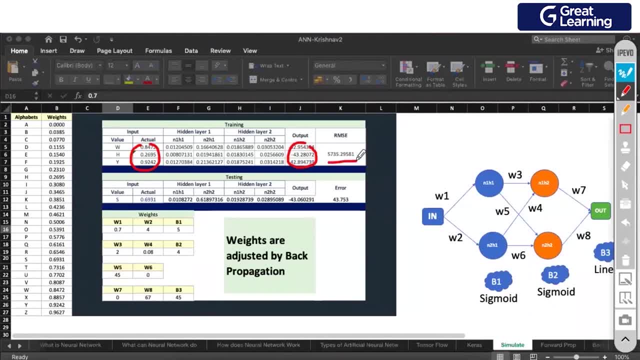 All right. Do you see now output input matching? Not at all right. Look at the loss function that I put: RMSE. That is around 5,000 plus odd something agreed. So whatever we Sorry, what is? what is the problem that we are taking here? 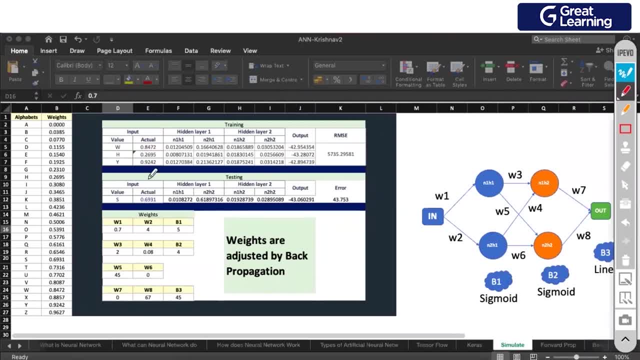 The actual and the RMSE output that you have. What is the Okay? so the first thing, what I did was I Multiplied my this with my current weight and Activation function. I have uses sigmoid onto that Now you have. you may ask me what, from where I got sigmoid? very simple: we wrote a. 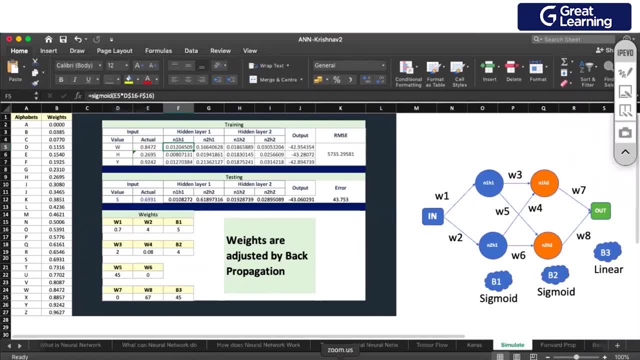 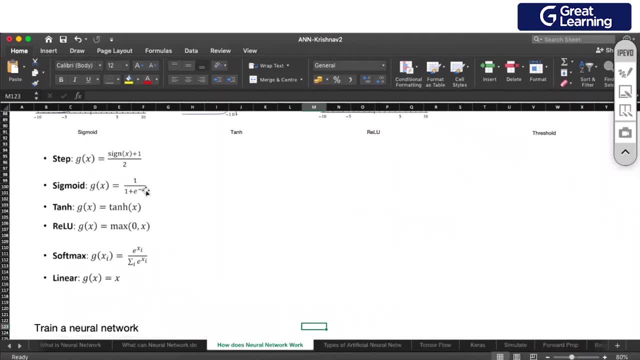 Logic here or a macro over here to simulate sigmoid. Now, what is sigmoid? on a very simple scale, sigmoid is defined by 1 upon 1 plus e power of minus X. What is my X? X is one of my inputs given to the sigmoid function. That's it. 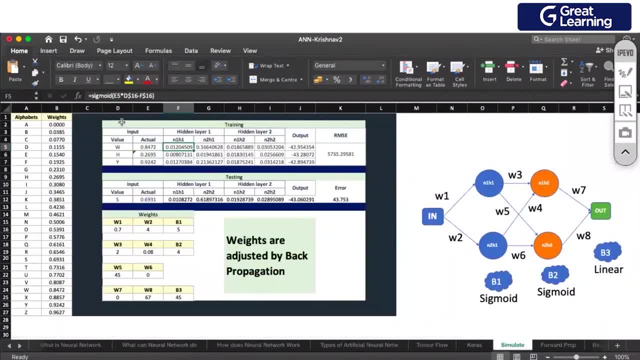 so What I've done is I have my own sigmoidal function where what I'm doing, if you observe the formula bar e, 5 into This one- Okay, got it. yep, minus my This one- what do you say? Bias factor? and I sigmoid it up. That means I, whatever manipulation I am doing down the line. 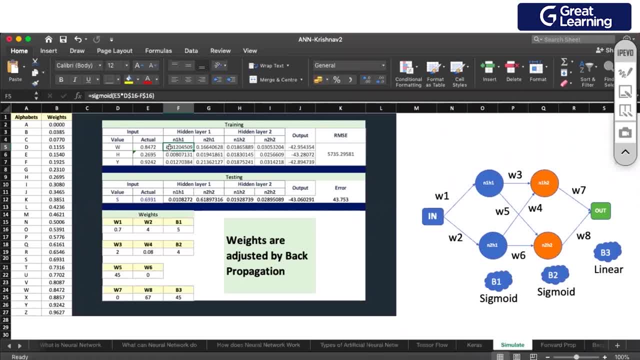 I am putting a sigmoid onto that, and when I put a sigmoid onto that, the value that I get is zero point zero one two, Which I have perfectly spoilt it up, because my original value is 84 and the value which I do after multiplication Is little weird. 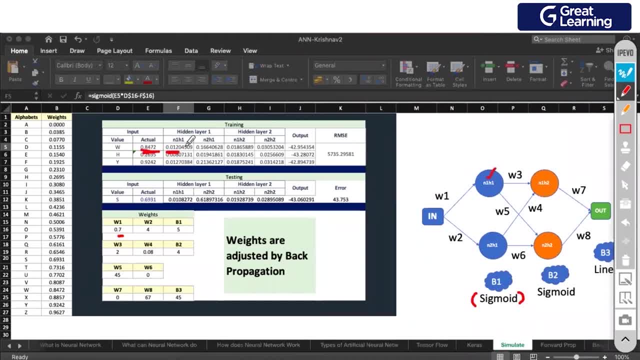 Okay then. so this is my n1 h1. same way I take this up multiplied with next weight, Put a sigmoid on to that and get this Okay. third one is N1 h2. so this one. so, if you remember, if you see here now, now we are getting inputs from two of them. 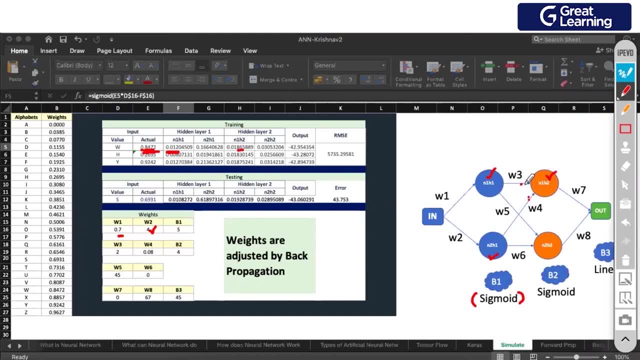 We are getting an input out of n2, h1 and also w3. same thing: Whatever goes out gets multiplied with the new weight Three. we'll put a sigmoid onto that as an activation and we'll throw it out. Alright, so our data is propagating from here to here. 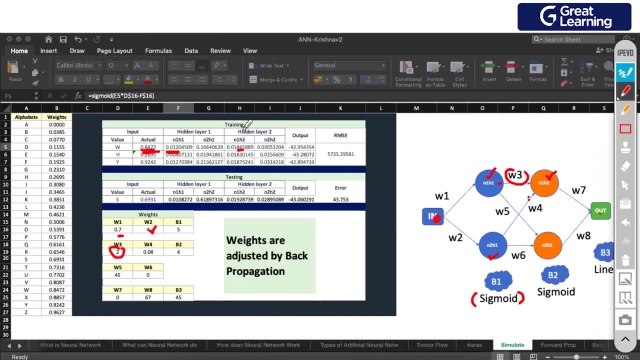 So when my this particular data propagates from here to the output, it becomes minus 42. And if you ask me why? it is all because of junk weights that we have put Agreed. everybody agrees to that. the weights are causing this issue, Right? so what? 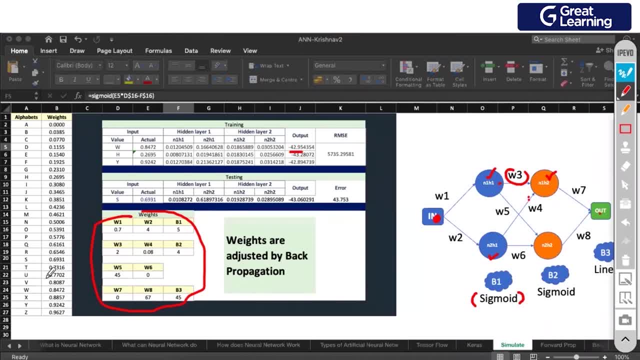 What we should do now. if weight is responsible for making this issue, We are supposed to go back and change the weights. now How do we do this? in neural networks, We call it back propagation. I will explain you with formula now, but for now, in excel file, What do we have is mean inside data. 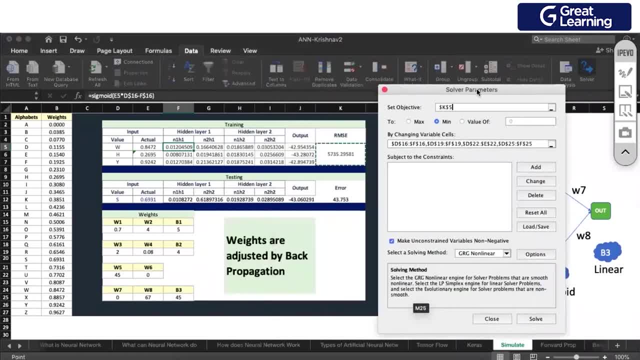 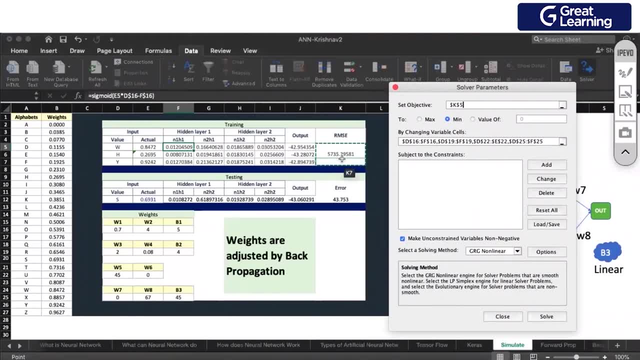 We have something called solver. I don't know if few people have used it. My intention here is to reduce my RMSE. now, Everybody knows What is RMSE. right Root mean square error. It's a loss function. What do you mean by loss function? 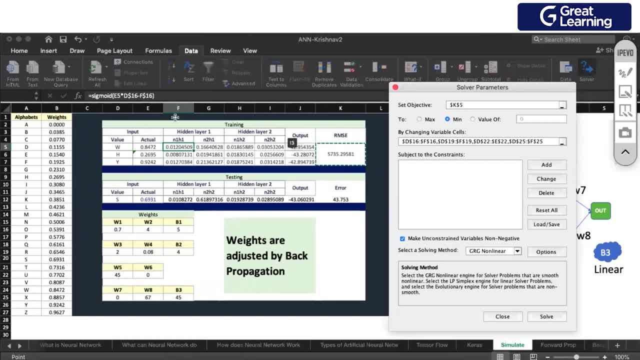 difference between my output, Predicted output, and the actual output. that is what we call is loss function. Everybody is ok with this RMSE. Alright. now, what is my intention here is to focus on my RMSE here, and My intention is to reduce my RMSE- agreed. 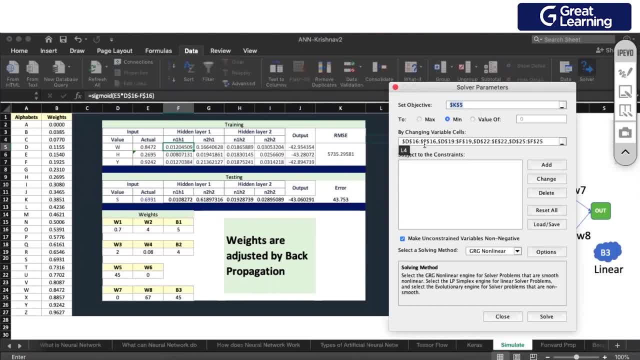 Yes or no. yes, Yes, we'll go to the formulas now. after this will, I'll show you in derivative way how to do that. next, what is my intention here? what I need to change such a way that my RMSE should reduce. can I say all of these junk weights I have given those? 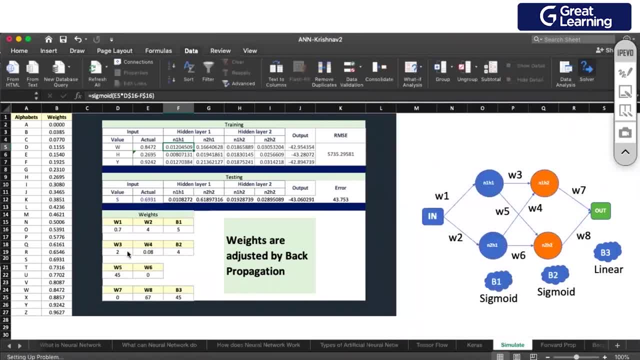 weights over here. now let me click on solve. it'll take some time, but you observe the weights changed and the weights when the weights are changing. now can you look at my RMSE? from 5,000 odd it has come down to almost 0. you 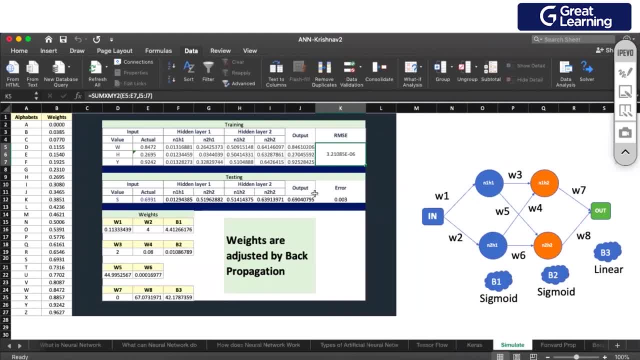 agree, 3.2 into 10, power of minus 6 is almost 0. yep, and look at my output now and look at my input now, can I say they are almost in sync, yes or no. so can I say I have designed a network here such a way that tomorrow 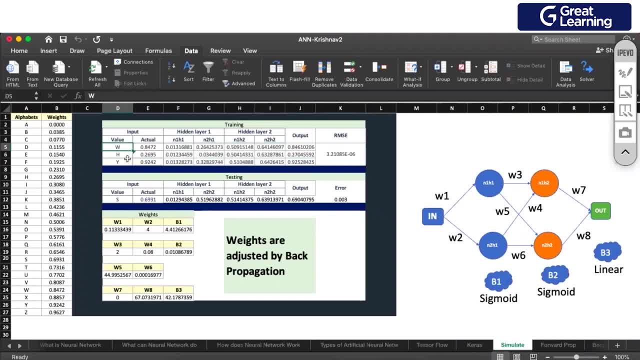 you, if I give this particular value, it is going to identify that it is W, or at least, if I give this value, it is going to identify it is. are you able to visualize that? now? let's test it. let's try to test it. so, for example, I have: 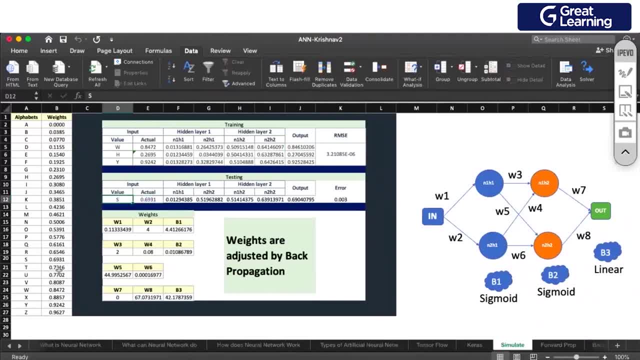 given a value, s. here s is what. what is the value of s is zero point six, nine, three, one. okay. so when I give the value, automatically all the calculations are done and the output that I get is zero point six, nine. zero four, zero seven, five. how I got this using these weights and the error that I currently get is: 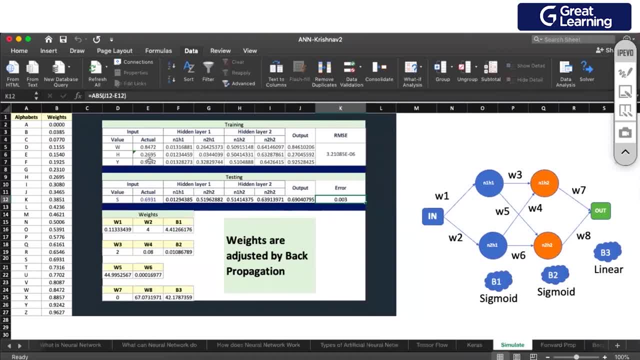 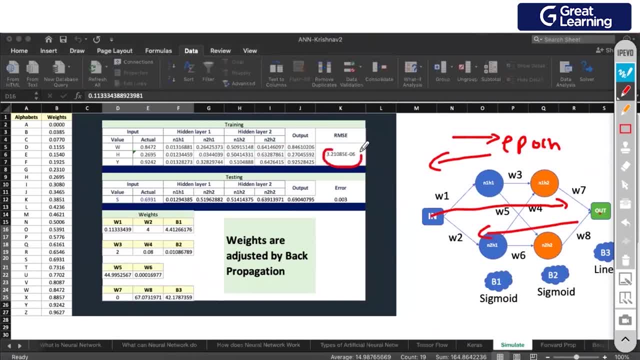 back till I find my loss function to be minimal, till my weights are adjusted to the very best values. this is the high level overview of neural network. so the solver, whatever it did, right. so it's. this is very, very easy and good to understand. the solver was just trying to adjust the weights and keep keep. 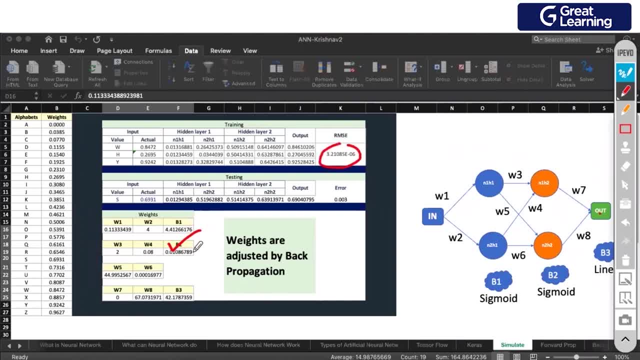 iterating, is it? probably it would have done whatever 8 to 10 epochs to get the right value correct. okay, how does it just just? is there any way? yes, there is a way to adjust that, so let me show you using formula. but before that I'll be. 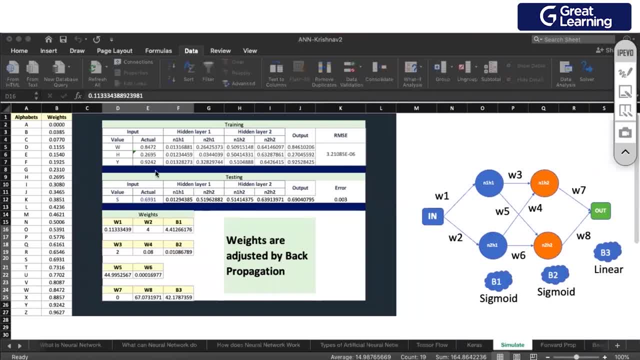 clear with two processes: forward and backward. now if I say for forward prop and backward prop, you will be able to visualize what I'm talking about. forward prop is your activation functions. backward prop is adjusting your weights. all right, yes, we'll come to that. we'll come to that one by one. don't worry about how do. 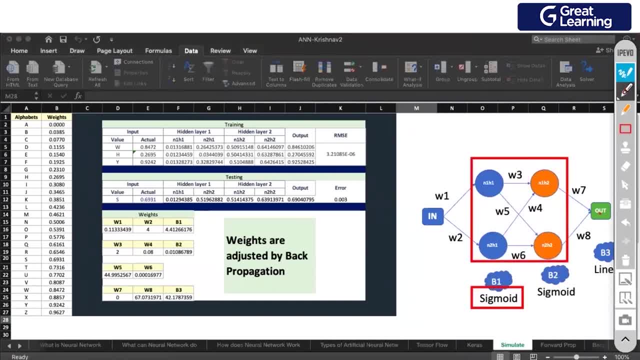 we put it and how to choose this and all. we'll go deep into that. and you also said that some of the neurons may not get active because the activation may not happen with all the neurons right. so how do we demonstrate it in this example? in this it's not possible in excel files. we have a limitation here of only using 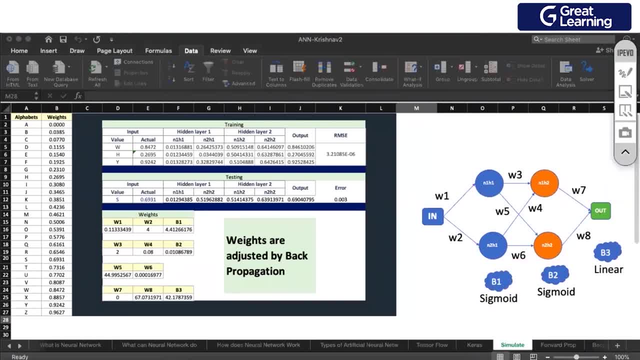 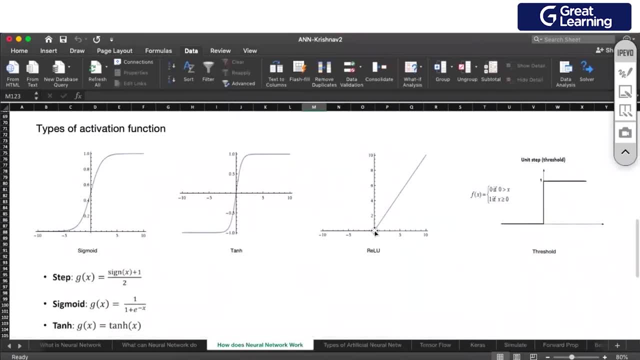 sigmoid. so if I use ReLU, so if I use ReLU, I'm not going to be able to get the right value. so if you look at my ReLU, if you look at the ReLU, any value which is in negative will be switched off. agreed, yes or no? will this ReLU allow us to? 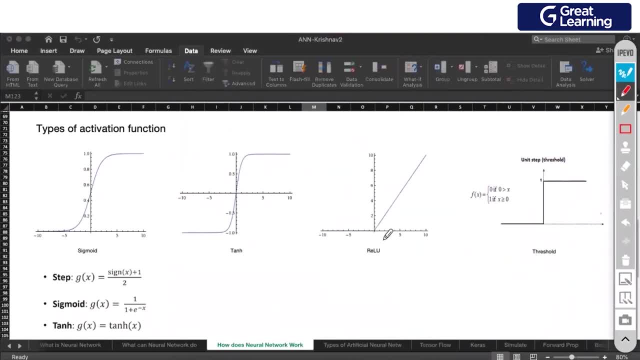 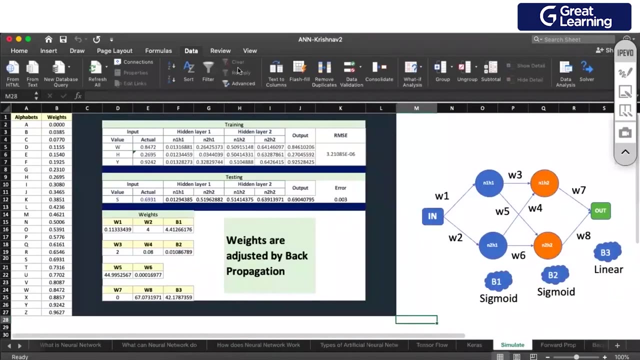 pass any negative value. no, no, it will be clipped off. very simple. you will see this in Python, Ramesh. and one more clarification: Krishna, can you just go back to that picture? see, like, from input to this NH 1, this W1 is getting passed, right. 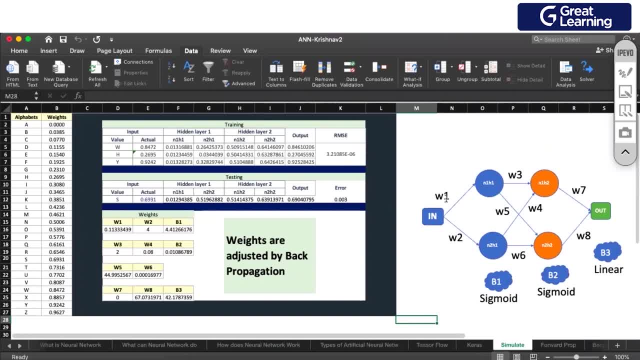 will the activation function work here or from NH- H1 to NH to only the activation function will work. yeah, activation function resides here: N1, H1. the multiplication happens here and then it goes to activation function here. okay, so from input the activation function will not work, only when it goes to n1, h2, the 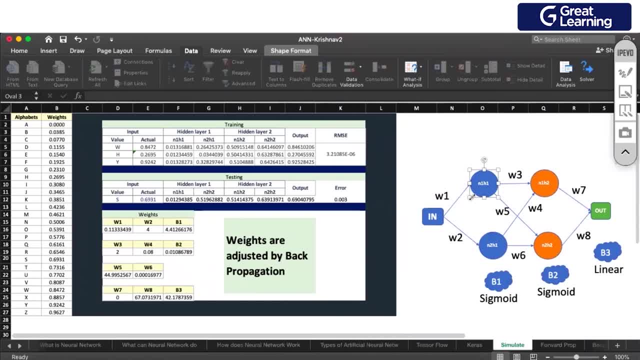 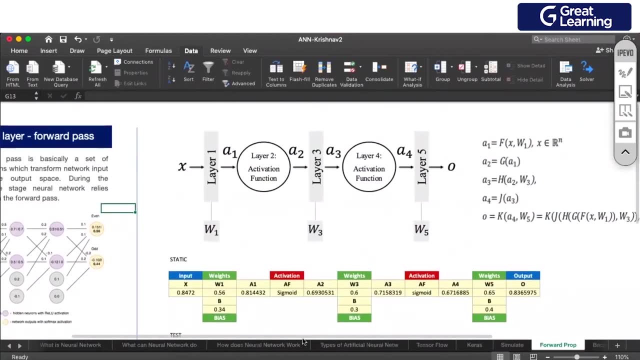 activation function will get: yes, right, yes, perfect, perfectly, yeah, yeah, thanks, all right, good, now let's come to some heavy maths now. so now you might, you people might- feel it's getting little heavier. so what do we do? so let me explain you. forward propagation in a more. 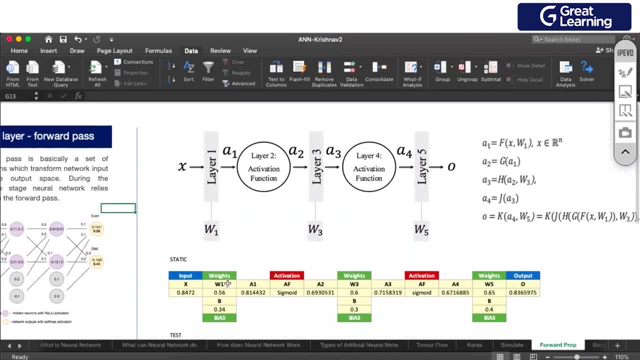 complex way now. so now, when i talk about weights, layers, activation function, now you will be very clear, okay, so now we'll not repeat what is activation function? now let us say i have got a weight or input, x. x gets multiplied with w1 weight of that line and i get alpha one. 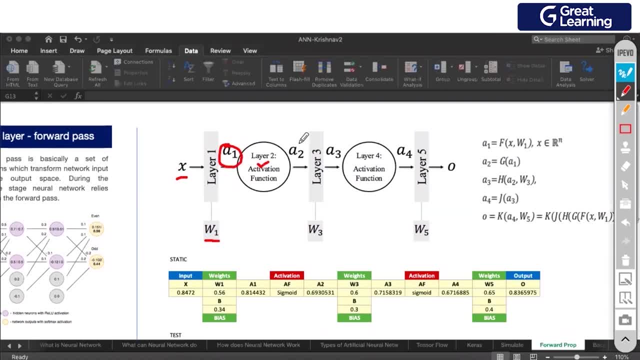 which goes inside an activation function. i get alpha, which gets multiplied with my next weight, and i get alpha one which goes inside an activation function. i get alpha and gets alpha three. alpha three or a3 goes into new activation function. it becomes a4. a4 gets 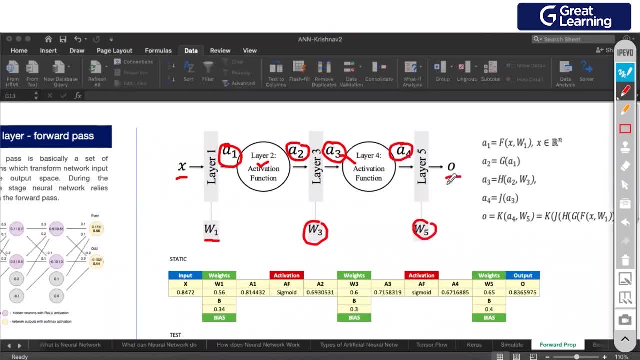 multiplied with some weight and i get my output. this is your forward propagation. okay, now the same thing you can see over here. this is my input, this is my weight one and if you remember i said there there could be a biasing factor, it is again a random number. we use it. so this into this. 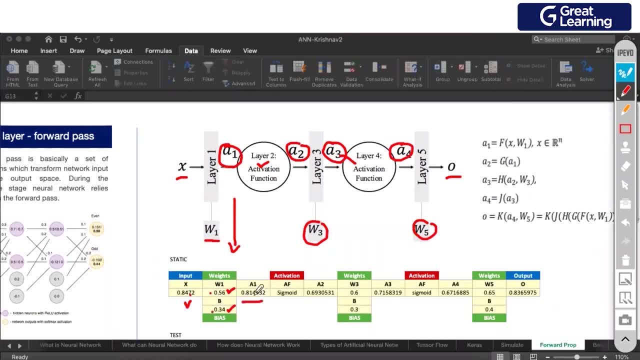 plus, this becomes this. then i pass this through a sigmoid function. so when i pass 0.81 through sigmoid i get 0.6939, that is your alpha 2. this one same process happens till you reach your output. so if you now observe, our input actually was 0.84 and because of this, whatever we did in middle, we 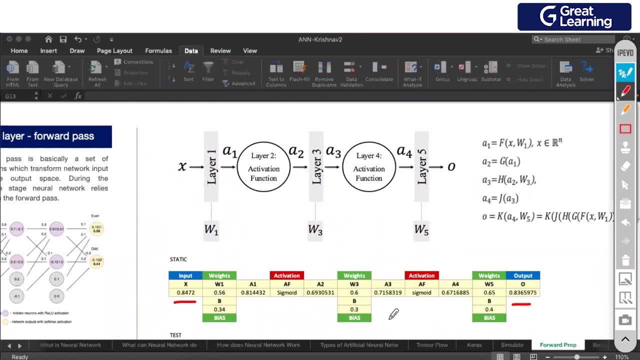 got some loss of 0.83 right. one question here: this weights and bias numbers, what they have input here. is it just a random number or random numbers? random number: see, if i change it. if i change this, it will change. do you? did you observe? it's changed values. it should be in a float only, or any. you know anything? 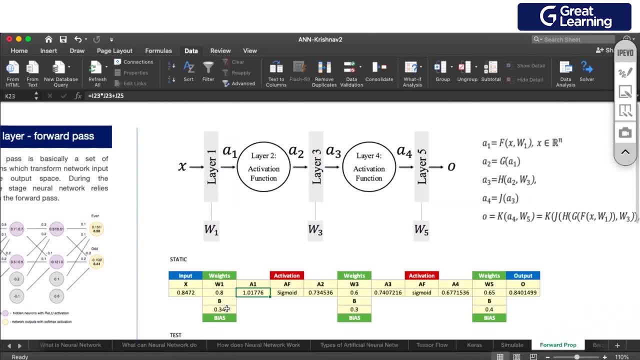 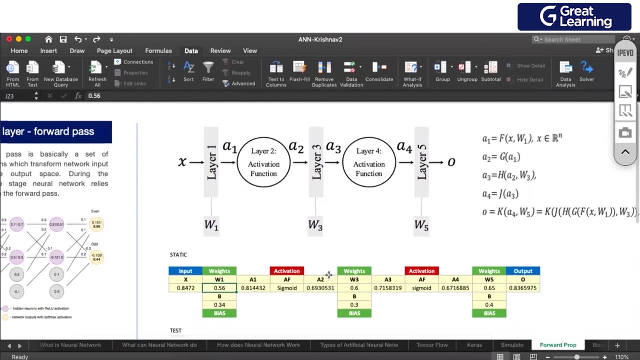 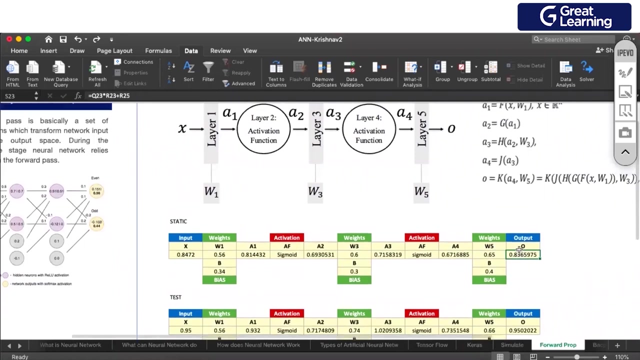 actually float is better. integers. uh, there is a function which will allow us to put only integers, but then there are some problems with that. i will show you why. all right, okay, so this is what is your forward propagation? now? any questions onto this? how this value became this value? any questions? perfectly clear, so you imagine, if there is a 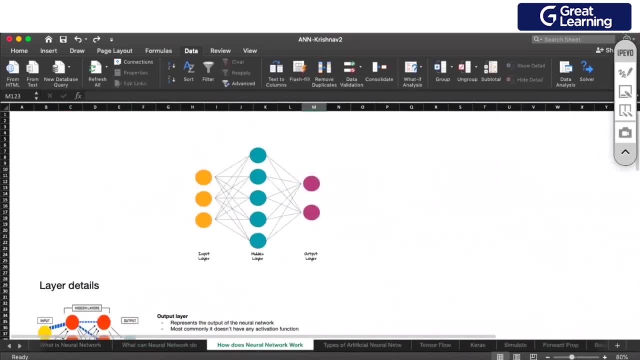 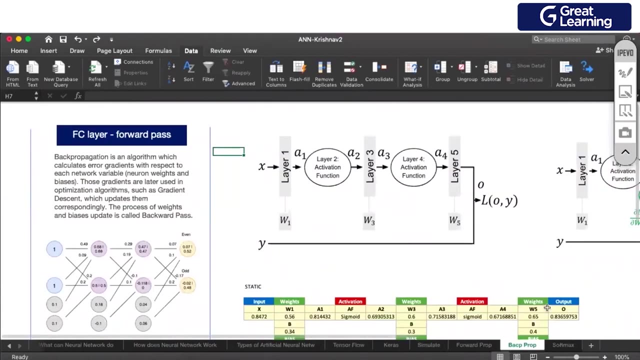 bigger network like this. say you have a bigger network like this. now, if i ask you guys, you know what goes in and what comes out. are you clear with that forward prop? yeah, yep, good, now let's talk about what happens in the backward prop and how those weights are learned now. so 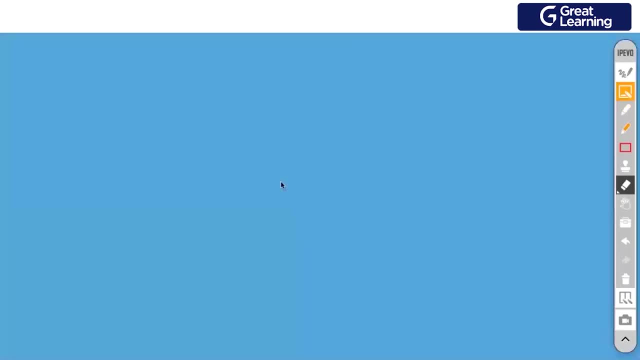 before moving on to backward prop, i will ask you guys a very simple question: what all type of loss functions you people know so far? what are loss functions we know? let us say at least three of them we'll talk about. what do you mean by loss function? why pred when compared with y actual? 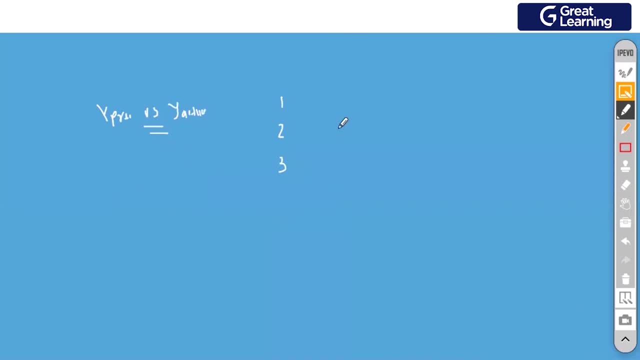 that's your loss function. how do you compare it? subtraction, read, distance, how far they are agreed mse, and i say rmse. yes, these are some of the loss functions that we know about right now. let's come to the scum function. now, let's come to the scum function. 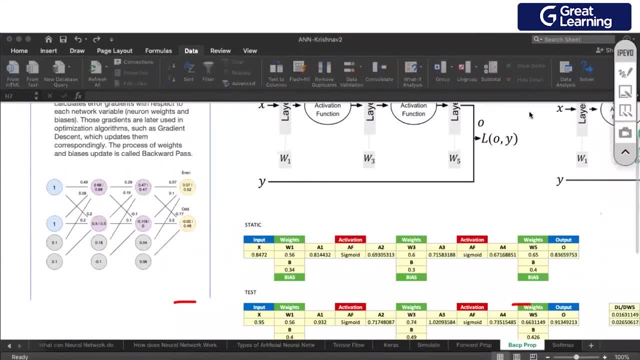 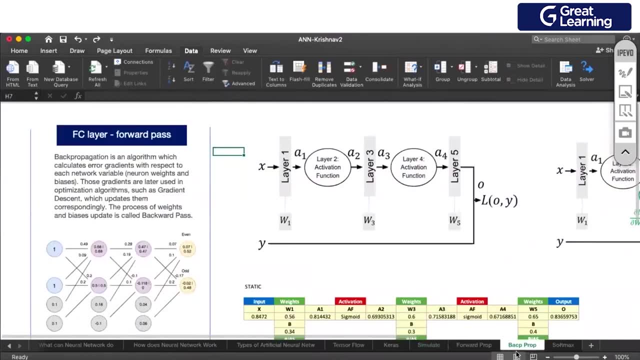 now let's come to the complex part of it now, how actually we learn the weights. now it was very easy for me to use solver and show you. very easy because you have a ready-made function. it worked. but what happens in the neural network? how network understands this? so say: this is your output. 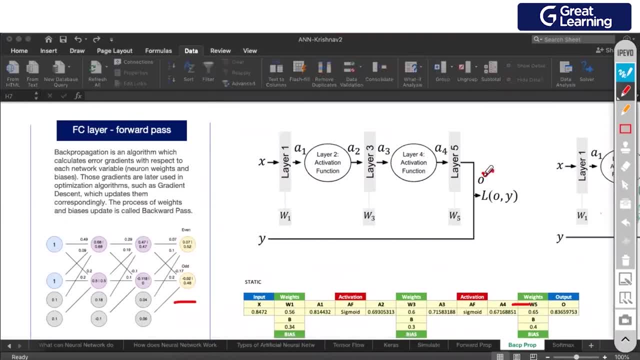 okay, so this is what you are supposed to get, and, sorry, this is what you got, and you are supposed to get y as an output. this is your actual, this is your predicted, so if i have a function which will take care of, what is the output of this function, so this is what you are supposed to get and this is. 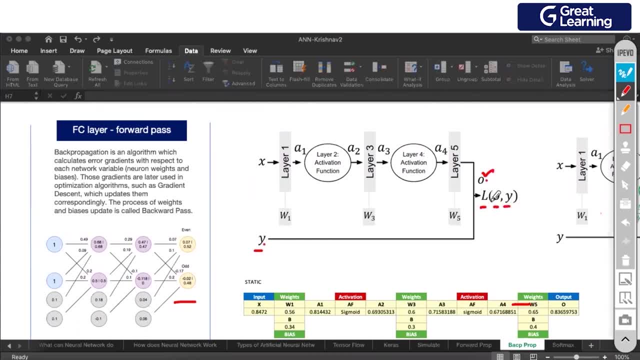 what you are supposed to get and this is what you are supposed to get and this is what you are supposed to get versus y. i will define this l as my loss function okay and what we need to adjust. you put the things which are in scope, so my current for my back propagation, only the highlighted part in red. 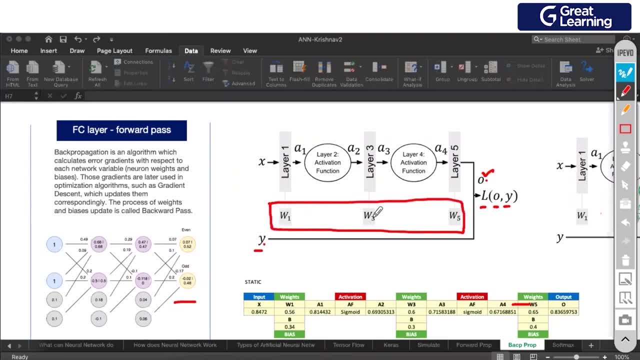 is in scope. that means we need to alter one of them or all of them, or combination of them such a way that my loss function is decreased. all right now, which mathematical function helps us to do that? my intention is by how much my loss function will change if i 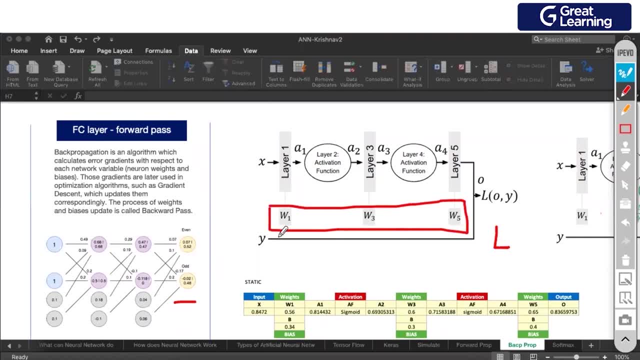 alter these? what kind of function we can use here? from our school days you can recall some functions. we have done this. you people know it, but we we don't know the real application of it. differentiation, perfect, perfectly identified. we will say by how much my loss function will change. 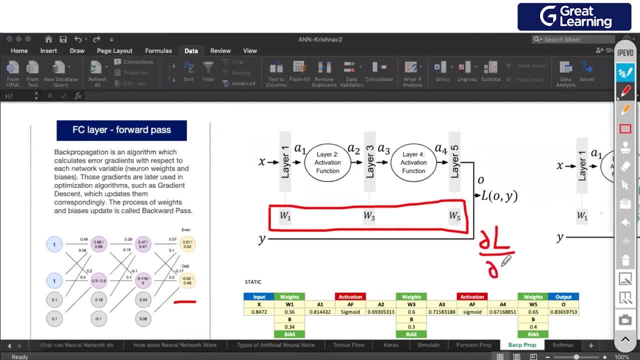 function will change if i alter, say, weight number five. everybody is okay with this. differentiations: yes, it's a step function, so by how much i should change so that this will reduce? very simple. now, if i want to develop a chain rule here, okay, now how do we do that? so now you may ask me, fine, 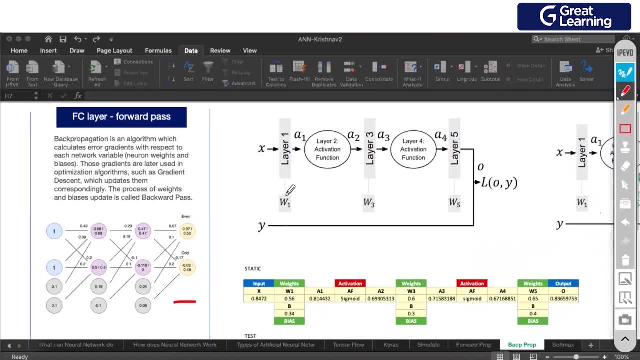 we got a differentiation, but how do you say which way to change and how do you derive the equation? so for derivation of the equation, we'll put here, so it's not needed, but it's just for your understanding of backdrop. i will say by how much my loss will change with respect to my 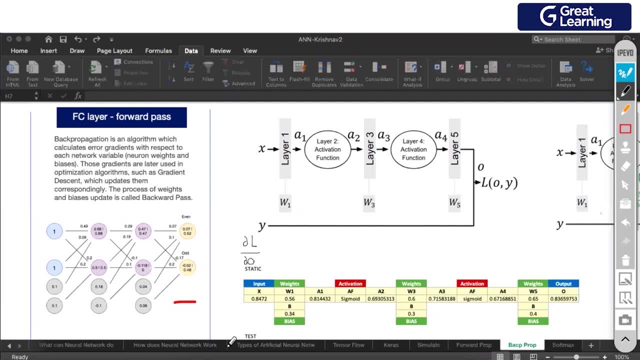 actual output that i have got, sorry, predicted output that i've got. that will be my first differentiation multiplied by how much my output will change with respect to my weight number five. okay, 粵 three should change with respect to my weight number three. how much my weight number three should change with respect to my alpha two? agreed, guys, you. 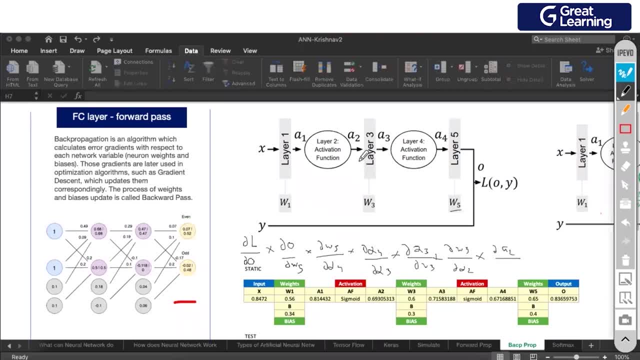 getting it, how much my alpha 2 will change with respect to my alpha 1 and how much my alpha 1 will change with respect to my weight 1, and we go anywhere further. no, no right, because weight and X is not dependent on each other in any way. agreed, now just think about it if you want to just focus on. 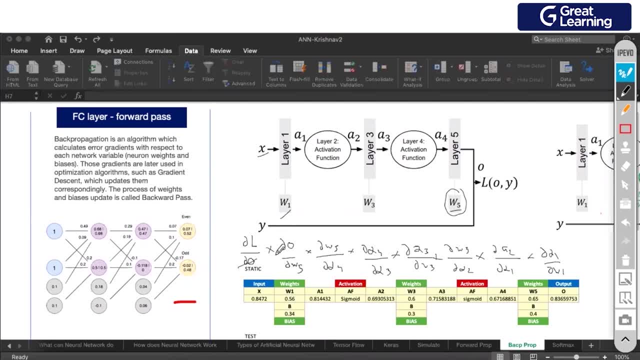 how much you should change this weight. what we should do: cancel this and this. what are we left with? and I say we are left with dou of L divided by dou of w5. agreed, yes, now keep canceling it up. what if I cancel this, this, this and this gone? 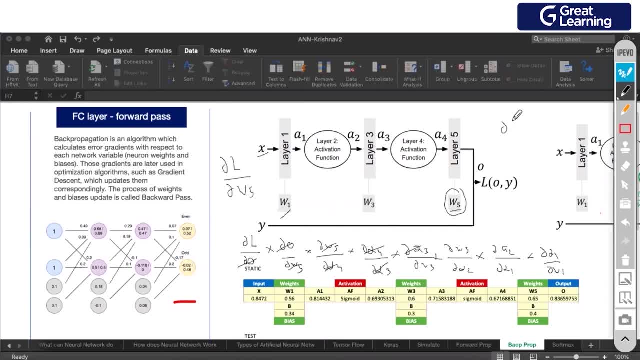 this and this gone now, what are we left with? can I say, dou of L divided by dou of weight number three: yes, yeah, right again. keep changing it down, keep canceling, canceling. what are we left with? dou of L with respect to do of weight number one, simple. so now can I say I have got a method to find out how. 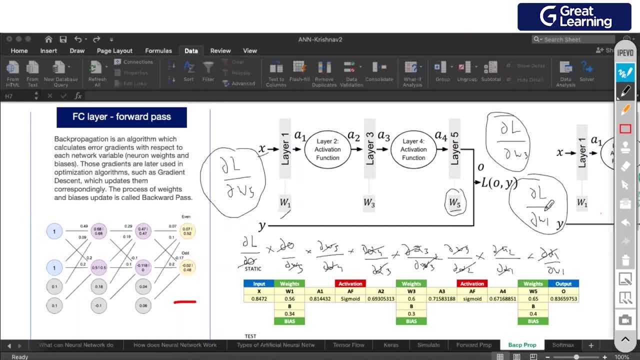 to control my loss with respect to all three of my weights. same way you imagine a larger network where there are so many weights, the same rule happens and the weights are optimized in the backdrop position. all right, simple now. so now we are changing the layer. one weight you can fix whatever you want. so 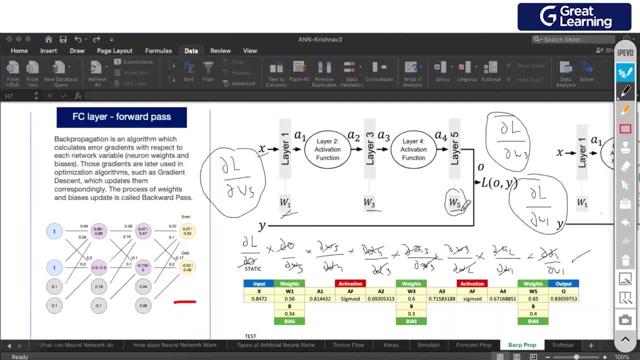 if you say you want to change all of your weights, you can change all of them. if you say I want to freeze this weight and change these two, you can do that as per the chain rule formula, right, okay? well, you're understanding the first week. you can assume that, yes, all of the weights are getting changed in one first back propagation. and 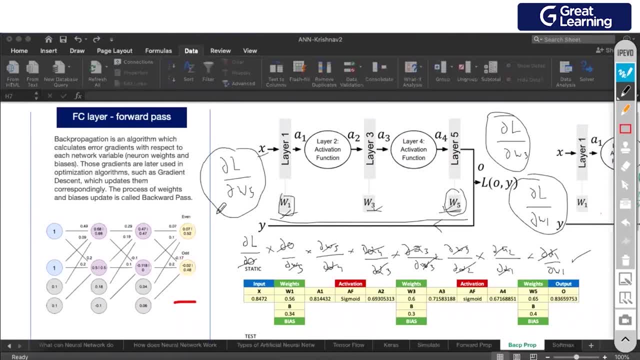 time? Yes, Krishna, is this automatic calculation or do we have to specify in the algorithm automatic, automatic, automatic? in Python we have something called optimizers. they take care of one line, will take care of complete optimization, the way we did it in the solver in Excel, same way we have it in Python. 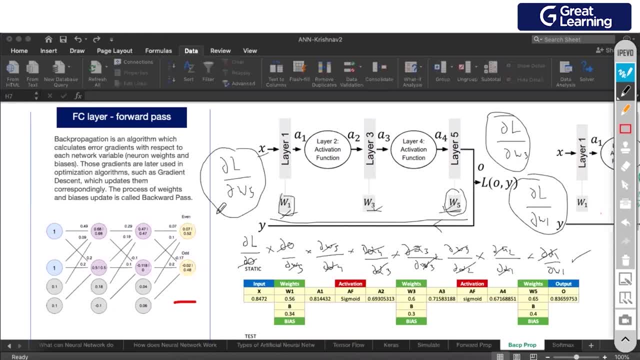 Okay, cool, yeah, one line, that's it, Okay, Right, okay, so today i will show you a neural network which can be designed in three lines. that's it, a very simple neural network classifier. very simple, you don't need to go very complex models, you can even do it a very three to four line up. that's it over. okay, now any issues with back prop? 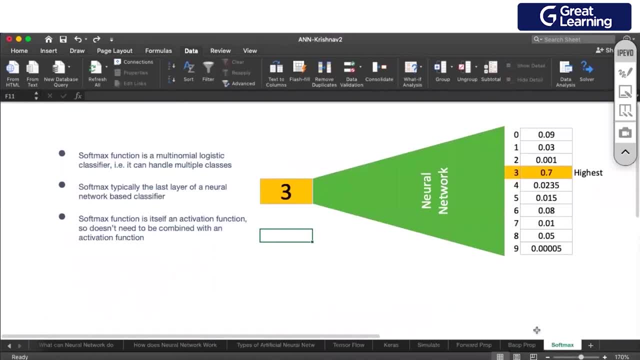 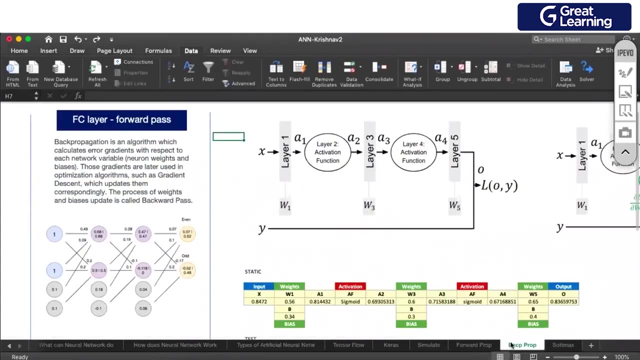 good, all right. so last one, just from my side. i know we have done this soft max function. can somebody tell me what was soft max again? but one more thing is all the calculations, everything you need to uh, practice or what happens in the python, python, python. you don't have to do anything. so 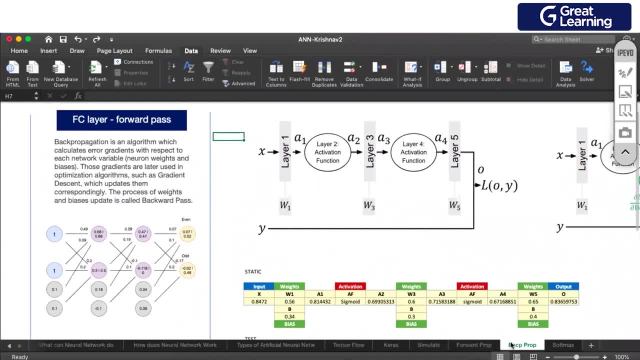 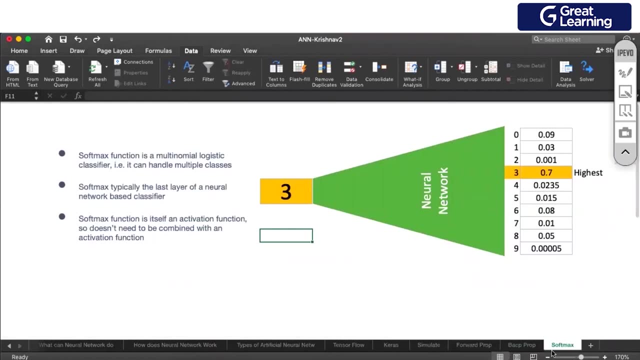 whatever, uh, maths i showed you know it is for your understanding. okay, in python, within no seconds you will be able to train your network, right, okay, final one. no more theory, now we'll go to practice. uh, what is soft max? do people remember what was soft max? 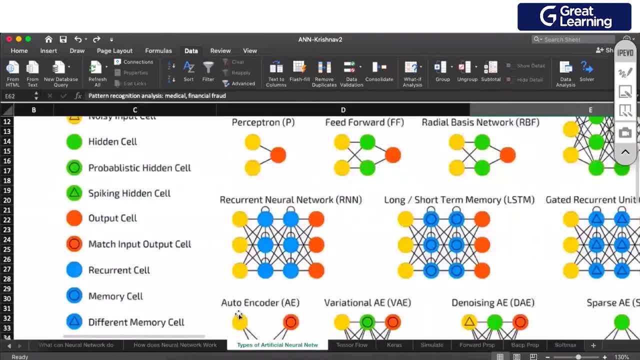 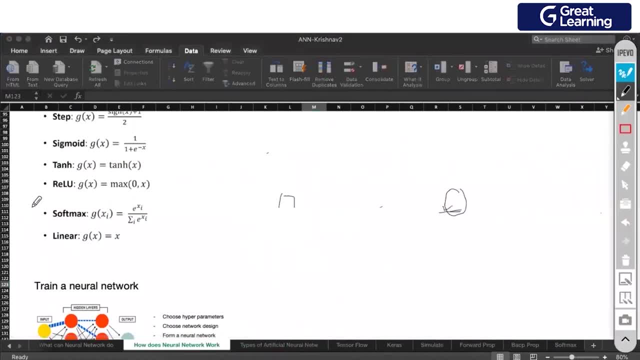 okay, soft max is an activation function. please remember, don't forget this here. soft max is an activation function to be used only when you have an output which is a classifier. if you have an output which is a regressor, you can use any of these. okay, all right, and you don't. 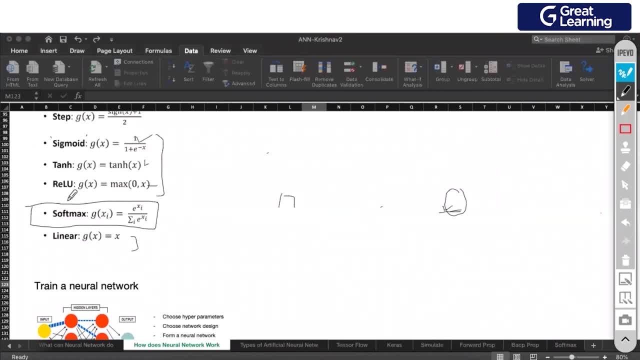 even have to worry about the formulas. you just have to remember the name. that's it. one name in python is enough to do all of your calculations good. so now can i say at least 30, 40 percent. you guys are clear on what is neural network. 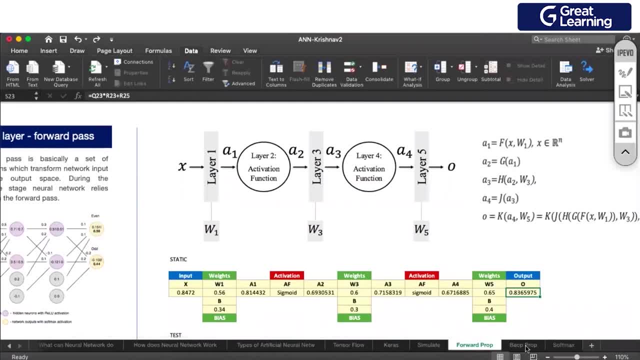 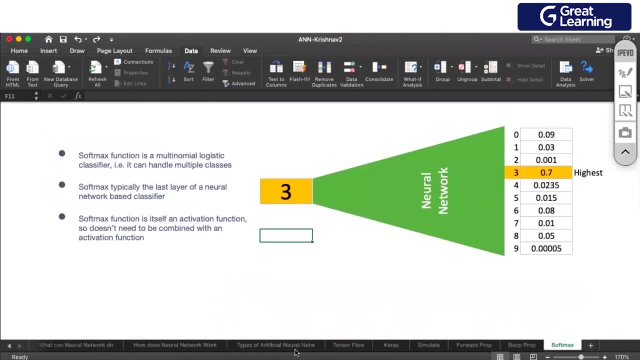 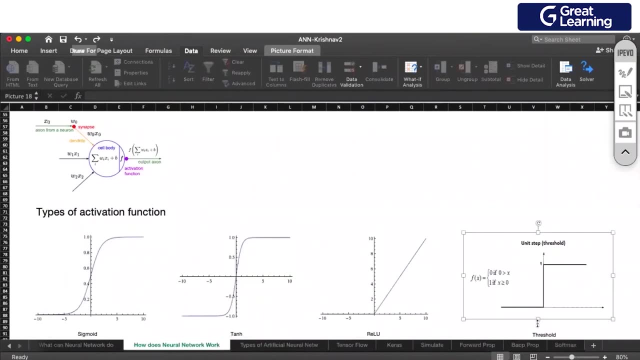 like soft max is mainly used for multiple categories. right for a single, for a single classifier. can we use sigmoid? will that be fine? yes, yes, you can do it for a single classifier. even you can use uh step function here. okay, zero, yes, yes, zero or one, okay, zero or one. that's it. even you don't want to use the classifier, no. 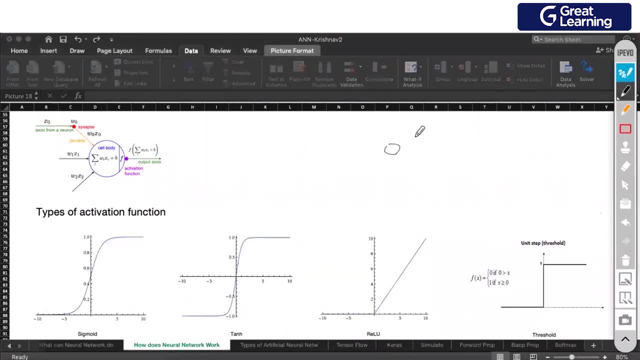 problem. we'll build a filter of our own, so we'll take the output and we'll say, if it is this answer, is this or it answers this anything but yes, you are perfectly right. for two classifications, where you have two classifiers, you can use any of these, not at all. question, one question, if, if from the 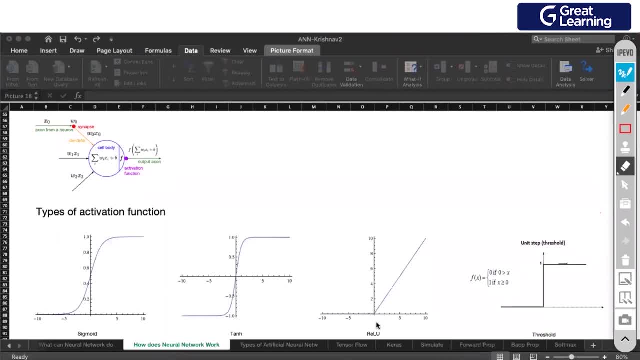 the video classes that the professor has shown us. so in that video class he told me that he told us that the reason why we have used don't use the step function and instead use a sigmoid or 10x, because there is the step function has a constant value, so we would not be able to calculate the 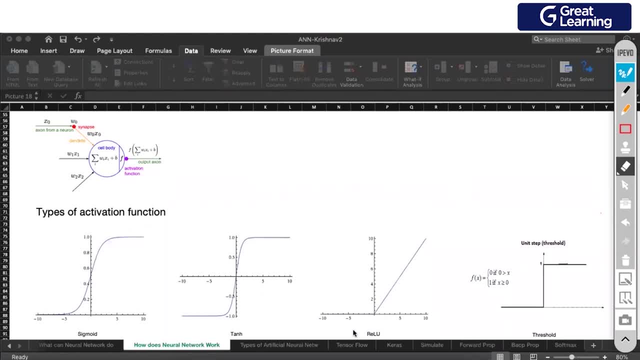 slope and hence the gradient descent would not work. the step function. my question is: why do are we using relu, and it has become more popular because half of the relu is also a flat. what is that is light and will not be able to calculate the gradient descent of that. no see, if you look at this, relu is continuously increasing for the negative value. 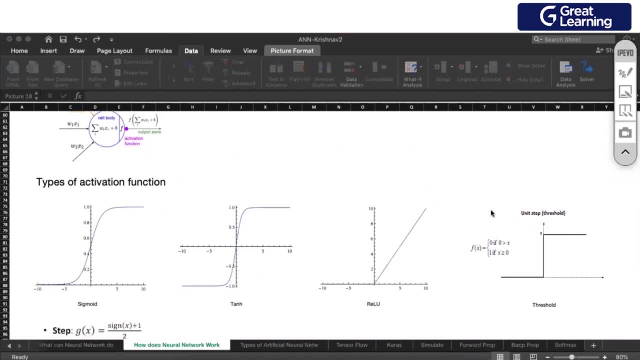 relu is not tracing or relu is not parallel to x-axis. did you see that? yeah, yeah, correct. for the negative value: negative value: it's flat, correct, correct, perfectly right. so if you ask me, yes, yeah. so if you are in the negative value zone, we will not be able to calculate the gradient. 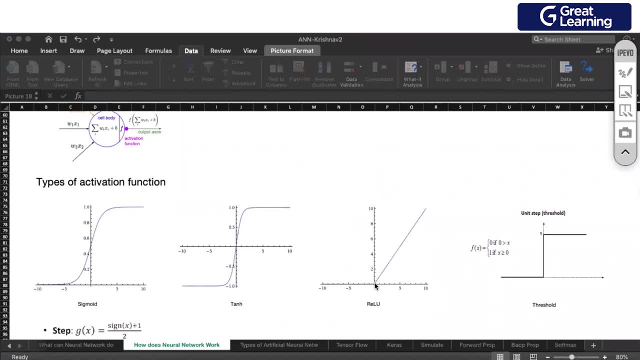 descent, i will not be able to move to the correct position. no, in that case i will say: let me, let me correct your, uh, let me correct your approach here a little bit. please remember: we are talking about a fully connected neural network. so if i go back, do you think this is fully connected? yes, 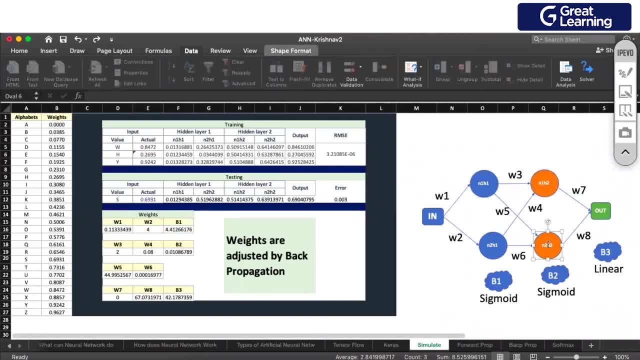 each neuron is it connected to the next layer. so even if one of the one of the function is clipped out, there is another function which will help to pass it through. you getting my point. let us see if this is a negative value. yeah, this is a positive value. and let us say this was relu. in that case, you are. 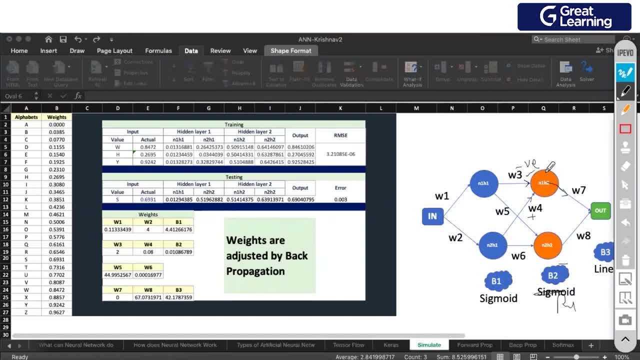 perfectly right. if only negative values going inside, it will be clipped off. but we also, along with that, we are adding one more line which will allow us to go forward. correct, since we have the having two inputs, there are chances that one of them is positive and it will allow. 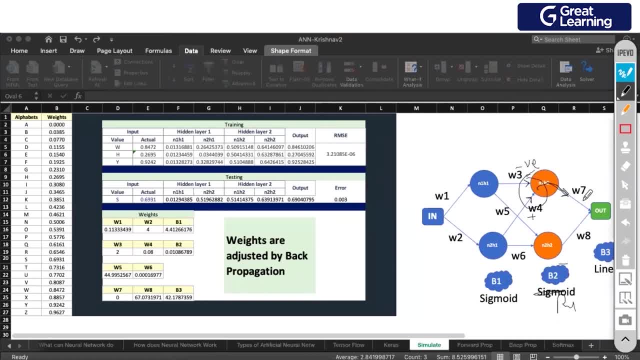 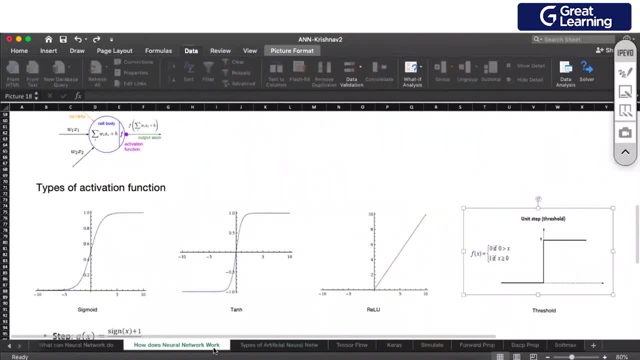 us to go forward. That's it, Yes. Yeah, so the same concept would apply into the step function as well, isn't it So in the step function as well, one value is positive, one value is negative. So even if one value 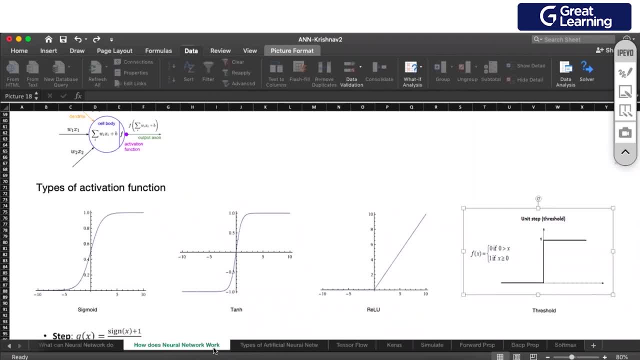 is negative. it would allow us to go through the next alteration. But the way it was taught in the class, it was from the point of view of the gradient descent, so trying to minimize the loss. And in order to minimize the loss, we need to know the slope or the gradient. 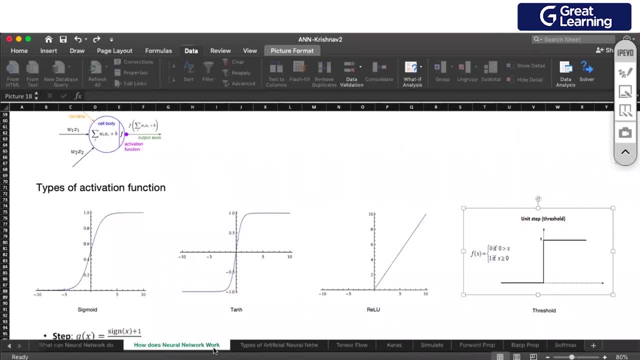 descent of the location where we are in the plane And if that is positive or negative, that would depend on where we need to go In the real function. half of the times we will not be able to calculate where we are in the plane and not be able to calculate gradient descent, and will not be able to solve. 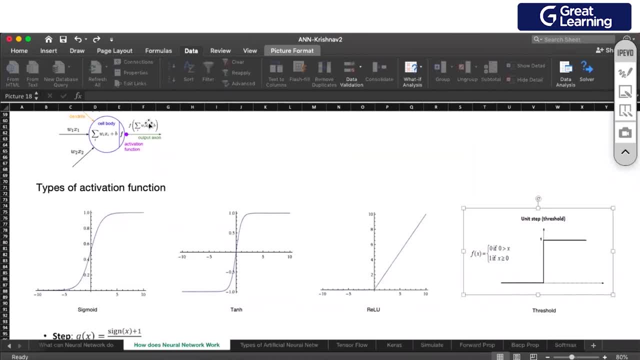 the problem from there Correct Perfectly. So now let me come on to gradient descent. Yeah, Yes, you're perfectly right. I just wanted to say something else in the ReLU that I might be missing. No, you are perfectly right on ReLU and your analog is perfectly right on gradient descent. 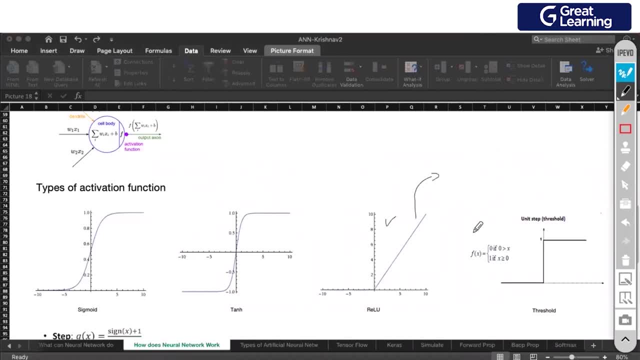 But I will try to reshape your gradient descent understanding And once more, so that you will be able to fit ReLU onto that. Yeah, But you are perfectly right. If, in case, we enter a negative zone, definitely you are not going to get anything out of ReLU. 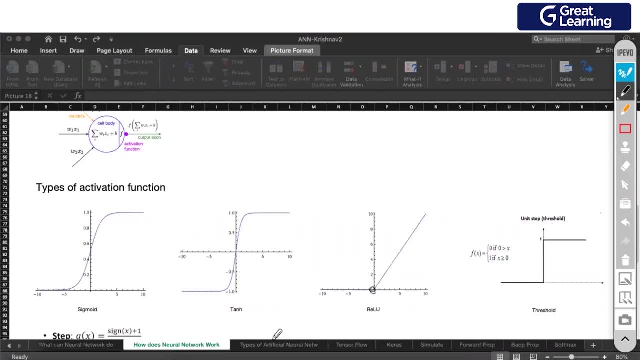 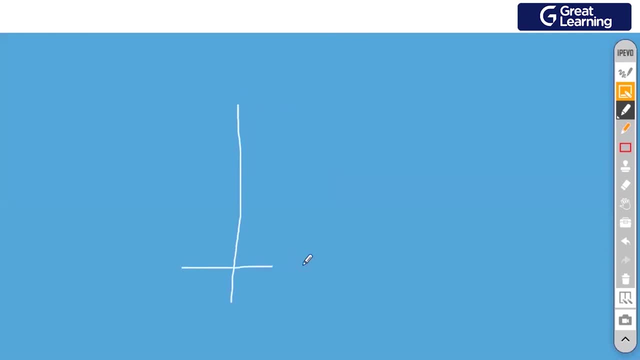 Okay, So let's now try to get a very, very detailed, or I'll say a sneak peek onto gradient descent. So what, as per you guys, is gradient descent? What exactly you mean by that? And somebody quickly let me know. 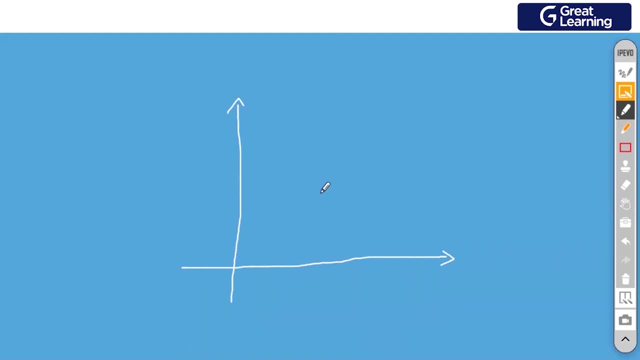 What is your understanding on gradient descent? Basically calculating the slope of where we are in a particular plane and trying to minimize the, trying to move into the right direction, go into negative direction or into the positive direction- in order to minimize the loss or any function that we're trying to achieve. 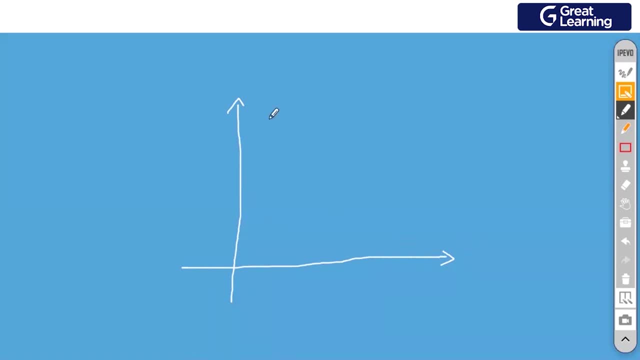 Okay, perfect. Now let me reframe that. Let us say: let's not use technical too much technical term like slopes and all, because when we do that, people get confused. So let us say: these are my weights, all right, and this is my loss function. 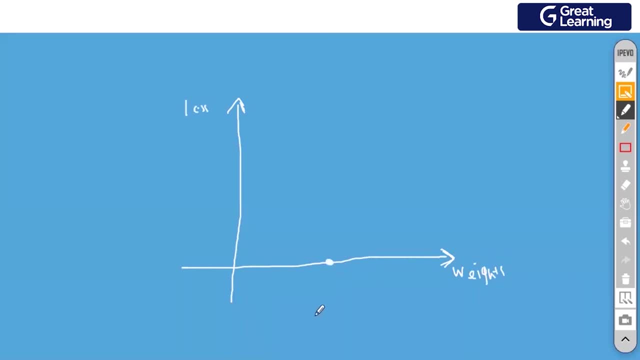 There is one particular place where the loss function for this particular weight will be zero. Agreed, Yeah, Every weight has one point where the loss is zero. at least Let us try to draw a diagram. Let us say we have a gradient descent diagram like this, for example: 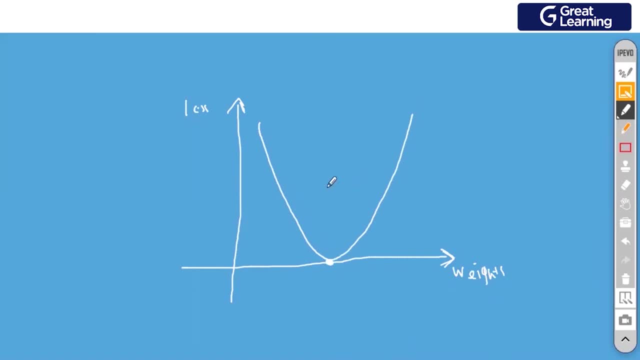 Okay, And also we'll drop a line over there Saying that this is the line of optimal weight. Now there are chances that you might be here. When you chose a random weight, you might be here. So when you are here, your loss is pretty high. 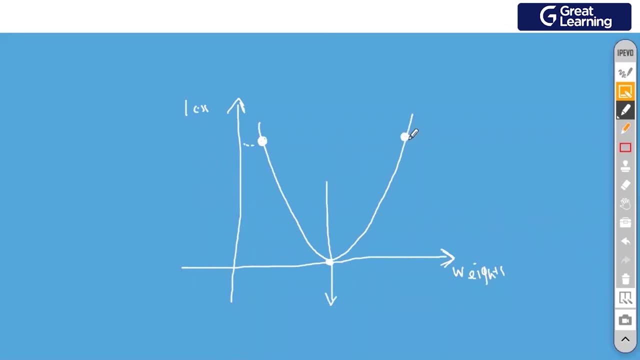 Agreed, Or else there are chances you chose a very high weight. We are not sure about it At that time. also, your loss is pretty high In both the cases. as Raju was saying this, you have to either reduce the weight or increase the weight. 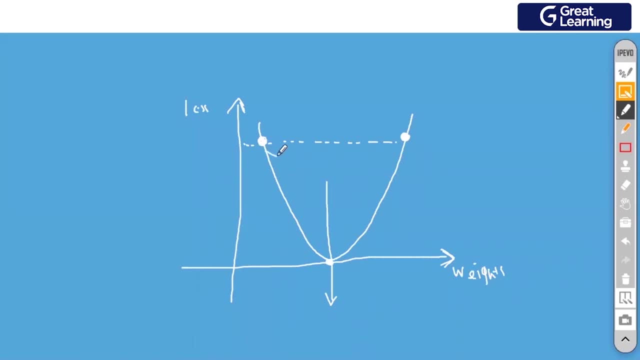 Direction of the weight Gradient descent. In this case, my direction is towards right. In this case, my direction will be towards left. Alright, Depending on the slope and whatever he was saying. Let us say there is one number or there is one factor called learning rate. 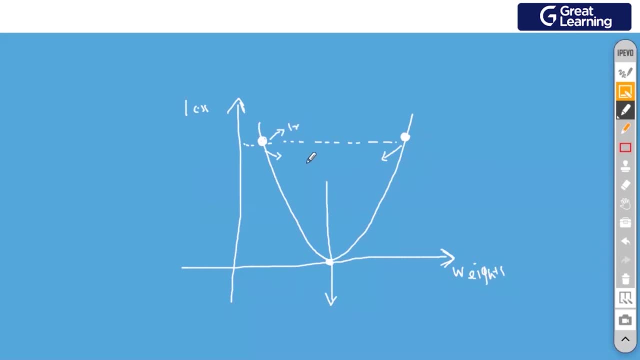 I tell my back propagator: yeah, whatever I am going to use in back propagation, I tell him that every time you make a mistake, every time you get a loss, you reduce or you move by some number x. So every time I have a back propagation my weight value goes by x values down or, in this case, by x values in this side. 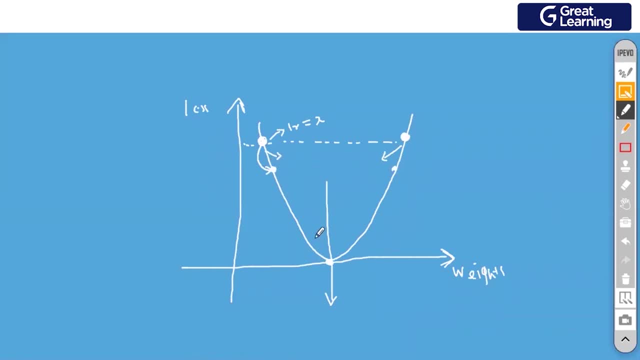 This keeps happening till I reach a spot where the loss is in control or I have reached an actual position of zero loss. So this zone, what I kept- you know the lines that I kept here- these are called sweet zone, Sweet zone. 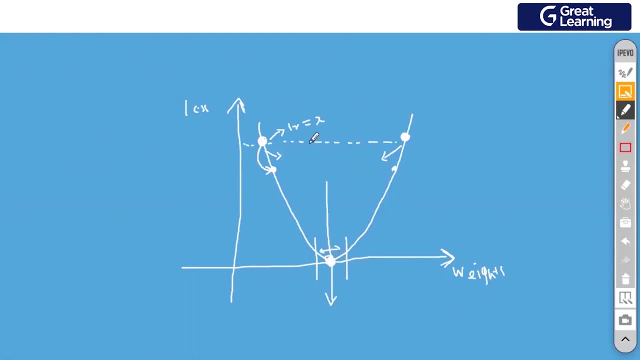 Sweet zone. Sometimes it is not possible to reach here. Now I will tell you why. Let us say you have chosen a value of 0.1. and let us say, when you kept doing back propagation, one time you have reached here. Now, if you add 0.1 to this, you are going to end up here. 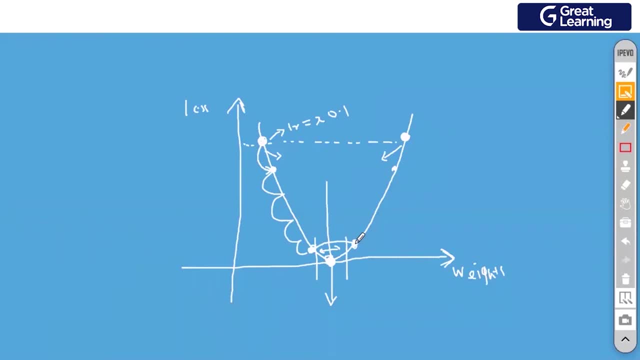 And if you end up here, what happens in next back propagation? you have to subtract. When you again subtract the learning rate, you are going to end up here. So this is what we call the oscillation zone. There are certain times because of learning rate. 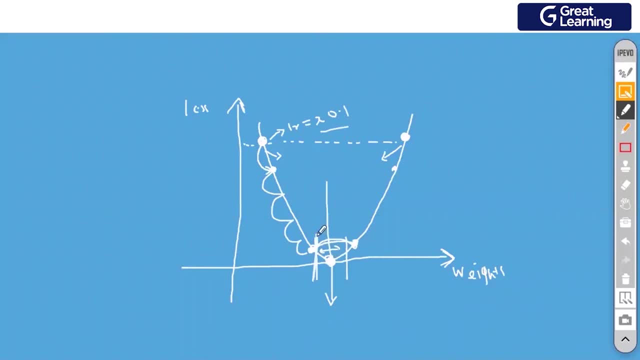 Yeah, You cannot be able to reach here. So in that case we can say that we will put a boundary saying that, yes, we are okay with this kind of weights. This is what is my take on gradient descent. Are we all in sync now? 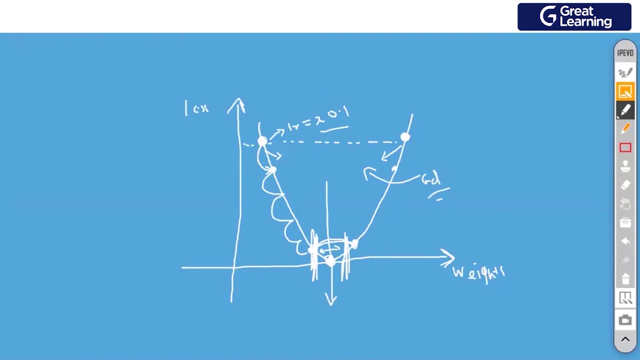 I think you people also have the same idea in your mind, Right? The only challenge here is to understand how to choose this and how many epochs on an average will take me to reach over here. How many back propagations will happen to reach over here? 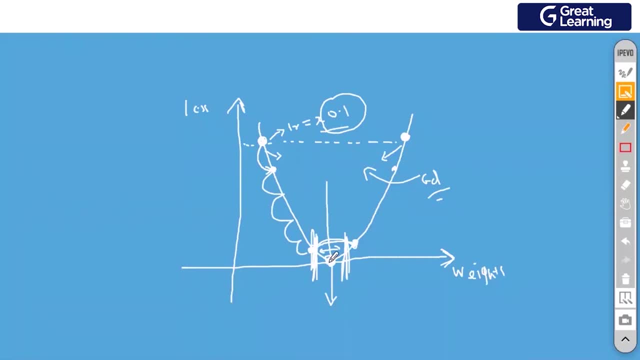 All right. So, Raju, one thing is: you are perfectly right on ReLU, So you are going to clip the negative part of it. But also remember we are not using only ReLU in the network. One layer could be using ReLU. 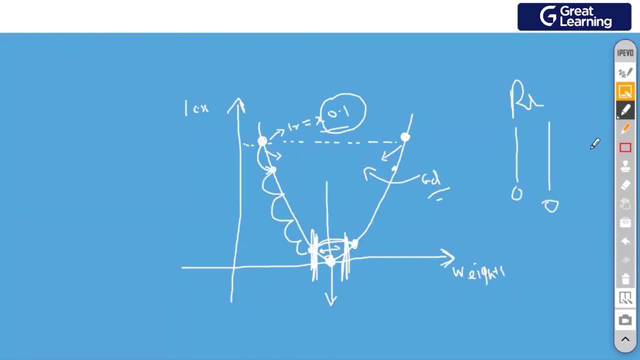 Another layer could be using sigmoid. also. One layer could be using softmax also. Since it is a combination of highly connected layers, it is sometimes okay to ignore certain neurons, even if they are creating a mistake. It is okay, You can ignore them. 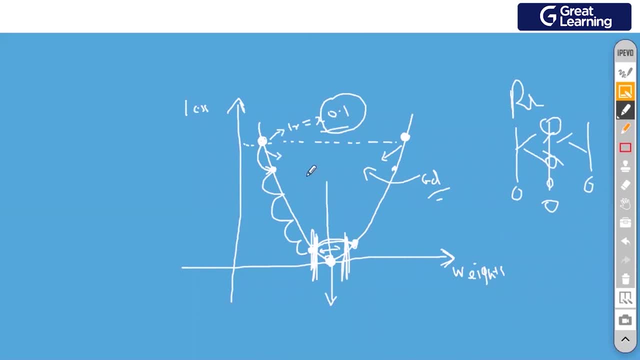 And they will also not create much nuisance in back propagation because of this gradient descent formula. I hope you got my point on ReLU. Yeah, I just wanted to know that there is something else in ReLU. Oh, it was Ashish. 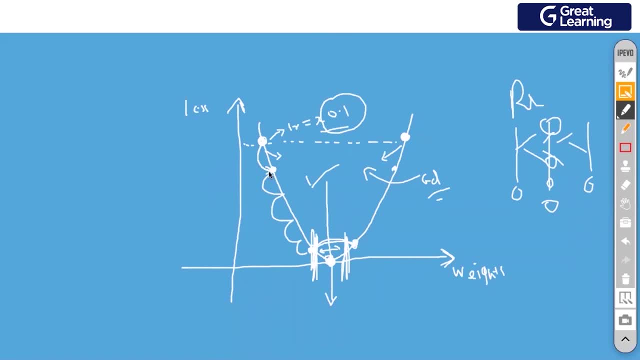 Sorry, Yeah, Ashish. Yeah, I just wanted to clarify that there is nothing else in ReLU that I might have missed, So it is very good. I am very happy it is you guys, Because my other batches were not very focused on activation functions. 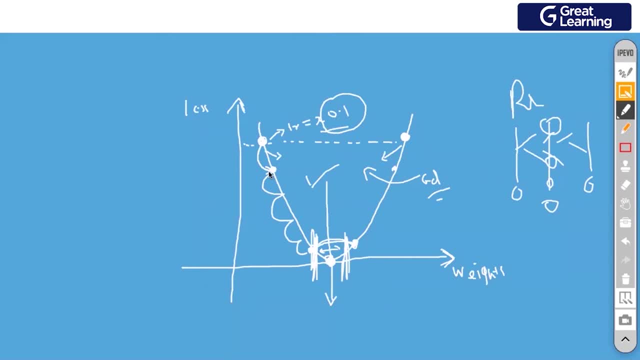 But it is very good to know this, because if you have a good idea of what is activation functions and when you use it, your neural network designing becomes very easy, Because you have to hand make this neural network. Yeah, So you have to choose activation function. 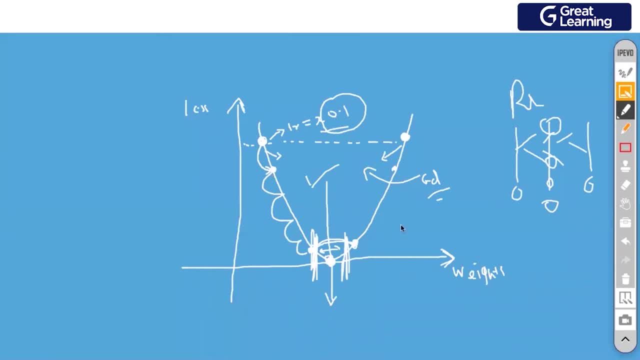 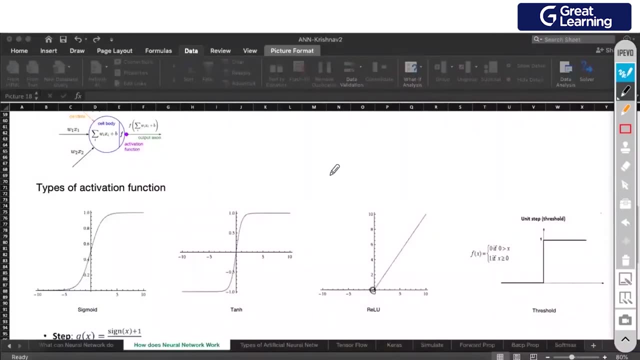 Yep, All right, Perfect, Good. So let's try to design one of them. So we are not done yet. There are some more concepts which I will show you one by one. So I think week two also I have covered almost using this. 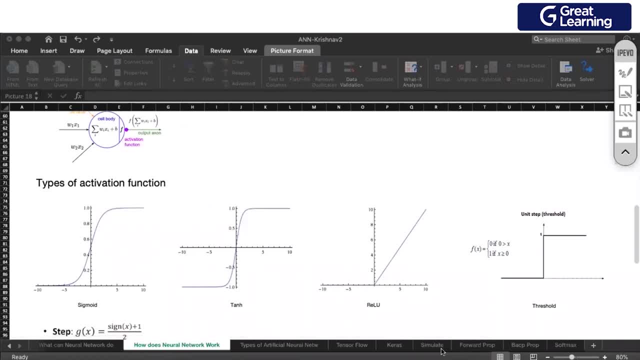 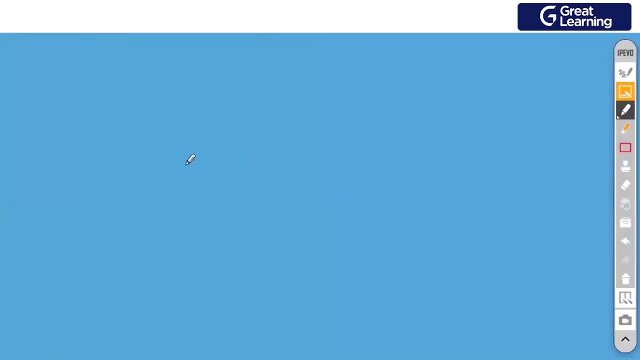 So I think your next week's video, the week two videos, will be very simple for you guys. Now, before moving on, I would like you to introduce to some of the libraries within neural networks. There are many, actually, And now there is a big boom. 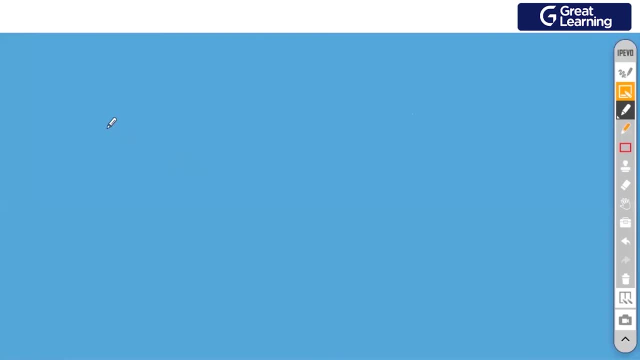 Many companies putting their own library Yeah. So the most important library for learning is TensorFlow. The latest version of TensorFlow- now it is just released- It is 2.0.. I am currently working on 1.0.. I am yet to migrate to 2.0. 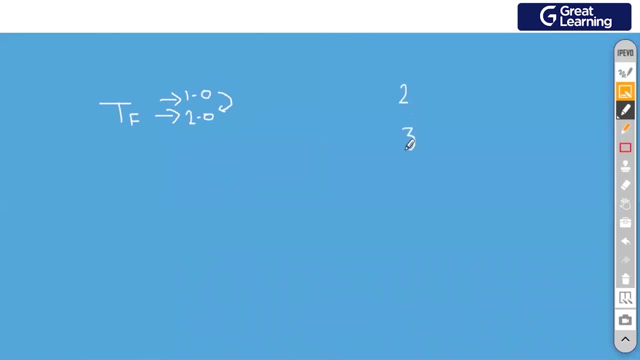 It is like you learned Python 2 and suddenly Python 3 was launched. Okay, So it is very critical for us to transfer this, because some of our codes are very heavy And, since this is new, I am also waiting for it to be stabilized. 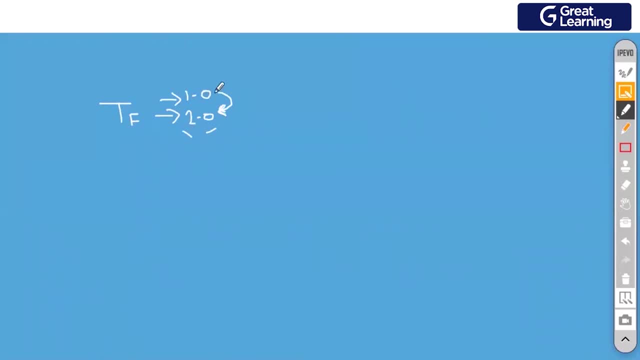 And I am also waiting for all the solutions available online. After that, I will migrate. basically, The codes will change. So this is TensorFlow. What is the use of TensorFlow? TensorFlow is an end-to-end neural net library which is owned by Google. 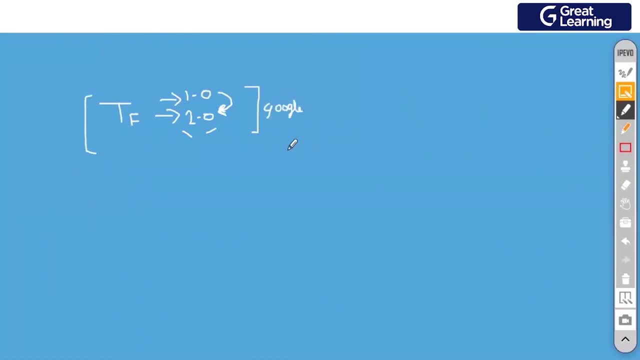 For now it is free, Not sure later, But it is owned by Google And what it does? It gives me the statistical power. So whatever back forward prop, back prop, activation, function, weights, whatever you saw, could be managed by TensorFlow. 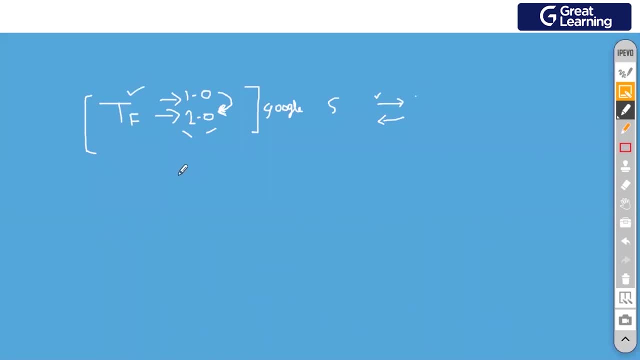 The calculations could be managed by TensorFlow. Good. And also, if you observe, there are certain hardware that we need. We need some virtual neurons who can hold the values, locations Right. Even TensorFlow can do that. We have something called TF Learn which can do that. 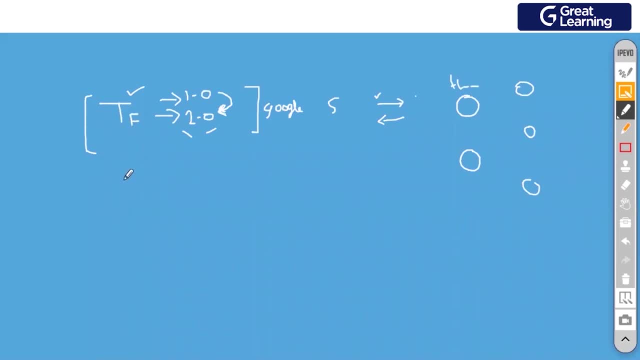 But to avoid it, what do we have? We have a better version. We have got Keras. Keras is a high-level API which sits on the top of TensorFlow and simulates a neural network for us. Good, Are we clear? 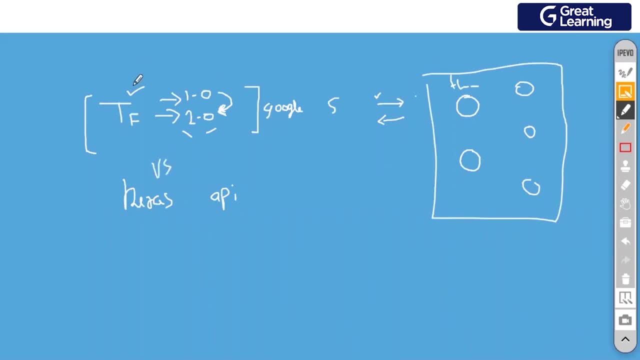 TensorFlow versus Keras. You can build a whole network here, also without Keras. Why do I use Keras? It's easy to define in Python. All right, We have one more called Python, One more called PyTorch. Have you people heard about PyTorch any time? 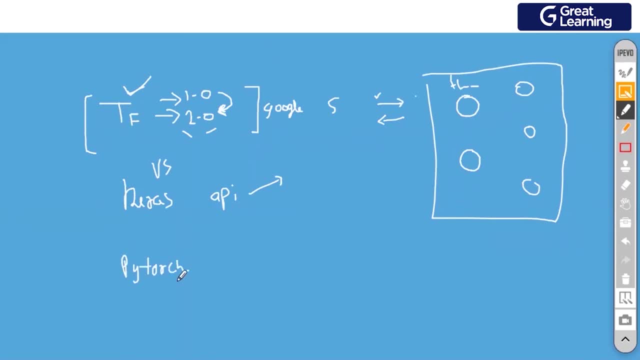 Yes, Yes, Yes. PyTorch is a very powerful library, Very powerful. The only issue with PyTorch is it's a low-level programming language. This is a high-level programming language, Like somebody just asked me that, while doing back propagation, do we need to do this manually? 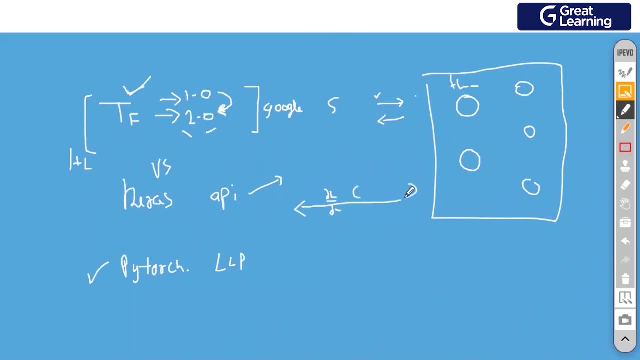 I said no. Why? Because I have a simple command which will help me to do it, Whereas in PyTorch you have to hand-build everything, Not now. Now, PyTorch is evolving, Yeah. So PyTorch is again a very popular library for academicians and researchers. 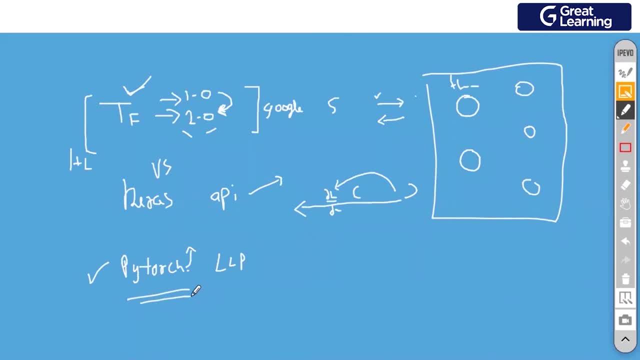 So, maximum majority of the times, when you look at an AI-based paper, especially from a university or a research company, they will be using PyTorch. Why? Because they can hand-make this thing, They don't have to depend on this. 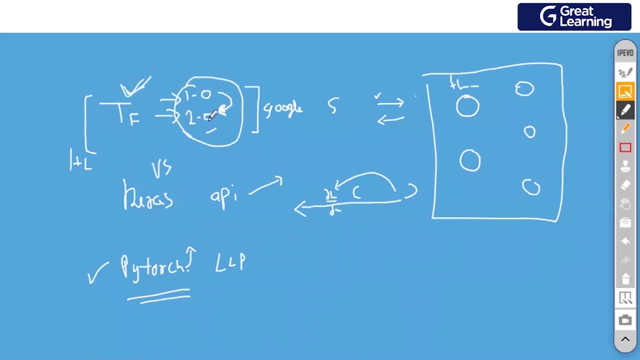 I am a big fan of TensorFlow, So whenever these upgrades happen now, I will be bound by this. I have to upgrade it, Whereas in this you can hand-make this thing, But it's a low-level one. It means you have to build everything from scratch. 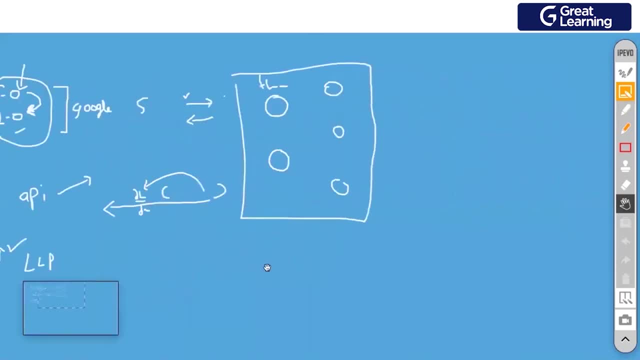 Okay, So this is PyTorch. Apart from PyTorch, there are so many libraries available, Like if I show you guys a library called, say, Swift, for example. So whenever you want to deploy your AI onto iOS or Android, this is one of the most popular libraries. 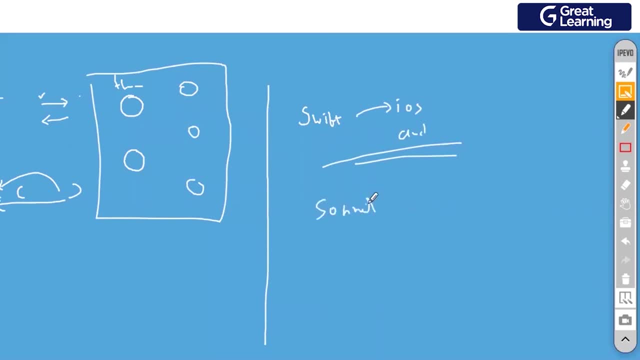 Sonnet. Sonnet belongs to one company called MindLearn, if I'm not wrong, And this company makes or publishes a lot of AI-based papers. You can use their codes to learn. The only issue is they do it using their own library called Sonnet. 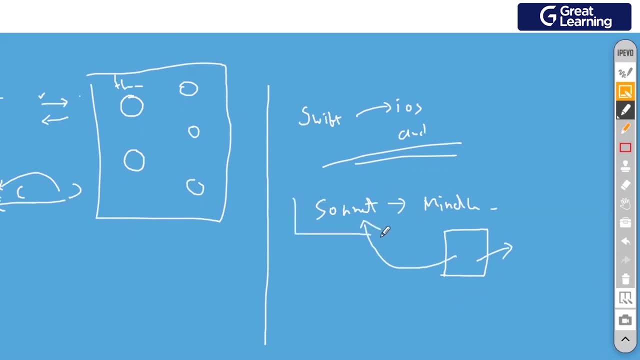 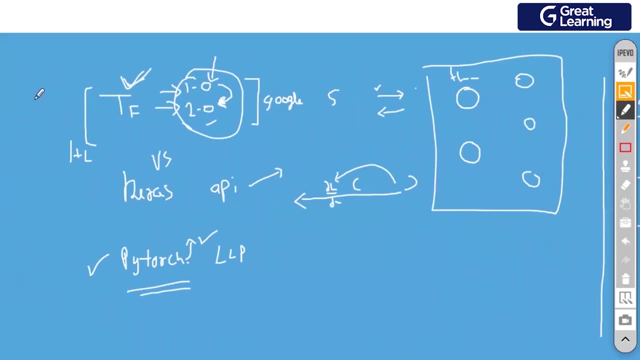 They do not use TensorFlow Keras, So we have to depend on that. Like that, there are so many of them available, All right, So the most popular ones. if you see now is for your starting purpose, These two are very good. 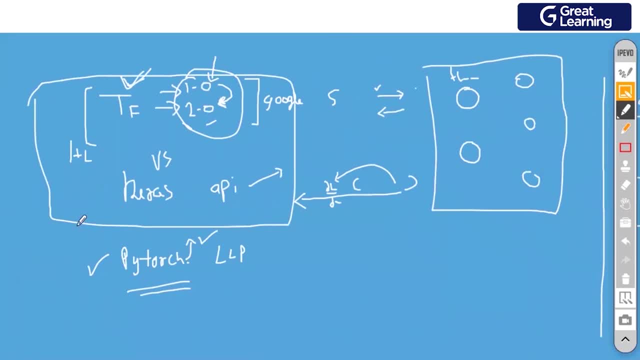 Please learn them thoroughly And after you master that, you can go on to PyTorch, So you have a complete exposure of all the libraries. Good, So these are the libraries. Especially, you should know the difference between those two. So I'll give you one example. 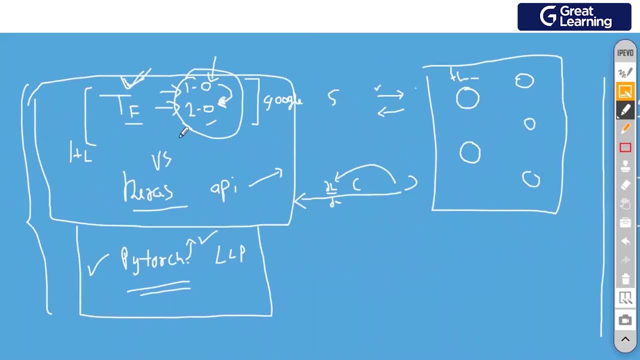 Recently I was taking an interview. I was taking an interview of one of the candidates And I asked him. He said to me I am from AI background And this is the harsh reality of our field. Everybody says, yeah, I know artificial intelligence. 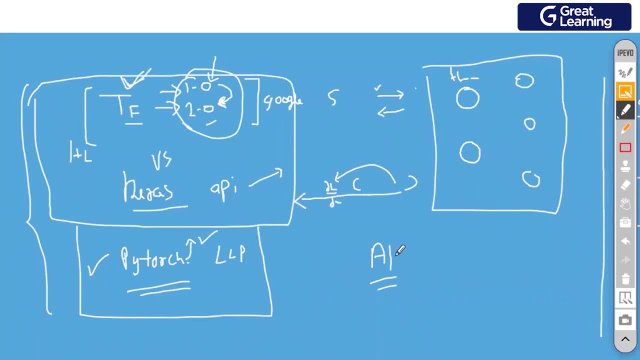 So I very simply asked him: okay, what are libraries you are aware about? So he told me TensorFlow and Keras. So I asked him: can I use TensorFlow independent without using Keras? He said no, This is where people will pick you up. 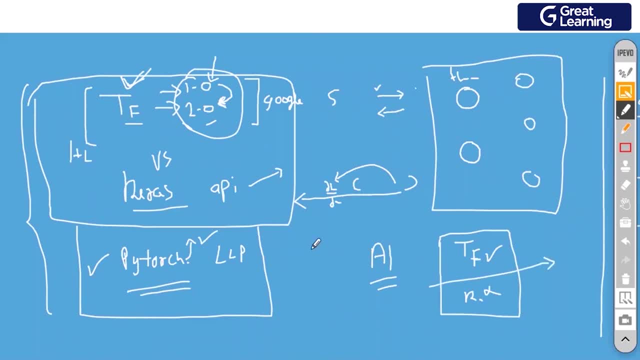 Saying that you have no idea about AI. So out of ten interviews that I take on AI, nine of them I rejected because of these reasons. So people would have seen the codes, They would have done it, But if we don't know the basic difference- where to use what- then it's very difficult to build a network in AI. 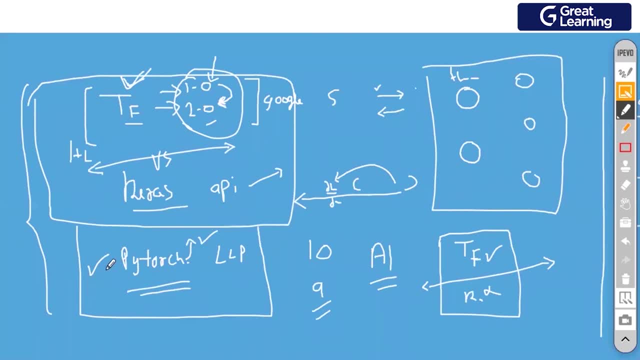 Because it's not a straightforward method, to be very frank. So, guys, please be very careful with these two And try to learn the documentation part of it. So both of them host online some documentation. Please keep it handy And keep in habit of refreshing your knowledge on both of them every three to four months. 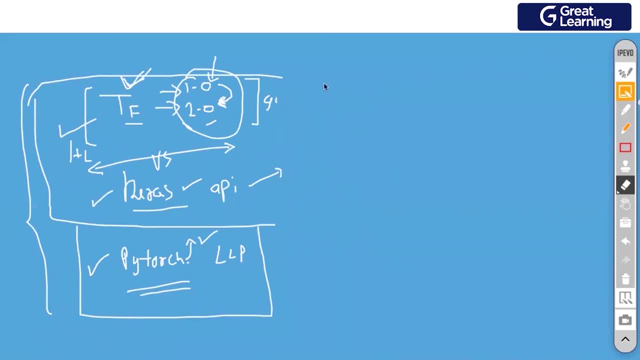 Because they keep updating it. They do a lot of updates. I have one question here. As you said, these libraries keep on updating, So I was working on one library that is compatible with Python 3.5. So I'm able to run the similar code on Google Lab. 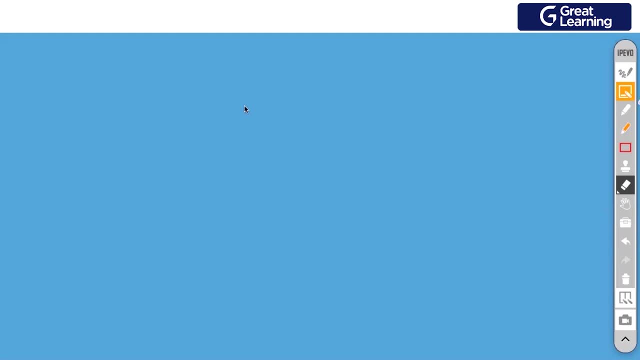 But I'm not able to run on my Python because I'm not able to install the library. So what is the solution out of that? How do we take care of this kind of problem? Yes, So what you can do is let us say: this is the code that you have put in Python 3.5,, for example. 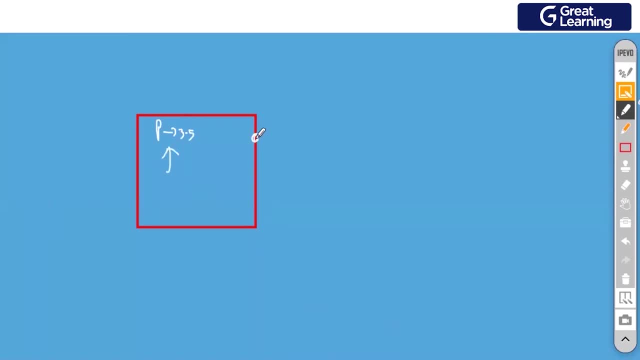 And it has got everything onto that. What we can do is we can pickle this up. We convert this whole thing as a function, if possible, And we will pickle it up. That means we'll store this function And we will use it as a- how do you say- API. 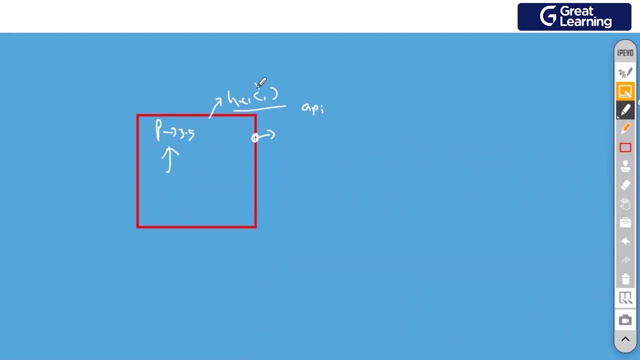 Get my point. So we'll define some inputs and outputs over here to the function. So say you have to give it. how do you say input file as an input? So we have to name the file here And that file has to be worked on. 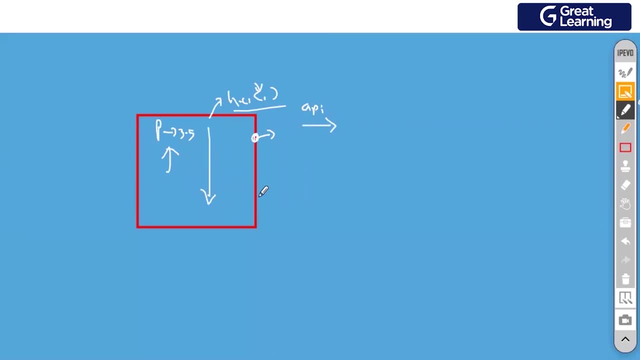 Yeah, I'm going to pick the that I can show you down the line. That is the worst thing you can do, But if you can see, if it is, unless and until it's Python 3.. I don't think so. 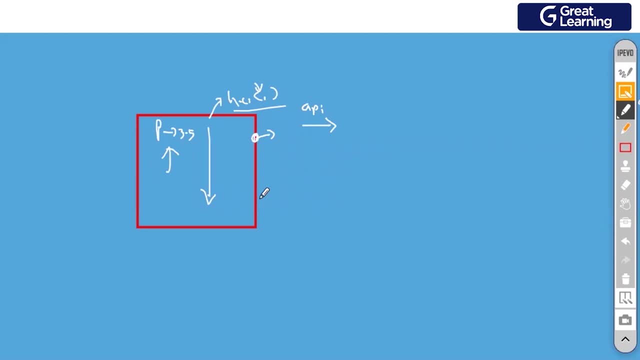 There should be a big problem. Did you check it out? Is it because of Python version or anything else is an issue? Are you sure it's Python 3?? Yeah, So I was watching a few videos on this particular library, So most of those, all those videos were on 3.5 Python. 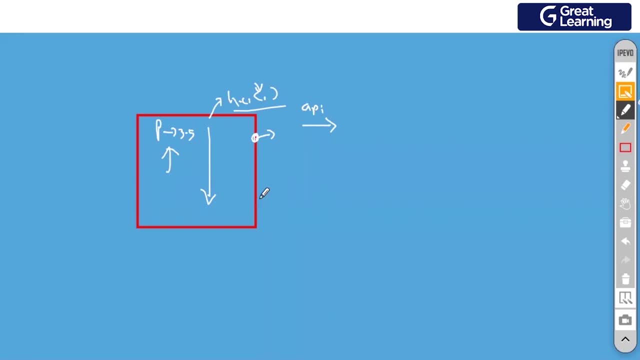 It was very straightforward, And So they were clearly saying that it should be working on Python 3.5 or 3.3, like that, and that's how we are installing it. So I have Python 3.7 when I am trying to installing it. 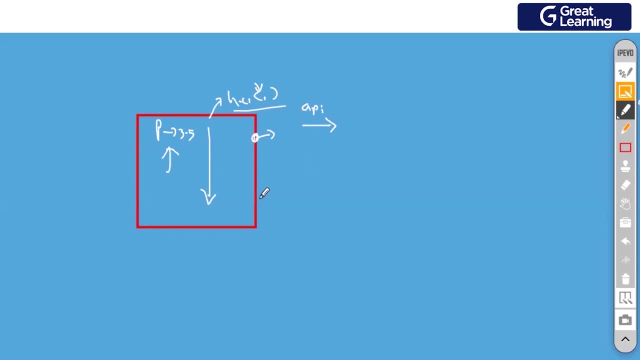 So it is showing that it is not installing. So it is showing a lot of conflicts. What is the name of the library? I forgot the library name. It's related to Qandar. Share the name with me. I have another machine with me which I use it only for R&D. 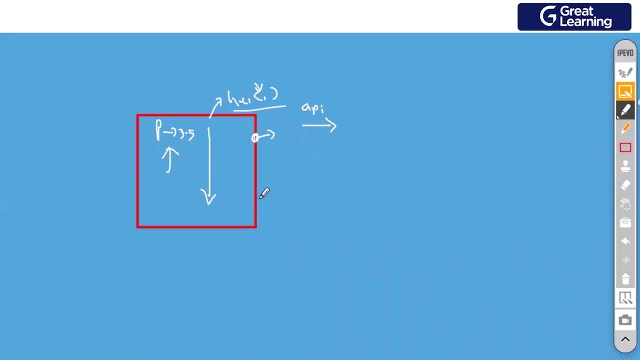 Let me downgrade myself to Python 3.4 and then try not even 3.5, I will go beyond that and let me try loading that. Let's see. Yeah, Okay, I will share the name with you, Okay. 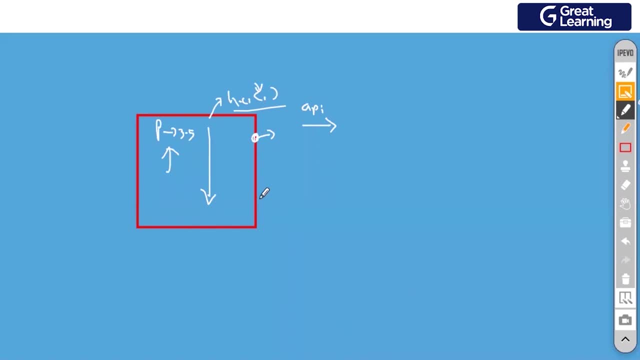 Yeah, Alright, Yes, there are sometimes possibilities like this. I will give you an example: The chatbot that I made. so I got one request from great learning saying that We want to install Python 3.3.. We want to use only TF TensorFlow to build a chatbot. 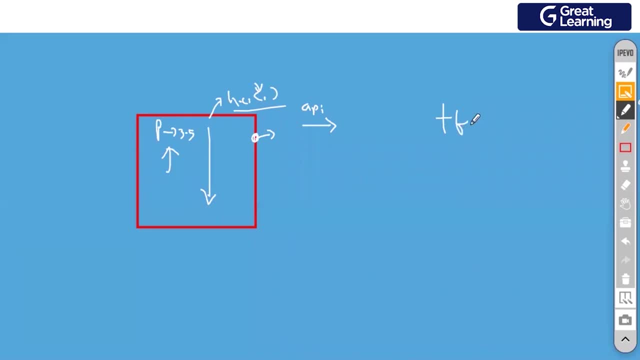 We don't want to use Keras, So what I did is to use TensorFlow end-to-end without Keras. we have to use something called TF-learn. Okay, TF-learn is not compatible with latest version of TensorFlow because they have changed this. 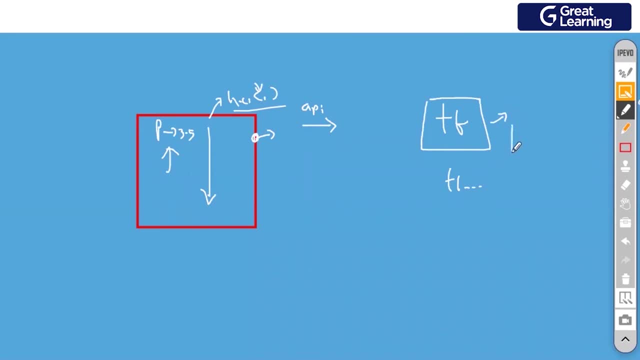 library here, Yeah, So what I had to do is I had to downgrade myself, let us say, from TensorFlow 2 to say TensorFlow 1, point something. And it is exactly like what Ashish said: it is not working below certain levels. 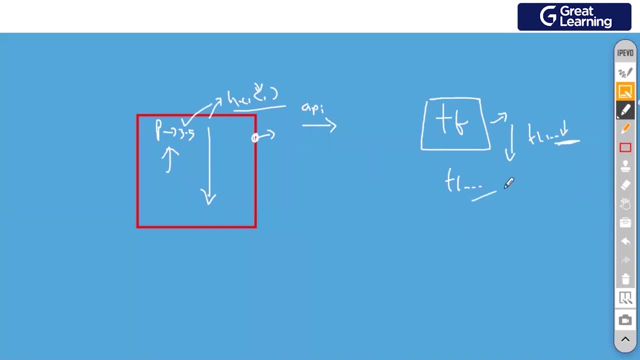 So I had to actually come down to one level below that, And then this thing fired up. So what I did was I pickled it up- Pickled in the sense. I know this is going to be a problem, So I converted this into a runnable function onto any of these OS. 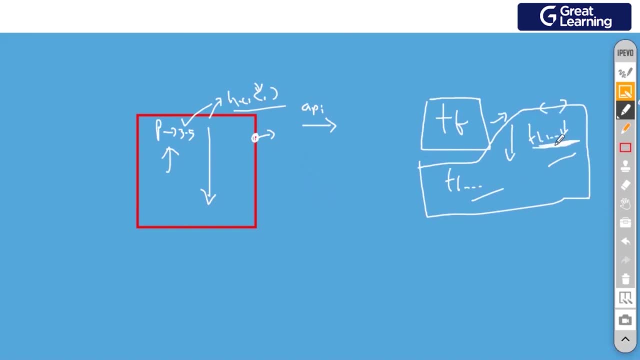 It was not that easy, because the files, the stuff has- what do you say? commands like import TF-learn. But if I'm using the current version of TF in my Python, definitely it's going to give me an error. Even this solution might not work that great. 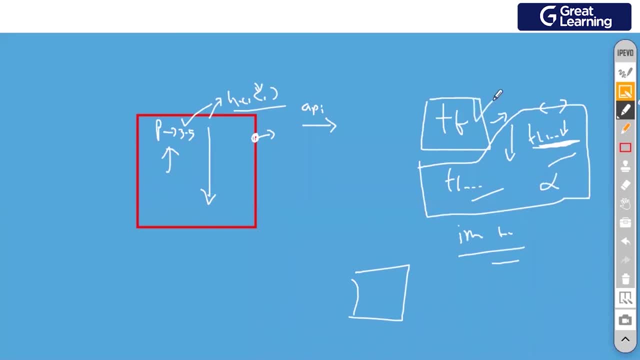 Yeah. So yes, since we are using something free, this will happen- and it has happened many times in my career where this is not working and we have deployed something. So what we have to do is we have to find a fix for that. 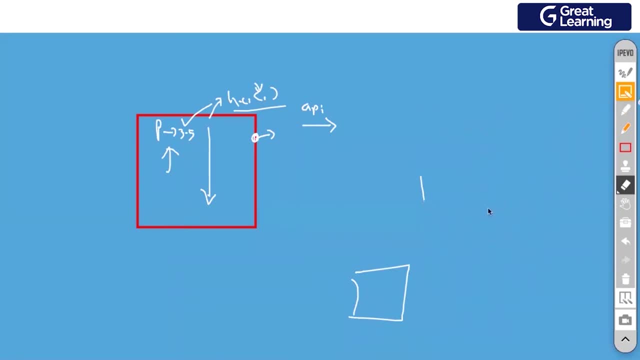 All right, Ashish, there are so many libraries, Yeah, Yeah. One more question related to this. So is it possible to downgrade the Python version or tensor version without losing the previous data that we have worked on? Yeah You, oh, that is a risk. 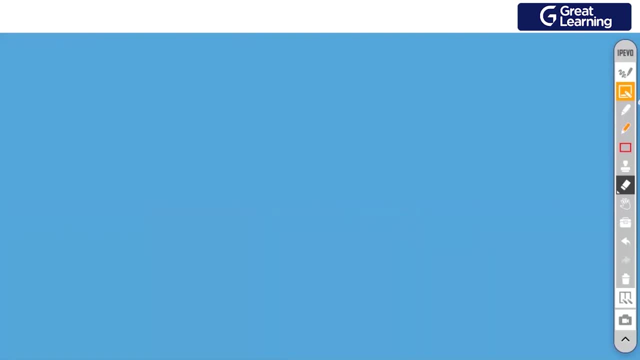 See if I downgrade. I just need to know if I downgrade, is it going to overwrite my, if I have a control of where Python is going and copying the file, if you know what I'm saying. your C drive- It is going to create one folder. 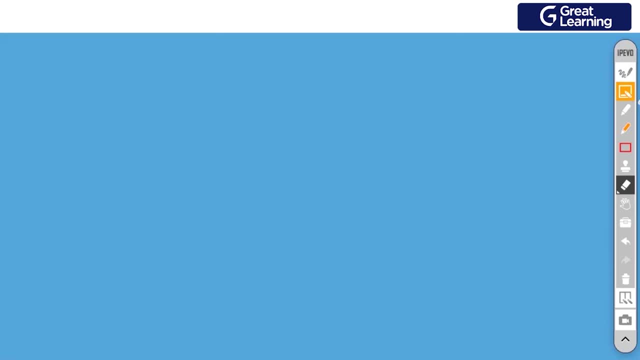 If it is going to overwrite my current folder, then yes, you will lose it. If it is not overwriting, if you have a control over that to create another folder, you don't worry about it. It's going to be as it is. 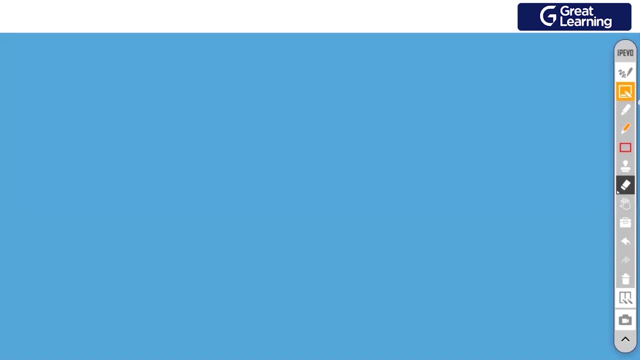 It's all about a folder, That's it. Okay, So if I save my files of the, so if I save my files into another folder and then try to download it, then it would not have any. Yeah, It should not be a problem. 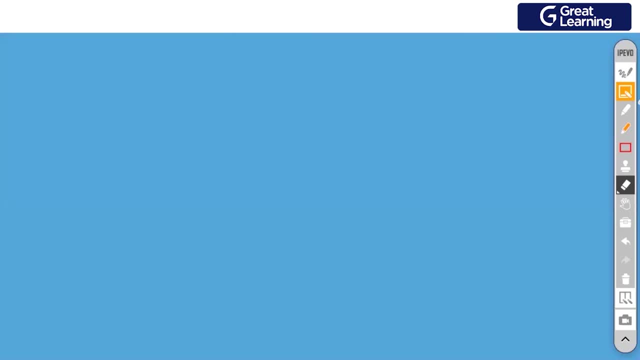 Yes, I mean is it? would I find a simple code using anaconda, or is there? do I have to uninstall Python and then install it again? Um, I think you need to uninstall Python and then you need to install the specific version. 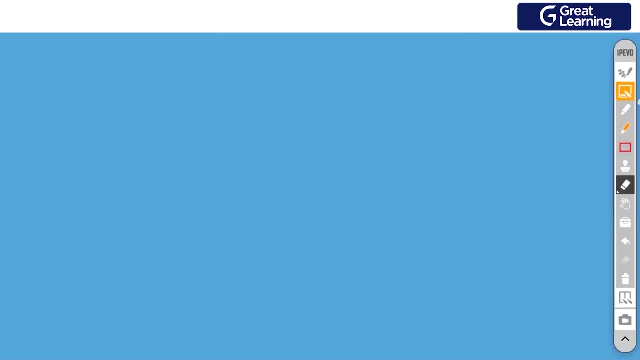 or if just look it out, just check out on stack overflow or geeks for geeks- any of these websites is there. Is there a place to run two of them? because I'm using Mac, right, So in Mac I have an option. 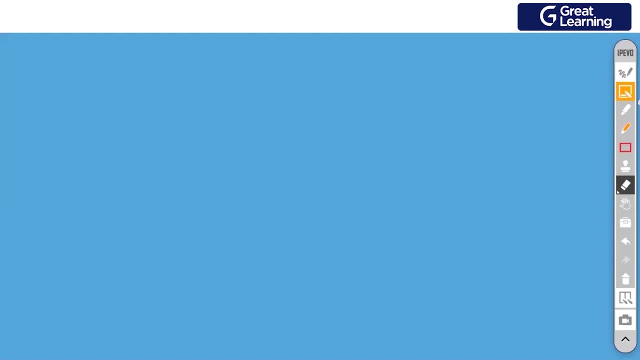 Okay, The original Python that I'm running is two, but I have an option to upgrade it to seven so I can run both of them. Okay, In Mac it is possible. So what you can do is you can have a Linux VM or, if you can have, a virtual machine. I 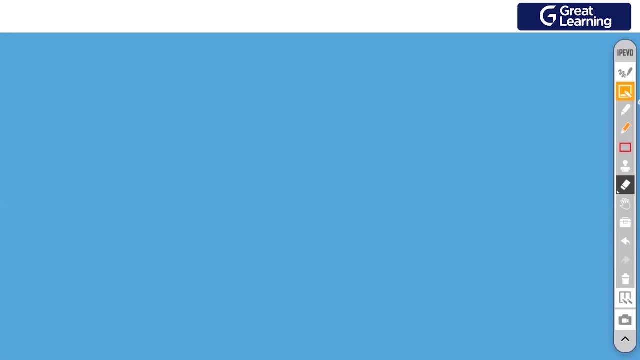 don't know whether you have done it earlier, but if you have a VM you can do it easily. You don't have to worry about any of this. But if you are doing in windows live, I will say: store your Python as you say, and then 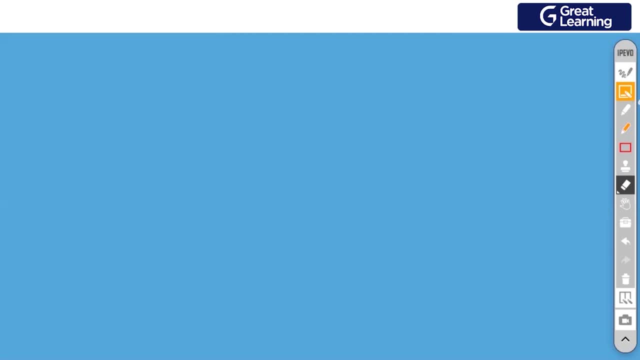 uninstall it and then reinstall the new version. This is what I know. Okay, But try to check on stack overflow If there is a command to have both of these versions and to choose which version to run them in. I'm not sure about it. 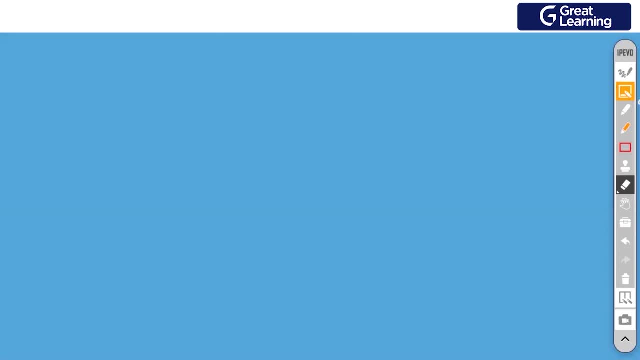 Yeah, How much storage you have in your Mac, Krishna? It's a simple question: One 28.. This is five year old Mac, So it is one 28.. Okay, Even I am having the same thing, So we just thought whether I need to upgrade or not. 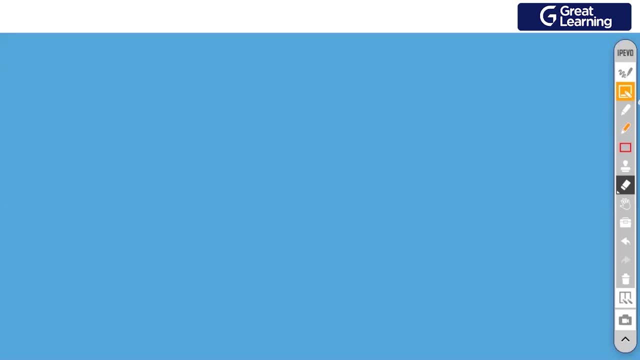 Okay, No, no, it is working Good. It is working Good, No problem at all. Okay, But yes, down the line, if you, if you talk about working on computer vision and all, then either you have to work on collab or you have to get a laptop which has GPU in. 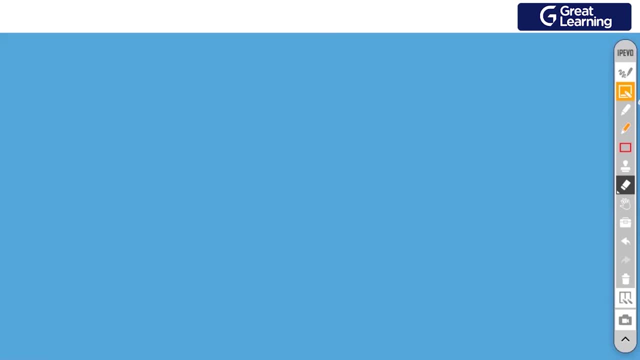 it, Otherwise your Jupiter is going to die in 15 hours to just train your network. Okay, But collab is now because of a lot of people are very happy We don't have to spend money on GPU now, but I don't know. 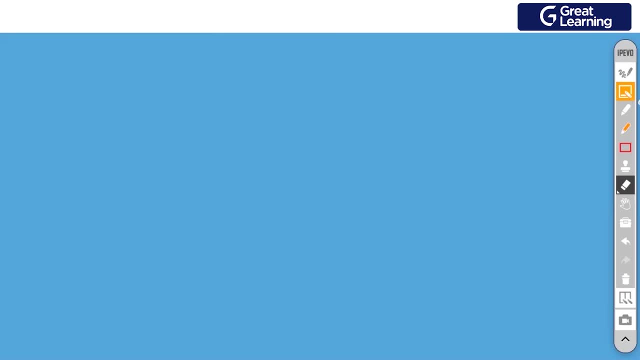 But if we go to AWS, you need to pay high right? If you go to AWS, Yes, Now Amazon, Azure, that is, Microsoft and Google. they are head to head on this. Okay, Everybody wants to conquer this space. Basically, 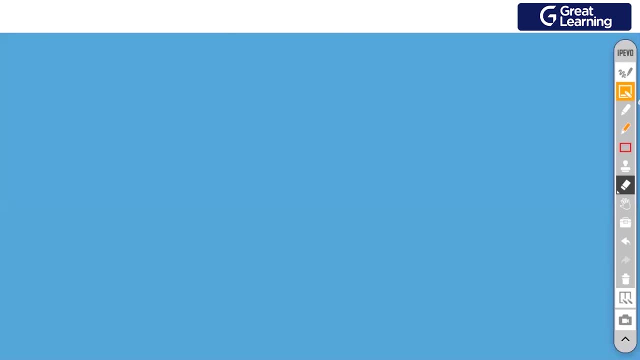 That's the reason Google is giving it for free right now, so that they will get you addicted. First of all, they are giving you, which is 32 GB in Ram- Imagine that- And there is no Python dependency there, So you can go and install any version, anything that you don't have to worry about what you. 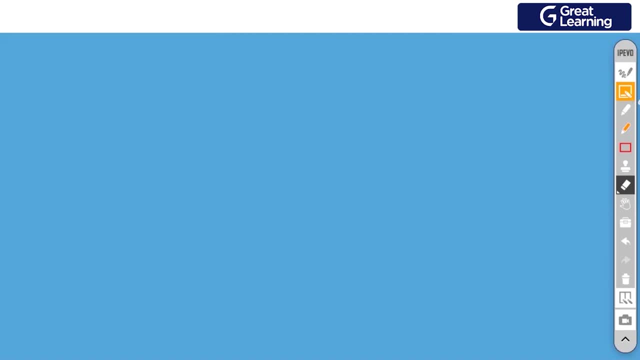 have installed in your machine. There's no sync with it, but the only issue is TensorFlow, And both of them belong to Google, So I'm not sure how long it is going to be free, to be very frank. And now Azure is also picking up. 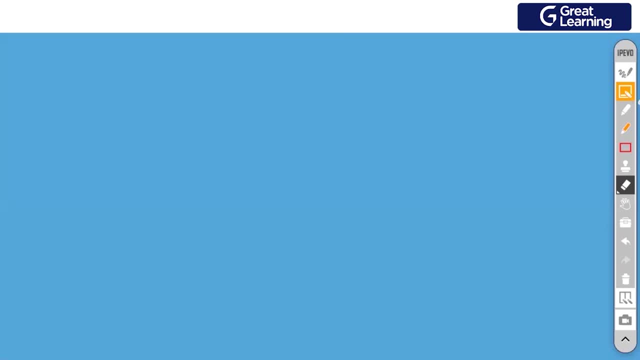 I don't know whether you guys have heard about it. Azure is making an end to end analytics platform within their own cloud, So it's going to it's going to be a big rival for our AWS. Okay, Yep, So if you guys can work. 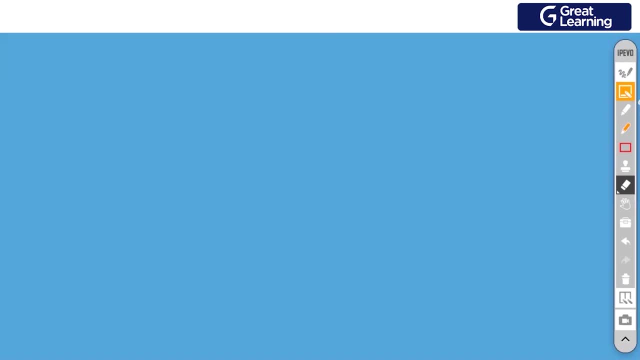 I had a conversation with somebody in the Google, So the idea of Google is similar to Gmail, So they want to be as long as possible. They have a good issue. Good, Good, That's good for us actually. Then you don't have to spend on a GPU machine. 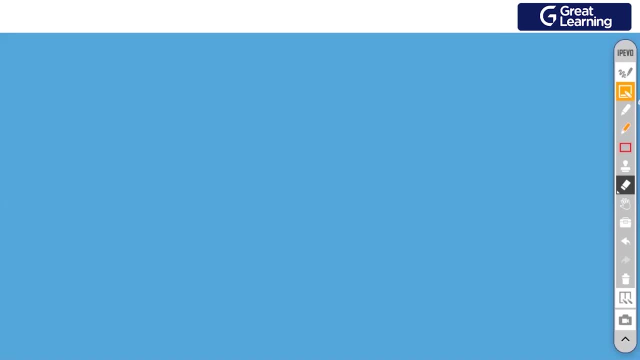 Right? Yes, Because one of my learners from the other batch bought a machine specifically with GPU. It costed him a lot, actually, So, But then this Colab came in, So it worked, But then I feel there are some issues with Colab, also that it's running in middle. 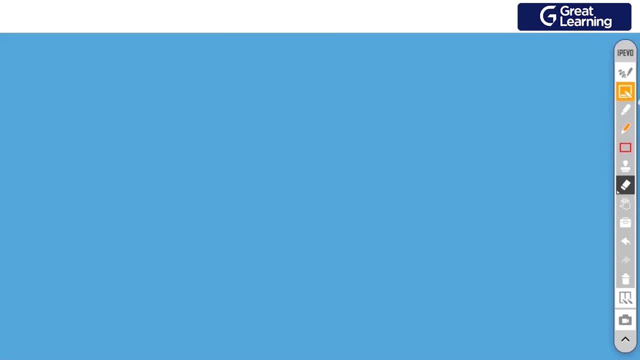 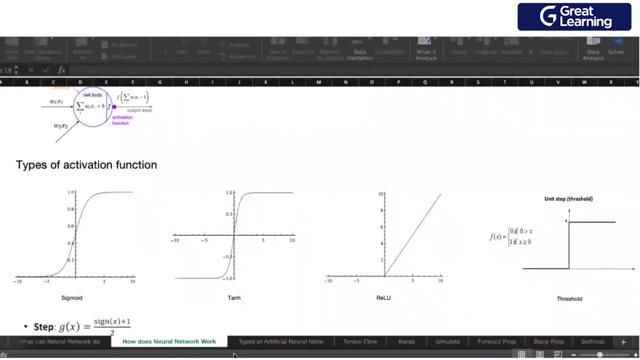 If it stops or your net fluctuates, It restarts, basically, Rather than restarting from where it was stopped. There are some issues, But yeah, there is a beta version, right, So they will upgrade it. Okay, All right, So let's come back here. 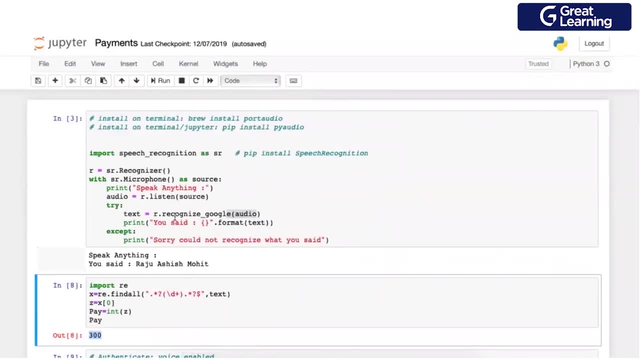 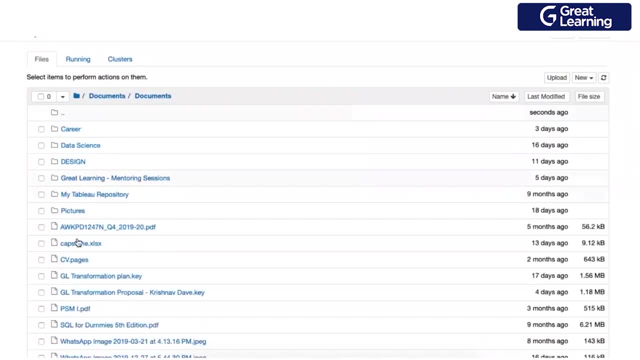 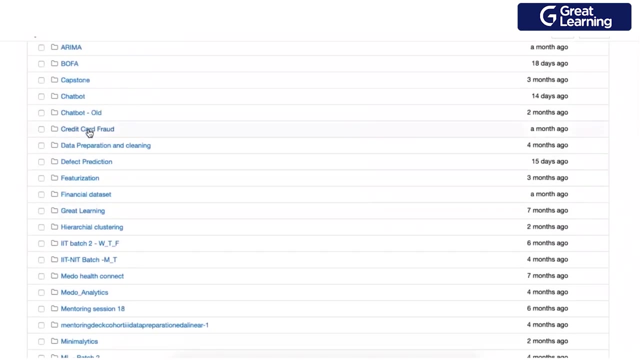 Let me show you one simple example Example of how to build a network, And then we'll close down the neural network part. Where is it Great learning? Where is my defect? prediction, Yeah, Okay, See, I have a very simple problem where I have got two columns. 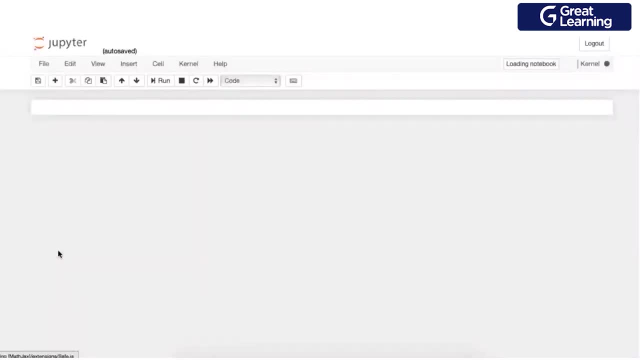 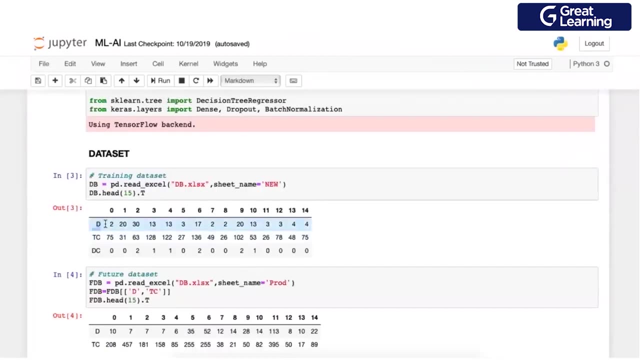 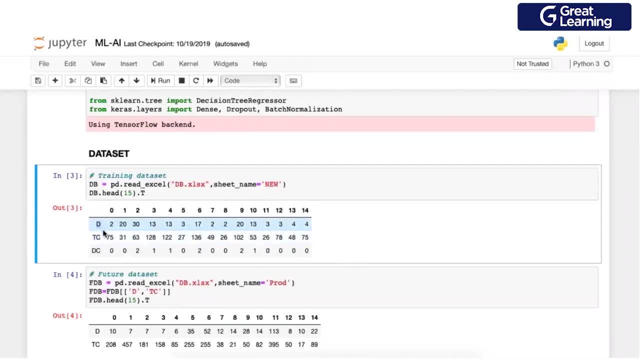 Okay. So I have this: some say number of days a person is working, or a test tester is working, for example, And I have another one where I can say: these many number of test cases the person is testing in this many number of days. 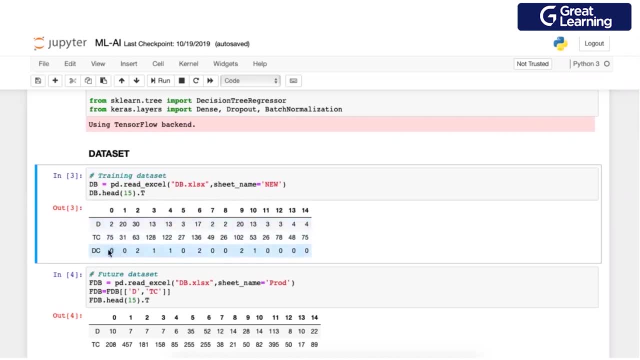 Yeah, And out of that the outcome, the target column is defect prediction. So this many of defects he is getting out of it. Yeah. Now what is my business problem here is what, if I can make a predictor here saying that in future, if I give these two values, 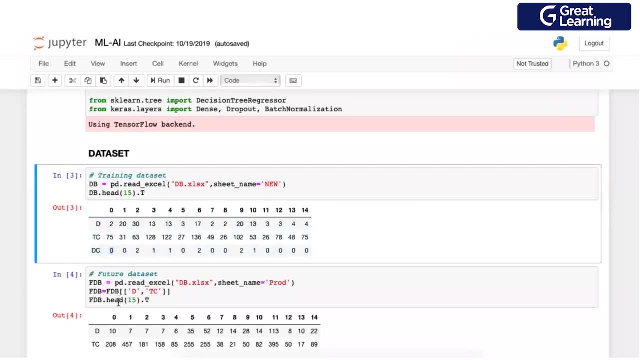 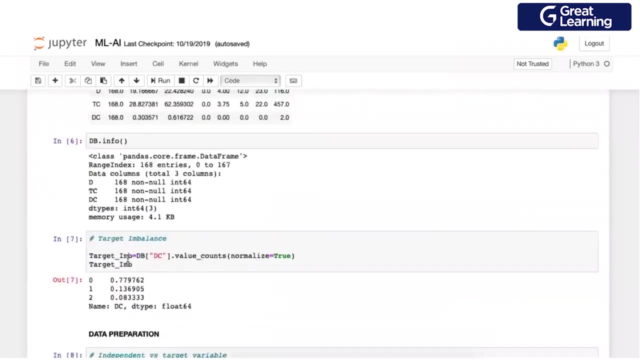 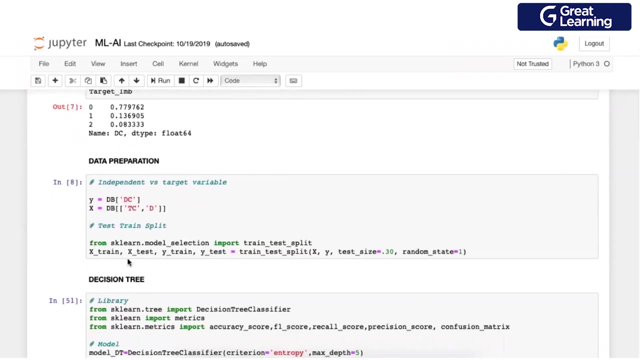 I should get an output like this: Okay, Let's try to build a model on that. So what I've done, first of all, is I have used all of our machine learning techniques, as usual, just to show you, guys, the power of machine learning versus here. 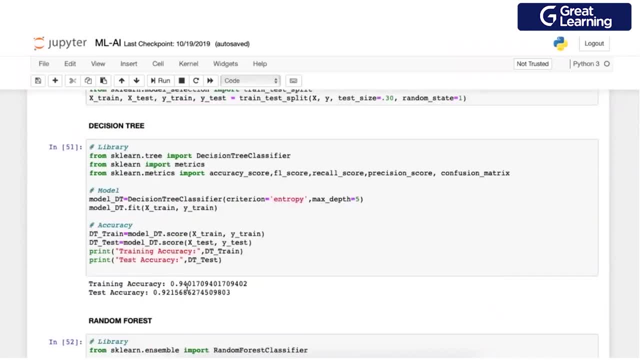 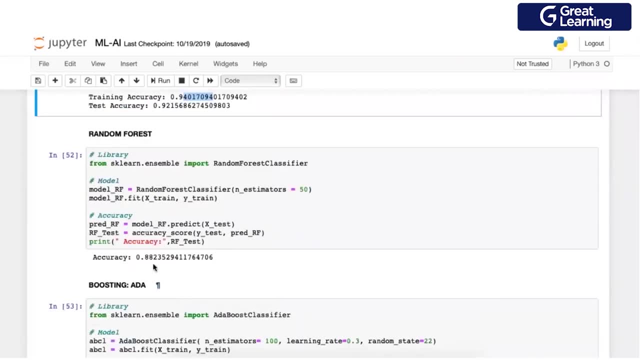 So first we are using decision tree and since I have done pruning already, we're not getting any overfitting issue and everything's good. as of such, Random forest is coming a little late. It's coming a little lower, which is 88.. 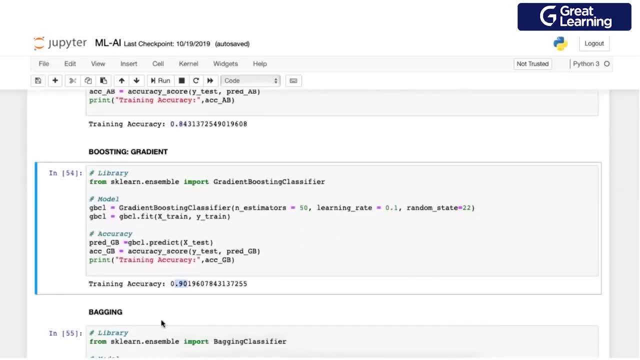 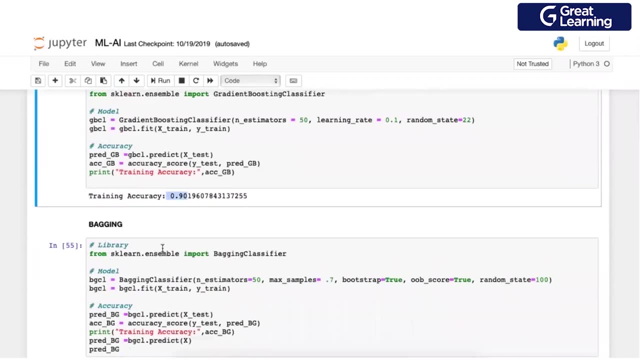 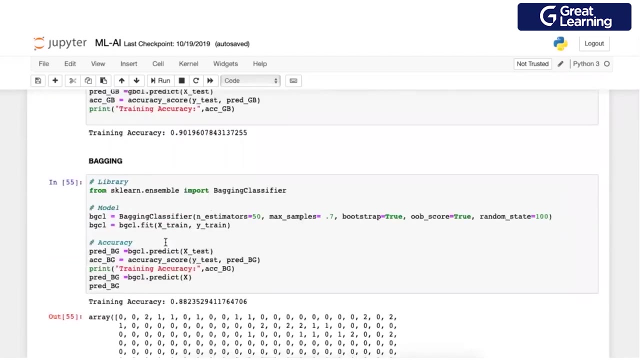 Boosting is 84 and gradient is around 90 and bagging is 88. So if you compare all of this, I feel bagging is sorry. boosting is doing pretty good, So we'll choose one of them. So we have made an ML predictor with accuracy of, say, 90%, for example. 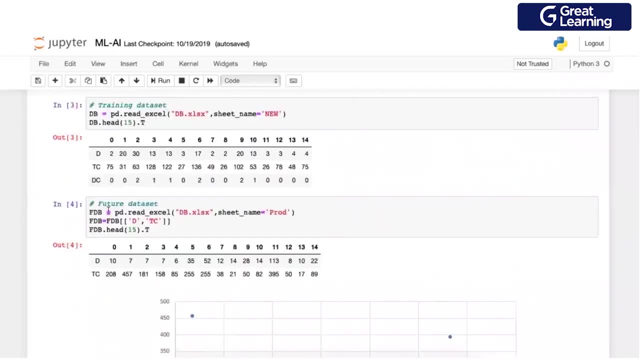 So this is a very simple way of doing an ML. So now somebody asked me: right, This AI, or deep deep learning, is pretty good, Then why are we learning ML? These? these are the things using which, on a very simplistic level, you can implement. 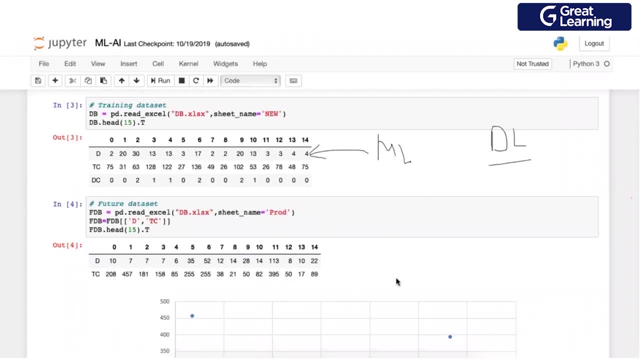 it. You don't have to. you know, go ahead and do back propagation for propagation and all that part, Some of the applications. or I will say right now, at least for next three years. that is what is my prediction, If you guys get on a real time data science project also in your company. the first: two to three years. you will be deploying only three years, Deploying only these kinds of things, to be very frank, because if the company is new, if the product is new and if the space is new, the company does not take a big risk. 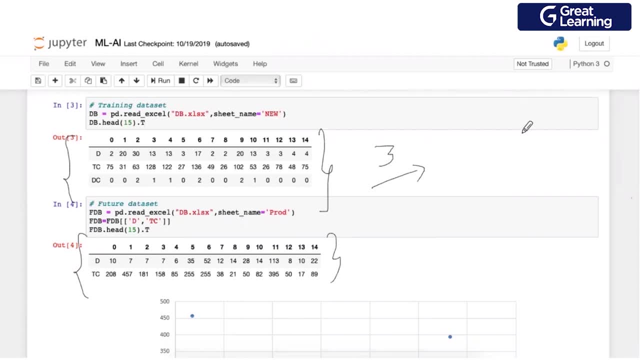 of implementing a high cost products. When I say high cost, it includes GPU, It includes deep learning, It includes training time. A lot of things are there which we have a we call it as KPIs for high risk products. 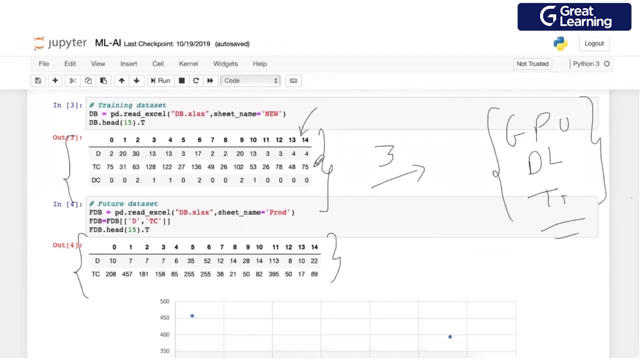 So what we do? first we penetrate into clients, trust Trust by using these kinds of simple microservices, And once they are confident enough, then we take them to deep learning. Yeah, So this is one example. You can say that, yes, this is where ML has an edge over DL. 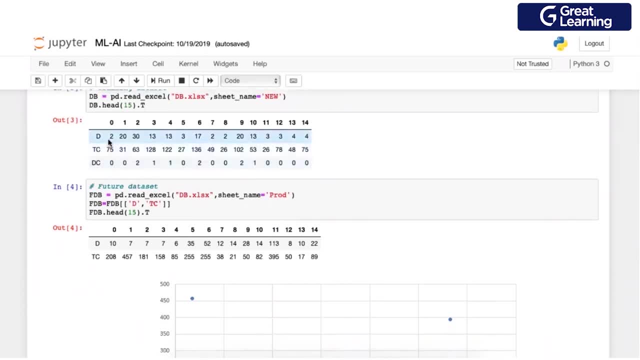 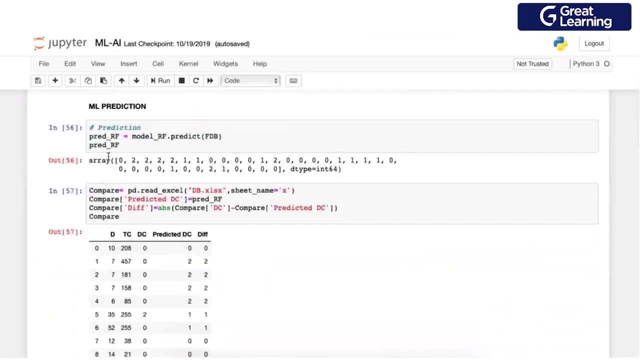 Simple levels. I don't expect you know to do image processing on all using ML, Not possible. Yep, Now to counter this up. what I've done is I have made a very simple neural network which starts from here, So you can forget whatever we did about. 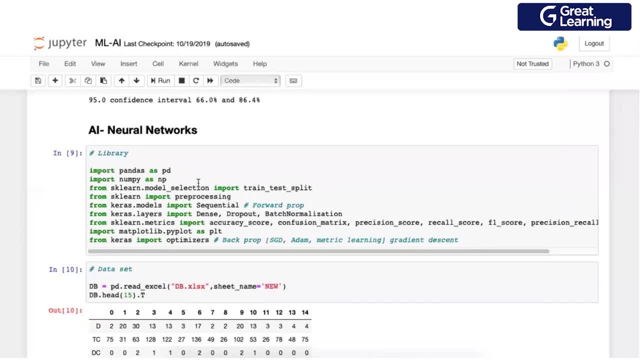 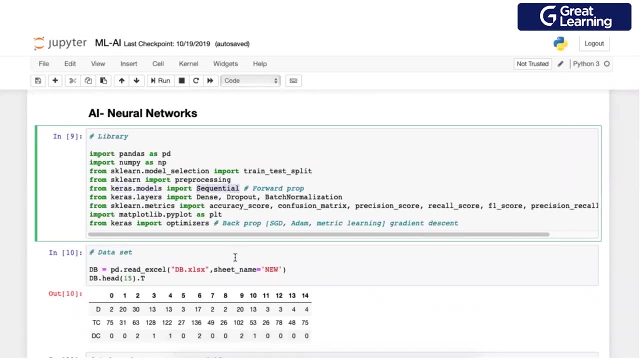 We know that our part. Next, what I'm doing is from Keras and implementing a sequential library. What does it mean? If you observe our Excel file, the simulation- I'm sorry, not this one- The simulation that we did. 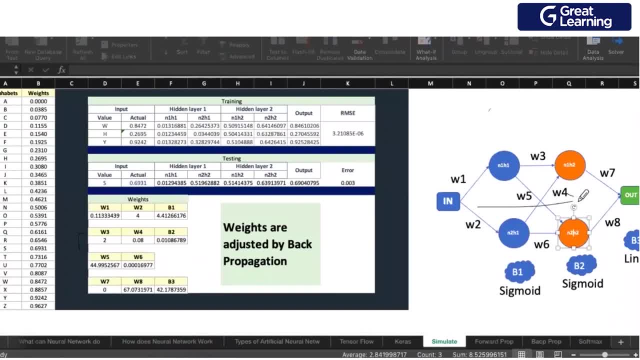 Don't you think this is sequential kind of stuff? This depends on this, This depends on this and this It's like a sequence. So the first part to understand encoding is we have to tell Keras that our model is sequential model. All right, 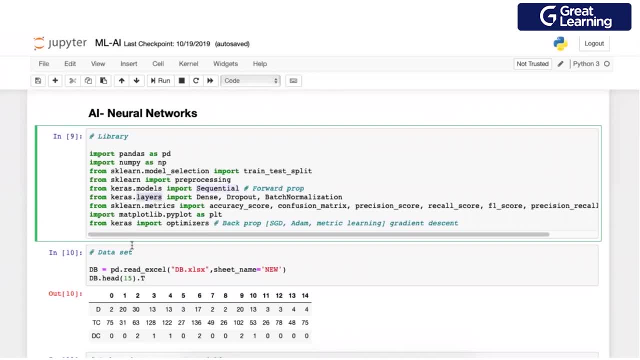 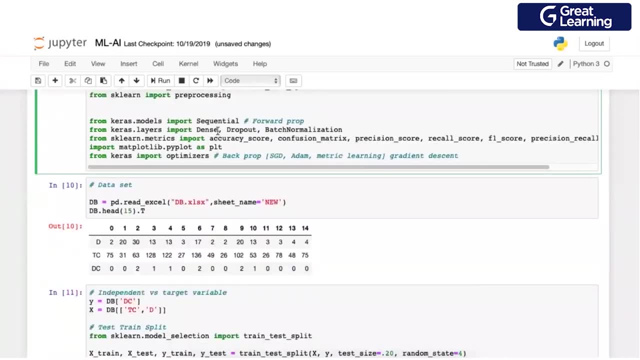 Next is: what layers you want under Keras. So if I yeah, what do you want under Keras? So, to add a layer, to keep adding those hidden layers, no, you have to use a command called dense. Next thing, if you want to drop out and if you want to do normalization, even it's possible. 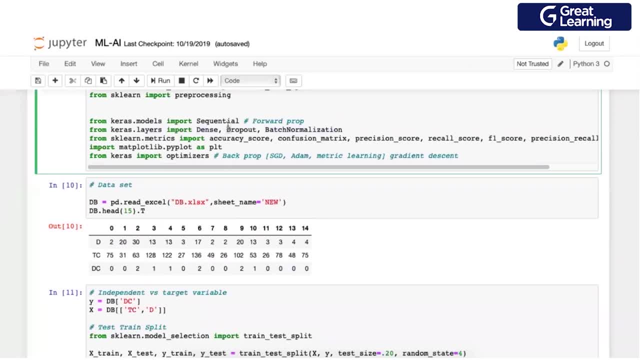 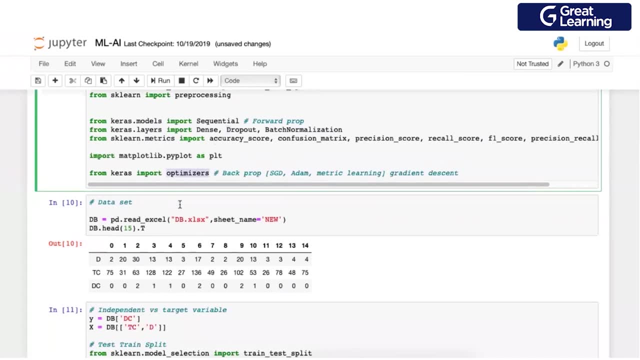 under Keras, So we'll we'll do it Okay. After that, we don't want a scale on and one more library as optimizers. So this is used for back propagation or gradient descent or to adjust your weights- Anything you can call about. 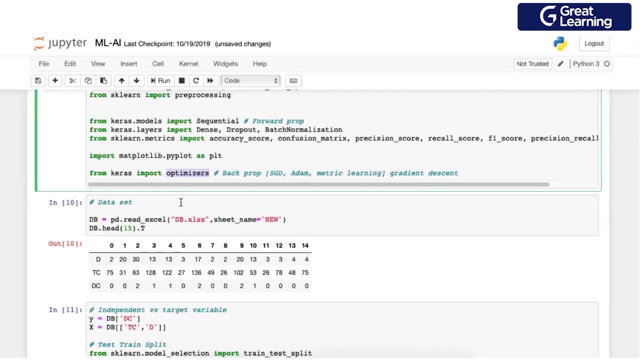 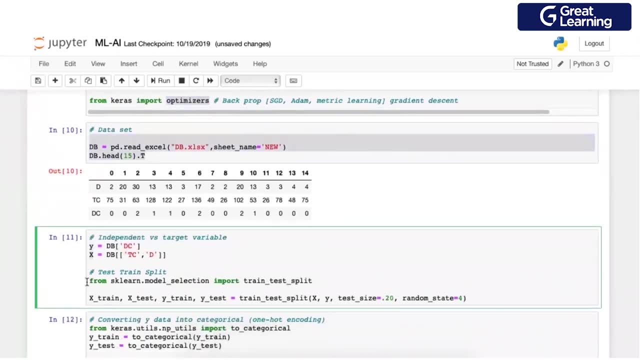 All right, Now let's go further. So, as usual, we'll import the data. No change in that. We will do. we'll define X and Y, No change in that. The only thing you have to be very careful is, even if the output is in the form of a. 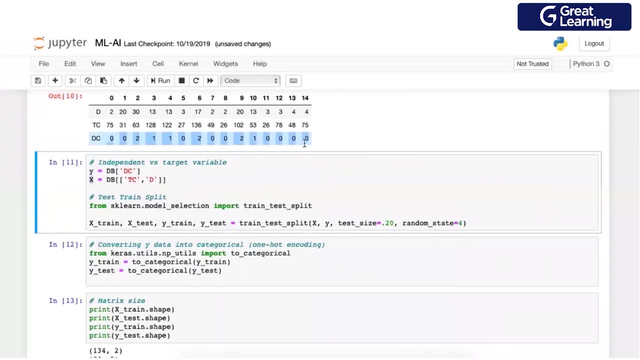 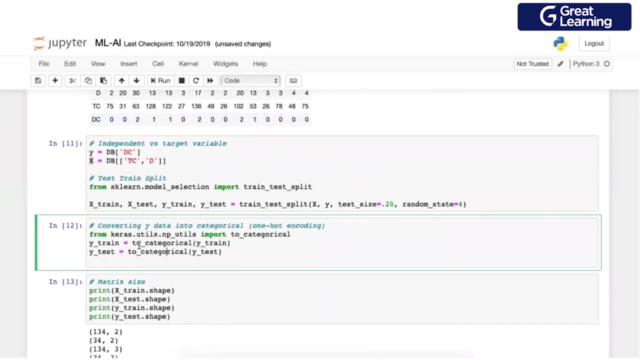 how do you say classes? yet you have to do a categorical out of it: category, in the sense you have to convert this into category, because if, in case, this looks like a category and it is not category, neural network is going to fail. So please be careful. 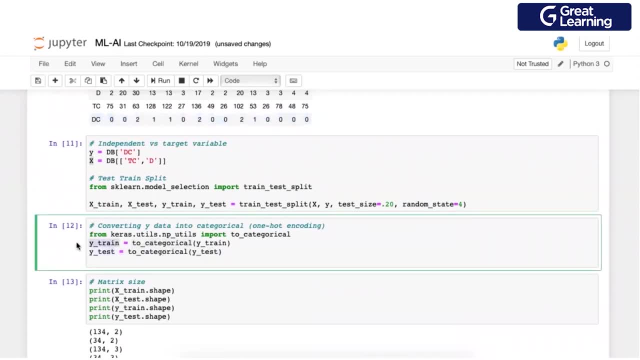 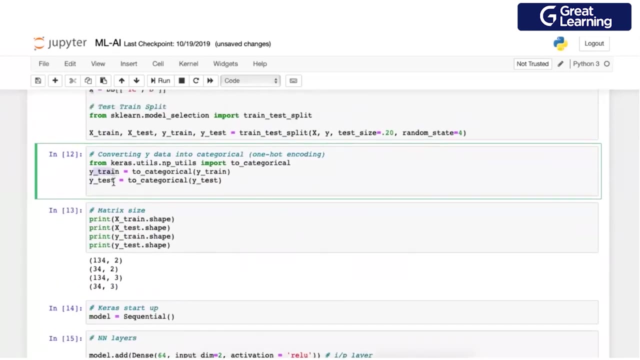 The output, the Y of each and every data in your data set should be categorical, no matter it is test or train, whatever it is. So either you do it before split or you do it after split. After split: the only issue is what I made a mistake here is they have to write two different. 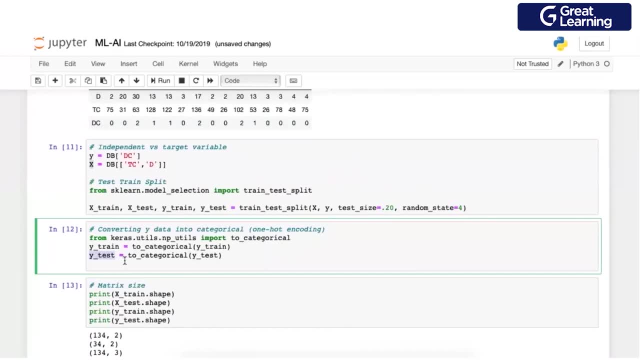 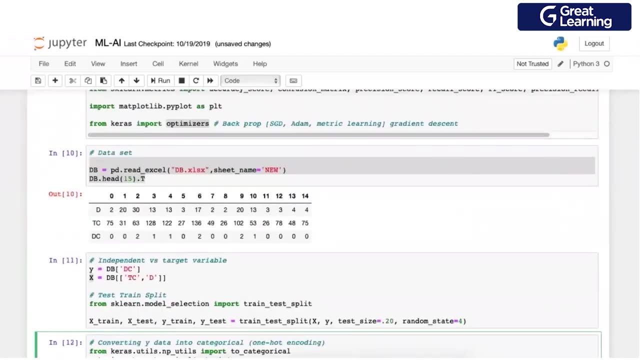 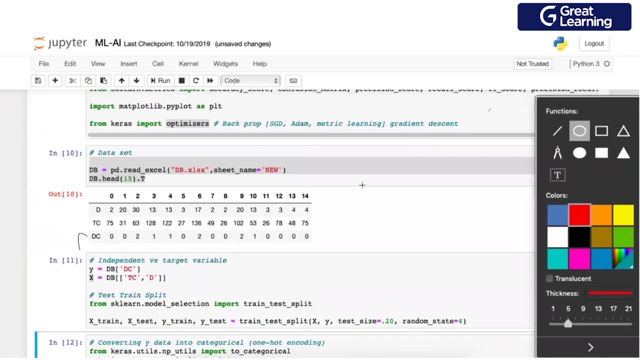 lines. What if I would have done earlier? It says one line was enough to categorize. All right After that. coming on to the inputs, Now can somebody tell me if I want to design a neural network here? Yeah, What should be my number of inputs? 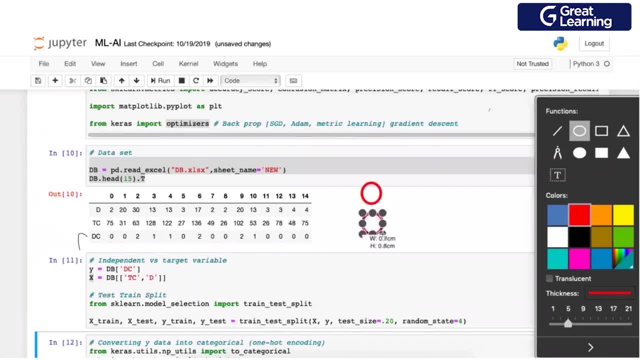 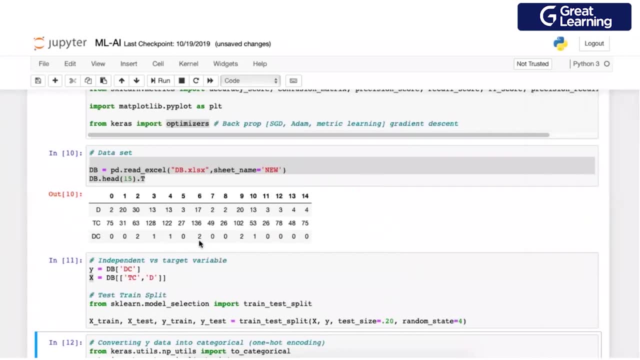 So I have to have some inputs, right? Oh, sorry, Perfect Two inputs, And what would be my number of outputs? One, Okay, I did not show you. There are actually three Zero one and two Zero one two. 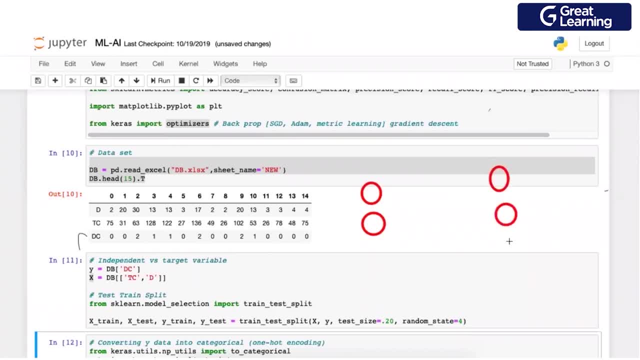 Okay, Perfect, So I'll have three outputs. Now, if I have three outputs, what activation function? I should use Softmax. Please remember that. No more relu and signal. Okay, So this is the input and output we designed. 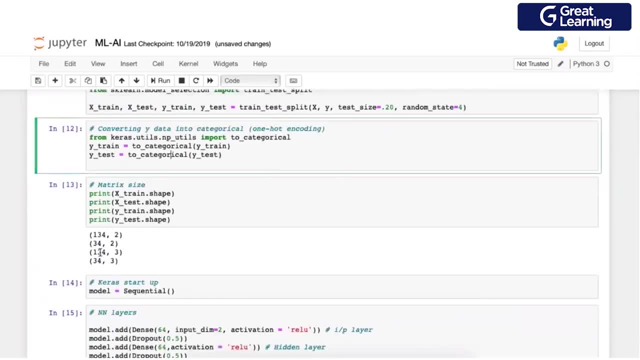 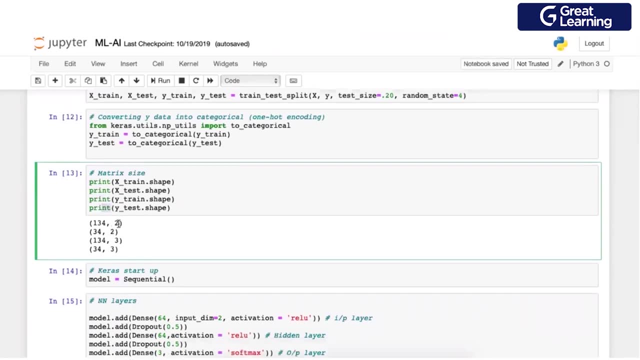 Now let's try to focus on the interior part. So before that, please remember, till you are confident enough to visualize all this, always print the shape of your test and train. So this will help you to design input. This will help you to design output. 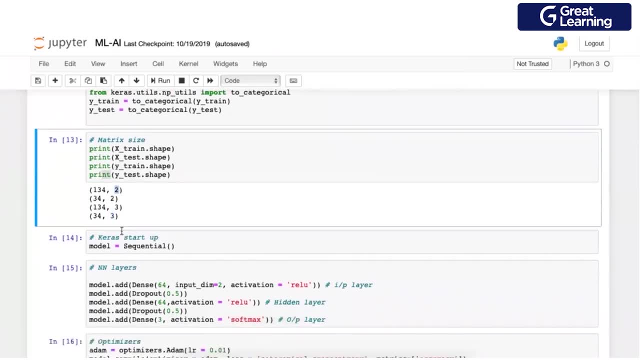 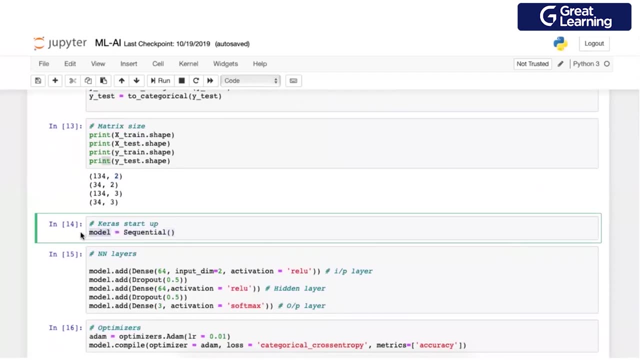 Got it: Three outputs, two inputs. So the first thing you have to fire up is you have to tell Python that this is a sequential model And the name of the model you're defining is model itself. And every time you make a change now you have to say modeladd. 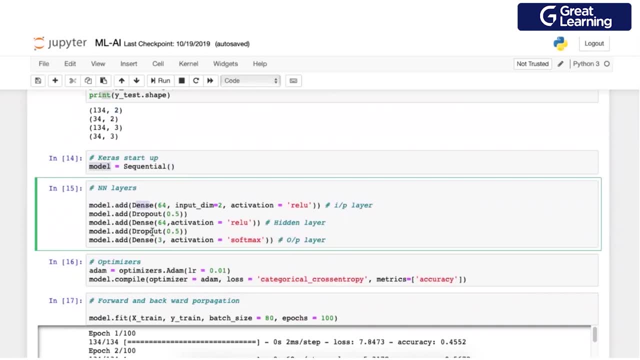 What I need to add? I need to add a dense layer. What is that dense layer? So, first of all, this is your first input layer. Now, in input layer, what we are doing is we are considering input layer itself as a neuron. 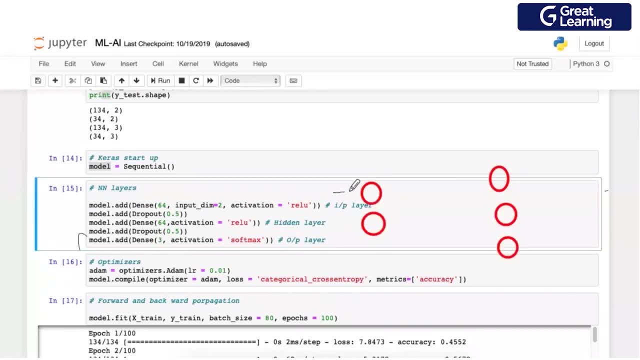 So you can say that yes, we are having a neuron here and we are giving input to it, So you can consider directly this as an input. Sometimes we don't take it up. Sometimes we start in new activation functions from hidden layers. 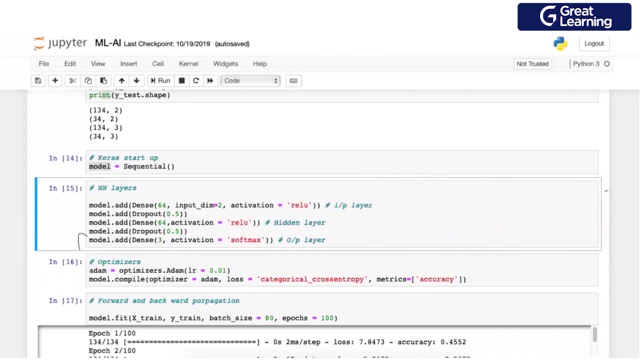 Yeah, In this case, what I've done is I am saying I want an input layer, I want an input layer of dimension two. That means I need two neurons and I need 64 weights. Now, if you ask me why? because my next layer is having 64 neurons. 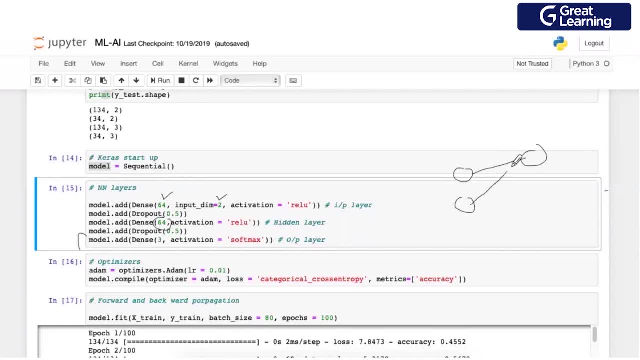 If you remember, each neuron is supposed to be connected to other one. So, like that, if I have 64 inside, I should have 64 lines of weights also Agreed. So this and this should be in sync. Next is I'm saying: 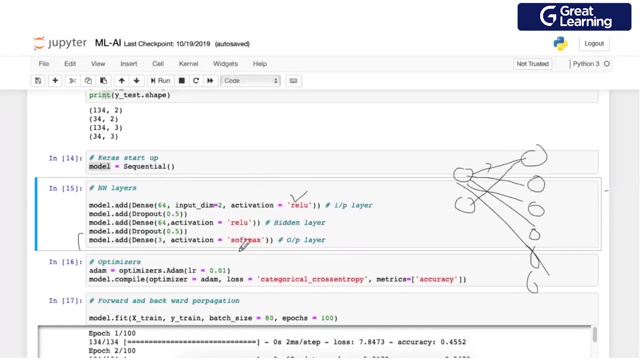 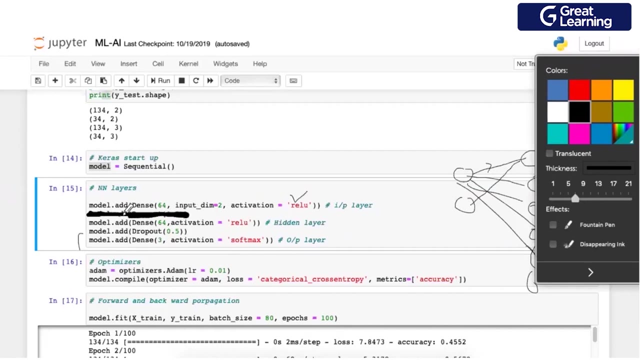 The activation function I'm going to use is ReLU for now. Now coming to. So please ignore dropout, because this is a. this is a topic from third week. Dropout means it switches off some of your neurons. It's a. it's a type of hyper parameterization or feature engineering in a neuron. 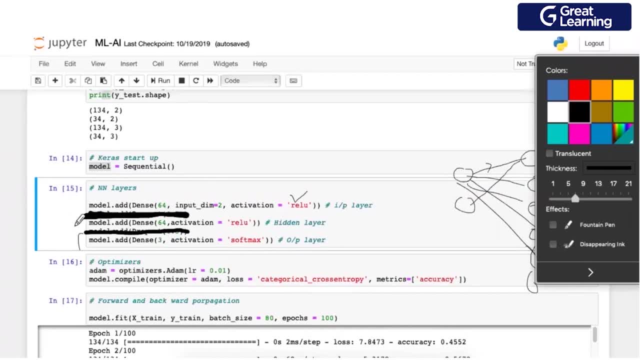 So please ignore for now these two. Next is I'm saying, is I will add another layer, That is my hidden layer, Such a way that it will have 64 neurons. Activation again is ReLU, And the third one is your output one. 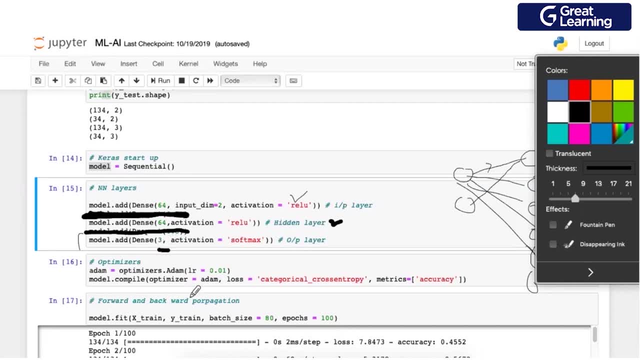 So output is, I'm saying is, I will add three layers. Sorry, I will add three neurons as an output. Activation by default is softmax. What if I have used ReLU here? I will get a regressed output. If I use softmax, I get a classified output. 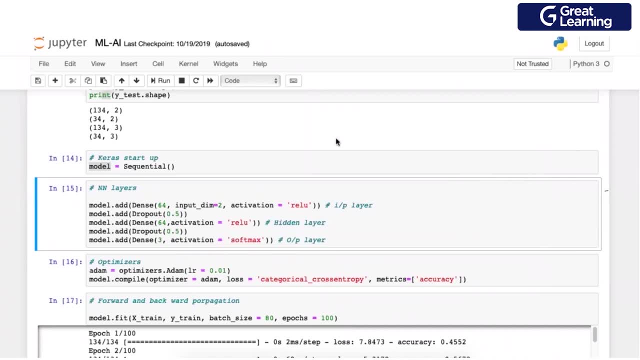 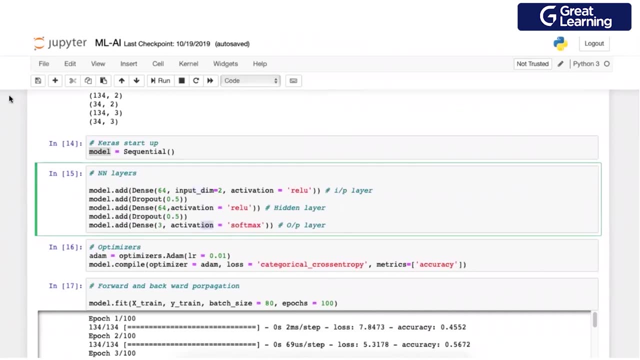 That's it All right. So this is your neural network on a very simplistic level: One layer, two layer, three layer. It is capable enough to deliver the same what ML gave us about Next. So we have done. We have created a hardware. 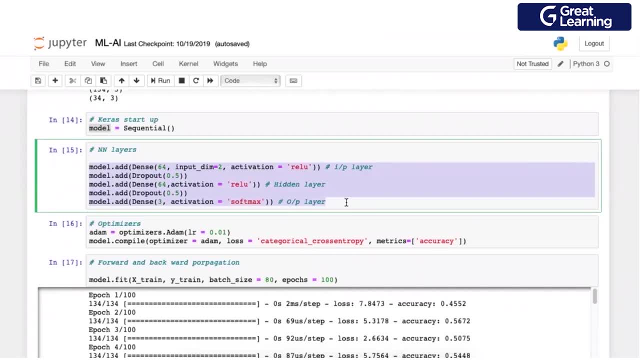 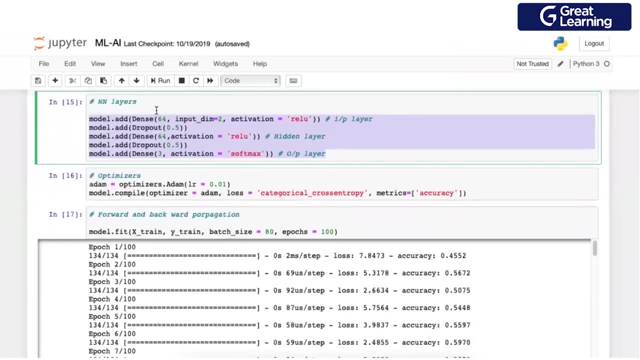 So I can say we have created an empty network. Now we are supposed to populate it. Now how do I populate it? Before populating it, we have to design backprop. So I can say: this is forward prop, This is your back propagation. 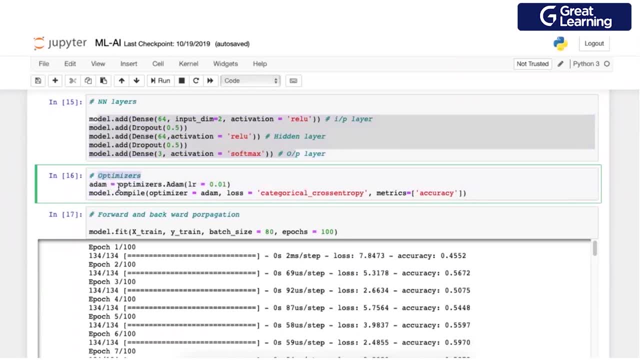 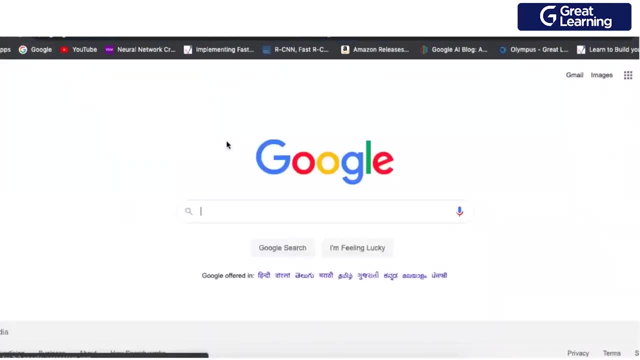 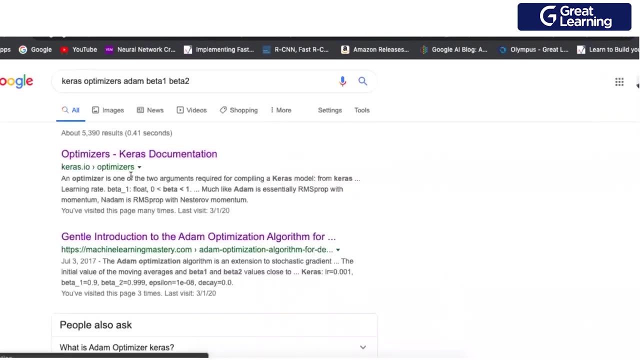 Back propagation is nothing but optimizers. So there are so many optimizers available. So if you want to see The list of optimizer, you can just go to Google Keras optimizers. Okay, This is the documentation which will help you to understand all the optimizers available. 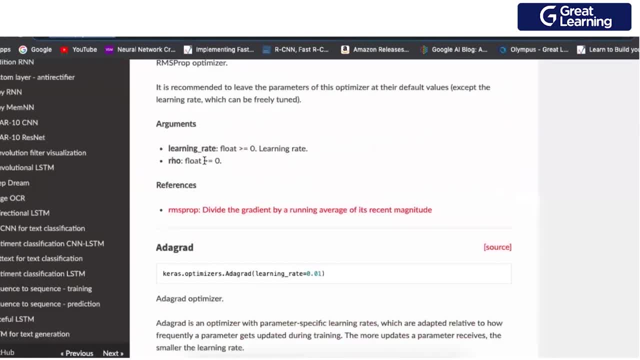 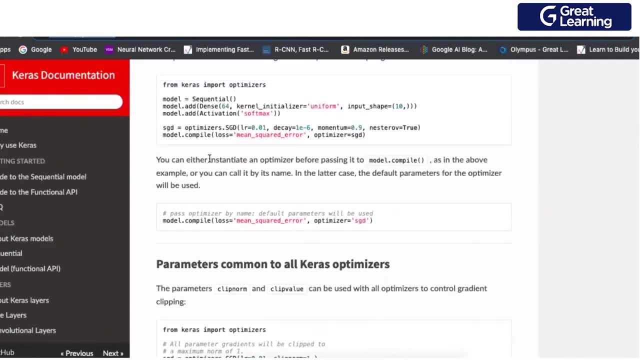 within Keras. I will show you each one in each case. Okay, RMS, prop, ADA, delta, ADA, grad Adam, SGD, all of them. I'll show you one by one. So for now, let's talk about a very simple optimizer, which is Keras. 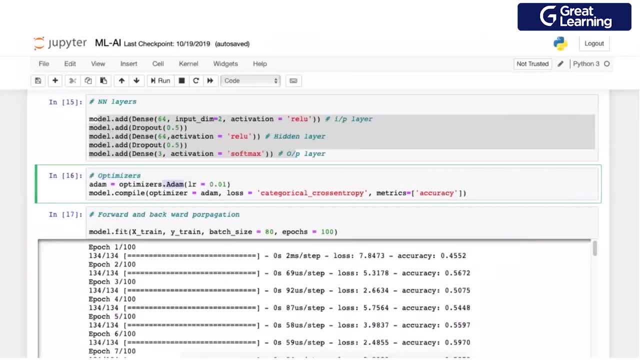 Okay, So for now, let's talk about a very simple optimizer, which is Adam. Now, if you ask me what is optimizer? Very simple. Remember dou L by dou of weights. The formula or the person who does this is this particular person called Adam. 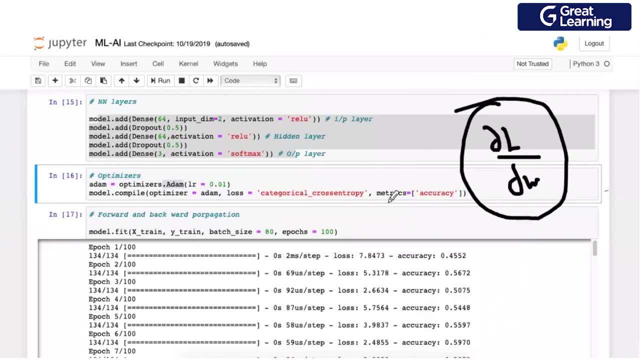 All right, Instead of Adam you can have SGD, RMS, prop, ADA, grad. A lot of things we have Depends on the application. what we are choosing In this case it's a very simple numeric application. Adam works the best. 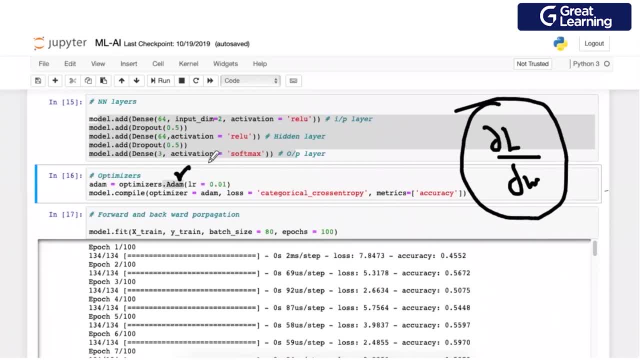 It is something like a ReLU, a generic. You can trust him for all the backprop. Okay, So let's see what we have here. Okay, So this is a very simple numeric application. Adam works the best. It is something like a ReLU, a generic. 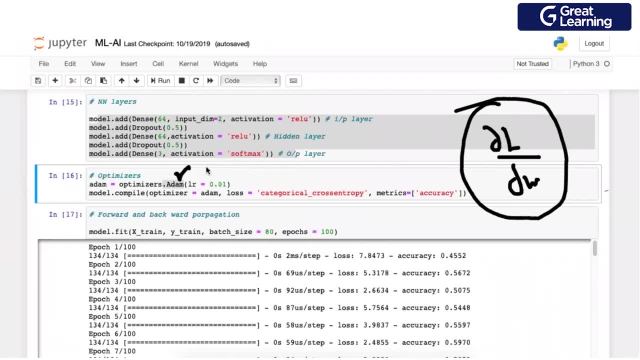 You can trust him for all the backprops And also you have an option to define a learning rate. So that is the. I keep it usually in two decimals: 0.01. if you want to be a little slow, If you want to be very dynamic, you can put large. 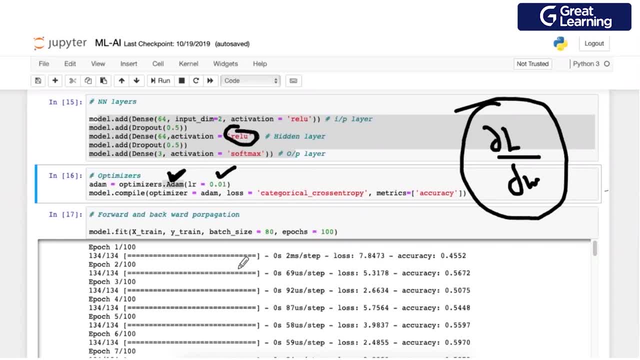 But if you have a large activation function- please remember we just discussed- it is going to oscillate. So it's not going to oscillate, It is going to be a little slow. If you want to be very dynamic, you can put large. 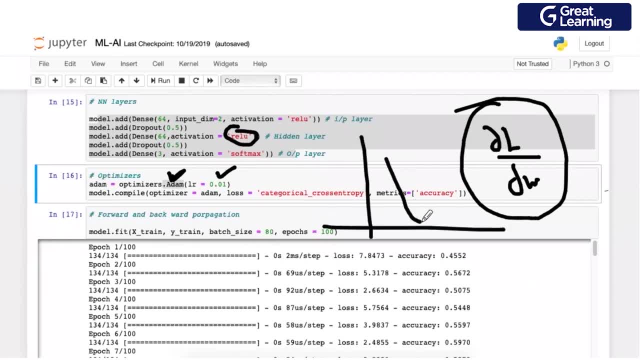 But if you have a large activation function- please remember we just discussed it is going to oscillate. Okay, Will not come to a rest point, But yes, your neural network training will be faster, also in the larger Learning way. So this is your Adam. Now you are saying: this is my model. please attach. 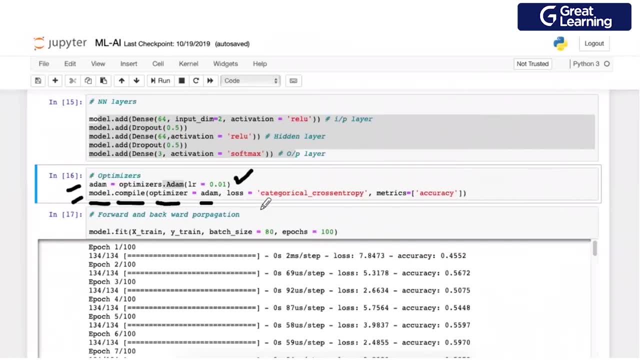 This optimizer, which is called Adam The loss. the way he is going to calculate loss function is nothing, But it is a categorical data and we are going to use cross entropy. guys. What is cross entropy? We know entropy right. What do you mean by cross entropy? 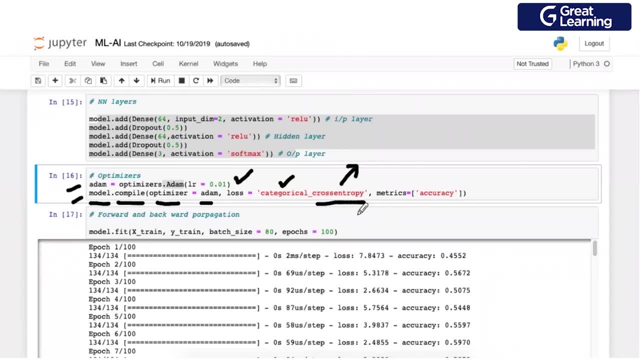 Have you heard or have I told you? I think I have not discussed. You know, entropy. Alright, so I do one thing: in next session I will give you some mathematic behind it and we'll try to see one or two Python examples. There are so many loss functions available in neural nets. 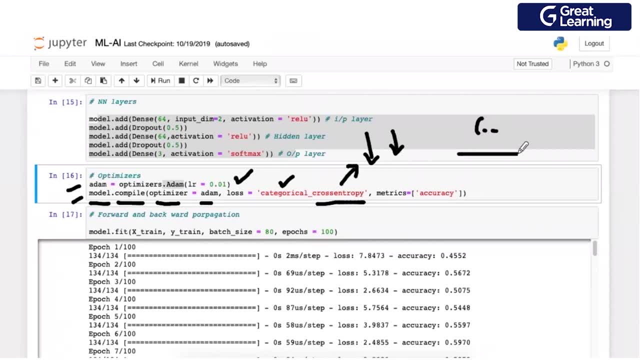 One is called cross entropy if the data is categorical. categorical cross Entropy if your data is pass. what do you mean by sparse? There are a lot of zeros as an in the output. in that case You can say that Yes, it is. 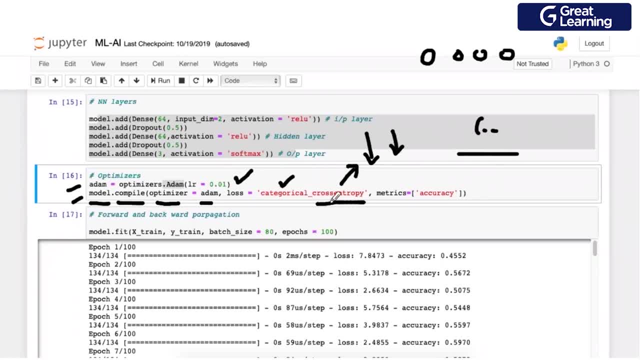 sparse, underscore, category underscore and cross entropy. you have multiple of them available for Now. whenever you see category, use this one. This is the best one. Post that what is what should be your checkpoint. So I am saying accuracy will be my checkpoint. do we know any other checkpoints? We know precision, we know recall. 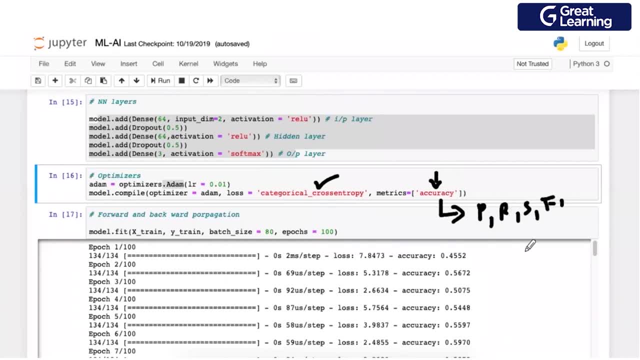 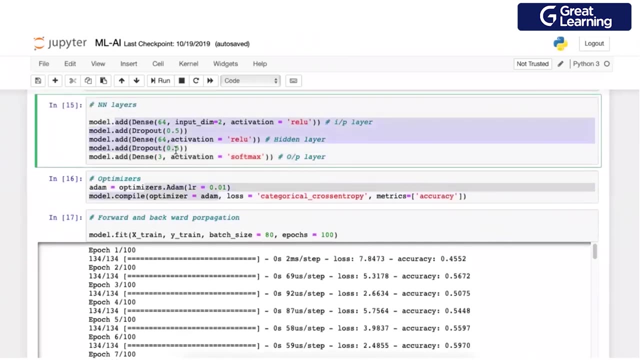 We know support, we know f1 score right, So this is what you can use. always, I will say: Use accuracy. accuracy is a very reliable factor so far. Next, what I do is so: my back prop is ready, My forward prop is ready. Both of them are ready. 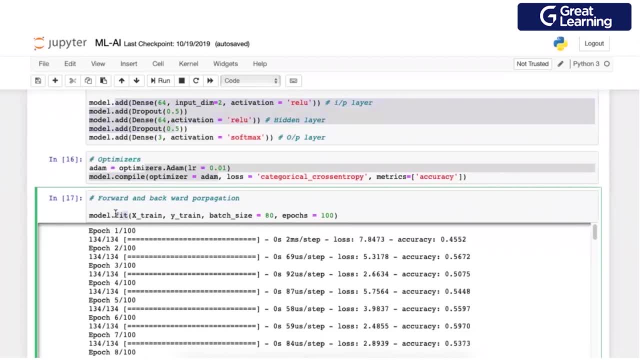 So you fire it up as usual from your machine learning fitting. So just take the model, fit it, fit on to what your training data. Okay, that size. now This is something new. That size means if your RAM is capable enough to fetch the input at a time. 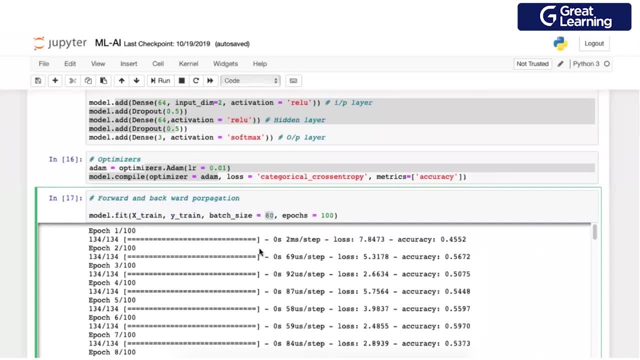 I would like to fetch input for next 80 readings. You know so, if you have a good RAM even you can put 800. So if you are doing a computer vision, image processing and all that, We usually keep batch sizes very big so that the fetching is faster. in this case, 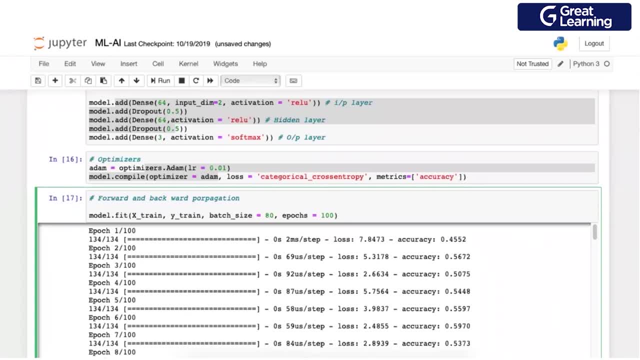 You can choose any random value, like it's something like our seed, if you remember random seed, But here it is about fetch executions. Next comes your epochs. Now, What is epoch? Please remember: one epoch is equal to one forward prop plus one backward drop. That's it. Now You may ask me: fine, How do we choose this up? 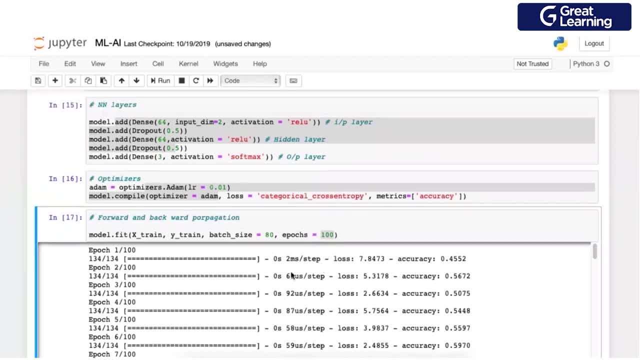 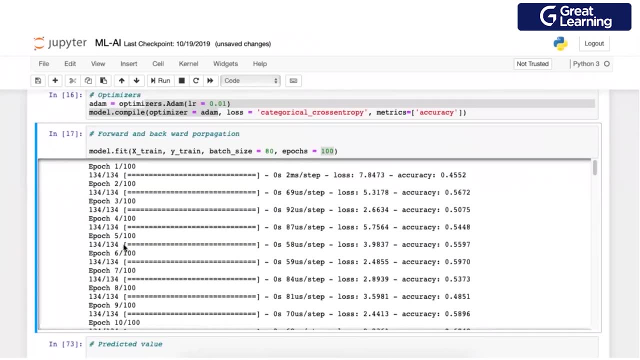 So what I would say is, first of all, You choose single digit epoch, say five, six, seven, like that- And once you do that, look at the first five epochs. So let us say these are my first Five epochs till here. look at the loss function: Yeah, can I say it is having a huge amount of change you observe. 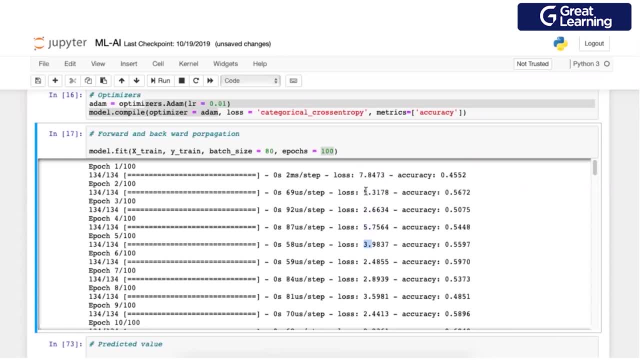 There is a considerable amount of change. a change difference of two is huge enough. So if you find in first five or ten epochs that the changes are very huge, then you say, okay, Let's use fifty hundred, two hundred, like that, or else you can check the accuracy if you find the accuracy is continuously. 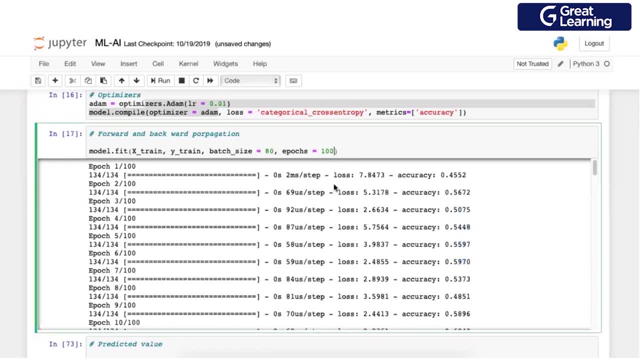 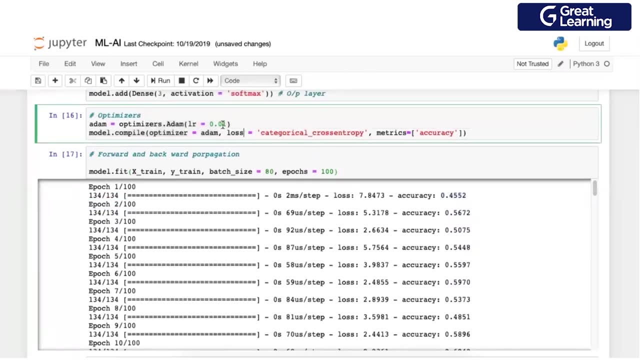 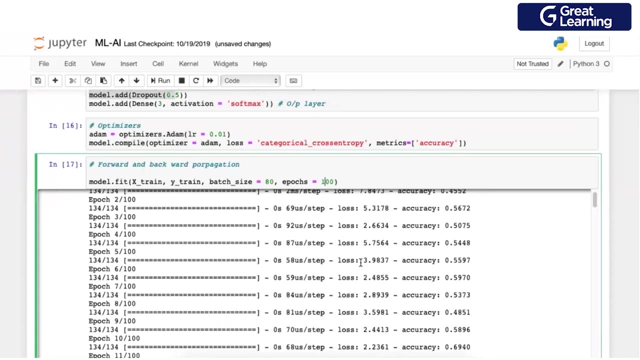 Increasing by a good number. then you say that, yes, if I have more deep box, more accuracy I'm gonna get. that means more number of epochs, more back prop, more back prop, better the weights, better the weights near are your accuracy, or I'll say, nearer. two hundred is in this case. when I ran for one hundred times I. 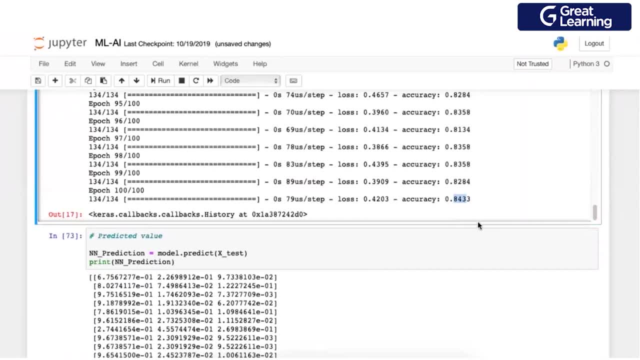 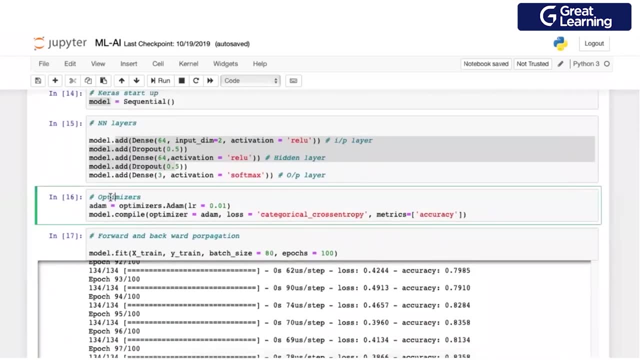 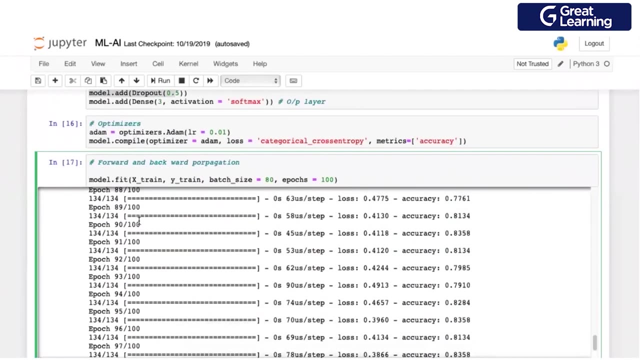 got an accuracy of eighty four. It is not as good as ML, because in ML we got ninety, But this is a very dynamic model. what does it mean tomorrow when my inputs change? let us say, it takes no time for me to retrain this. i know even our ml takes no time, but in ml we have to do hyper parameters and all those things. 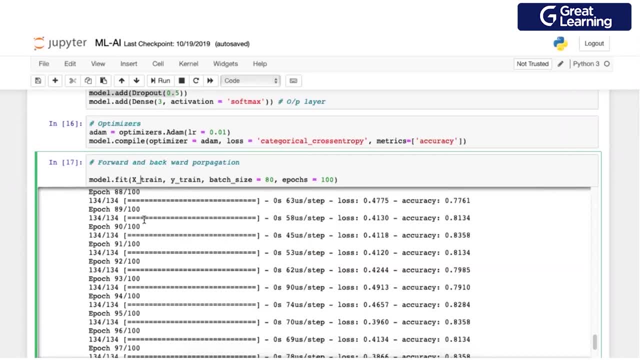 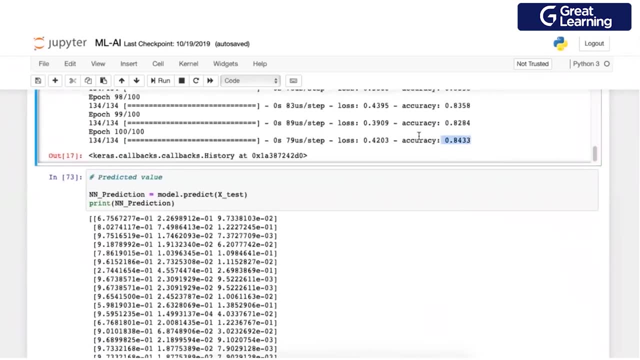 feature engineering and we have to take a lot of pain to again redo. in this case it will auto take the changes and auto adjust the weights and at the end it will try to show us results somewhere near us. there are certain weird cases where you might find ml has an edge over this. yes, 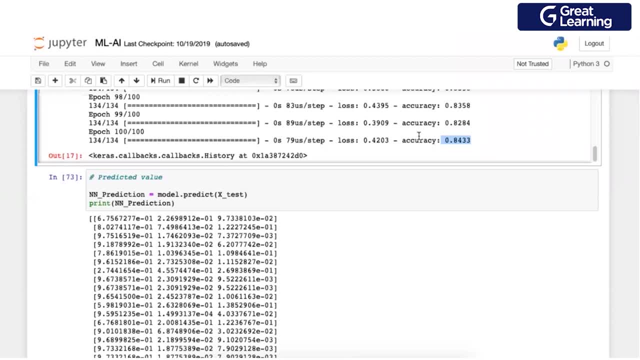 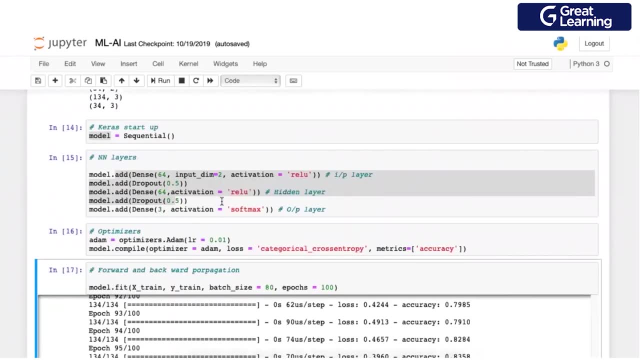 but more or the less deep learning should be good. all right now, what do we do? let me show you what is soft max. so, if you remember, the output was soft max, how many? three of them. so look at this: this is the predicted output that we have got. 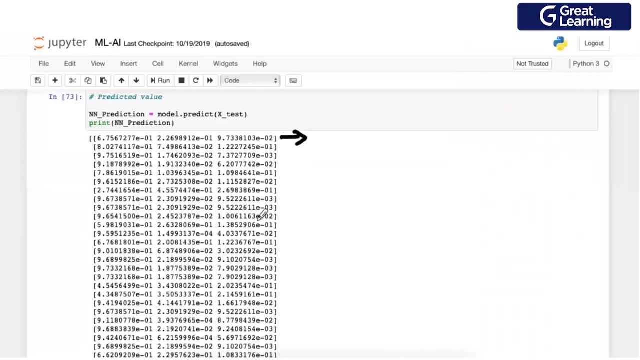 now, what are these? these are nothing but your probabilities. soft max will pick up, so all three of them will get a probability. so let us say, if i have given an input and i'm, so i'm expecting answer is three. that means one, two and three. so soft max will give me a probability. what 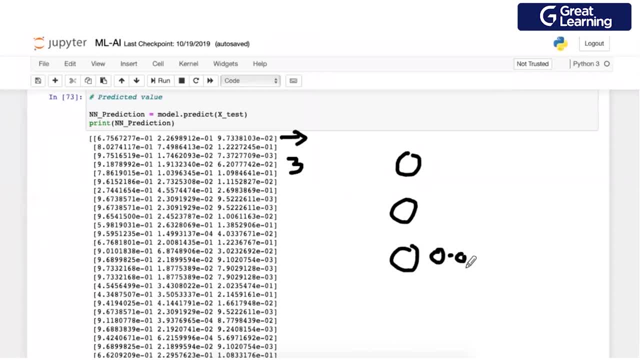 is the probability that? the answer is three. let us say the probability is 0.9, this is 0.7, this is 0.3. the soft max will pick up the neuron which has having highest probability. so just to show you, guys, this is the probability that we have got and if you see the highest probability, 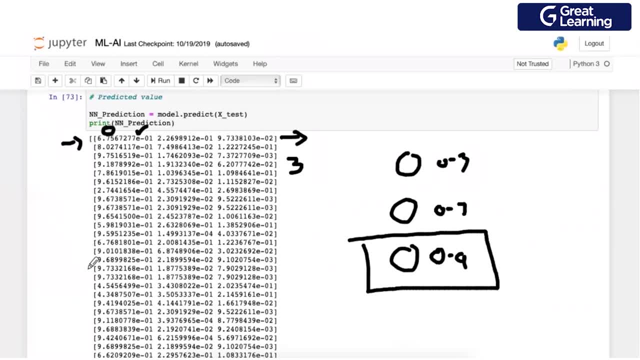 this is the highest probability that we have got and, if you see, the highest probability belongs to this particular person. so the answer is zero. so my classes are zero. one and two. all right, you don't have to do this just for your showing purpose of soft max, that's it. and 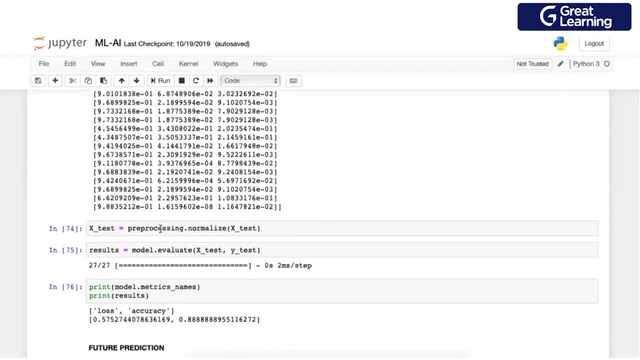 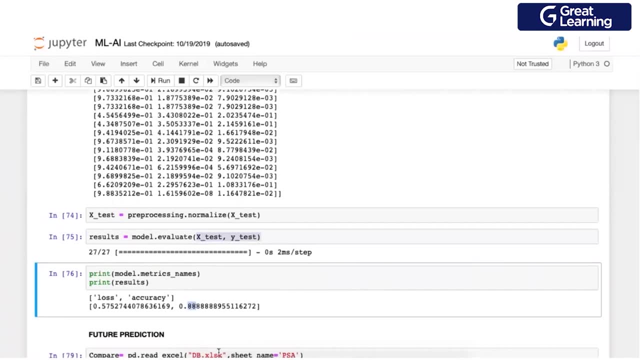 finally, you do your testing part of it. so you take your model and run it or evaluate on your test data. so when you do it, i get an accuracy of around 88, so which is a little more than 84 i know. so what we would have made a mistake here is why it would have shooted. 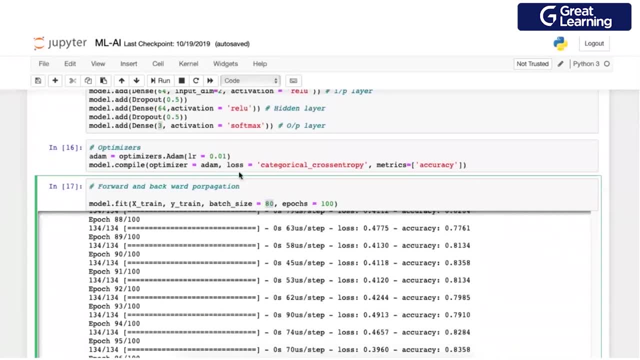 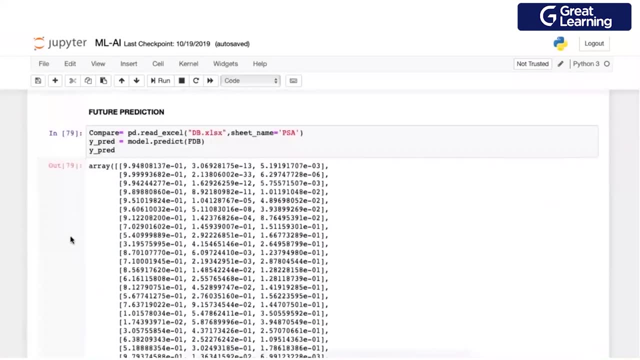 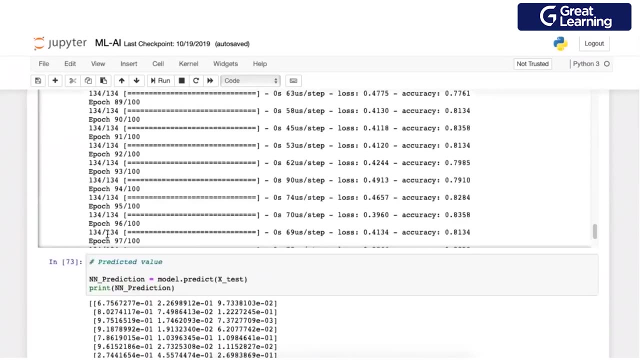 up high is because of a bad size or number of epochs or learning rate. so you can go back and just adjust it somehow. so i can say that, yes, this works good. on my testing data i got an accuracy, say, of 88, perfectly good. so this is how you can train a very simple neural network. so i will again. 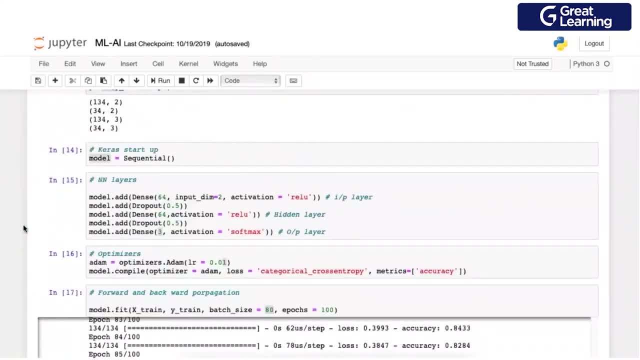 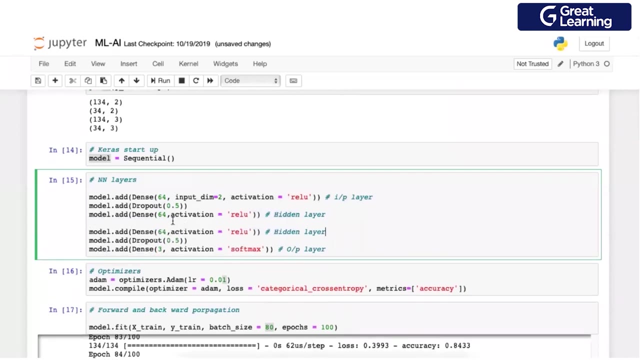 request all of you is: pick up some of your machine learning, old data and try to build a model like this and see how you are getting, and then try playing around with more layers. so now, if you want to add a one more layer, what to do? very simple: copy this, put it now. when you put it, you can keep the same. 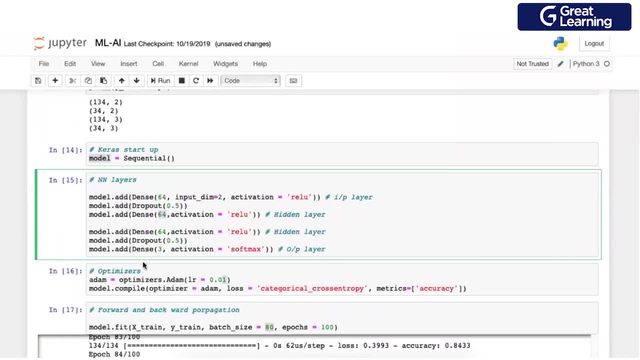 number, not a problem. now you may ask: okay, how did you get 64? there is no logic for that. so what i do is say i start with some number. say i would have started with hundred. if i have hundred weights, my next layer should have hundred neurons to take it up. if i want my numbers to diminish, i will say my. 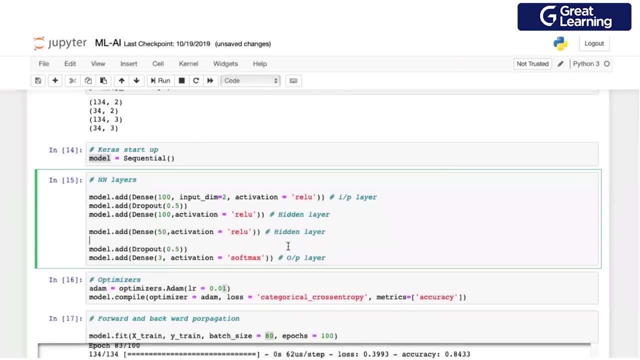 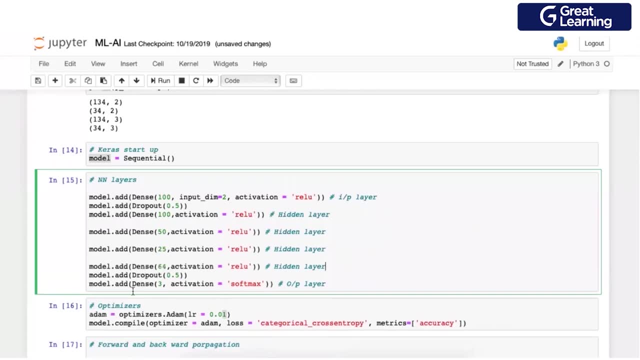 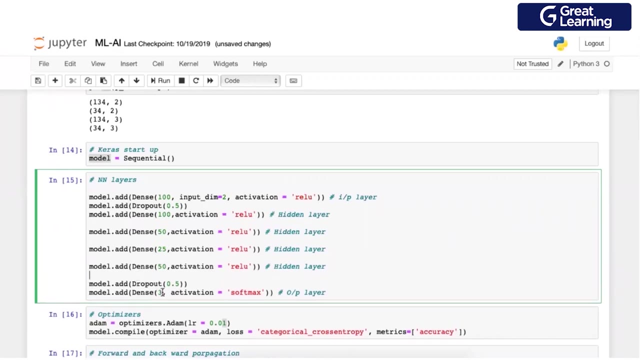 next layer will have 50 neurons. you can have one more hidden layer here saying that my next layer will have 25 neurons. if you want one more, you can say: my next layer will have, say, 15 neurons, you can. you can double it up, not a problem, and from 50 it will converge to your wish, all right. so some of my other batches: 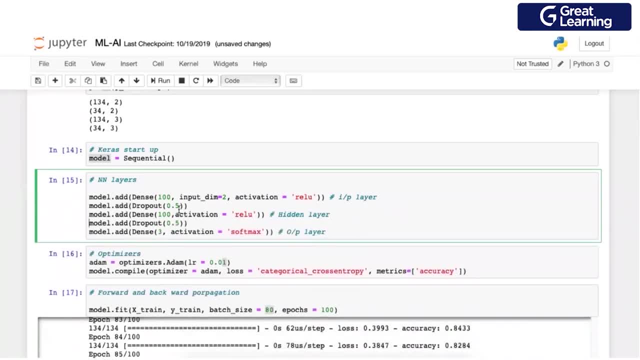 is also asking me if i can give some mathematics behind it, how to design this. i will again say there is no proven math that how to choose these numbers optimally. but yes, I have got some links to some blogs where they have done some equations, but that is specific only to their data, so you 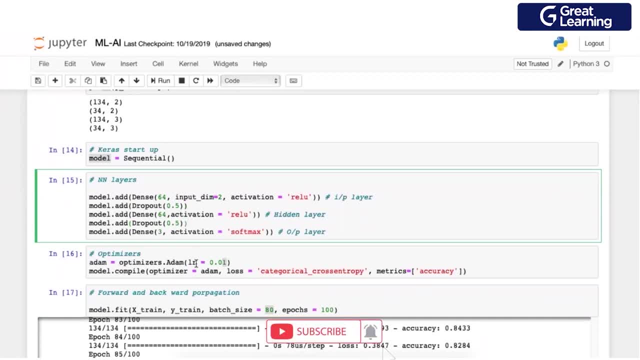 can just take some learnings and more or the less this is the way you identify clear. so try this up on your old data and let me know how comfortable you guys are on forward and backward. alright, so I am done. so I think we have covered for. 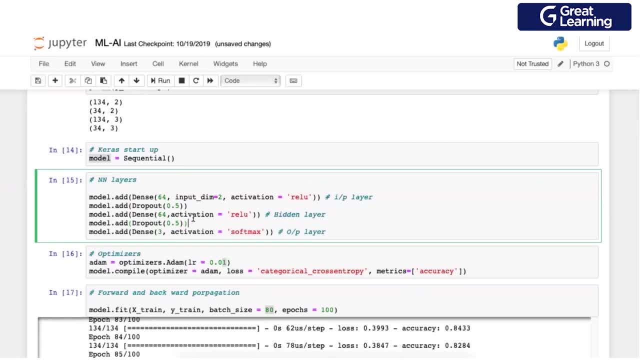 one and half week now, because forward, back and all were part of our next week. but good, I feel if I show you something you should also understand, so I don't want you to miss out anything. yeah, so I think we are going good. we will almost complete everything by next week or by third week starting, so we'll have some. 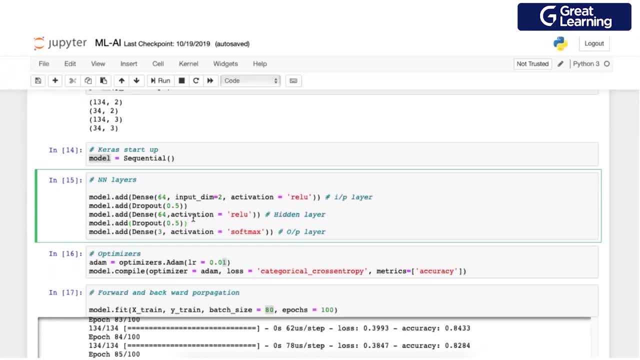 extra one hour and try to show you some deep learning. more networks on to this. yeah, image classification, text classification, all that we'll see down the line. we'll do some social media analysis. you 'll see some data types and all those things using deep learning. okay, good, any. 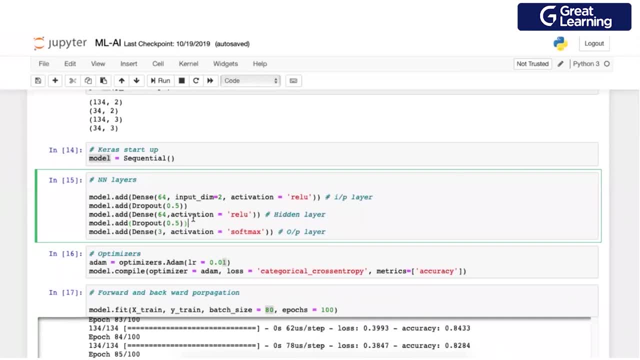 questions for me, or we can just one question: unless and until we find out the correct number of hidden layers, do you feel that ML is going to have advantage over AI? deep learning, yes, correct, correct. so what one of my learner did was- he is very ambitious enough to find the answer for this- what he did, he. 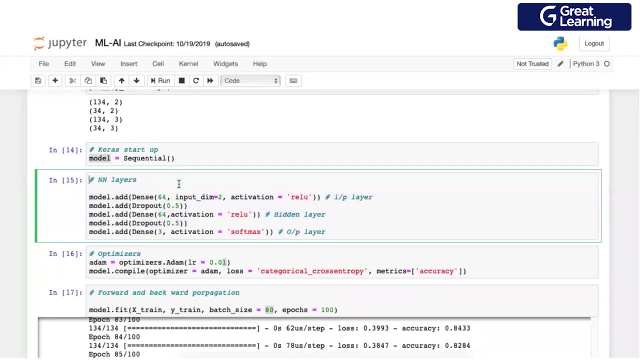 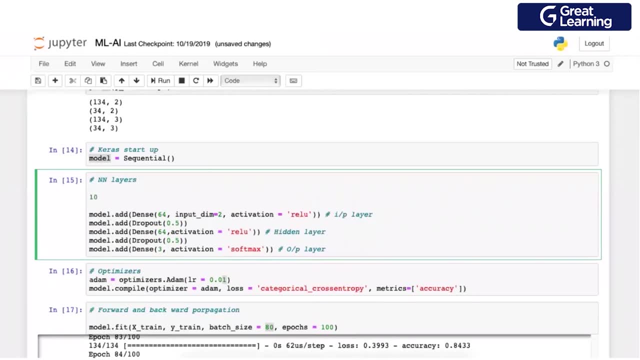 did critic on this. he said he did search. he put lot of layers. so let us say, in grid search he said it okay, I won. number of written lips could be 10, it could be 20, it could be 40, like that he started and he ended up spending two. 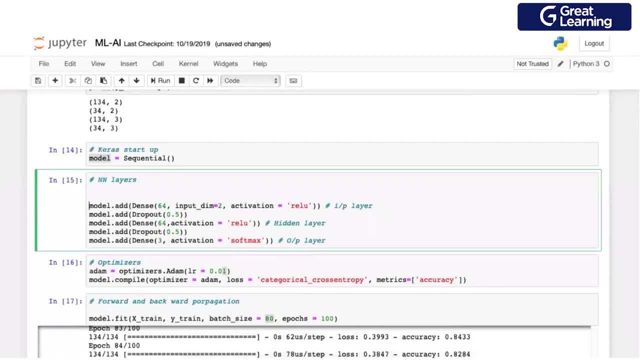 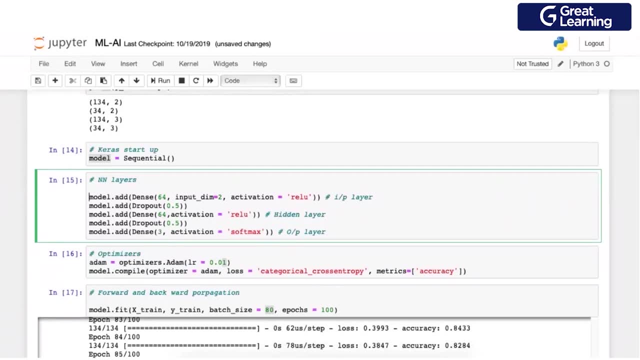 or three days for the neural network just to run. that is real confusion about, about. or, if we have, if we have a very, if you don't want to take the pain of mix matching this stuff up, yes, ML has an edge onto this, but ML cannot work. or I will say: 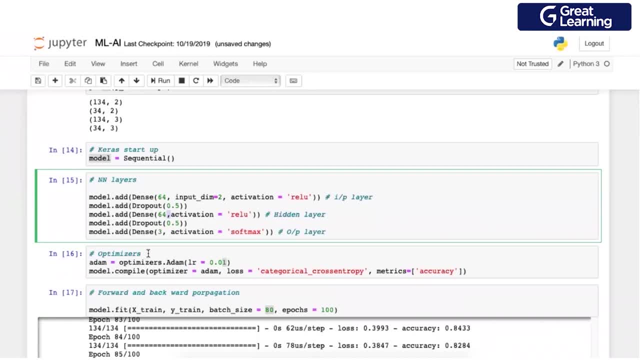 supervised learning cannot work onto computer vision and NLP so by default, this is the only backbone for image processing and text process. okay, okay, yes, so anyway, people come back to this. but yes, if we don't have time to and patience to basically do this, you have ML has an edge onto. 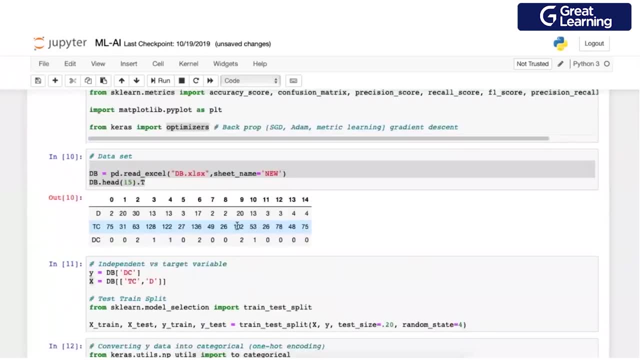 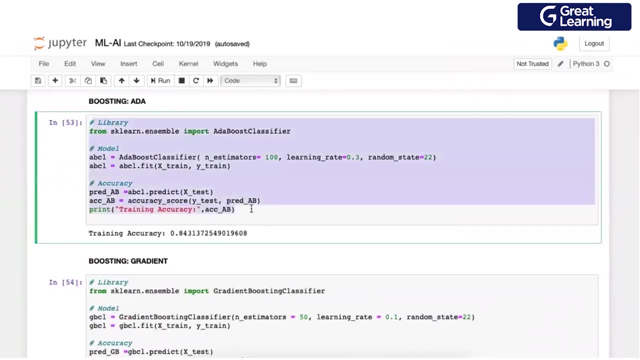 that I agree with you perfectly and I am clearly saying here: in this case study, I still feel boosting is having a big edge over the other one because it's a very simple algorithm. in four to five steps it is giving you everything, whereas in ML we had to do a little. 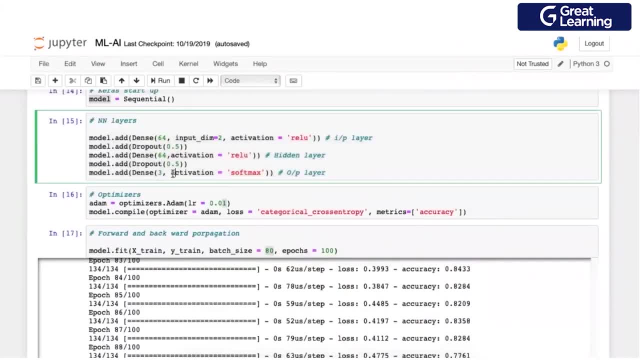 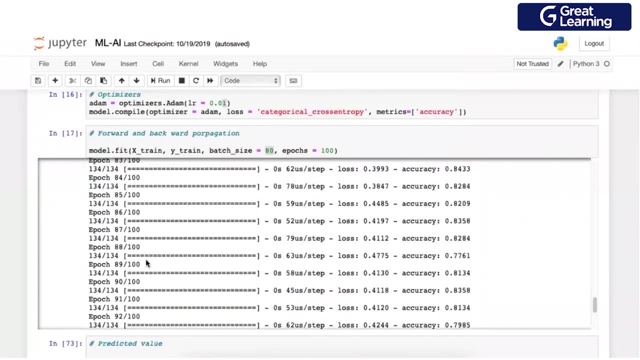 bit of an extensive part of it, but on the long run this is far better, I feel, because it auto corrects, auto launch itself, auto corrects its own weights also, okay, okay. so again, to summarize very quickly, the whole game of neural network is to adjust their weights. that's it. 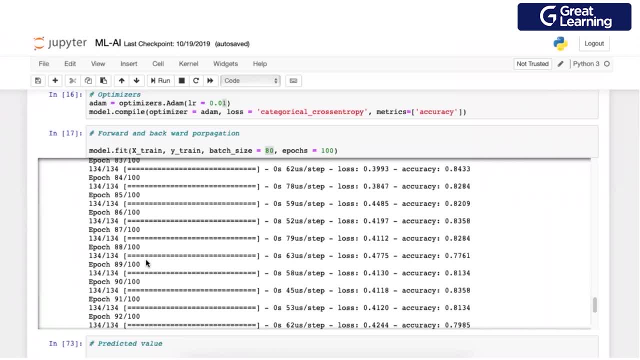 how do we get this? weights? we will do in week three what are different type of weights. for now, please remember weights are random, but also we have a provision where you can control your weights. you will see down the line in your third week when you do hyperparameter. 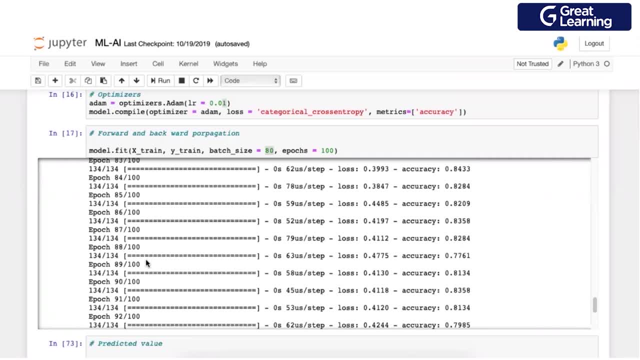 all right. and second thing is there is two type of propagation happening: forward prop, backward prop. forward prop is to spoil your output. backward prop is to adjust your own or adjust your loss function good. next is you have three layers: input layer, which should be in sync with number of columns or features. 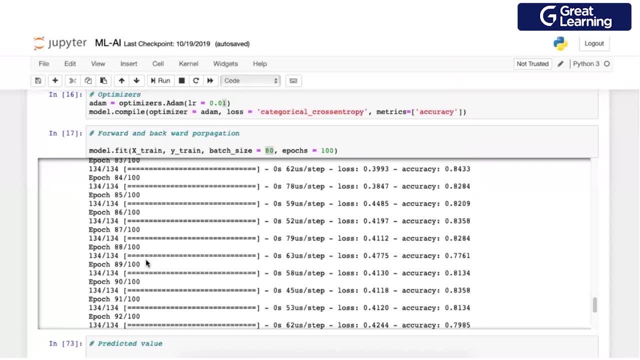 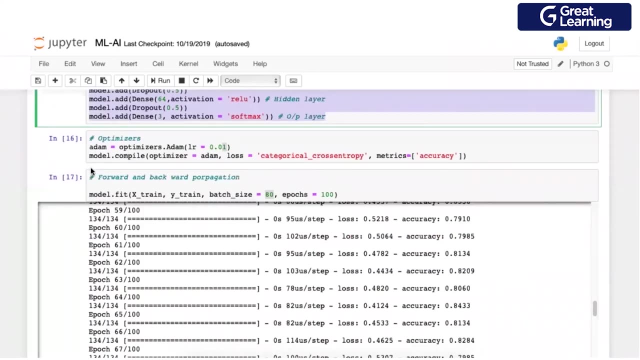 available output layer should be in sync with total number of categories you have on your output column. good, and the hidden layers. that means a big myth and I will say: start with a with a number like hundred, 120, 150, and then keep reducing it halfway, divide by three or 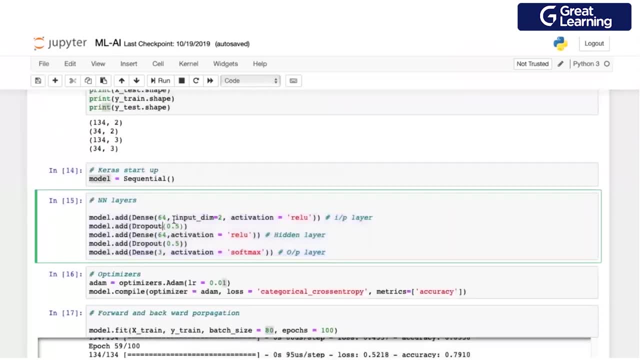 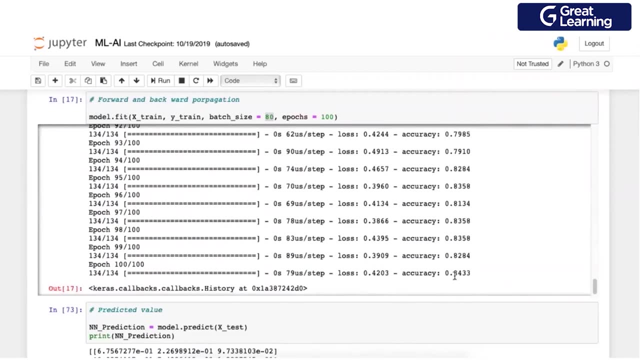 divided by four. but yes, it's a cumbersome process. we don't in one shot. see, I got this, but not always. we can get an 84% accuracy in a shot to the very front and still I stopped at hundred. you know, if I have gone further, I would have. 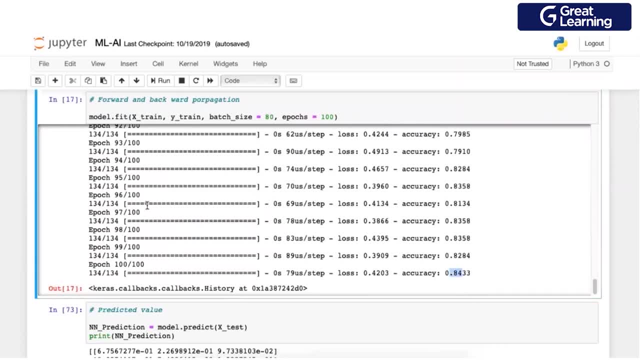 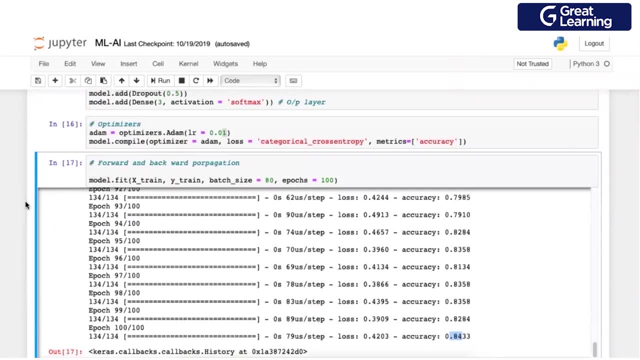 got at least 90 plus accuracy. yes, so this is the overall summary for neural networks. good, so now can I say the. the concept is little. the border is one little less on the understanding part. now, I think if you go back and watch the videos, no, I think. 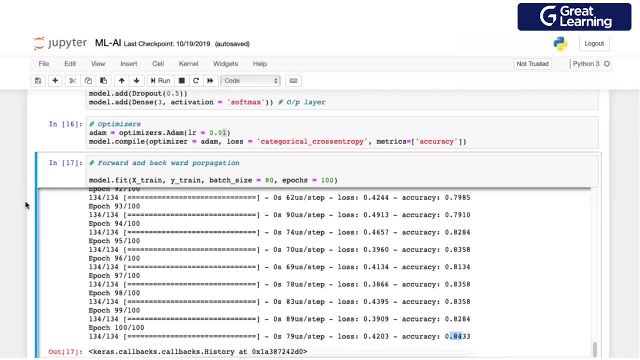 more the theory. what professor is explaining would be more interesting. yes, the way for computer vision. computer vision is going to go on a different level again. we may need to use glasses to correct that reason exactly. but yes, next five to ten years from the, they are for deep learning. so, and last ten years? 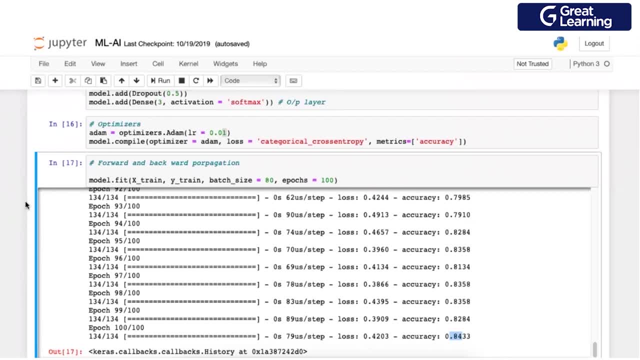 where for machine learning. now there has come for deepness, because you remember I showed you guys Auto ML, remember that code which will auto take our input. I don't know some of you were there with me. yeah, I think some some session in Camel. Camel is auto MLE, so you can. 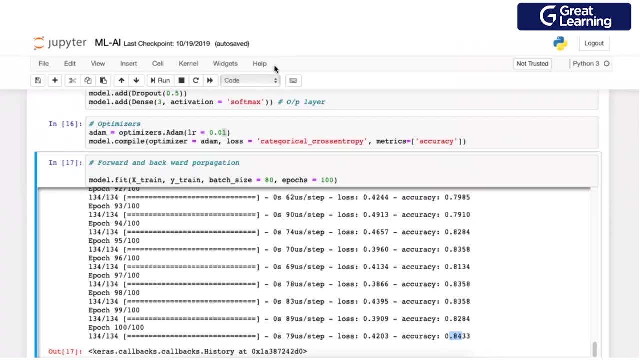 easily replace a machine learning data scientist who knows only machine learning, with that piece of code. if you want me to show it again, I will show you guys again. so already in my work and some of the codes that I do here for my newer batches, I already use Auto ML on. 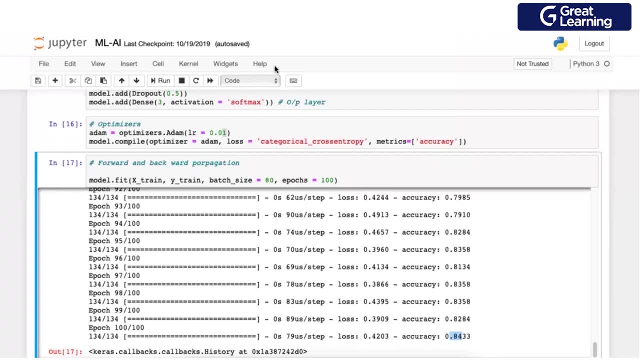 to that I don't need any more. I will use Auto ML to get my predictions, and it is becoming very common. now. even Google has come out with something like an Auto ML which is similar to that, as your already has it. so now, if you want edge, yes, deep. 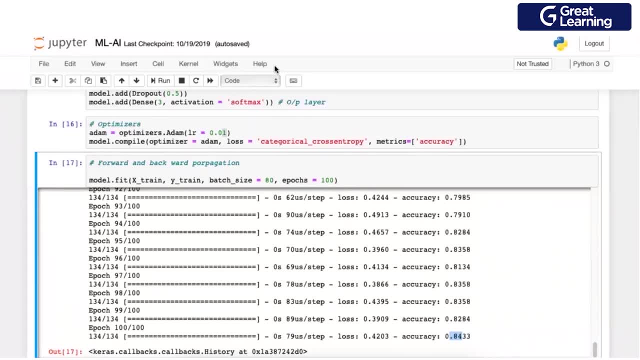 learning is the next one. because we do not have Auto DL as of such, it takes some time to come, okay, so take it in the slow manner. we don't have to rush. that's the reason we have designed this particular module, so that you get adjusted to noodles and we will go and 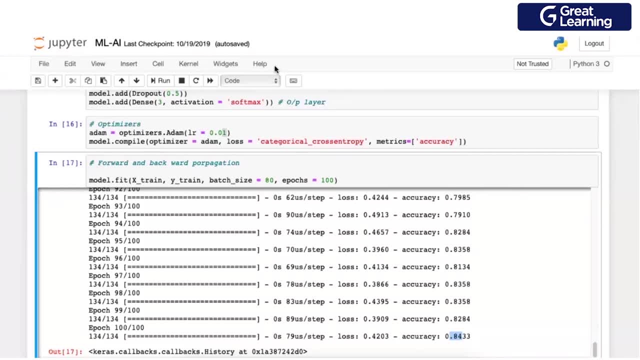 we will run basically from computer. next one, all right, so please understand each and every factor here and don't miss any. my new details also any issues? anything? drop a no post on your group. I will try to answer that. yeah, and what I showed you today was very simple. next, 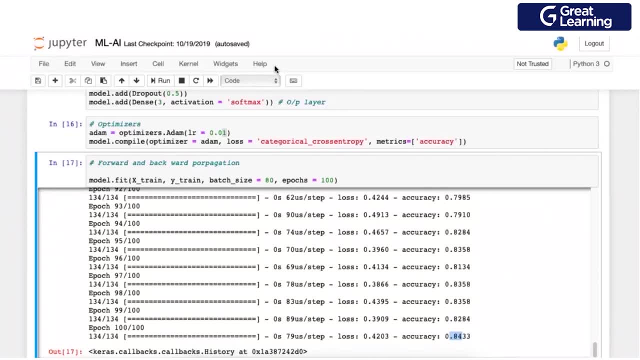 session will scale it up. we'll try to design more complex models. okay, I'll show you something on to text and image processing also right away in next session, so that you get a good feel of not only categories and regressors but also other- but I'm not sure how many of 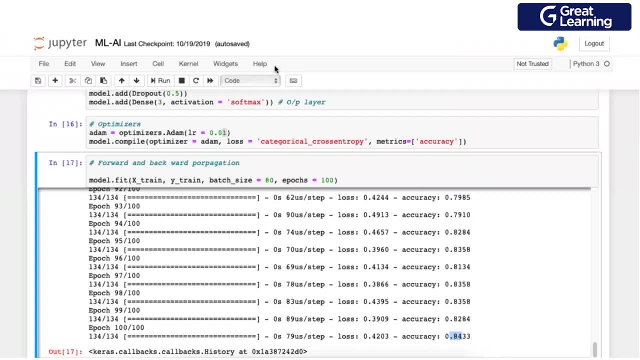 you will use this for regression and categorization was already. you have a min for that, so the edge comes in something onto image detection in face detection, expression detection, sentiment analysis. but anyway, we will not use neural networks for this detection, right? we use convolution only, right? no, no, no I. 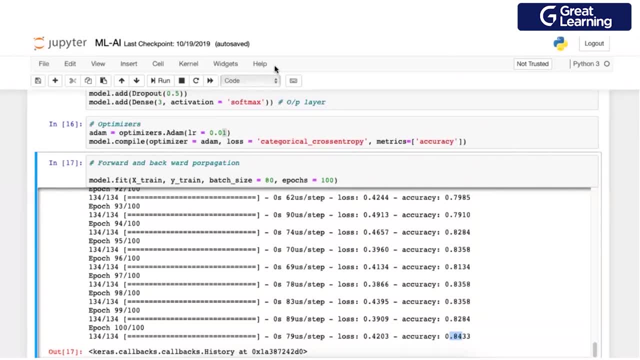 will show you so your first project for neural network. no, you will make you use KNN for image processing or image detection. okay, so, yes, and you are perfectly right, convolution is the default one, but we will make you use neural network to detect an image and, opposite to that, we will make you also. 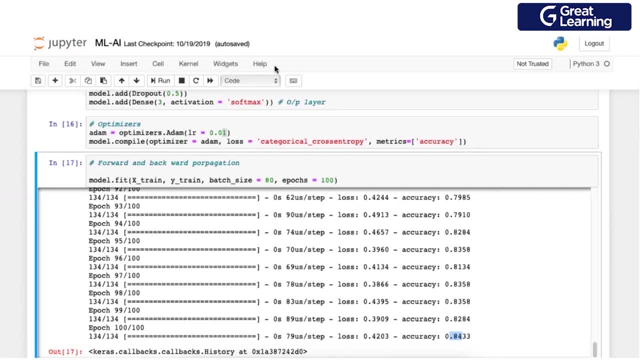 do KNN to protect the image. and then the reason: we do it just to show the difference between ML and D. okay, you can use VM to detect images, or to I can say not detect, I will say classify images. if I give you a number, seven, let us say: 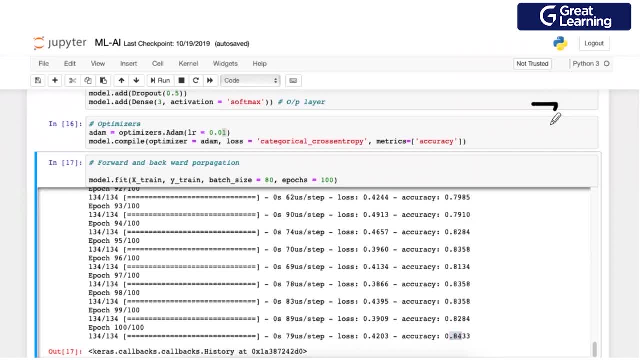 you have an image screenshot, and that image has something like this. I can use SVM to identify what it is and display this. this image, it represents number six, but convolution is a better way to do it, so we will see in next module why it is better. what makes convolution better? 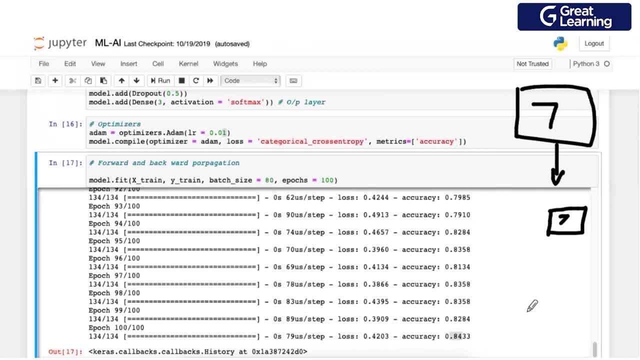 than neurons. and even we have better version than convolution. we call it RCNN- regional convolution neural network. we have more better version than that. we call it YOLO, and it is still evolving. we are not happy with that. also, it is still evolving, so we are going to do a complete 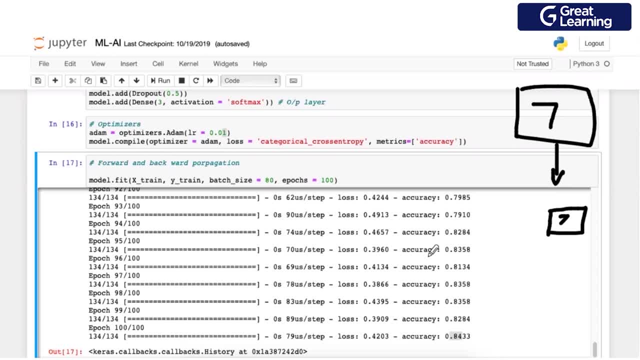 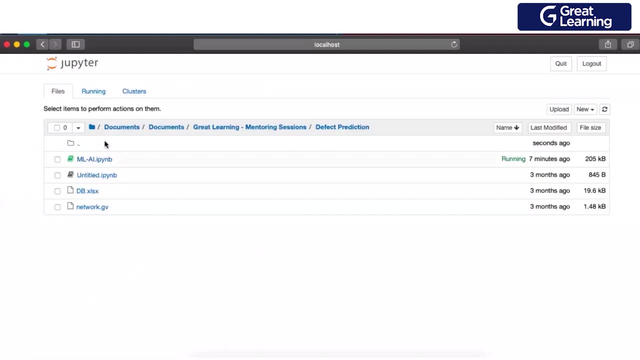 8 week session. 8 week module: on to computer vision. it is a very long module. we will spend 2 months on to that. alright, perfect. so I think there are no questions, let's move on. so, Ashish, I will take you to your code and I have a very similar. 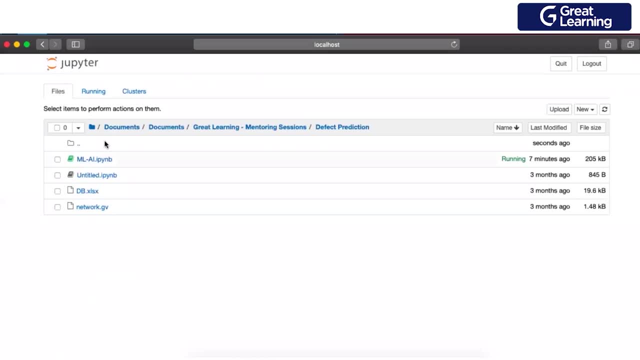 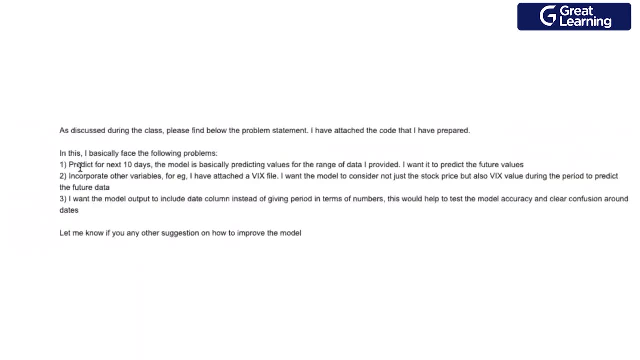 code to that I can help you to give that. it also does the stock prediction only, but I will give you the next 10 days for the range of data I provided. I want to predict the future values. so you are using LSTM here, right? I saw you have used LSTM, right. 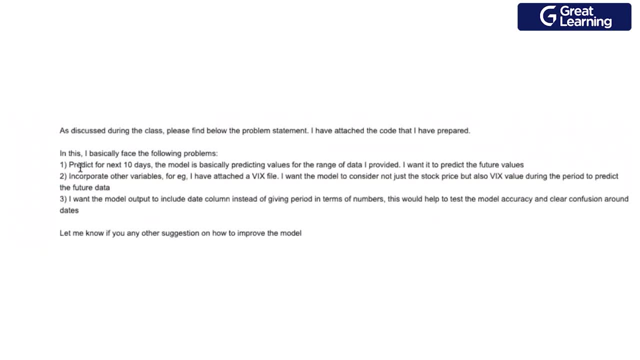 so is there any issue here? because I did not run it through as of such. so, if you go to the bottom of the code, there is a chart that I have made it. if you go to the bottom of the code. yeah, is it correct? yes, yes, yes. 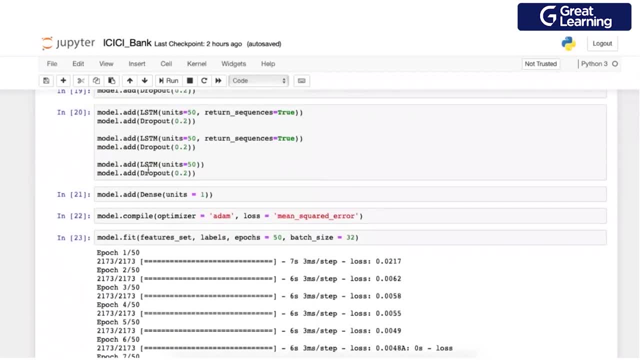 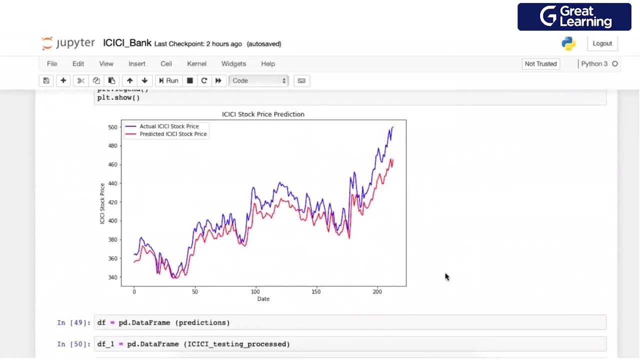 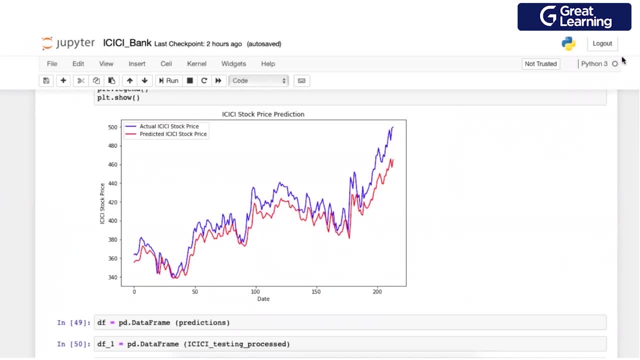 so, for example, let's say, on a day for 5, the Blue Line, if you see it peaks out. after that the Red Line also peaks out. so it is happening in delayed format. it is just doing just predicting what has actually happened, not predicting the future. 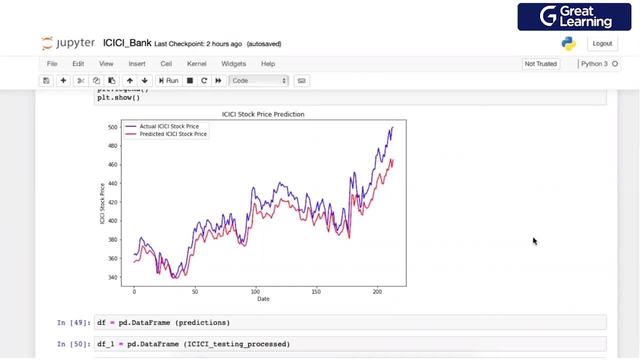 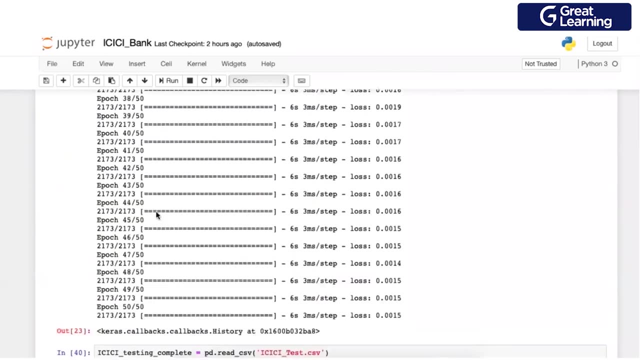 Correct, Correct, Correct. Got your point. Got your point. Okay, Then I need to analyze the whole code step by step. Uh, why it is happening? So are we missing any values here or the network is issue? We need to check this. It was. it's a very complicated Okay. 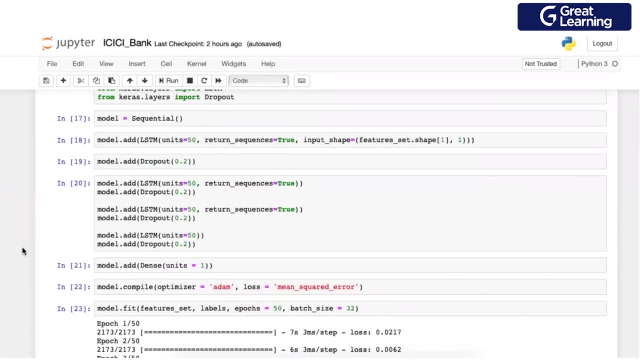 I have all the values of the data. The data is, but I'm not sure about the code, because I just bought it from many places and it had to put it together. Okay, We'll do one thing, Ashish. I have a solution for this. Meanwhile. 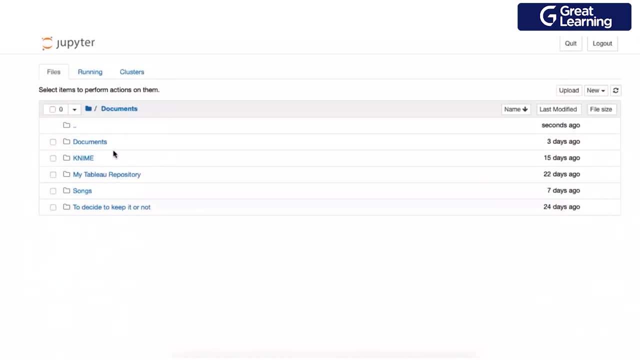 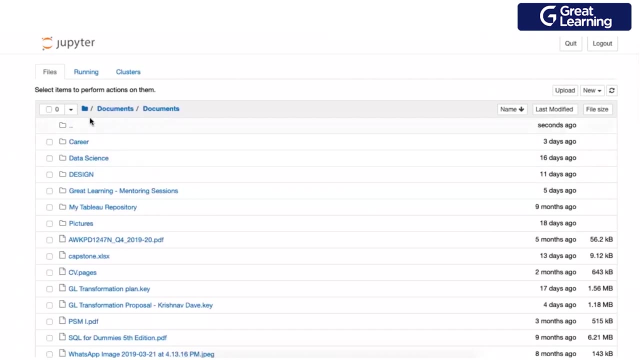 I work on this, correcting this code. I will give you one more code of mine. So just between us. Okay, So you can just modify it and then use it. Um, give me a minute, Where do I have it? I have it. 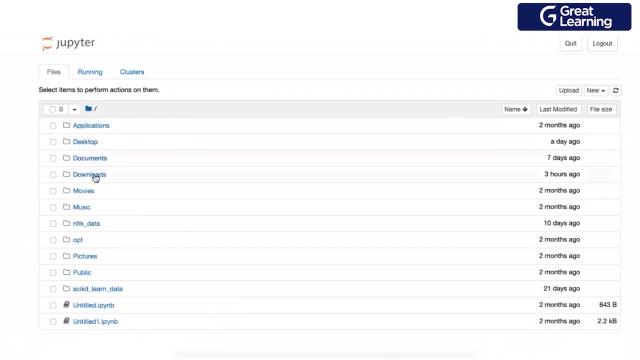 LSTN CS. So I have something like this which predicts stock markets. Yeah, It's a little customized code, So it is almost similar to what you have done, Except, what do I have here is I have got a huge amount of corpus. 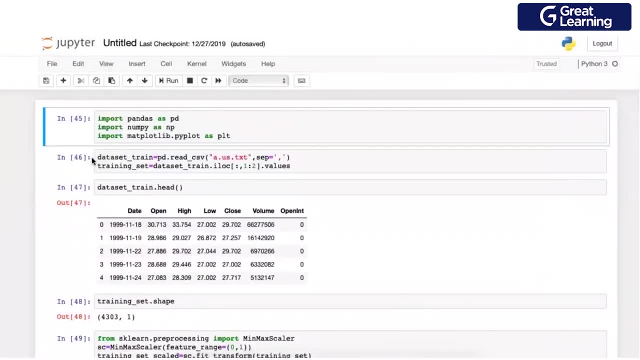 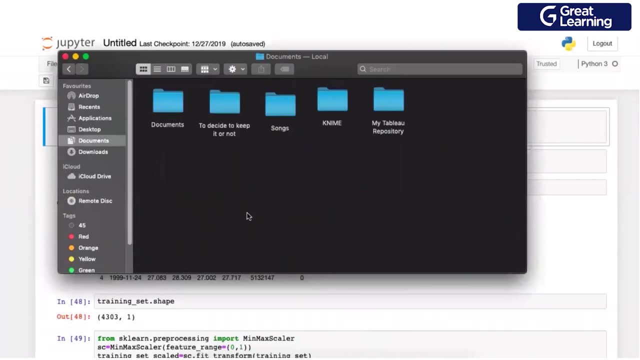 Now, if I look, if I show you the corpus that I have, might not be exactly the same as yours, but you can use it One minute, Okay. So I have a lot of corpus here and I'm going to show you the corpus that I. 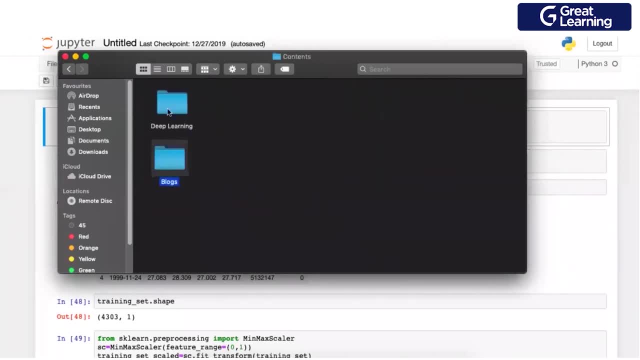 have. I'm going to show you the corpus that I have. This is what I have, Okay, And this is the way each company's talks are there, Okay, So what I will do is I will share this code with you. It is a self-explanatory code. If you know, LSTMs. 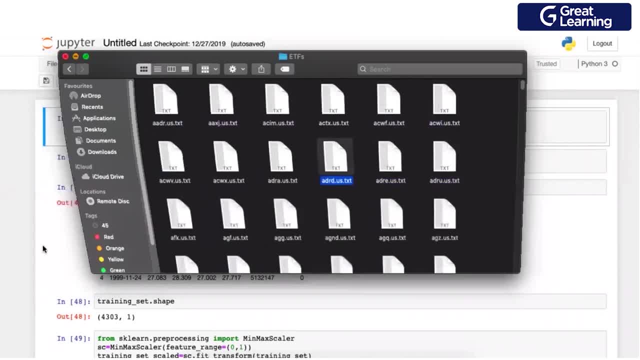 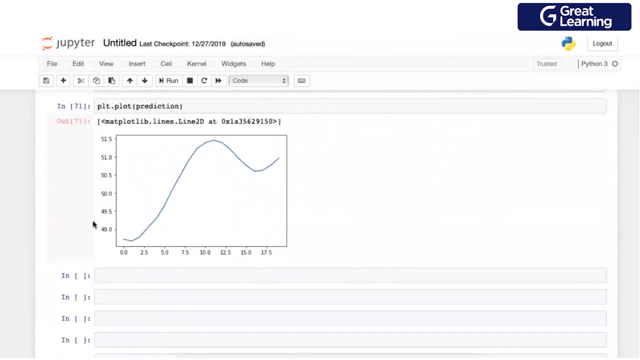 then I don't think so It'll be an issue for you. What I am getting is: I'm getting, yes, next 18 or 20 days of prediction. I'm getting it. So this is my prediction basically: Yeah, So prior prediction: I'm going to get it on the next day. 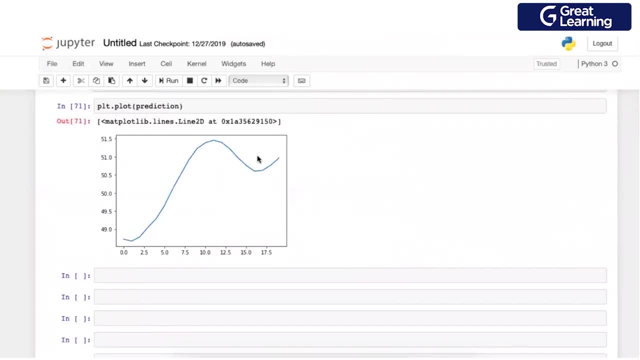 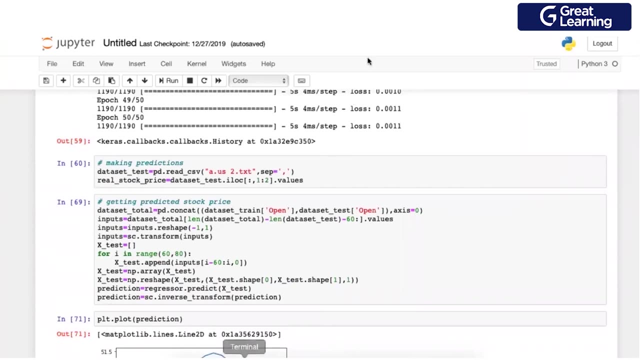 I'm going to get it on the next day. So I'm going to get it on the next day, Okay, Okay. So that's it. Okay, right about if you are able to fix, take some content and fix it Parallelly. I will work on line by line of this, because I 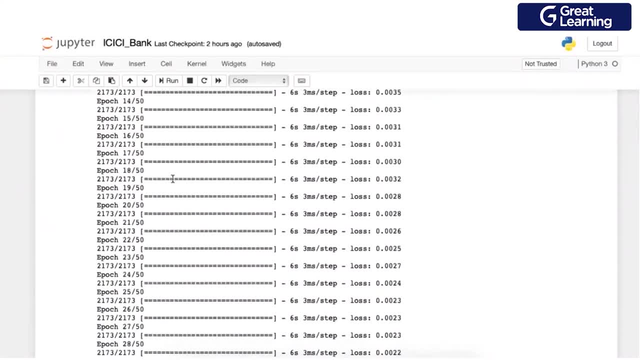 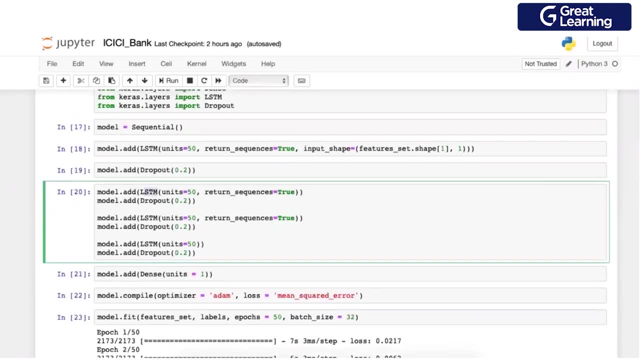 need to understand the whole flow. First of all, it's not a simple, you know task. Again, I need to break this up Because usually what LSTM do is LSTM has two parts. I don't know if you know this. LSTM has two parts. You can use LSTM for encode and then decode. 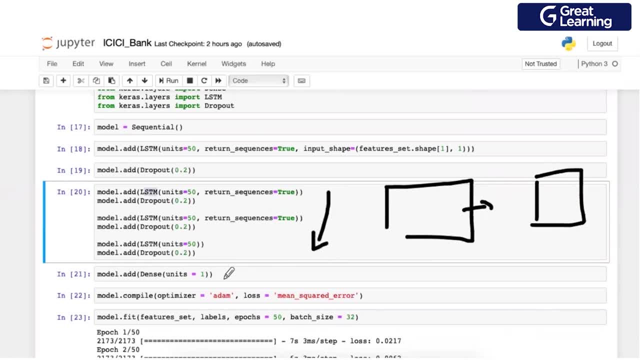 I'm not sure if you just used it for encoding part of it or have we put a decoding layer? I think it is just an encoder, basically Yeah, Let me optimize your code and then let me analyze why that 10 days, or whatever gap you are seeing, is happening. 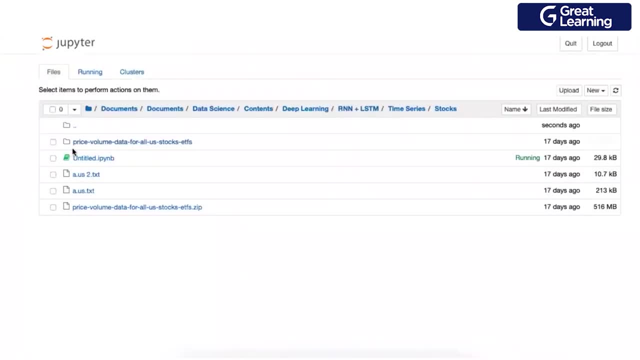 Yeah, One more thing I want to include in this code that I think would be really helpful is to incorporate other features. Other features Would be able to help us build the stock price better. So if we can include it, because most of the LSTM code that I saw on the website- 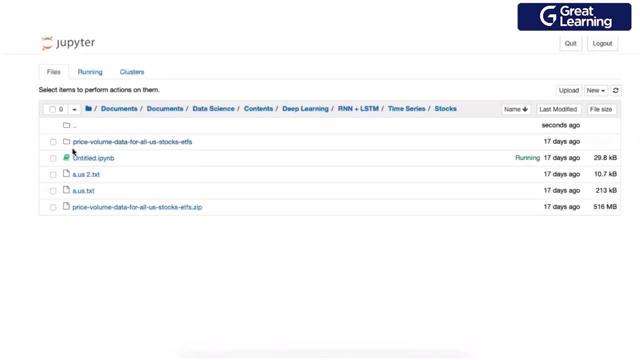 they only inflicted on one value, either on the closing value or opening price. So if we can include other features that would be able to, that would be. that would help us to build this price much better. Okay, perfect, Let me check it out. Okay, so I'll do one thing, Ashish. 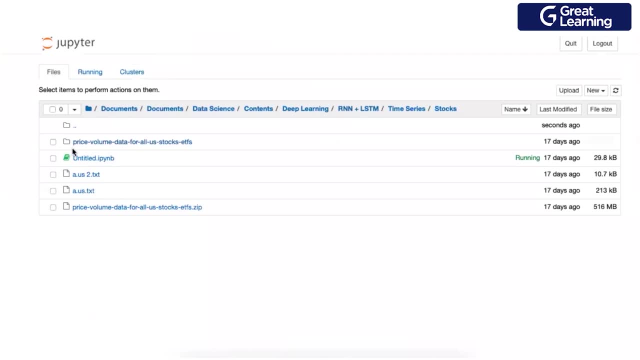 first let me solve this problem, because it looks like to be a complex, I'll not say Very complex code, but yes, when LSTMs are in, I'm sorry, when LSTMs are involved it is little complex. So first I need to understand the design. 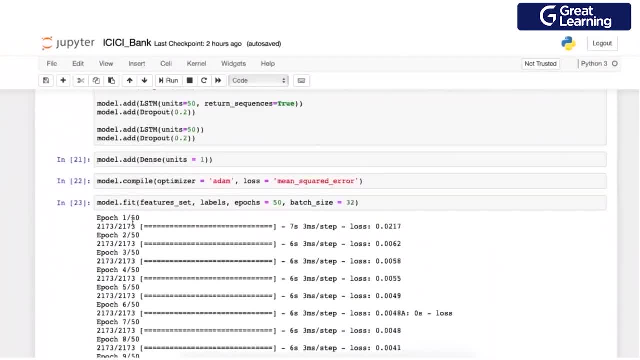 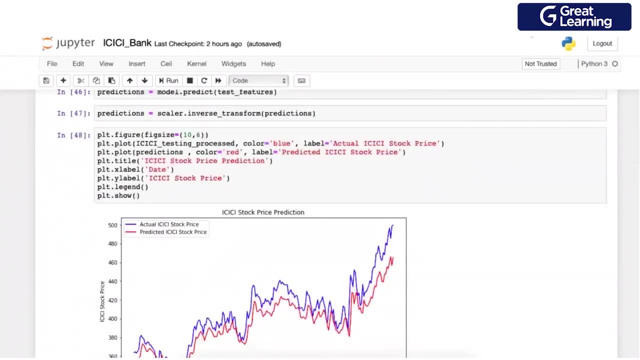 of the network. First of all, why it's 50, 60, 70.. What is it making this way? And probably, once I get hold of it- I don't think so- It should be big trouble editing this. Okay, cool, I'll share this with you, My code. 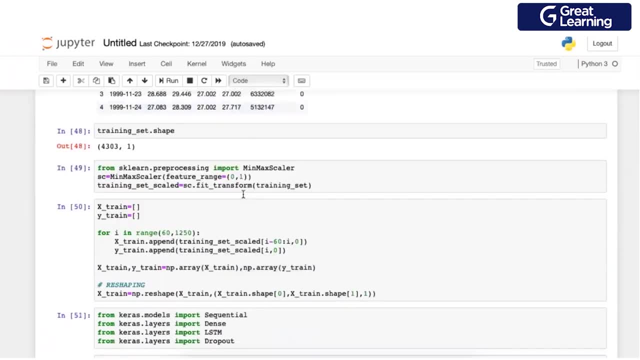 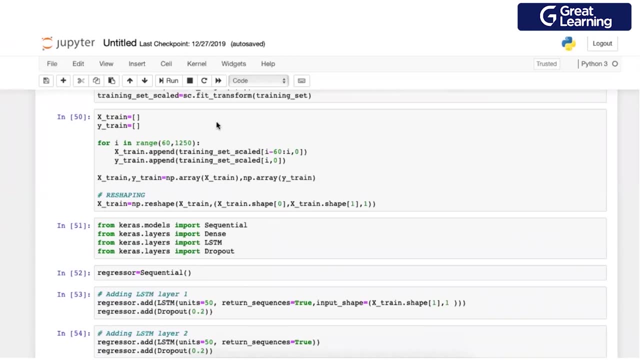 of LSTM predictions. Check it out. Okay, Yeah, All right, Perfect, Yeah, Ashish. one more thing. I just a reminder. There is one guy called Ganesh who has just joined our bash today. He is email He has. what do you say? 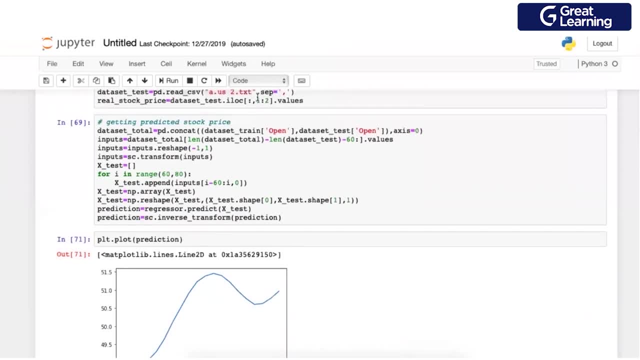 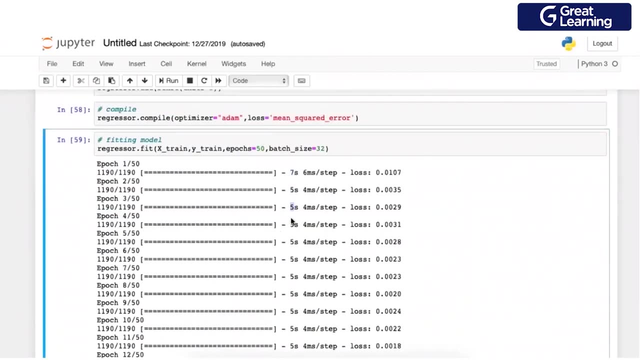 This is a little difficult way to do time series, Because tomorrow something changes. No, you have to train your network and I don't know how much time it took for you. I think the epochs are not that heavy. Yeah, no, it actually. 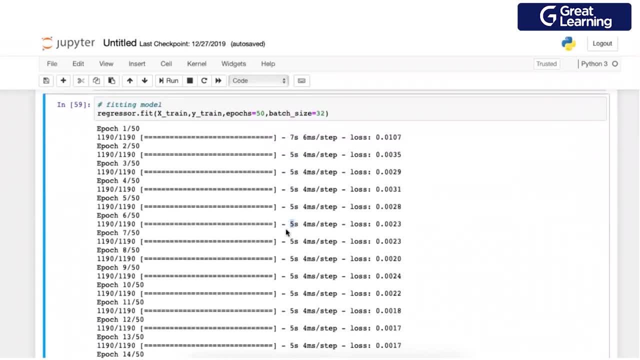 took me. It took me around one hour to train this code Correct. Now, just imagine tomorrow If the content- back-end content- increases. no, the training time will also increase. So first option: what I would request you is if you are deploying this somewhere or if you're doing for your. 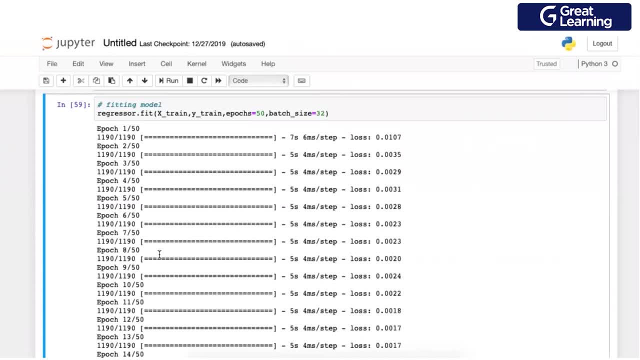 own knowledge. perfectly good, This is very good. But if you're deploying it just to deploy it eventually, the intention is to deploy it eventually, So just check the cost of it. cost in the sense because whenever you have, you have to retrain your model. no, you have to retire your initial model. 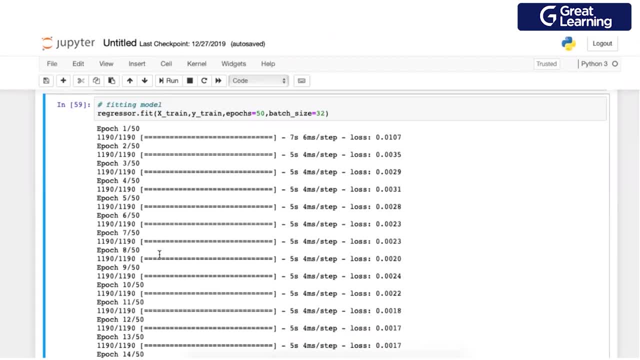 first, Then you have to pull it back, and then you have to retrain it and then push it back, So that non-operational phase. no, you have to calculate the cost for it. So if you are okay with it, no issues. First option should be. 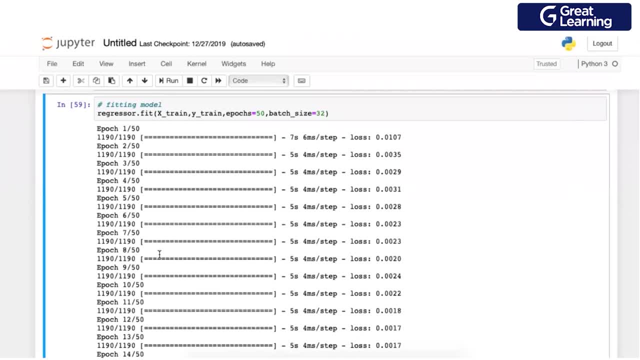 ARIMA. Second option should be LSTX, to be very frank. Well, the reason I train it on a daily data is that because it would not involve too much cost in execution, because I didn't take the manual decision after it predicts the data whether So my intention was actually. 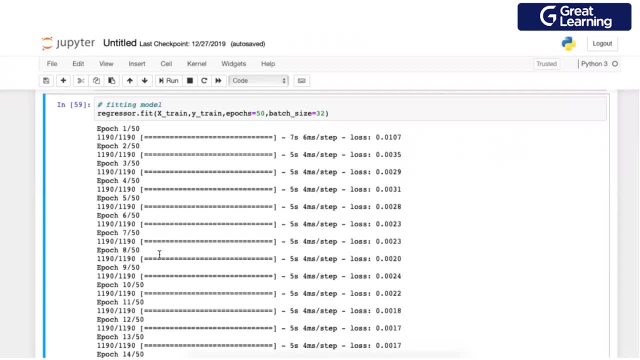 to do it on a live data, on a ticker by ticker or second by second data. So that would be- I'm not sure, because if it takes a one hour to run the code it would not be possible to do a trade on that kind of data on the. 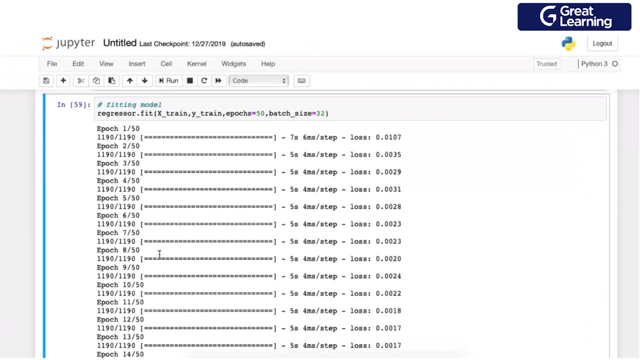 live data. So that's what I was thinking. So is the deployment different from what we are doing? So it's first we are trying to create a code, once we are satisfied with the code, How the deployment takes place. How the deployment takes place. 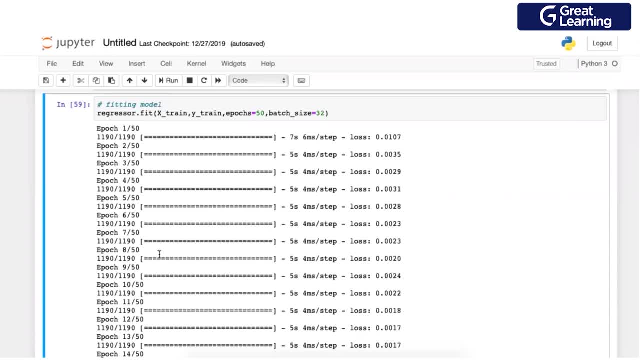 Where do you want to deploy this? Where do you want to deploy it On? where Deploy it? on my broker account. So, using my broker account, I would say, yeah, it's a web or web? Okay, I will show you right away. It's a web, right? 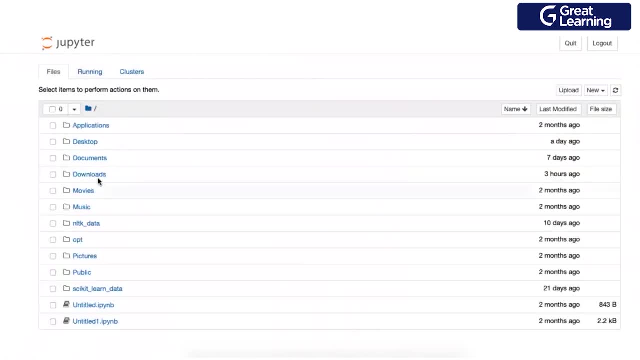 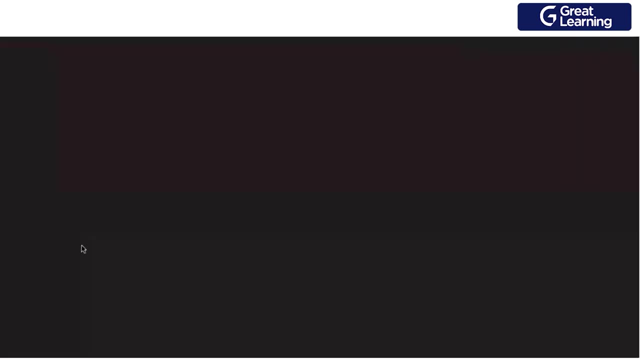 Yeah, it's a web. Yeah, it's a web. Let me show you. Yeah, let me show you right away. This is not our LSTMs, but, yes, this is one One minute. So we use flask, basically Ashish, to do this, and I will give you. 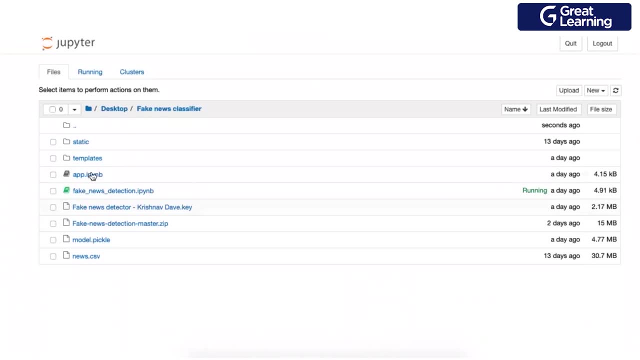 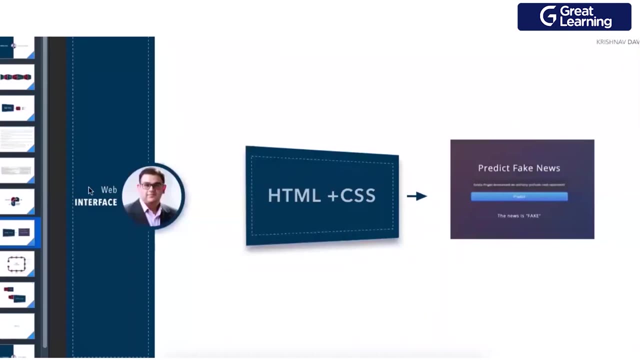 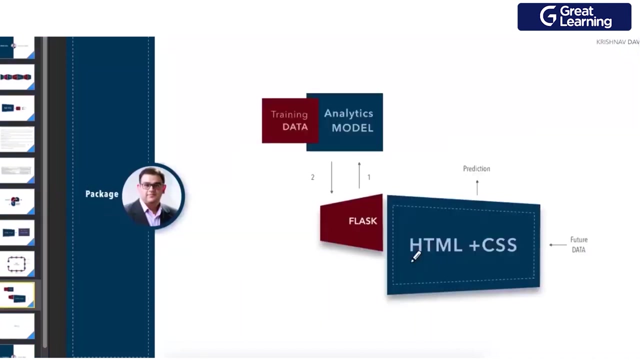 this code also so you can deploy it immediately. and this is my app. So the overall architecture, if I show you, just give me a minute. So the overall architecture is that my intention is here to make HTML web, which I have done it. Okay, so this is my HTML and this is my CSS: some styling. 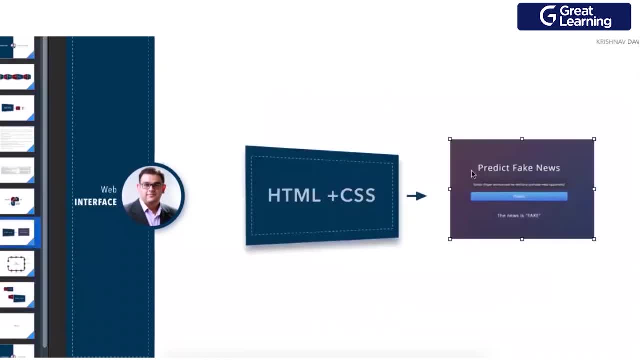 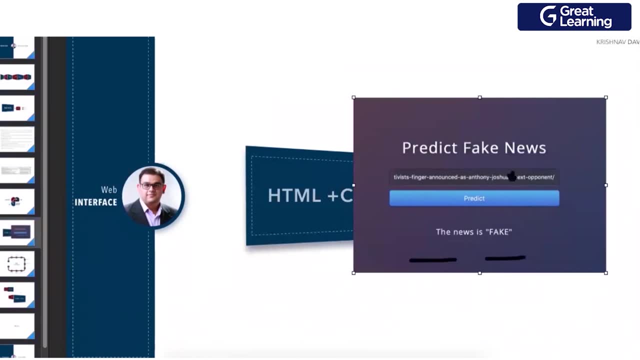 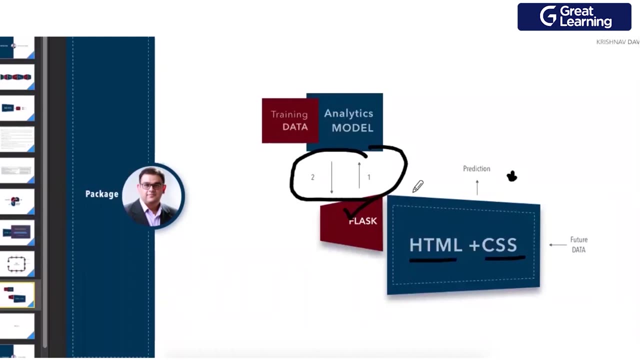 I've done to create an interface which looks like this: Okay, okay, and this particular thing is very simple. You have to just put a URL here. This URL will be given as an input to me in my code, So I use flask to convert whatever I'm talking in python. with respect to 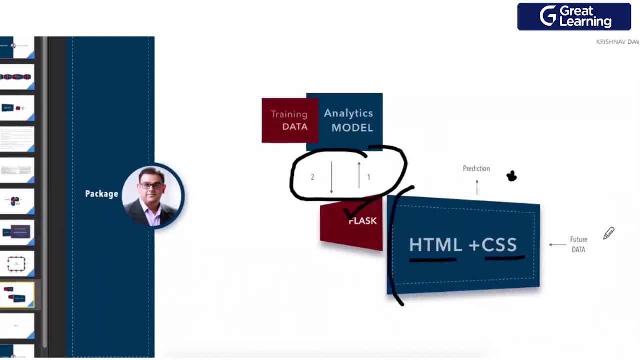 what HTML and CSS understands, very simple. So I am taking a link from a user- Why a flask? and inputting it into my model, which is pre-trained on some kind of data- It's a neural net model, Okay. and after that I'm saying: I'm replying back to the HTML using flask. 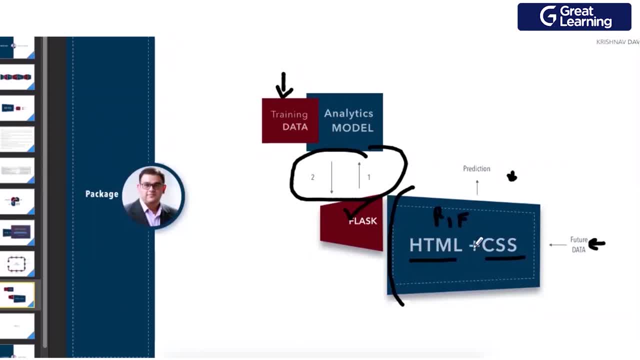 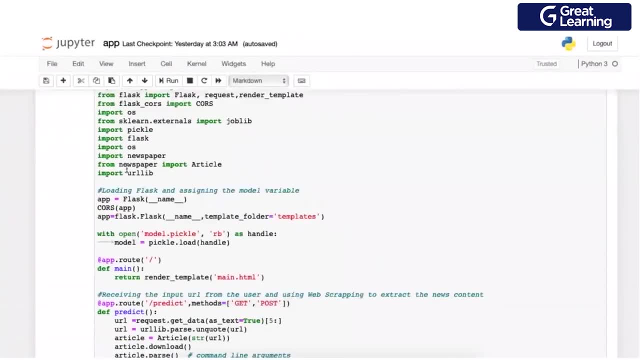 saying that it is a real news or it's a fake news. That's what we are doing. All right. Now, how do we do it? Let me show you the code. The code is very simple. Let us say if I can run this before that. 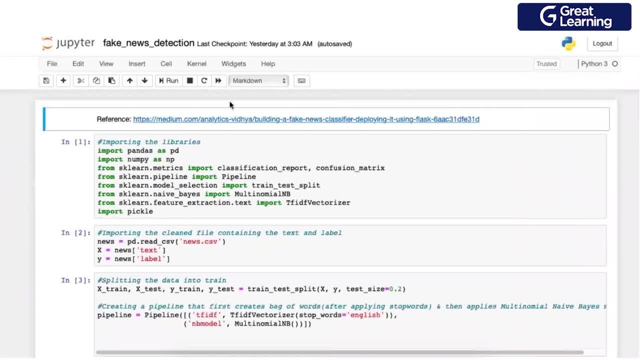 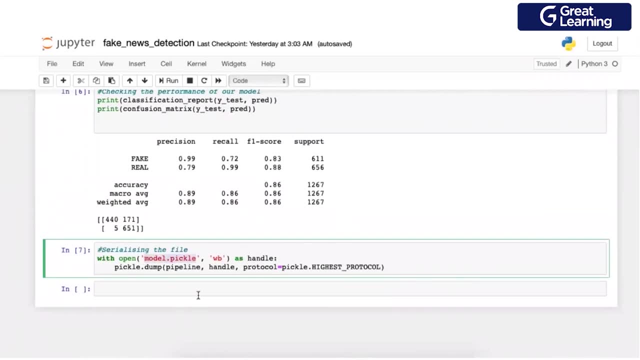 Yeah, So this is the flask app. So there should be one application which you have to make it after you are confident with your model. What you have to do, it use of pickle it. If you see this, this is called pickling. 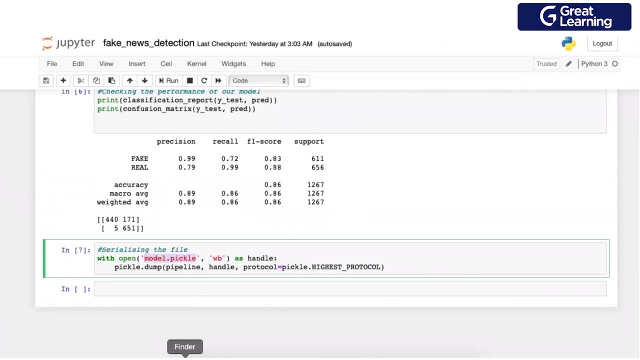 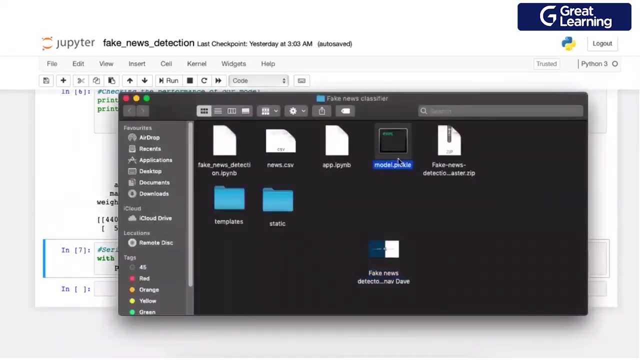 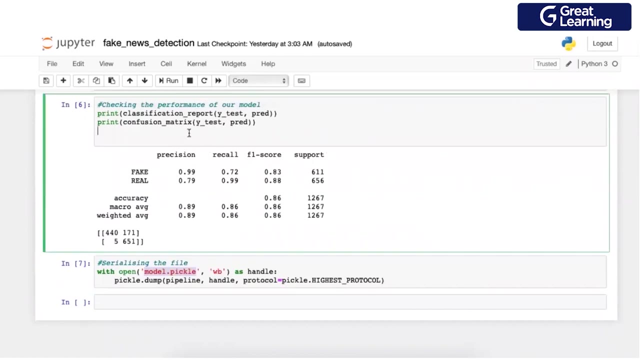 Pickling is like converging your model and storing all the supporting files onto a location which can be called from anywhere. So this is my pickled package, which is nothing but my name based model that I've designed about. Okay, any model that you design. 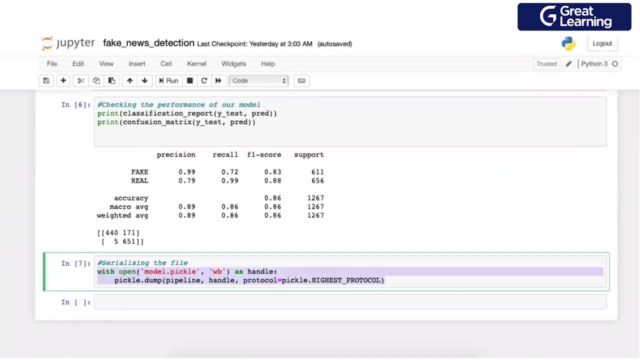 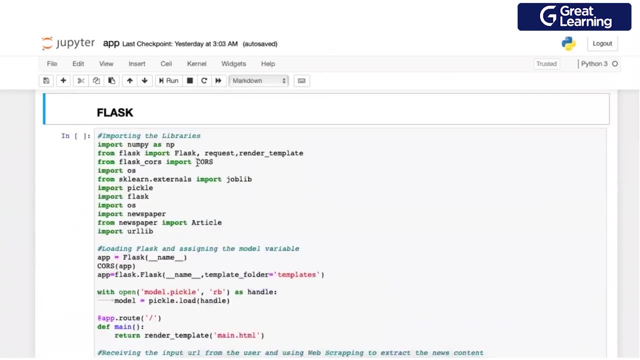 Pickle like this. So this is the two liner code which you can use to pickle, and once you run it, you'll get a pickle file like this. Now your job is to import this pickle file in your real app. So this is my real application and also parallelly. 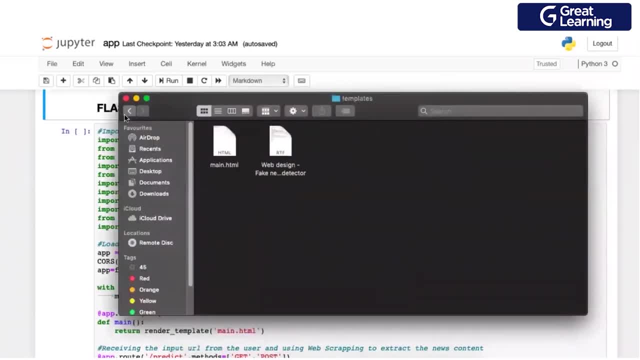 I have deployed a web page, So this is the link to my web and is the CSS which I have written on that, basically some Styler. So whoever is handling your application will be having access to both of these where your website is hosted there. 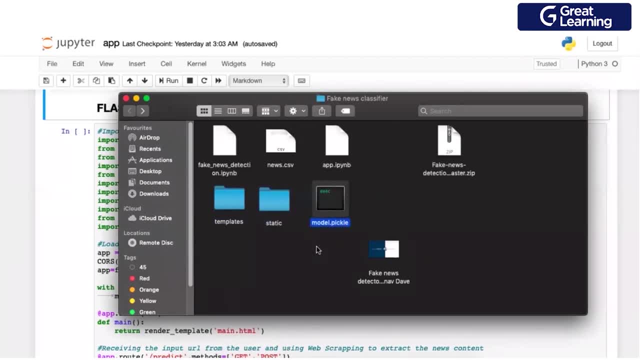 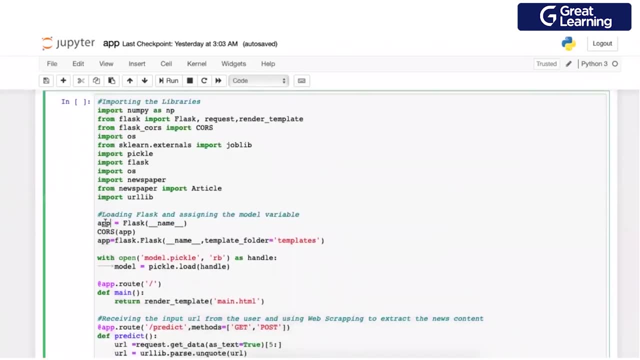 You have to go and drop this Pickle file, basically, Okay, okay, Along with the file There is a code, So this is what we call it as flask. Now, what does flask do? is flask allows me to create an app inside that app. 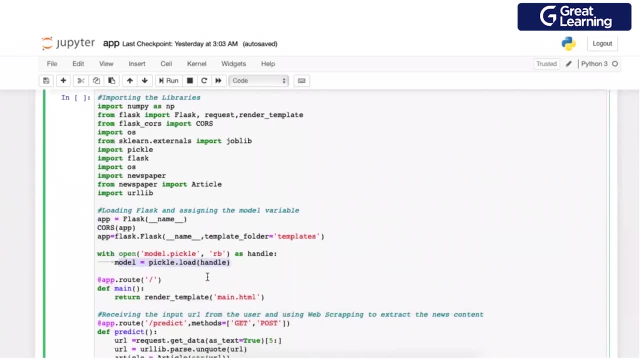 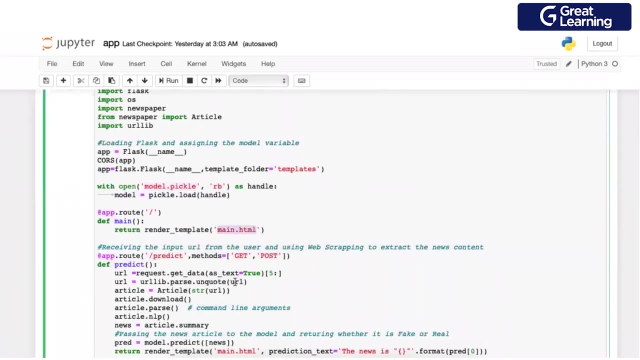 It allows me to load my model, If I have one. this is my model that I picked up, You remember. next is it allows me to connect my HTML page link here. If you have an IP or if you have any other thing, you just put it across. 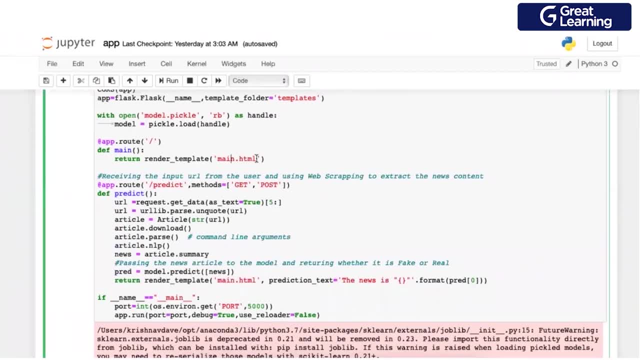 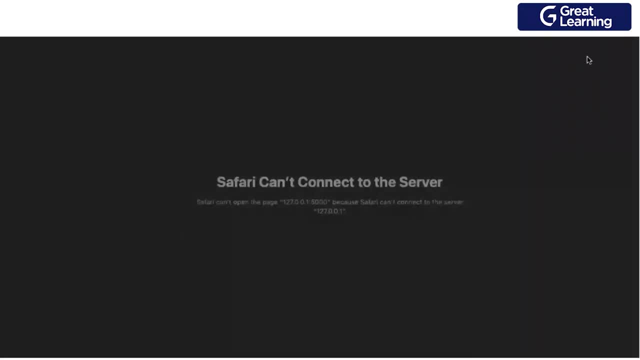 here. Next is what you want to do with it. So, if this is the HTML page, what do you want to do it? So, my HTML page. what I want to do is let me run it. It is not okay. It's not active. 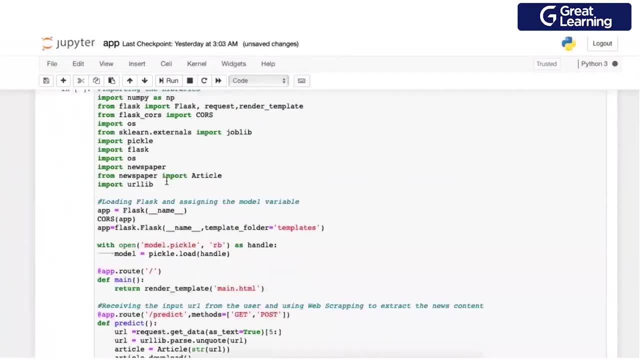 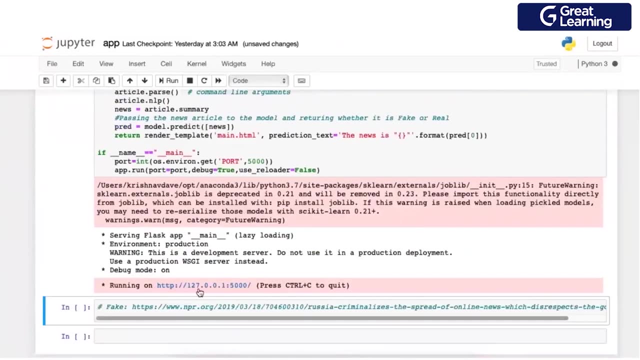 So let me run the code and I'll show you. It'll take some time, It's not that fast, But yeah, you just have to run it once. Once it generates an IP, IP is ready. Look at this. This is a fake news predictor. 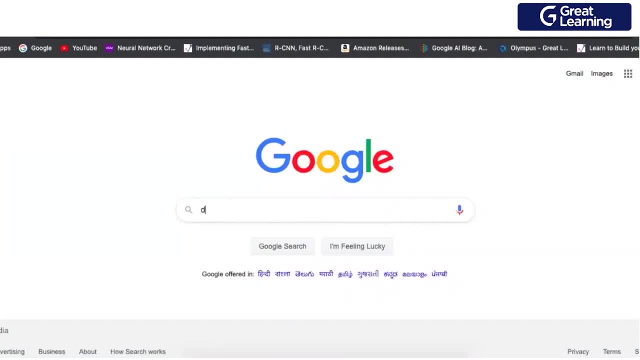 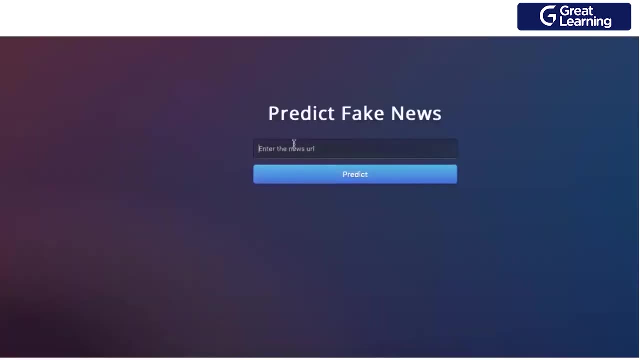 All I need to do is I just need to go and, for example, let me say I will pull some junk out of it. I have to just get the link, go to my web, publish the link here and say: predict it might take some time. 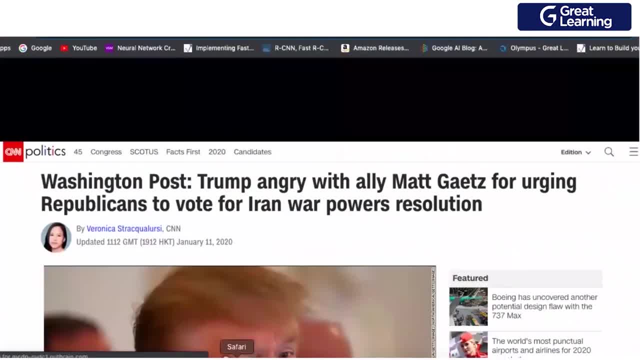 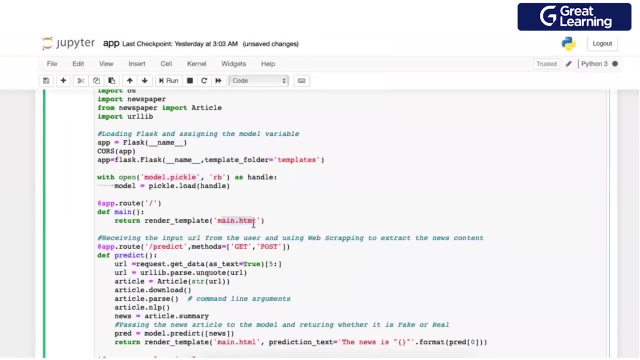 The news is real. So this is how I am telling, I'm telling my app that, first of all, this is the model that you are supposed to use from python. This is the HTML HTML page and, inside HTML page, What you are supposed to do. 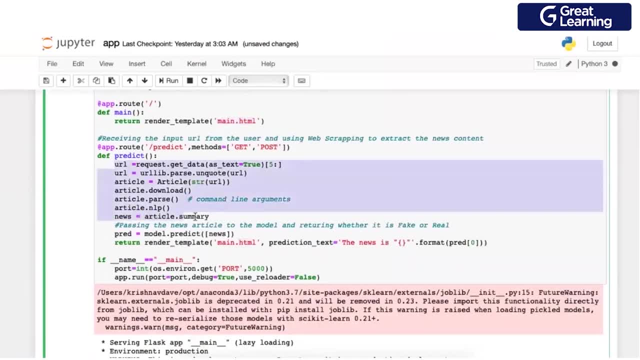 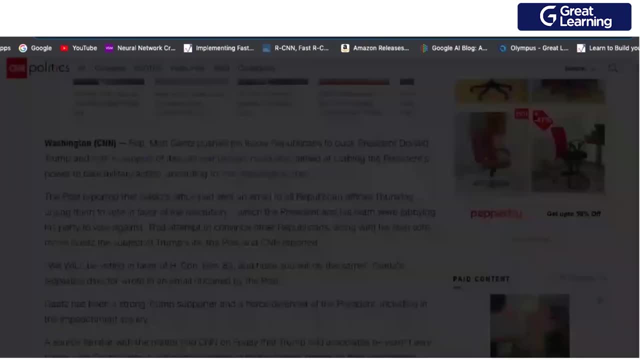 You are supposed to get my text. This is called web scrapping, If you have heard about this term. that scrapping is like converting the data on the web onto an understandable data which could be passed to a python model, Something like a data set, input data set or database. 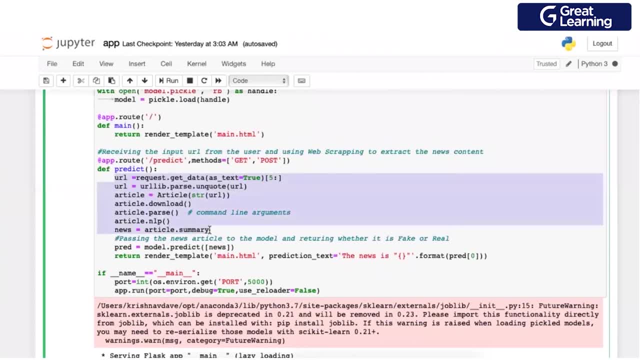 Yeah, so this is your. whatever you want to do with your inside your HTML, you to define here. So, in your case, what you have to do, in your case, you to publish a graph or give some Numbers. that logic should come here, Actually, in my case. 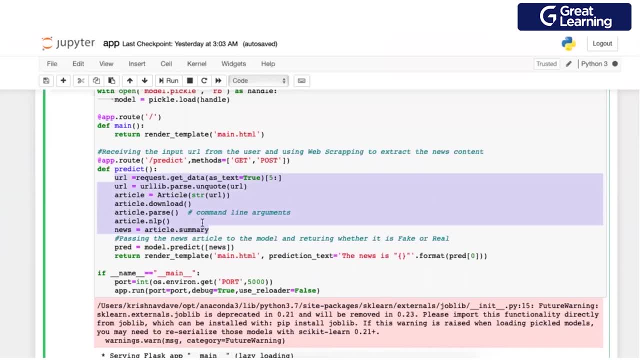 What I want to do is to give an order is, for example, model is predicting to the stock price would go up, So it to send an order to the broker account that is to buy the share, and he also send us a simultaneous order giving a stop-loss or a target price order so that he some execution.